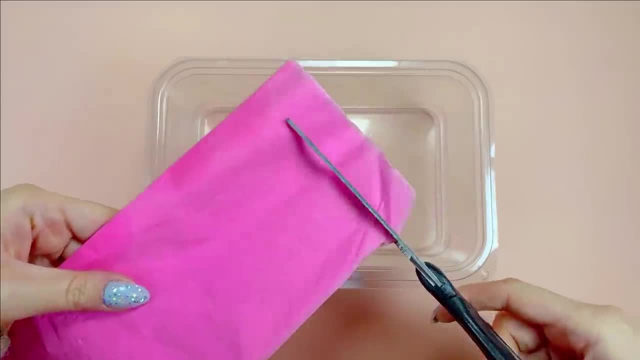 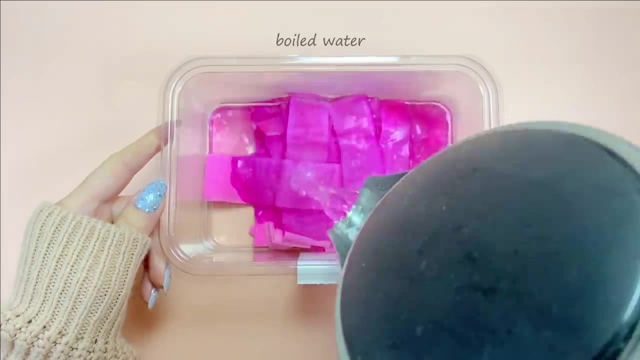 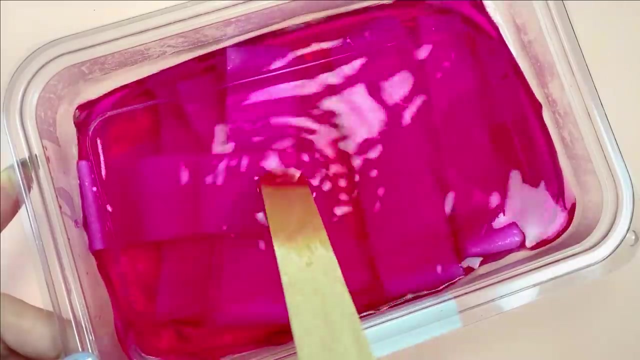 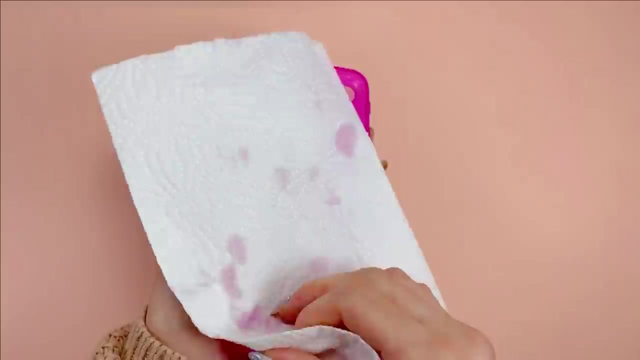 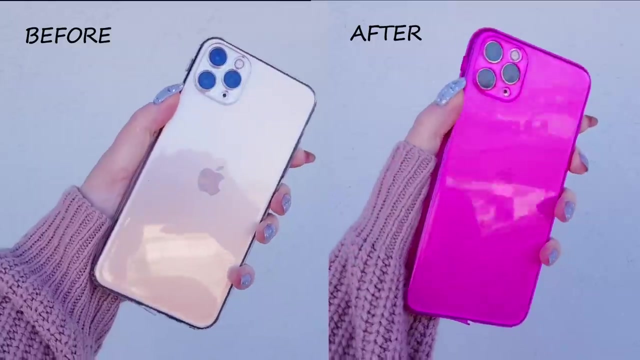 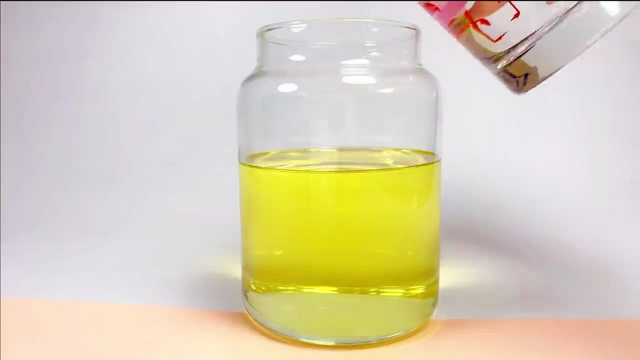 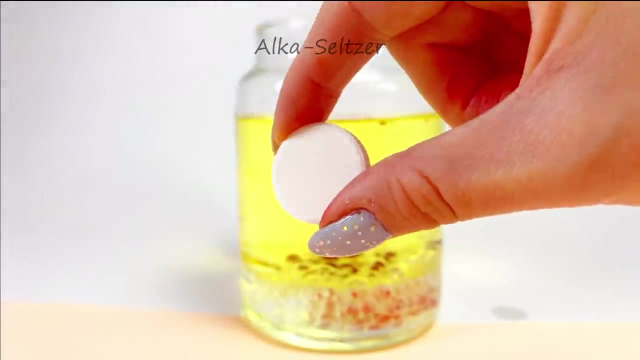 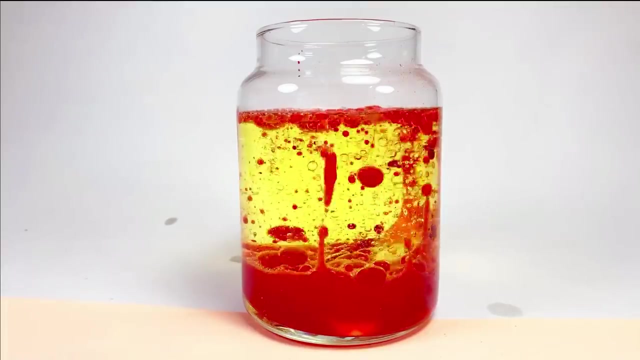 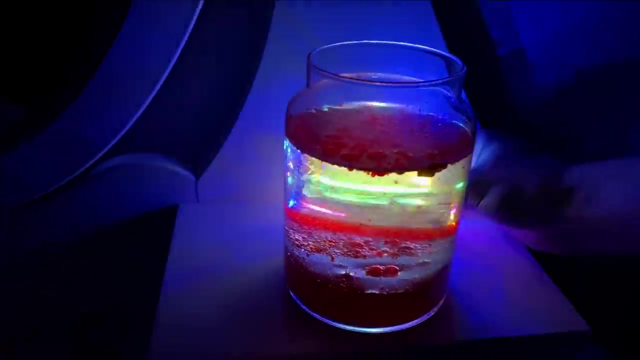 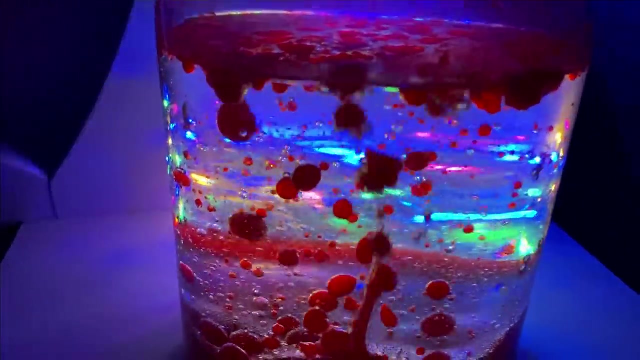 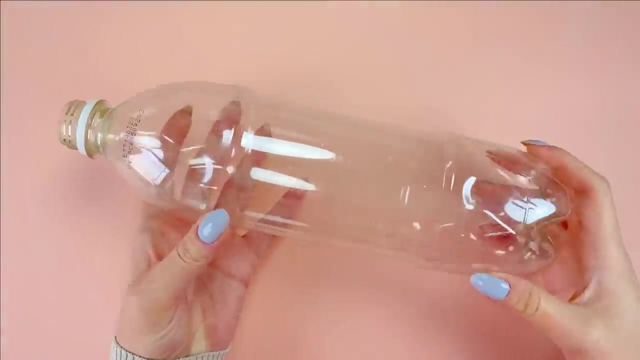 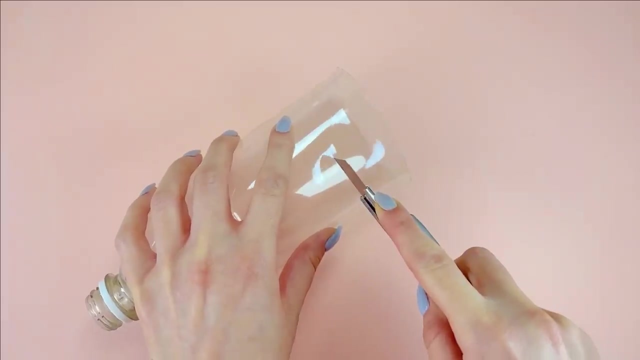 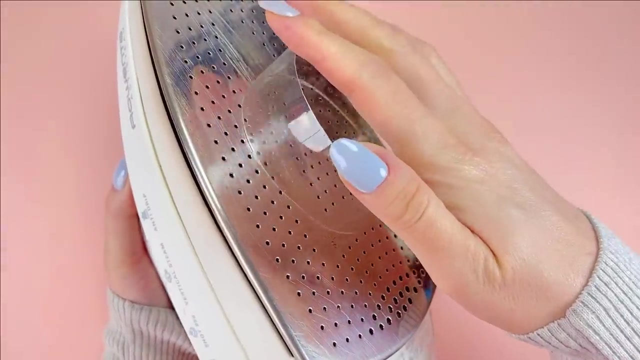 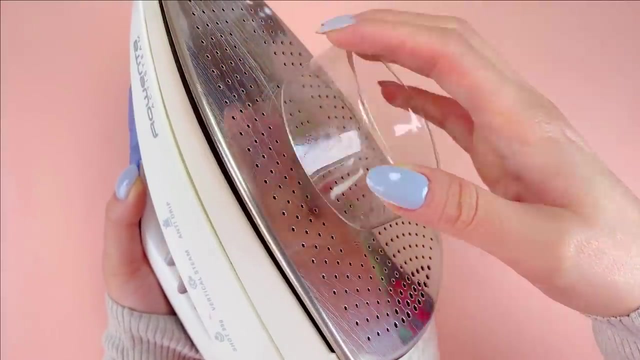 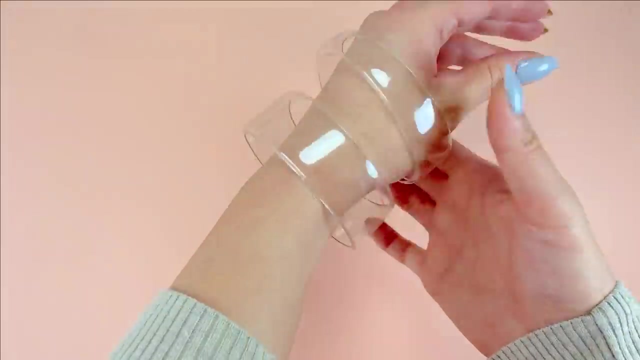 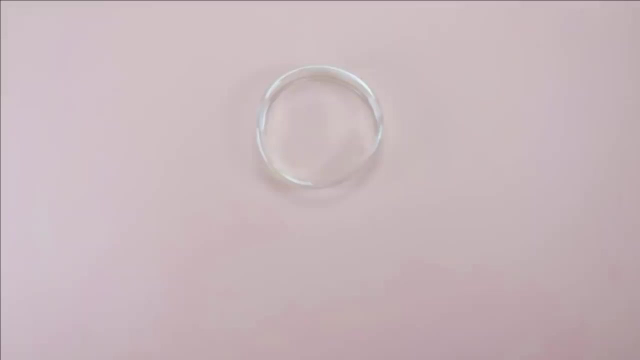 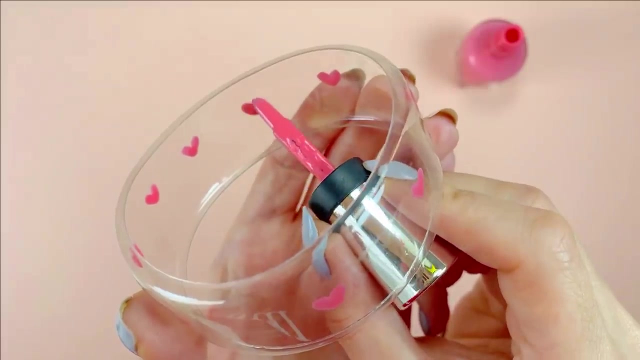 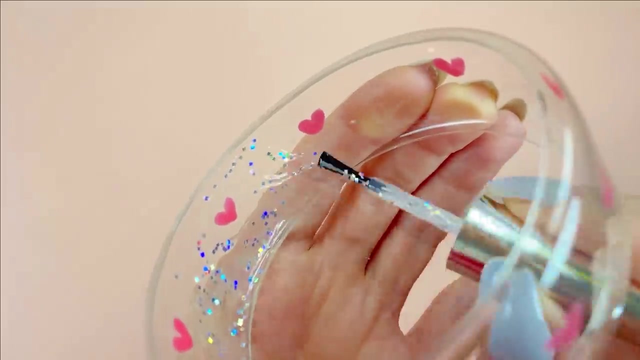 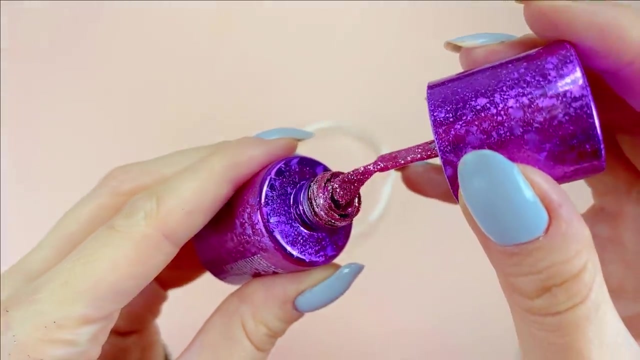 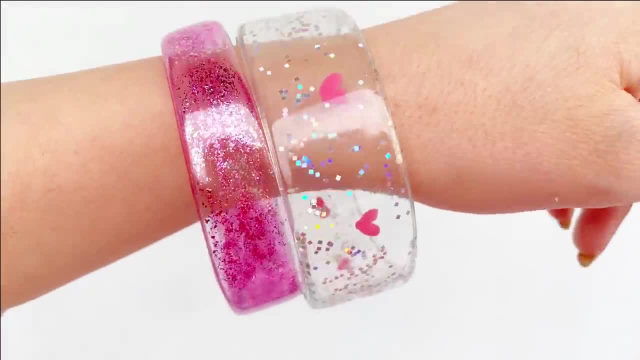 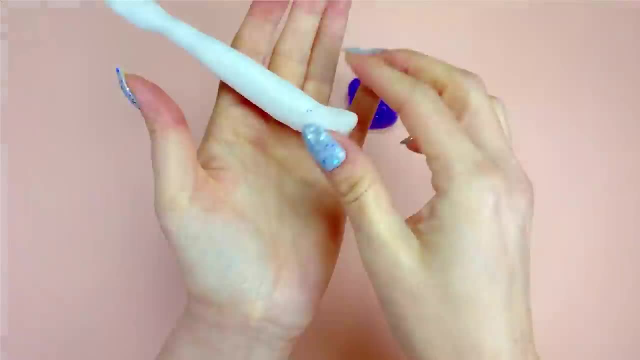 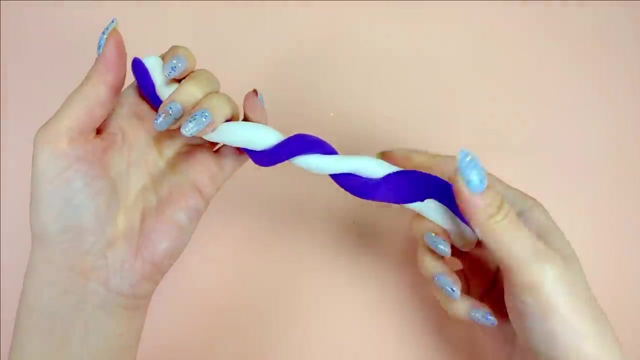 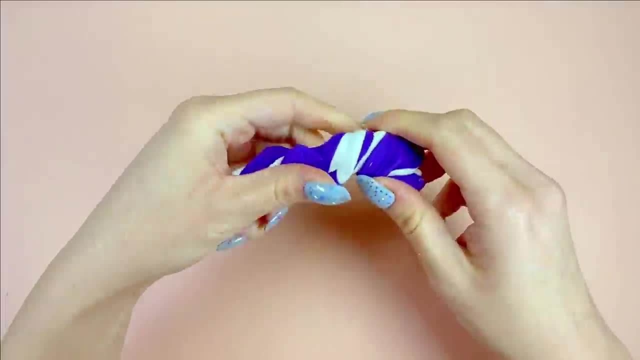 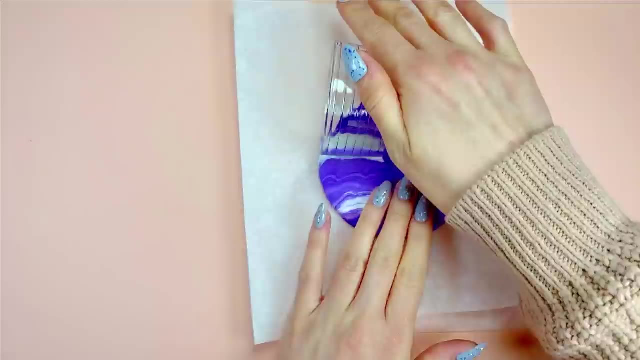 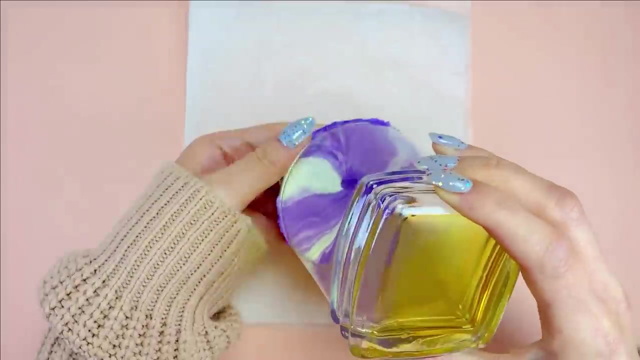 But some days I'm feelin' so down and ain't feelin' so pretty. yeah, But I go on lovin' myself cause I don't need that bit. yeah, Cause I get high and low. yeah, dust it off and shake it off. 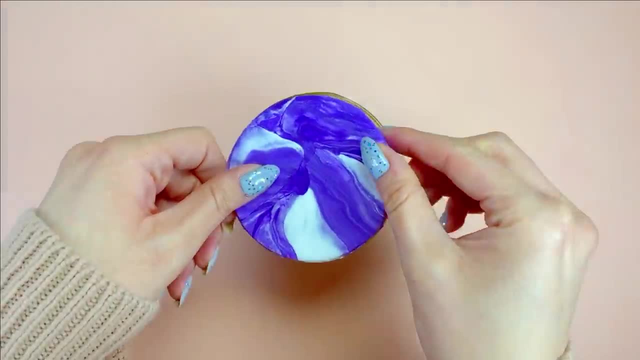 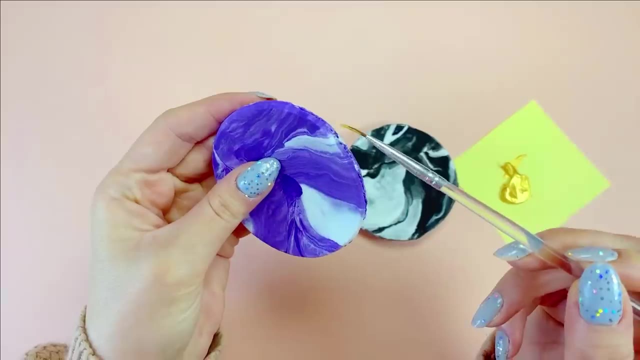 High and low. yeah, dust it off and shake it off, Don't matter what they say, I'ma, I'ma do my thing. I'ma I'ma do my thing. Just watch me. I'ma do my thing. yeah, I'ma do my thing. yeah, I'ma do my thing. yeah. 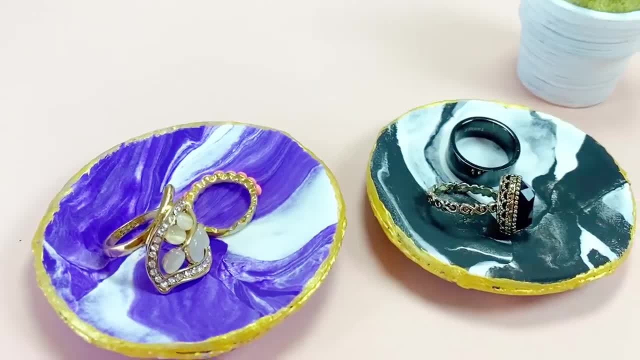 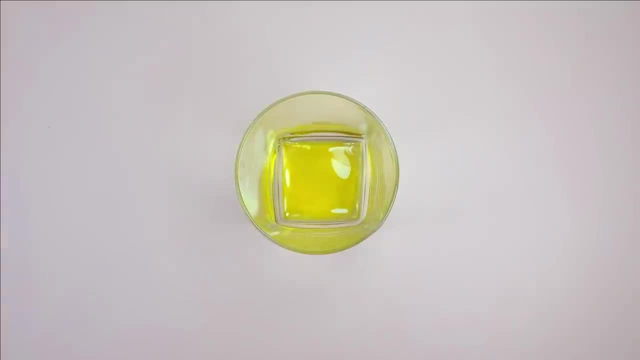 Just watch me, I'ma do my thing. yeah, I'ma do my thing. yeah, I'ma do my thing. yeah, Check my nails. they lookin' fine. put my hair back feelin' prime. Look out, baby, I'm on a roll. 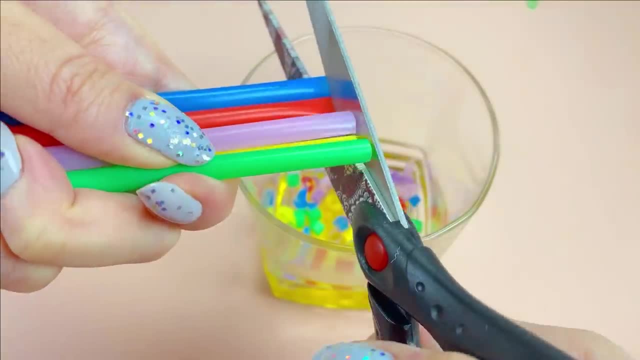 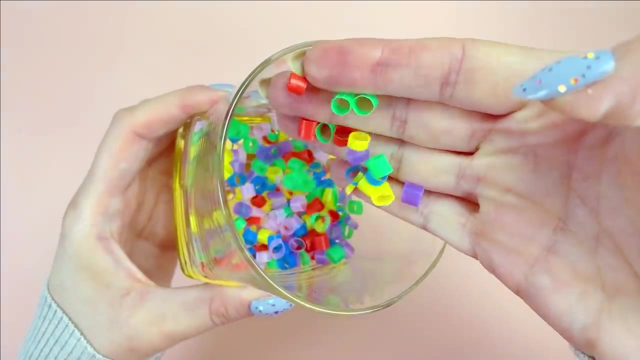 Feel the beat. it's comin' strong, make me wanna clap along. Feelin' good, but I'm not feelin' fine Wherever I go. But some days I'm feelin' so down and ain't feelin' so pretty yeah. 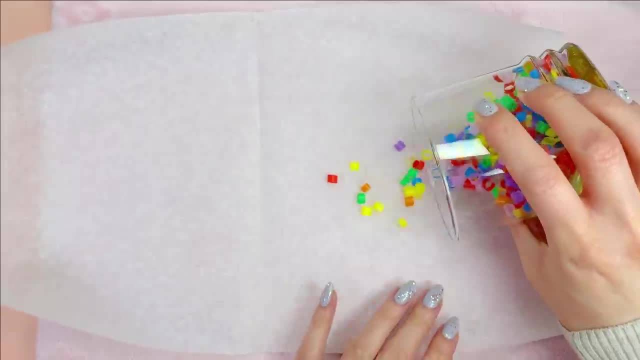 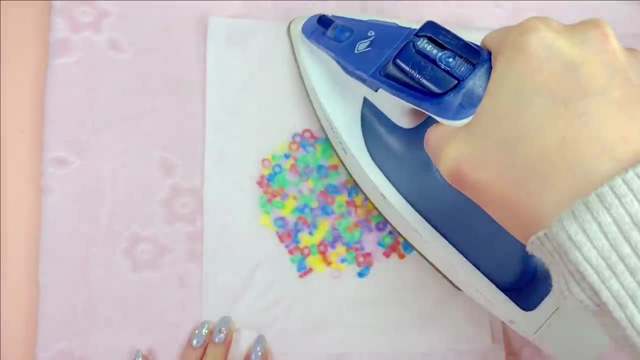 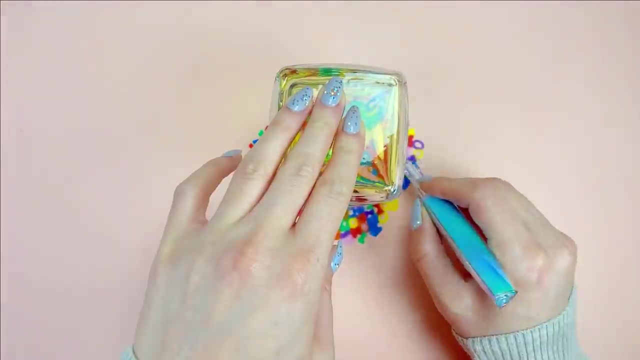 But I go on lovin' myself, cause I don't need that bit. yeah, Cause I get high and low, yeah, dust it off and shake it off. High and low, yeah, dust it off and shake it off. Don't matter what they say, I'ma, I'ma do my thing. I'ma, I'ma do my thing. 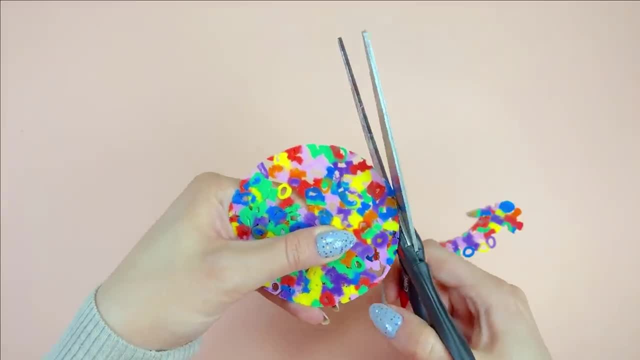 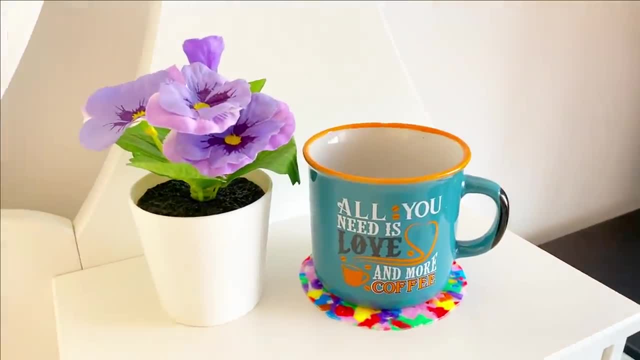 I'ma do my thing. yeah, I'ma do my thing. yeah, High and low, yeah, dust it off and shake it off. High and low, yeah, dust it off and shake it off, Don't matter what they say. I'ma I'ma do my thing. I'ma I'ma do my thing. 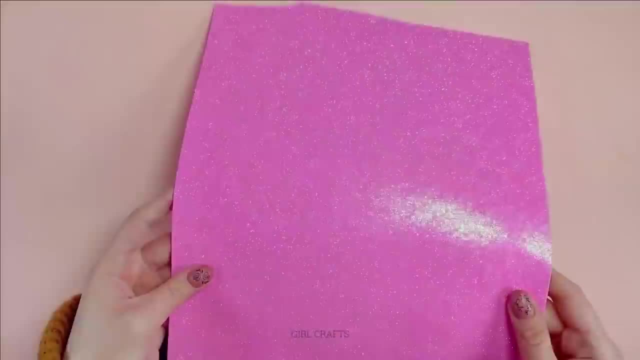 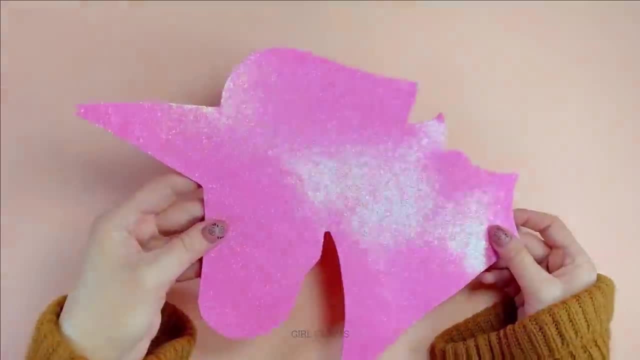 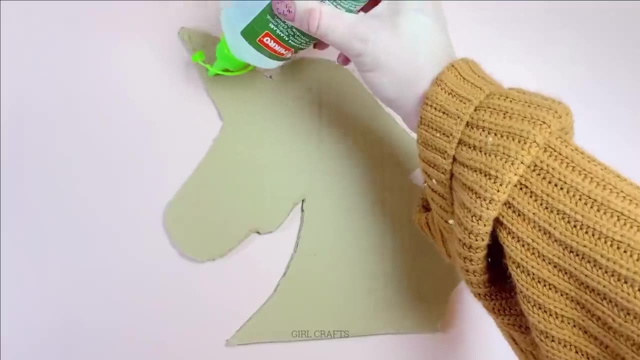 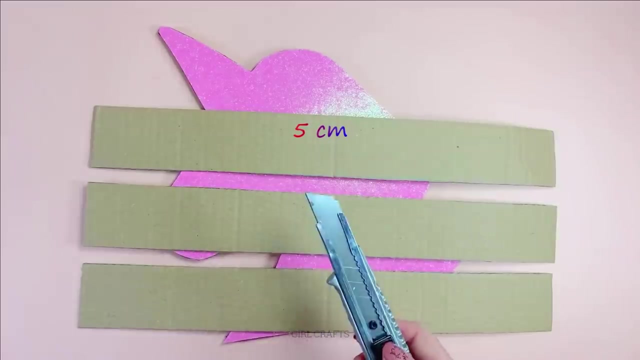 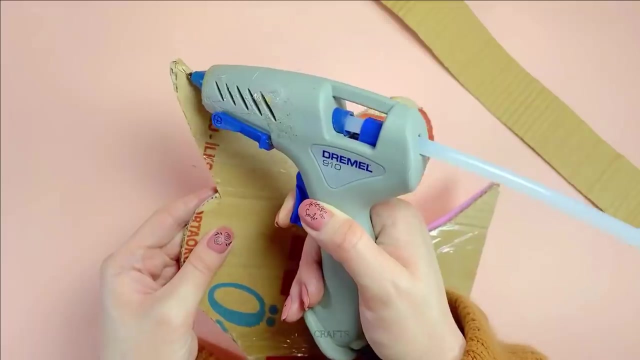 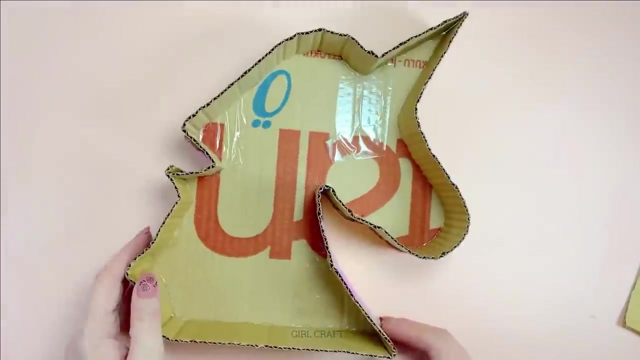 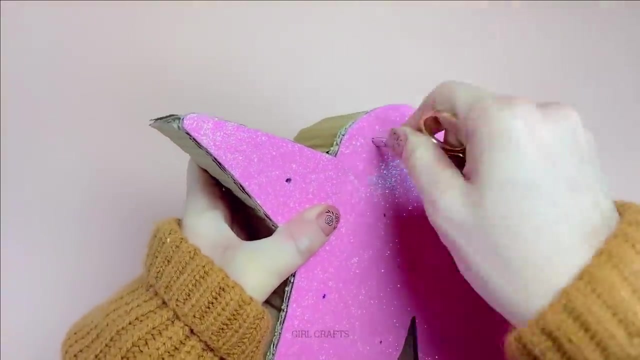 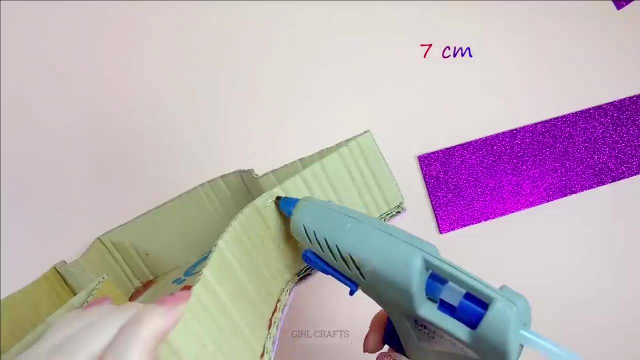 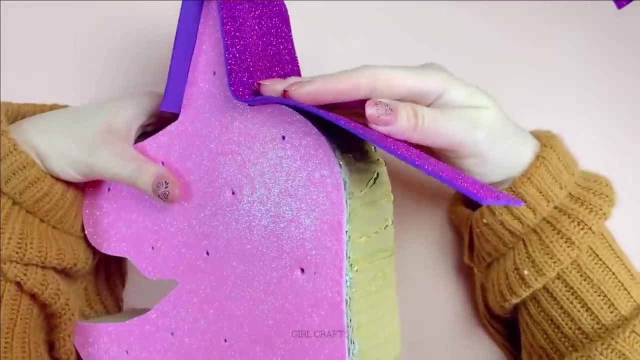 I'ma do my thing, yeah, I'ma. I'ma. I'ma do my thing, Just watch me. I'ma do my thing. yeah, Just watch me. I'ma do my thing. yeah, Oh, don't hesitate. it's only harder the longer you wait. 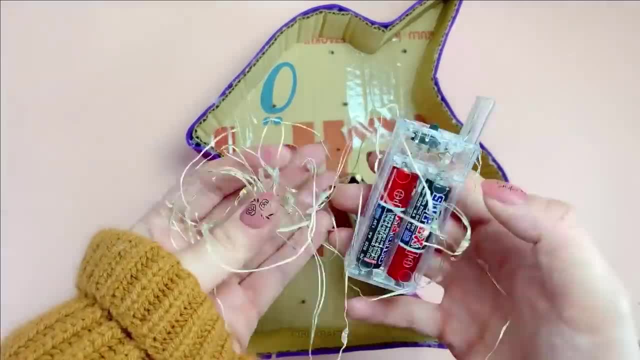 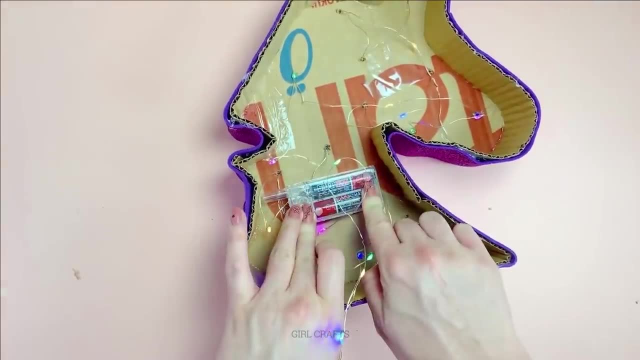 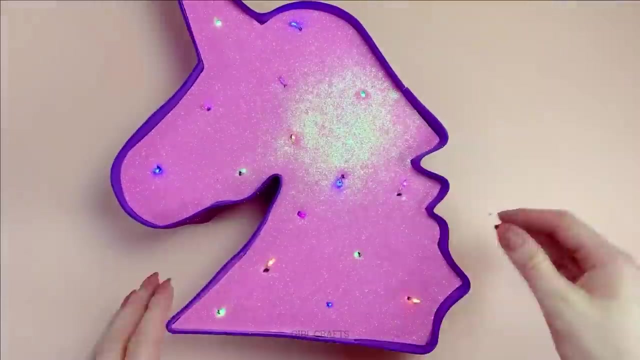 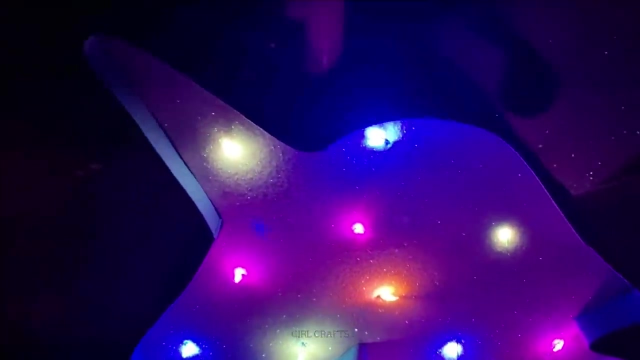 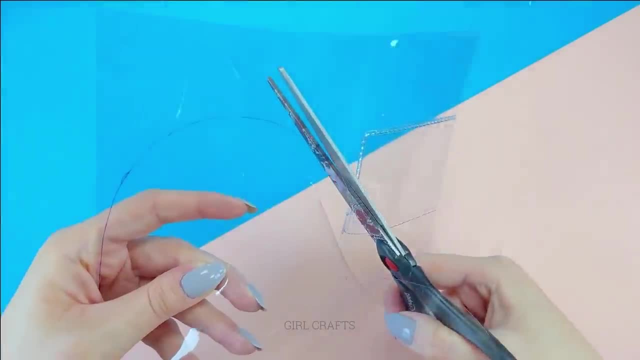 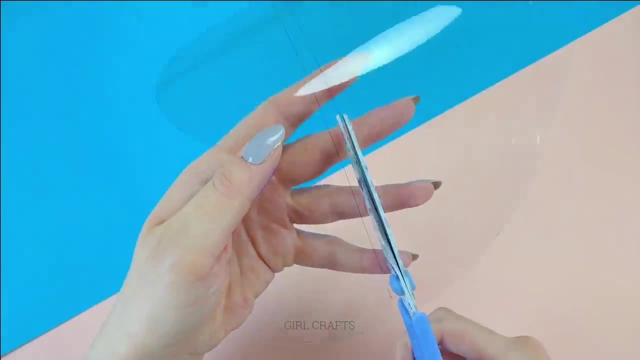 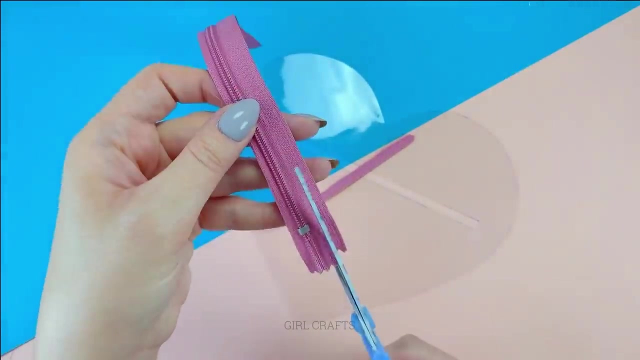 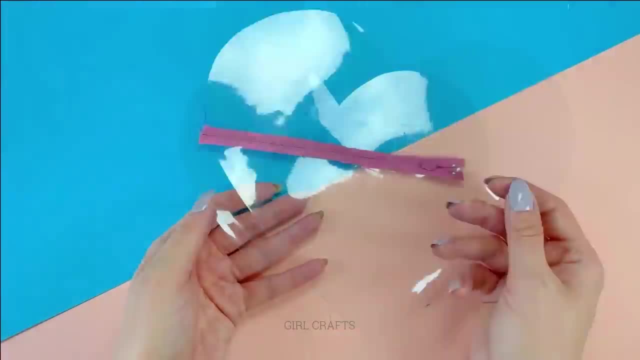 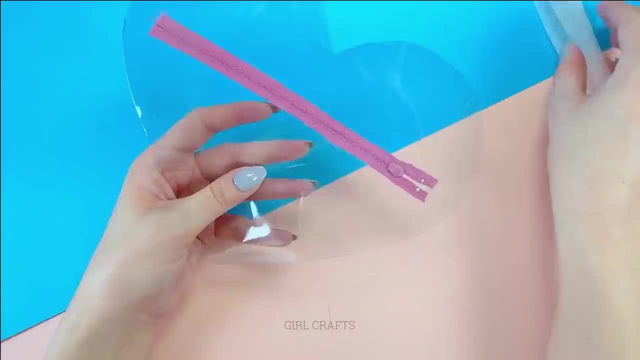 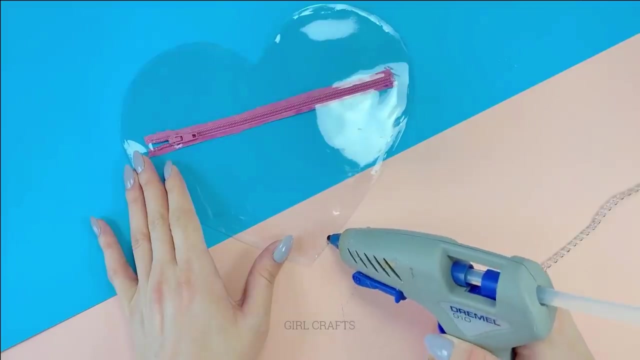 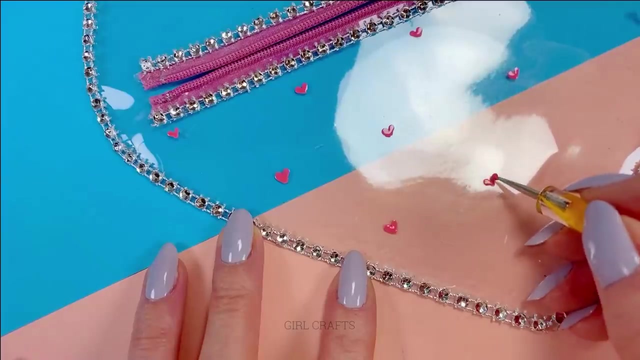 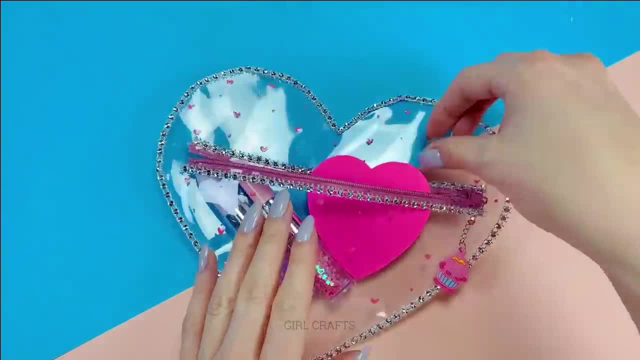 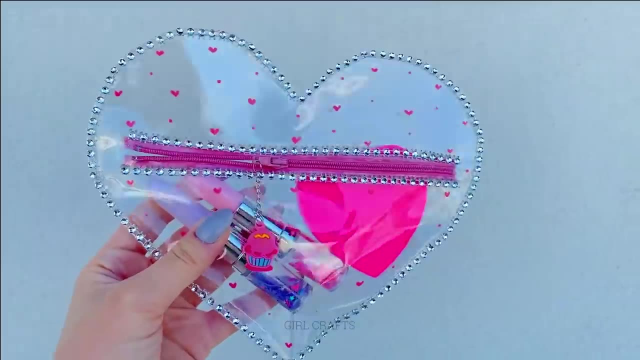 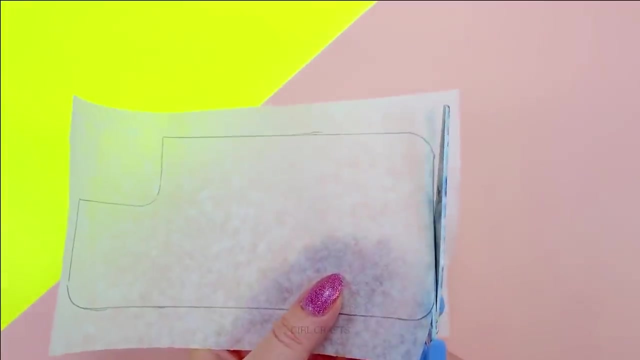 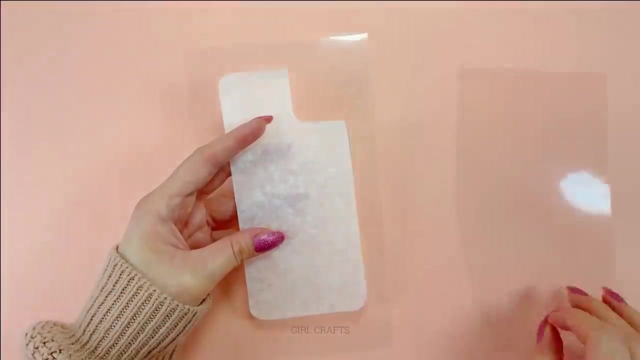 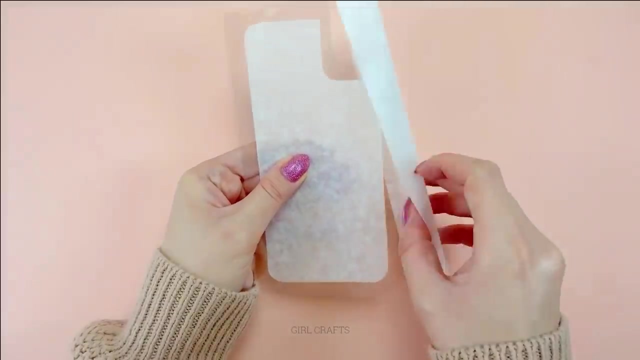 I won't waste a moment. I'm gonna give it all I've got. What have we got to lose? I bring the best of me. you bring the best of you. What have we got to lose? I bring the best of me. you bring the best of you. 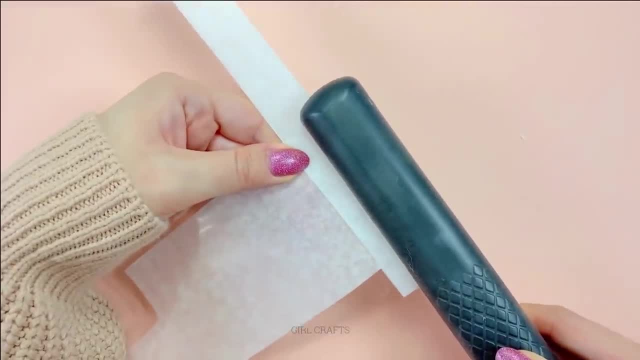 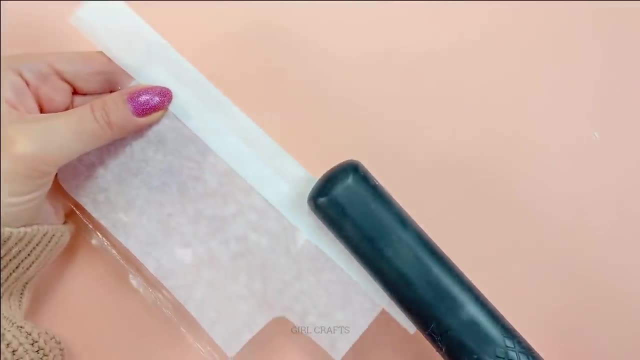 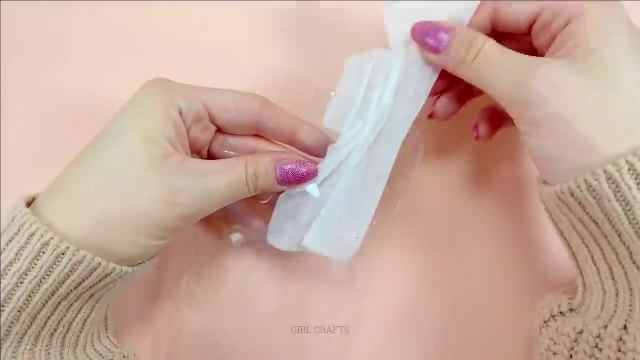 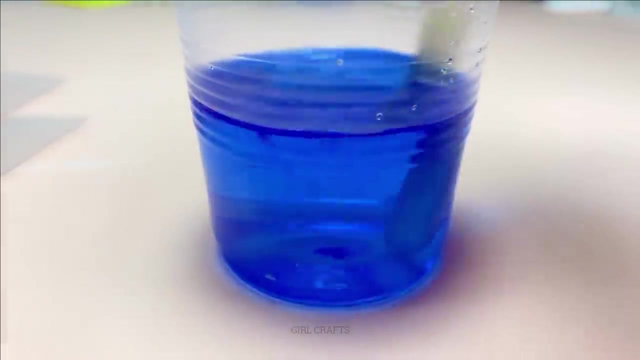 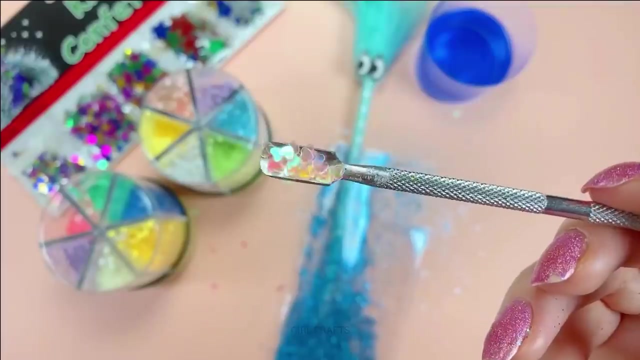 Go on, don't hesitate, slowly, harder, the lonely way. Follow your heart and show the way And all is said and done, it's clear to me that you're the one. We won't let time come between us. No, I won't waste a moment. I'm gonna give it all I've got. 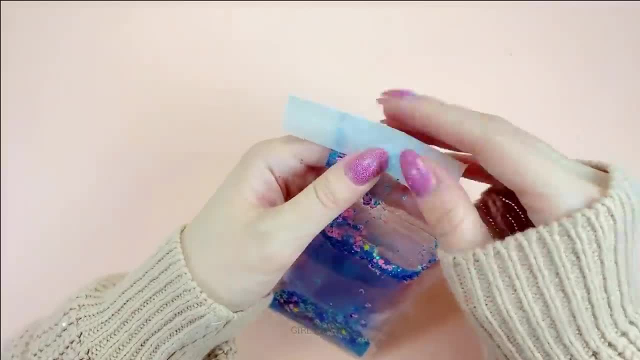 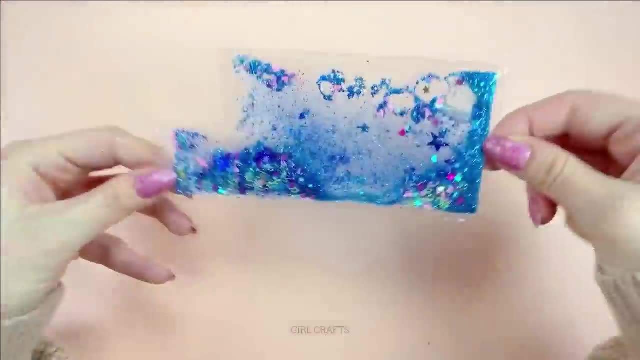 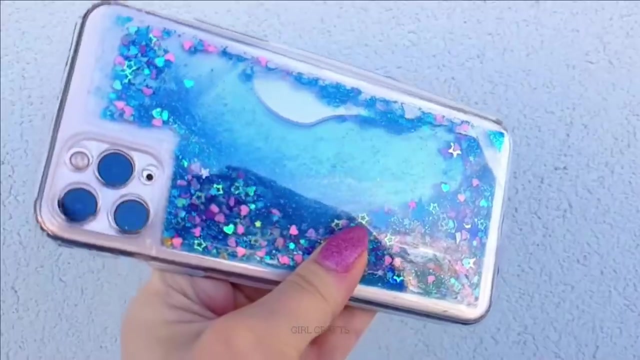 I won't. I won't waste a moment. I'm gonna give it all I've got. I won't waste a moment. I'm gonna give it all I've got. I won't waste a moment. no, I won't waste a moment. I'm gonna give it all I've got. 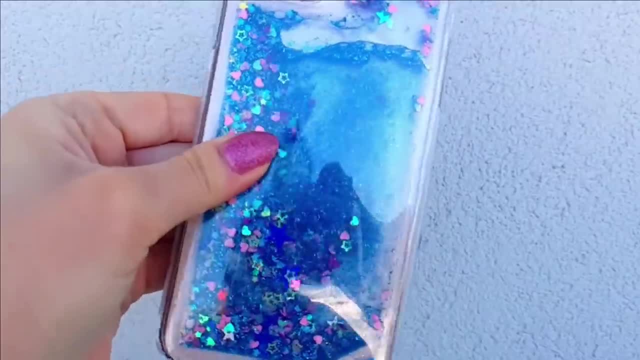 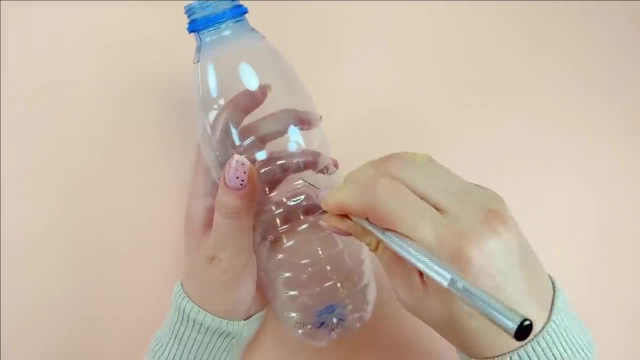 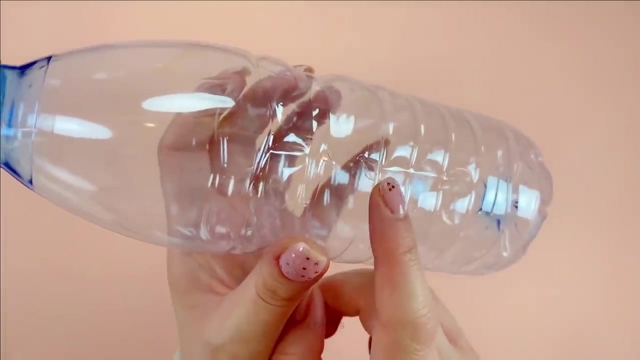 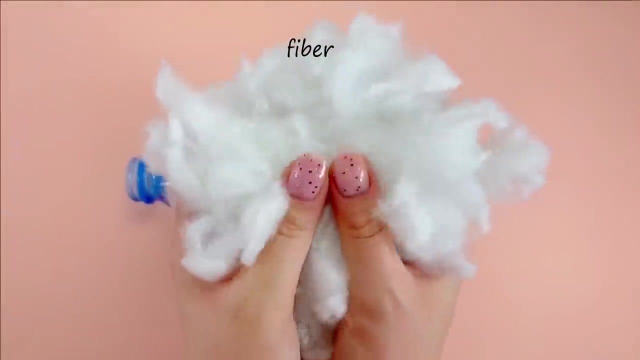 I won't waste a moment. I'm gonna give it all. I've got It's 3.2 from the driveway of my house To your apartment where I am waiting now. Come on, don't think night's young, let's go. NYC, Portland, Austin, Anaheim. 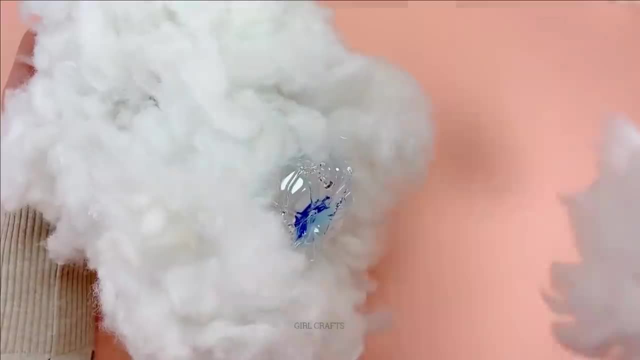 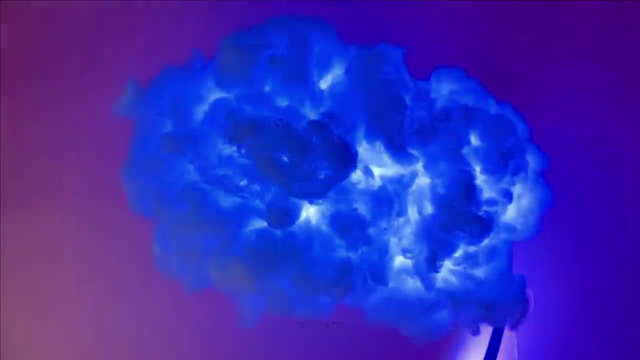 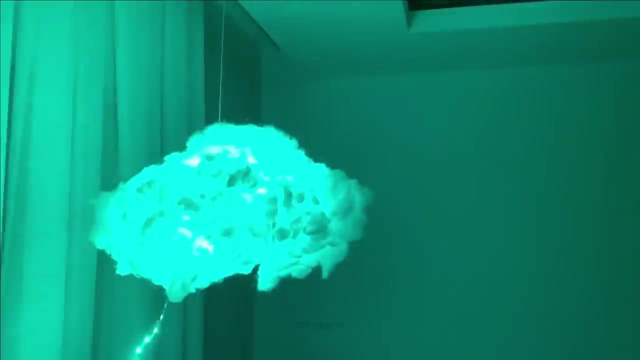 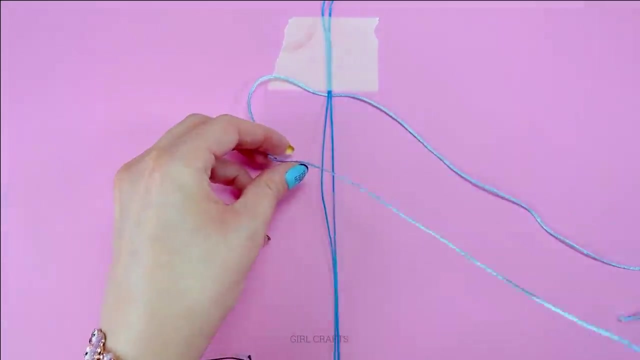 Maybe not Anaheim. keep an open mind. I'm just saying, baby, let's go, I don't care, I don't care. Anywhere. Like a river connects to the ocean. This paving touches wherever we're going, White lines flying by. Who knows what we'll find? 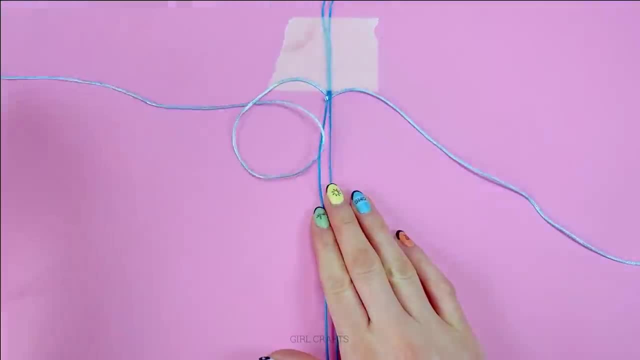 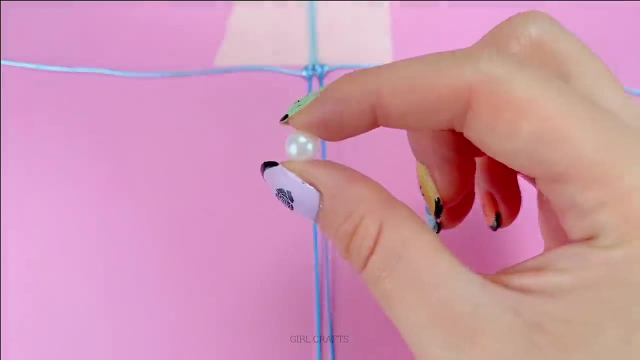 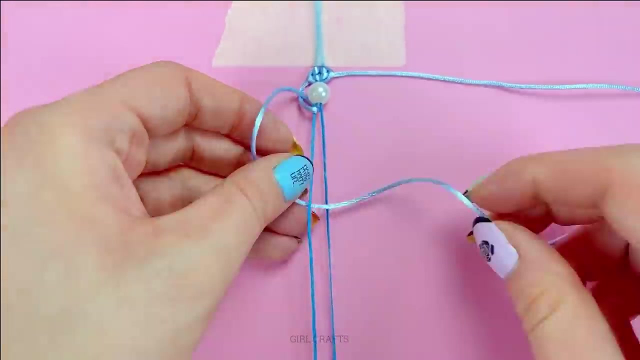 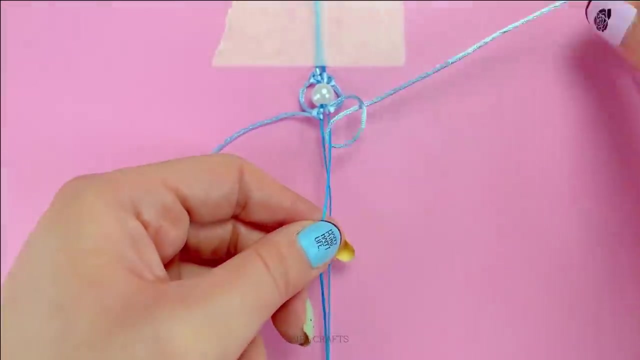 You and me tonight Drive, Let's drive. When's the last time we dropped our things And went To the ocean, Woke up somewhere that we've both never been? Growing up doesn't mean getting older. Maybe it's just left turns off familiar streets. I just wanna come back with a memory. 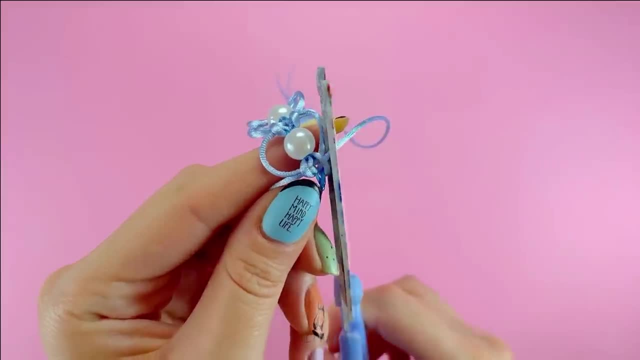 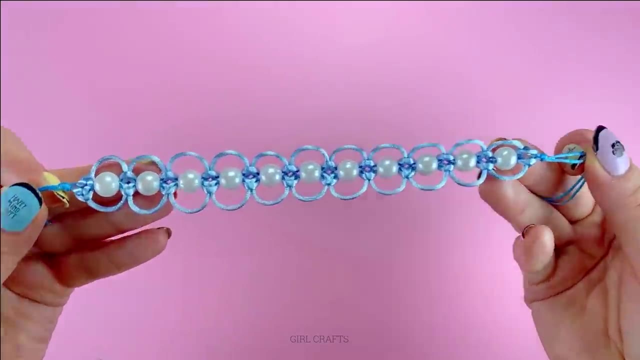 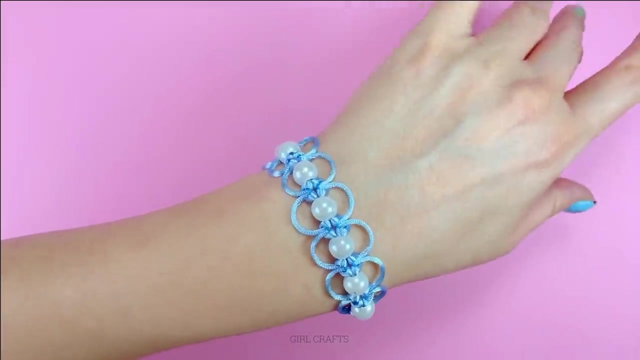 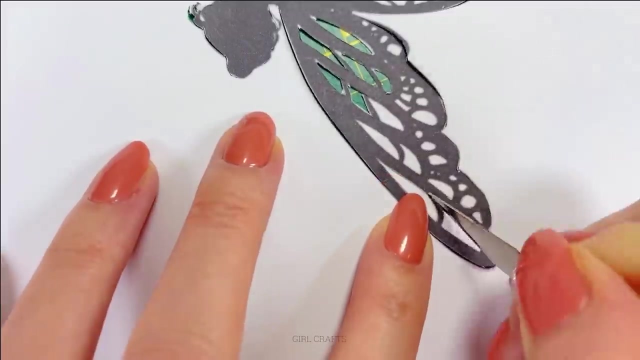 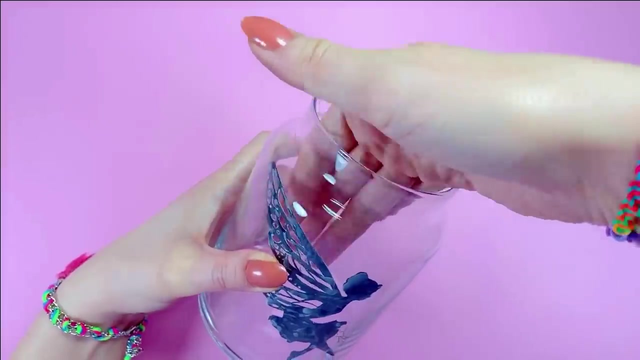 Growing up doesn't mean getting older. I don't care Anywhere. Like a river connects to the ocean. This paving touches wherever we're going: White lines flying by Who knows what we'll find, You and me tonight. Let's drive. Let's drive. Remember when we were young and free. 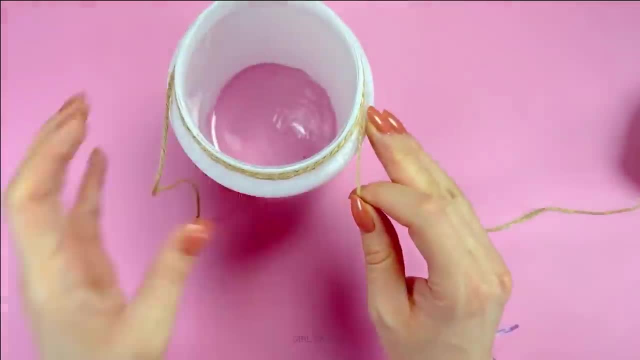 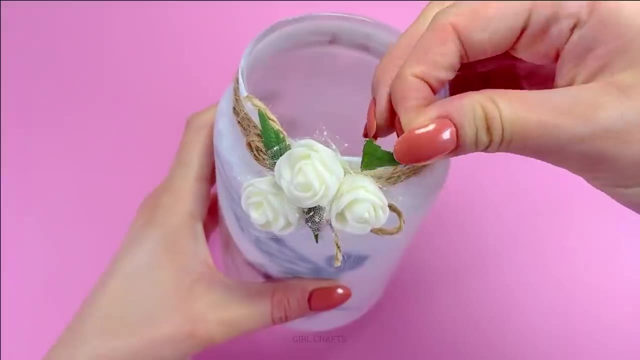 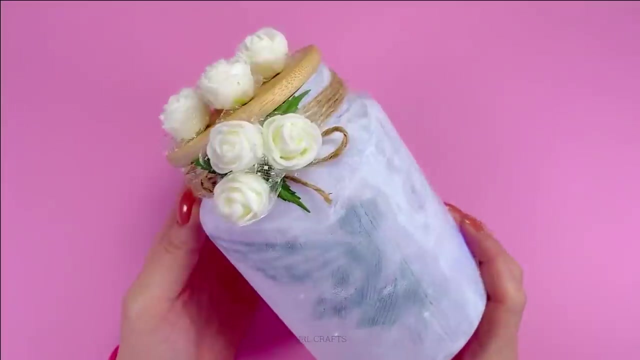 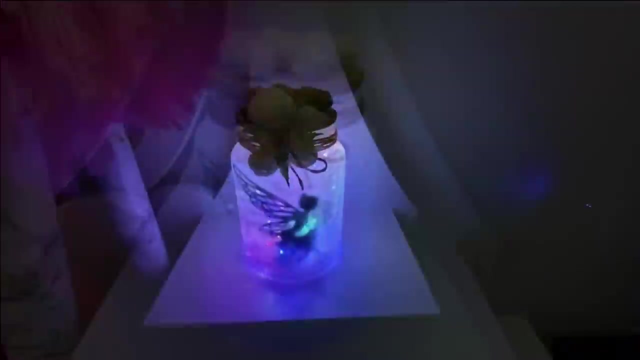 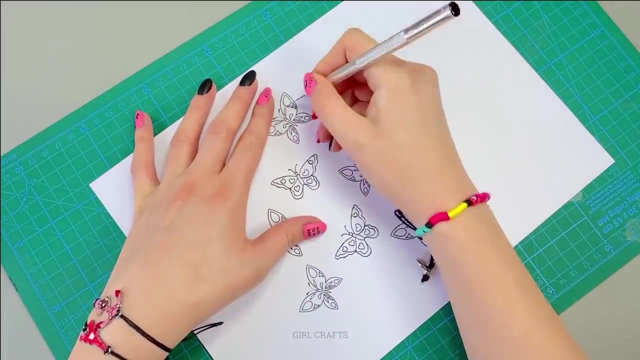 All the way it used to be. Tell me, can we get back to normal 3.2 from the driveway of my house, Your apartment where I am waiting now. Like a river, connects to the ocean. This pain it touches wherever we're going, White lines flying by. 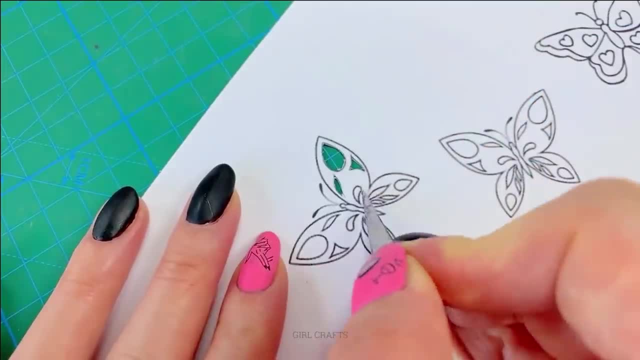 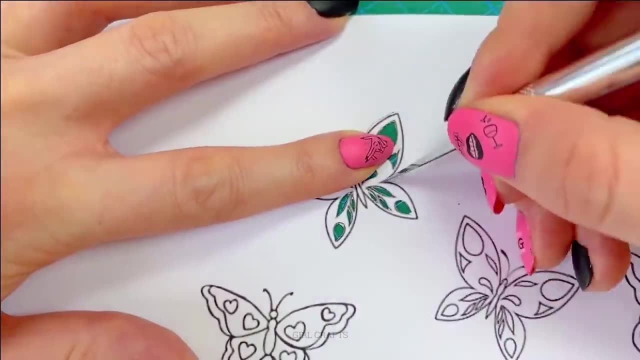 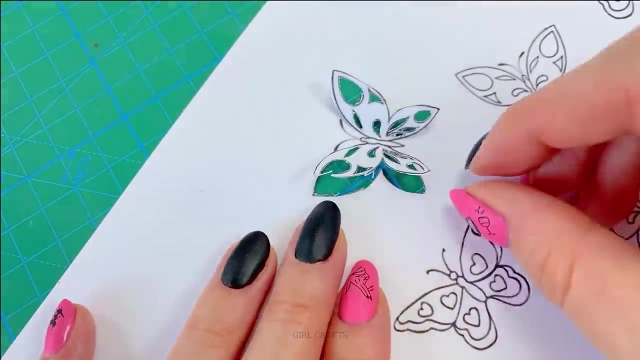 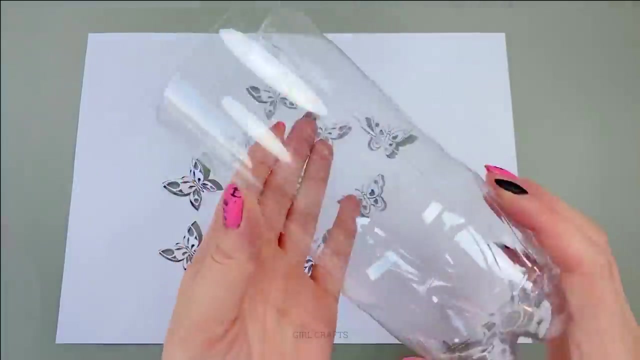 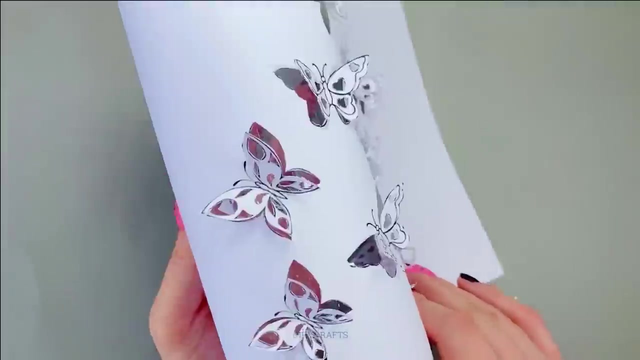 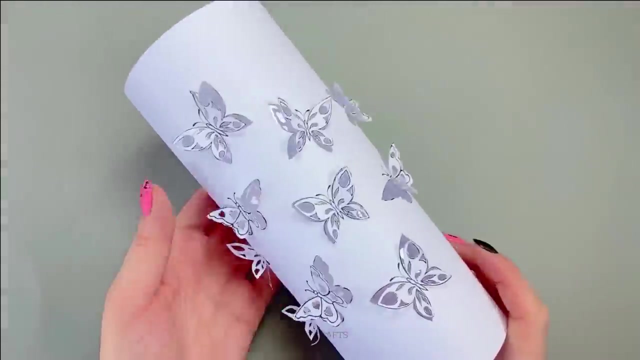 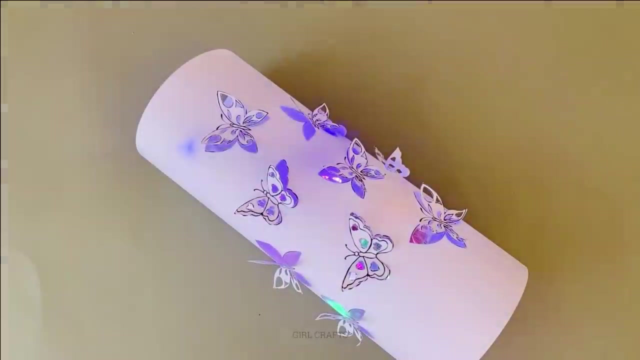 Who knows what we'll find, You and me tonight. Like a river connects to the ocean, This pain it touches wherever we're going, White lines flying by. Who knows what we'll find, You and me tonight? Yeah, let's try, Let's try. I left it all for a while so I could deal with it. 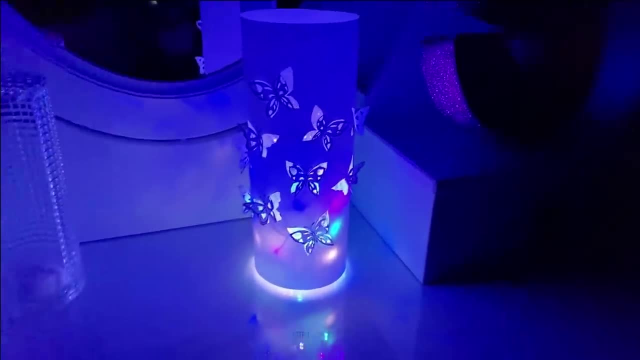 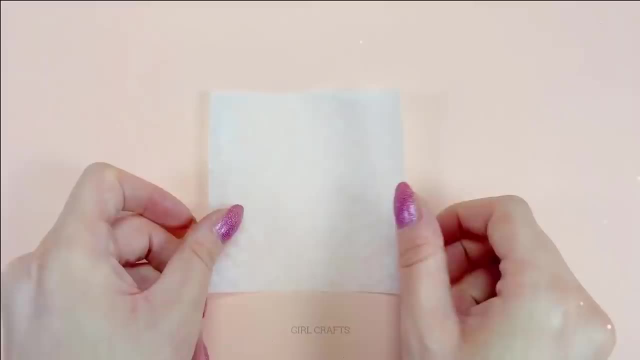 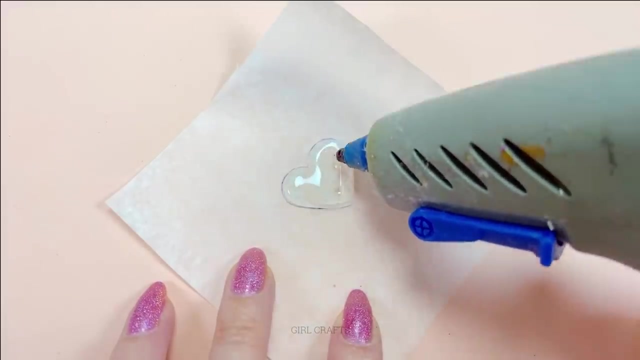 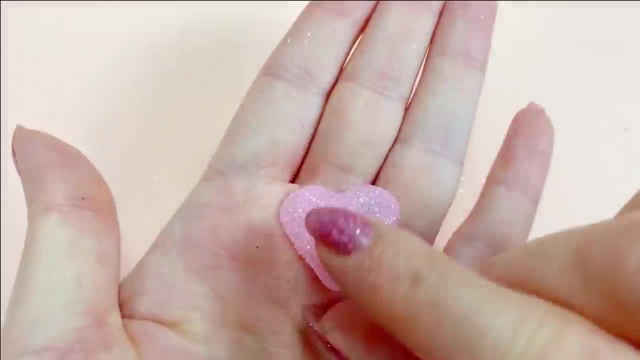 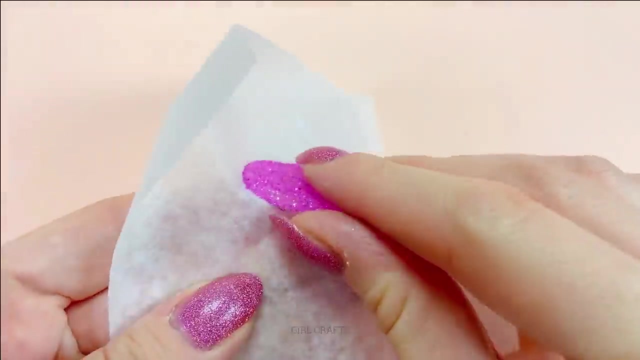 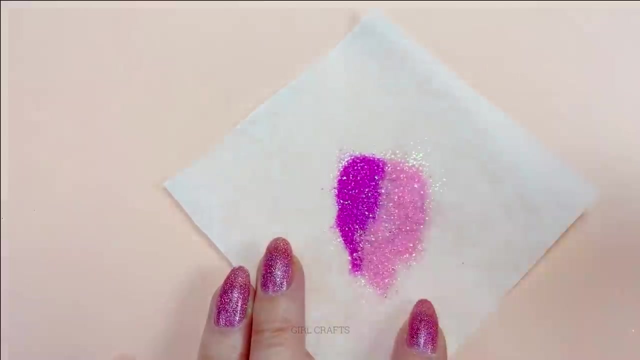 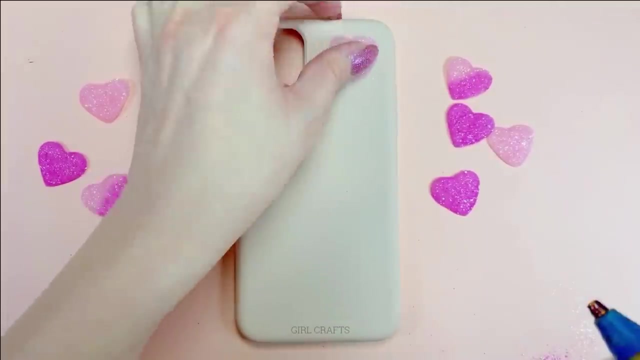 The 9 to 5 and weight of my rocky relationship. But then I met this girl on a holiday. I never felt before. I tickled when she said Monday. Now I gotta hear more The consequences, I gotta run with it. I wanna feel like this: Put your arms around me, baby. 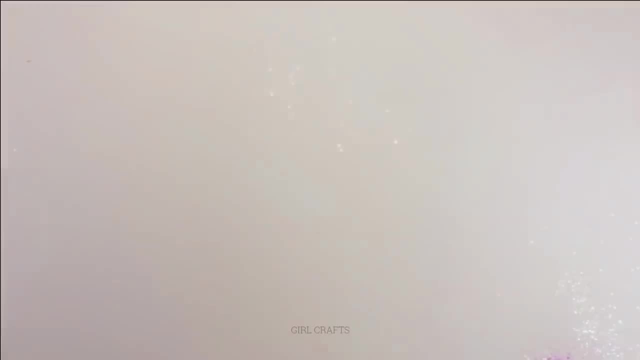 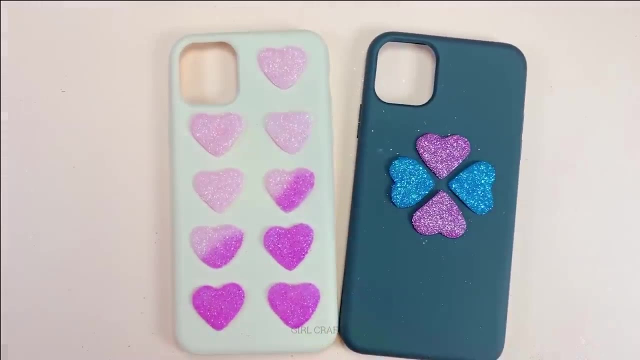 Don't hold back. I-I-I-I. I wanna be like this: Find a way to stay and burn this plane ticket back. Can't trust myself. I never thought I'd break. My heart is broken. I can't believe. I let it go. I wanna be like this. 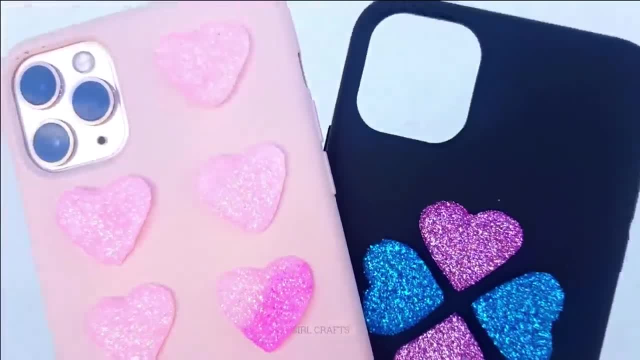 I'm never gonna think of this. I gotta hold on to this. But I'm afraid I can't hold on to this. This pain, it touches wherever we're going, Like a river connects to the ocean. This pain, it touches wherever we're going. I never thought I'd break. 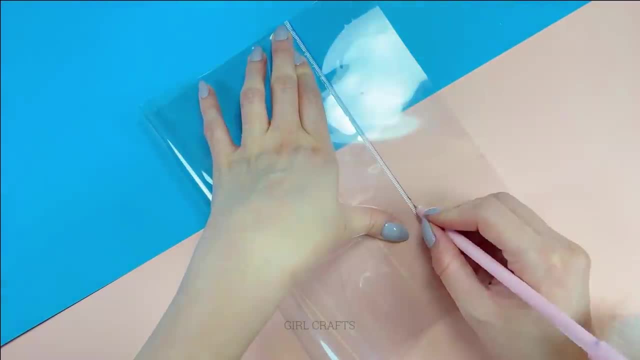 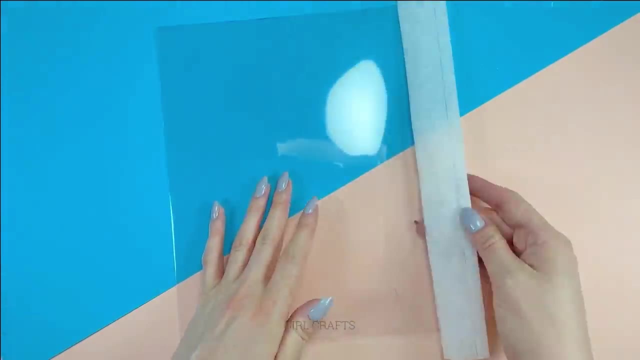 My heart is broken. I never thought I'd let it go. This pain, it touches everywhere. I gotta hold on to this. My heart is broken. It's all in my body. Mmm, mmm, mmm. she slid me some ecstasy in the form of a kiss. 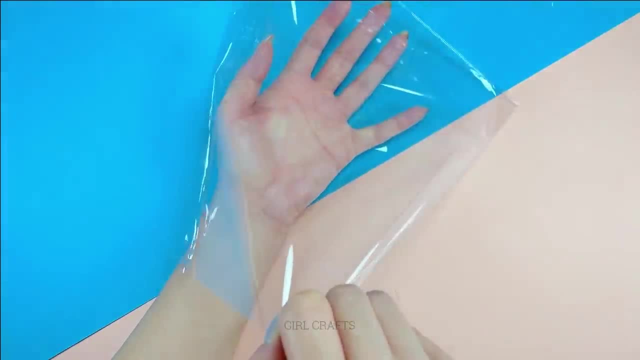 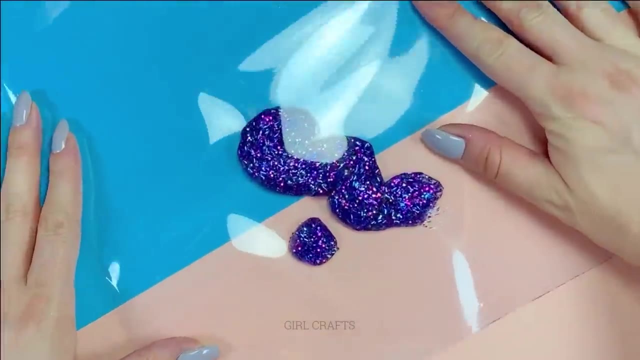 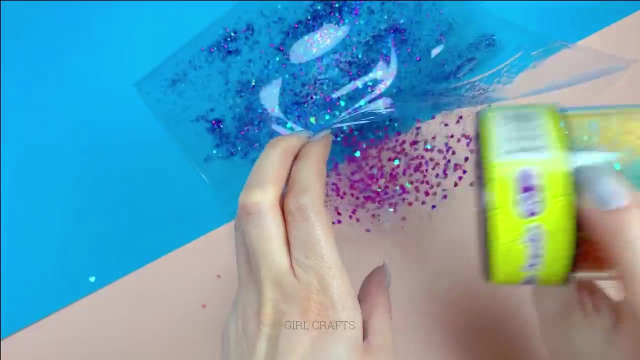 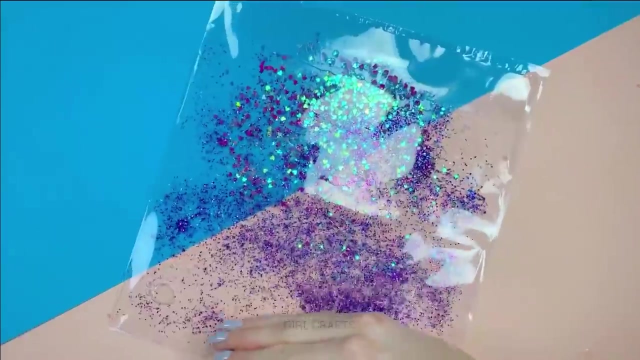 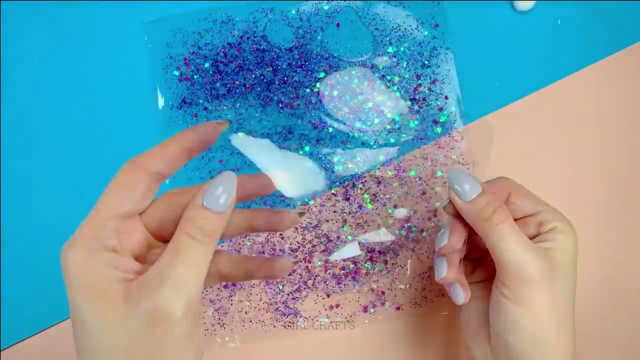 Now I can taste the salt of the sea, yeah, from her lips. Ooh, the consequences. Ooh, I gotta roll with it. I, I, I, I wanna feel like that. Put your arms around me, baby, don't hold back. 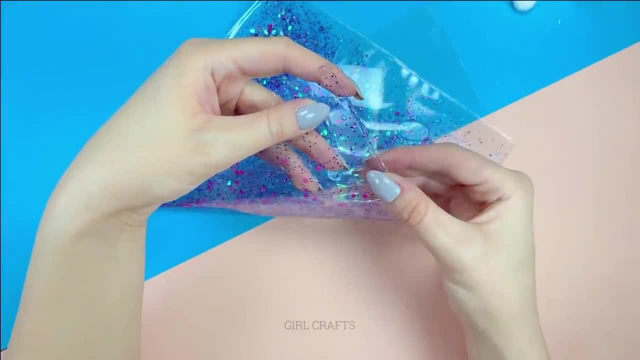 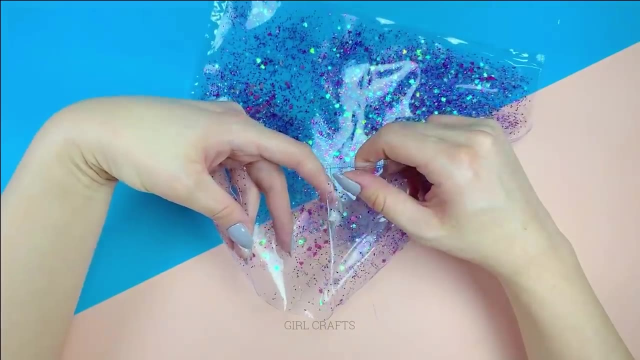 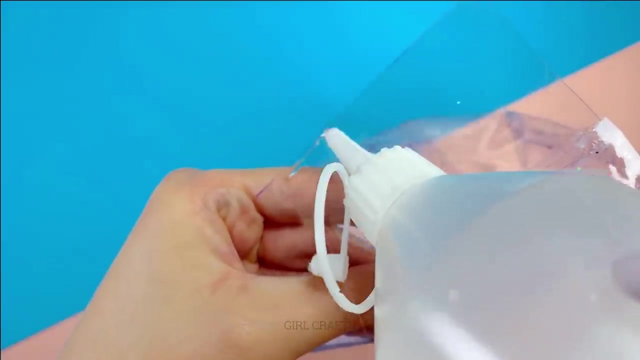 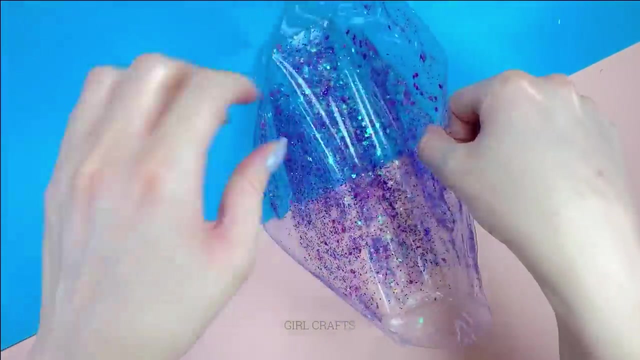 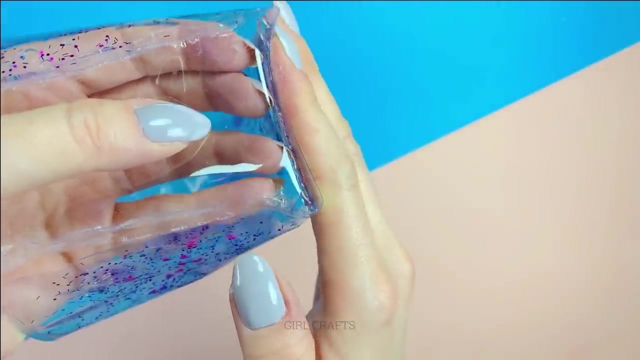 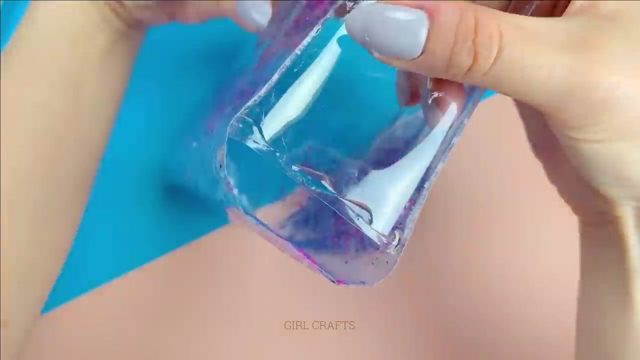 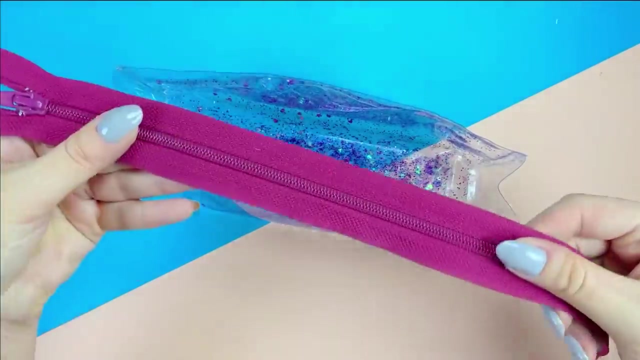 I, I, I, I wanna feel like that. Find a way to stay and burn this plane To get back My baby. she don't understand. When I crossed that sea, I became a different man. I, I, I wanna feel like that. I, I, I, I wanna feel like that. 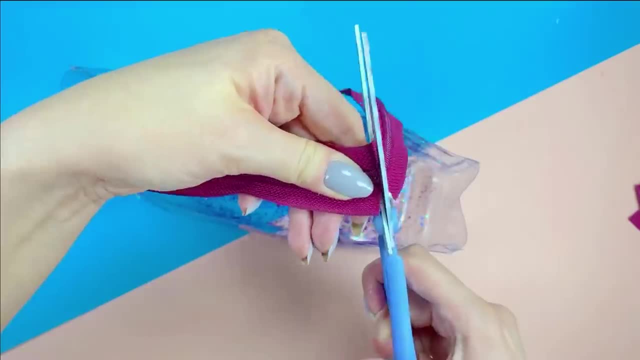 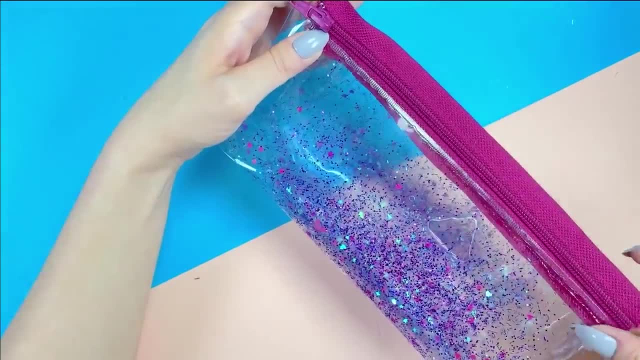 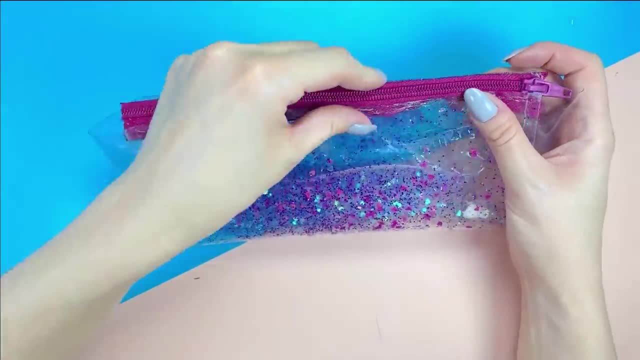 I, I, I, I wanna feel like that: Put your arms around me, baby, don't hold back. I, I, I, I, I wanna feel like that. I, I, I, I wanna feel like that. I, I, I, I, I wanna feel like that. 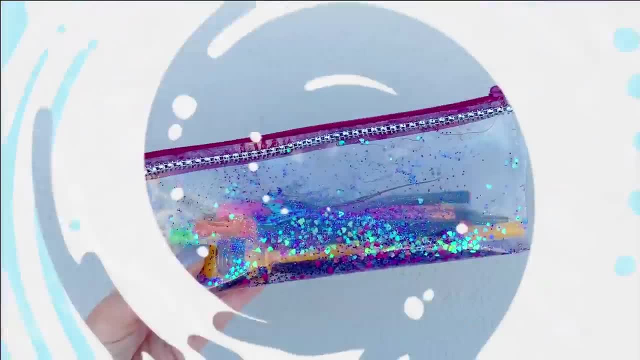 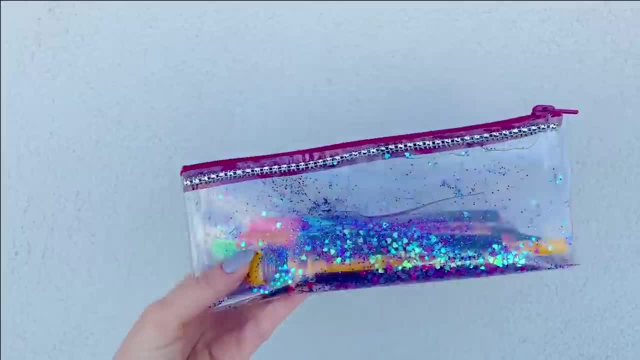 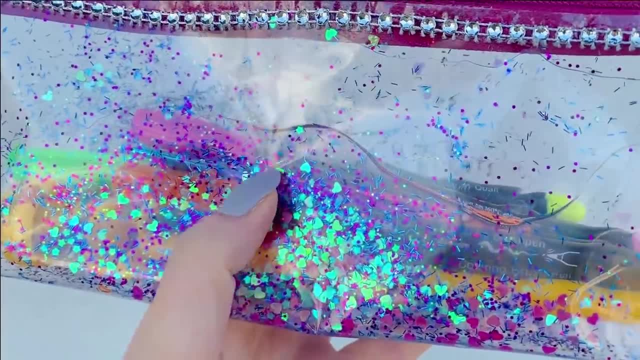 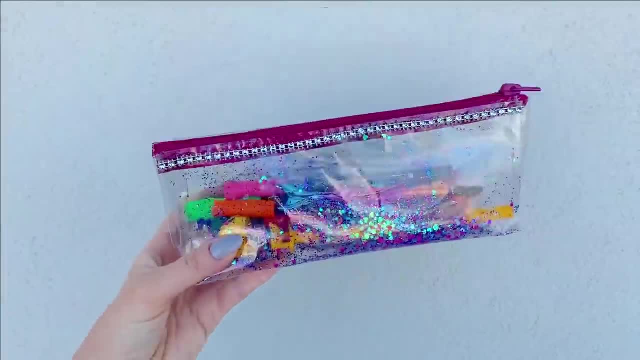 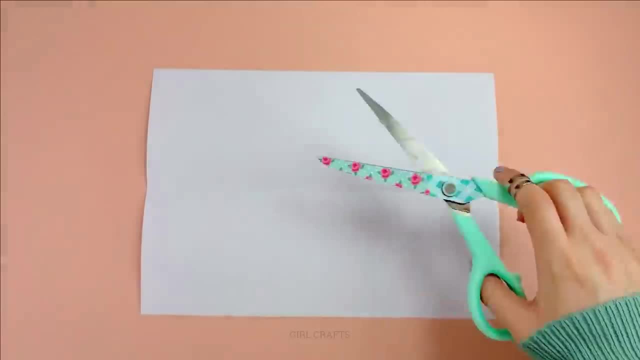 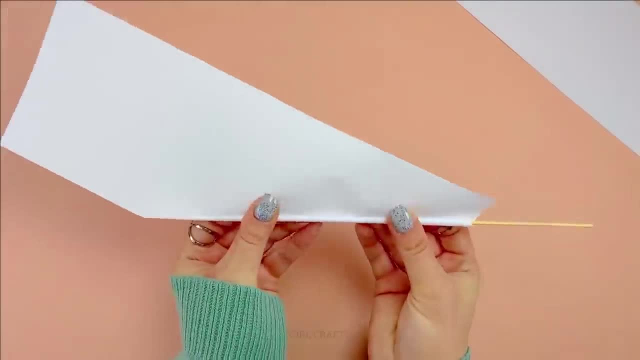 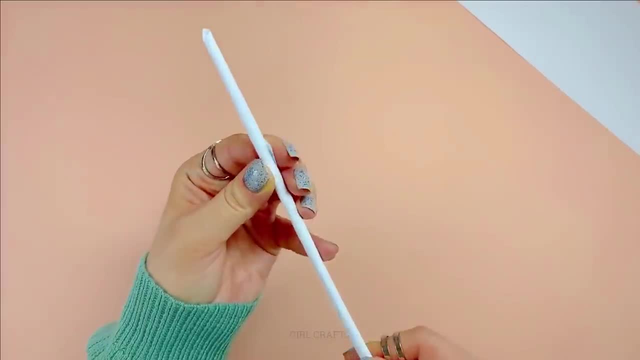 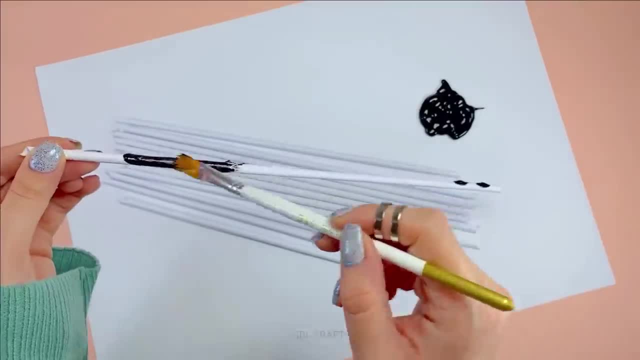 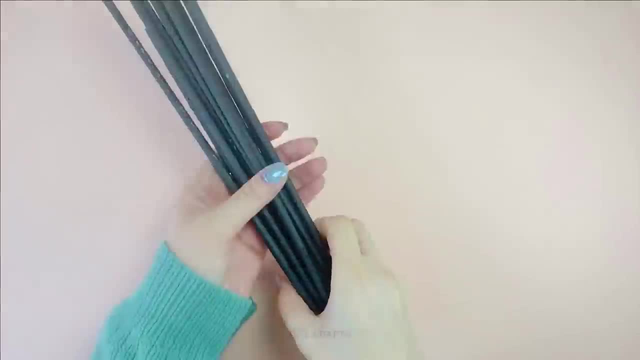 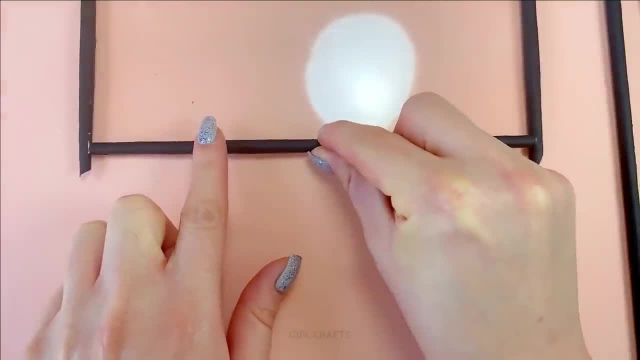 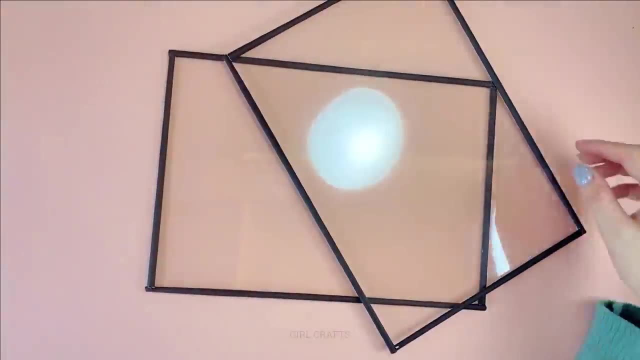 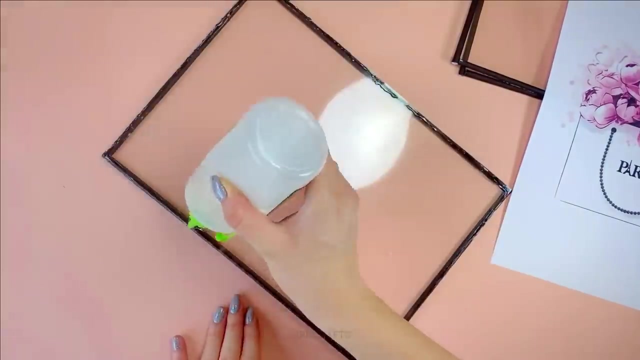 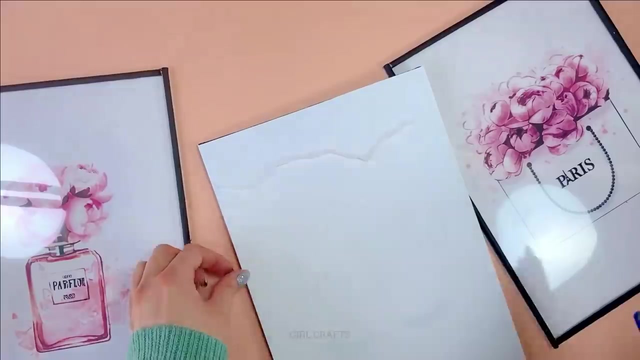 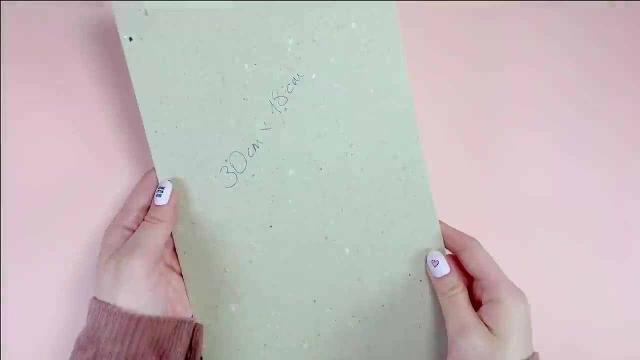 I, I, I, I wanna feel like that. I, I, I, I wanna feel like that. Imagine all the things that we could see. Don't you know that life's a dance. Come take my hand And fly away with me, Make my heart race in a hurry, lose my every worry every second I'm with you. 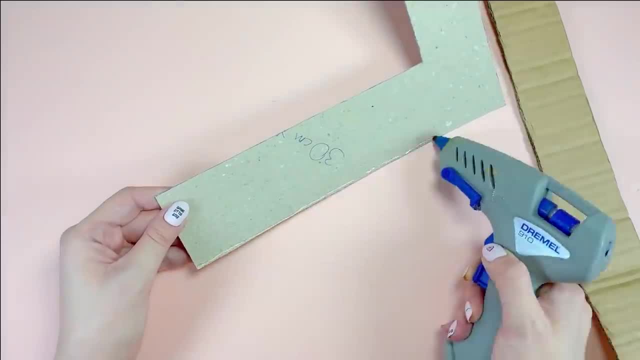 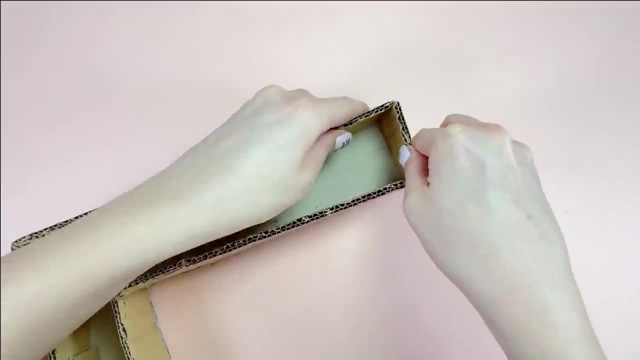 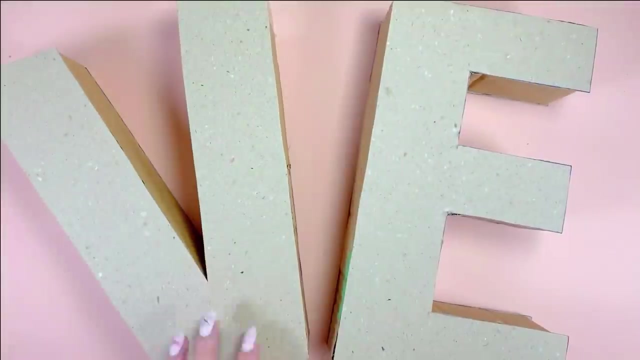 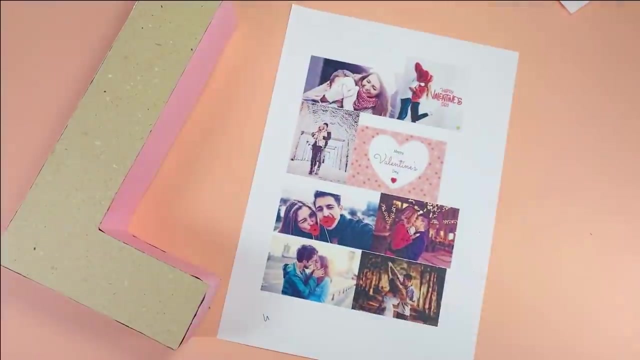 We'll turn all the pages, check off all the places. every day is something new. Don't that sky look blue? yeah, Come fly away with me. imagine all the things that we could see. And don't you know that life's a dance. come take my hand and fly away with me. 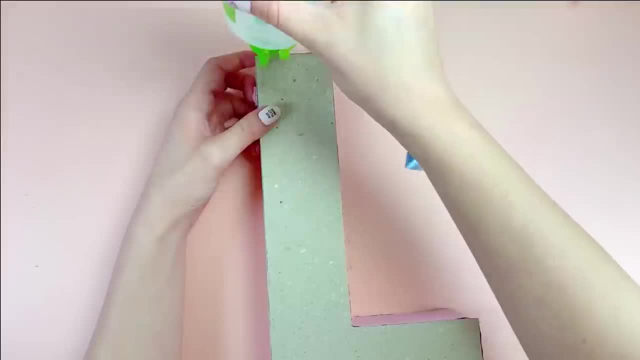 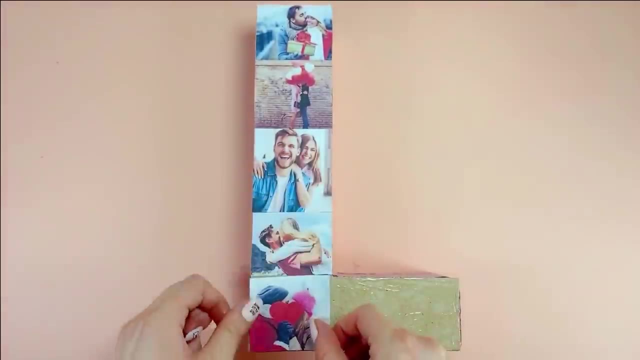 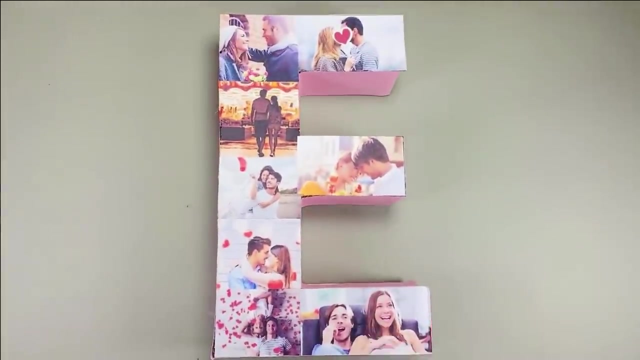 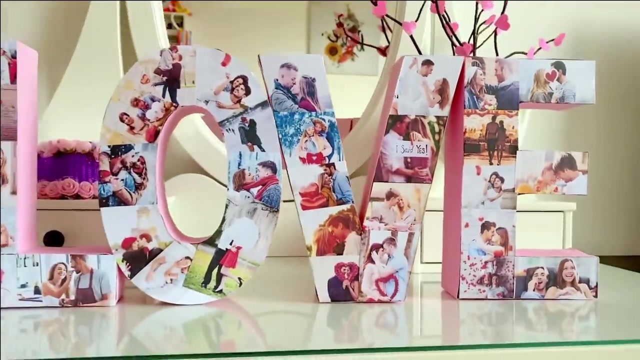 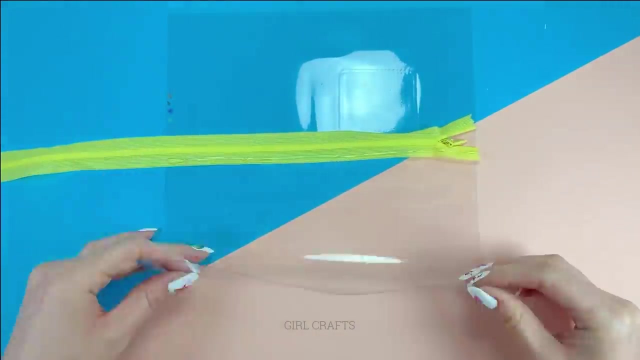 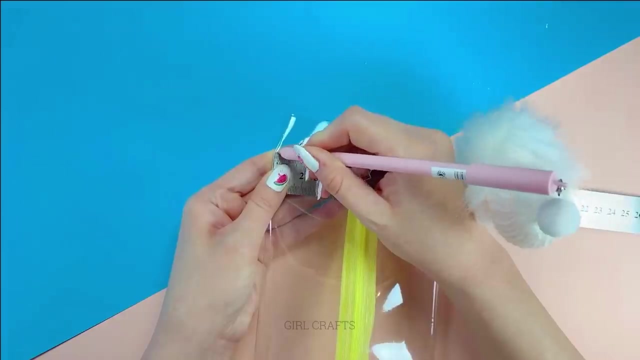 You're my sunshine. You're my sunshine Every morning, light up every moment, Make my every dream come true. Oh, I can't describe it. Took my tongue and tied it, Sent my heart over the moon. Come, fly away with me. Imagine all the things that we could see. 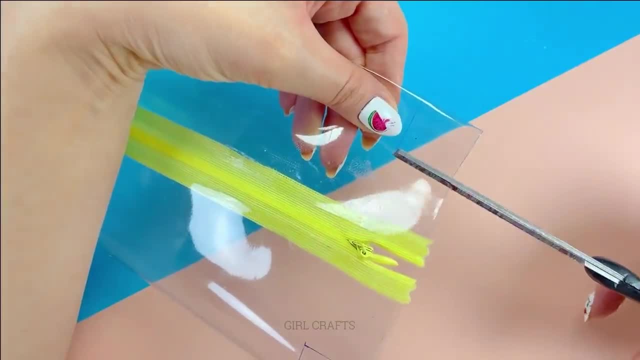 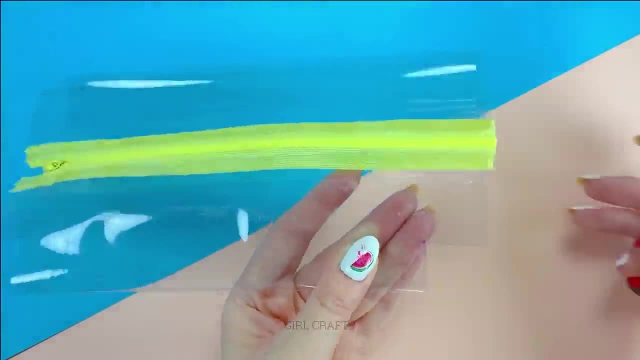 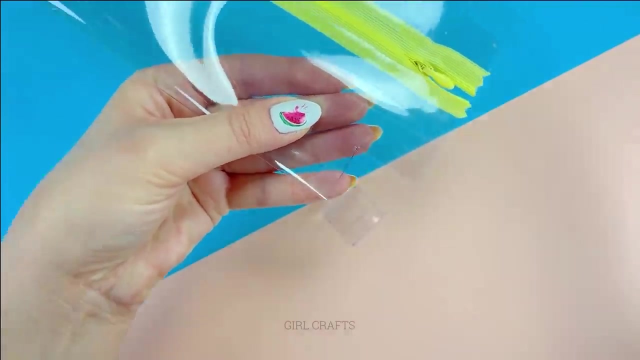 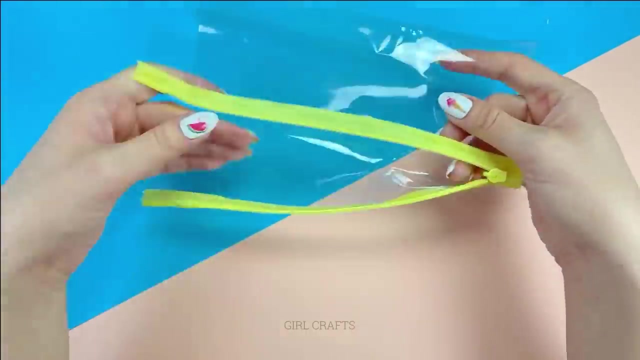 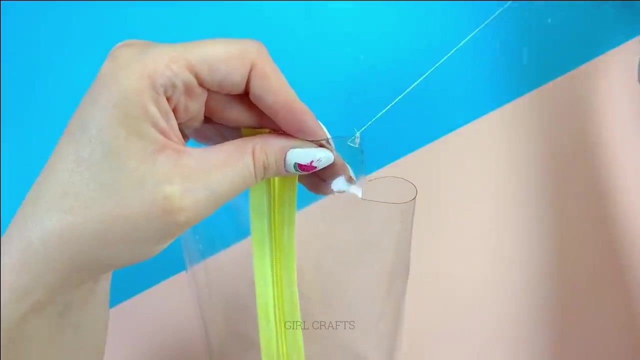 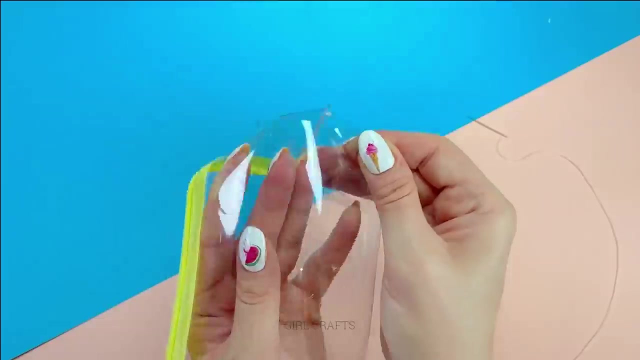 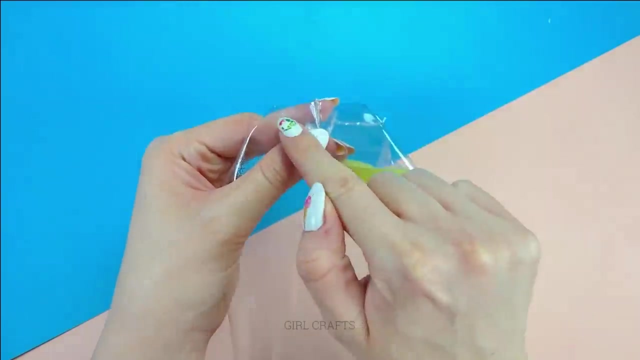 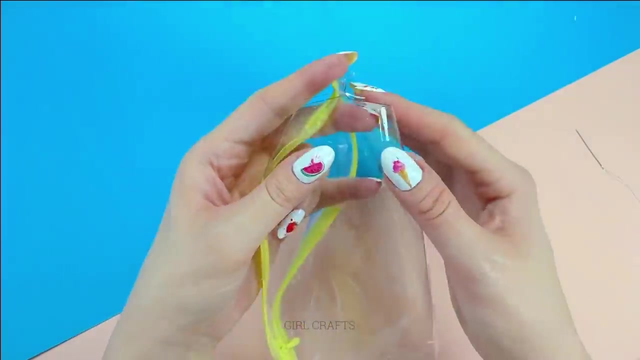 Don't you know that life's a dance? Come take my hand, Fly away. fly away with me. Imagine all the things that we could see. Don't you know that life's a dance? Let's not miss our chance. Come fly away with me. I don't want to think like that. 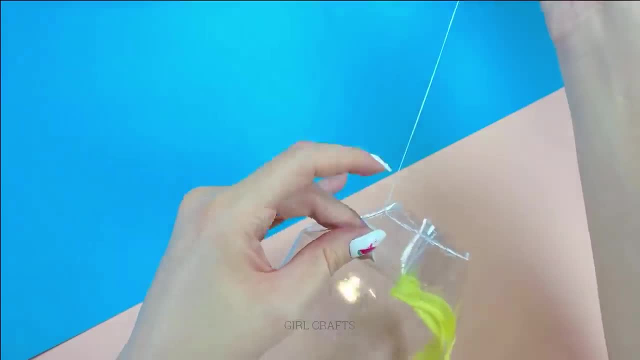 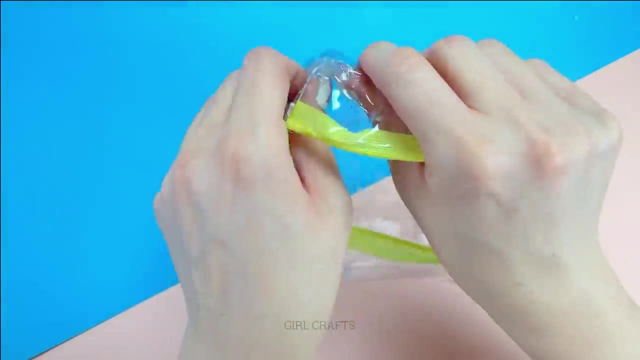 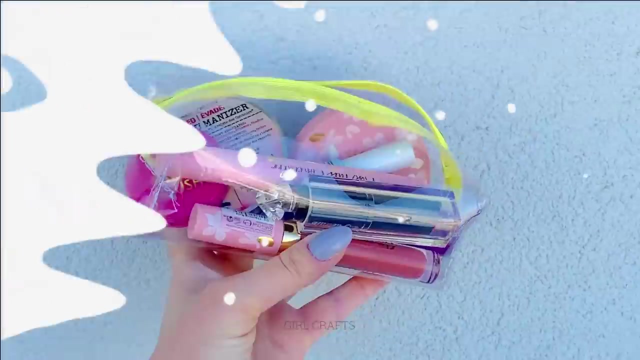 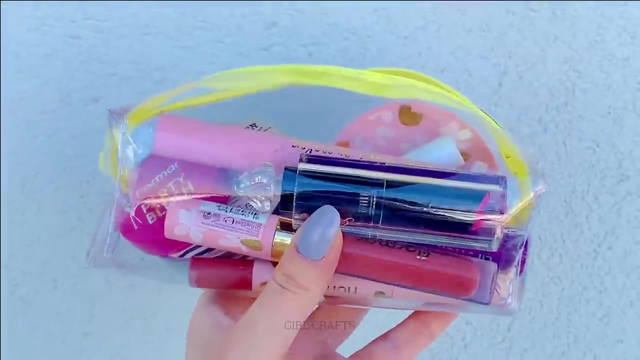 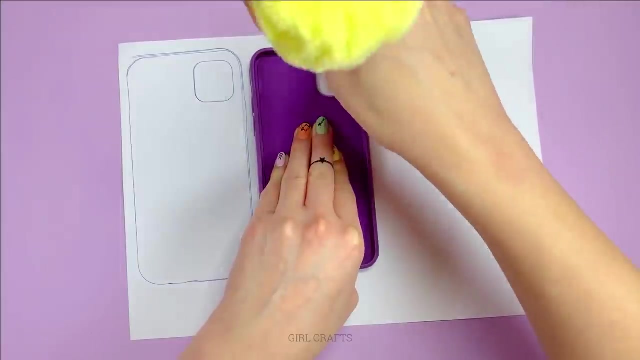 I can't stop and turn right back. I can't stop and turn right back. Oh, oh, oh, oh oh. We grew up. Can we change the day? The roads run, We'll get through the rain. Oh, oh, oh, oh oh. 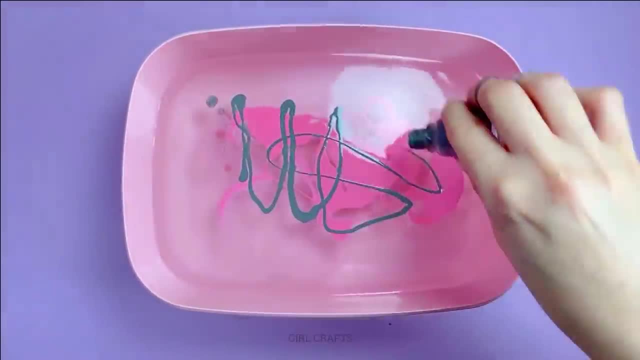 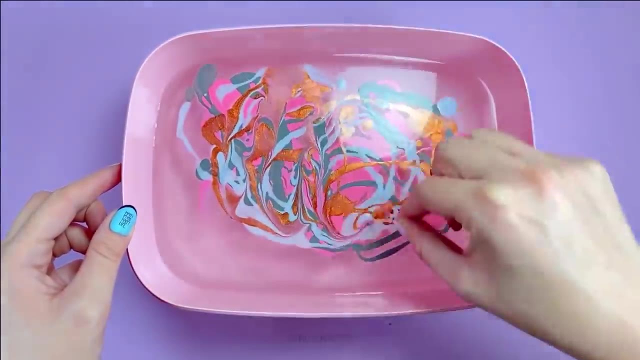 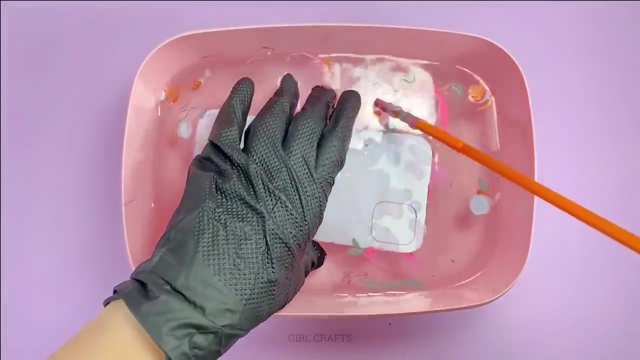 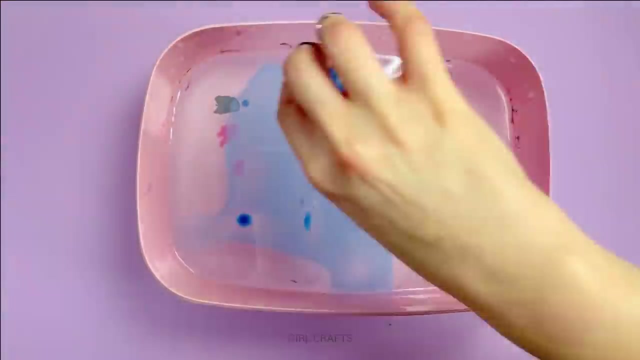 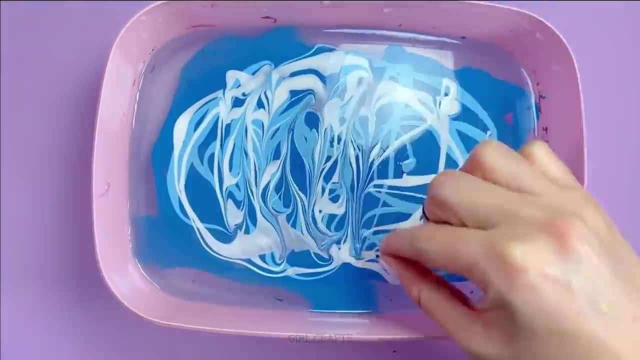 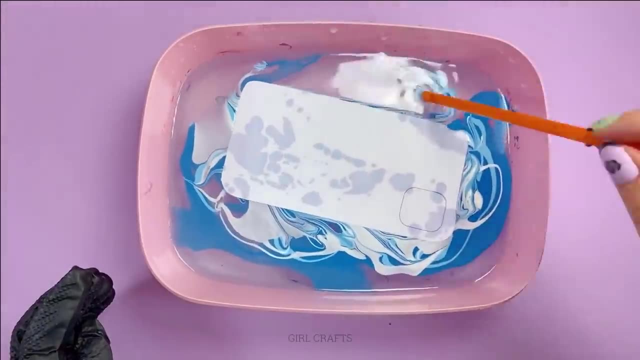 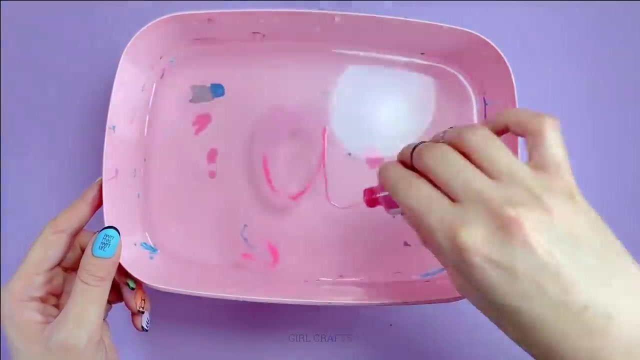 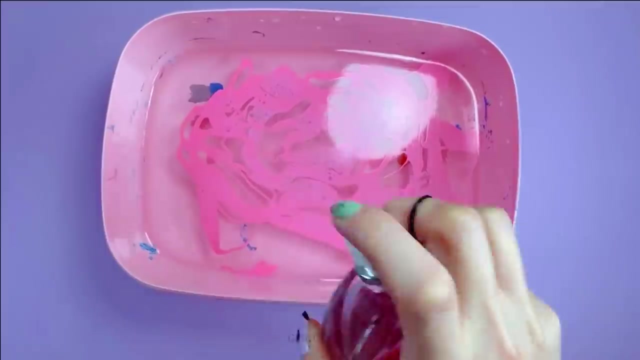 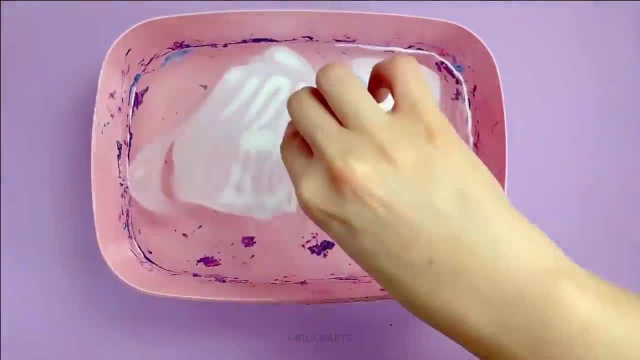 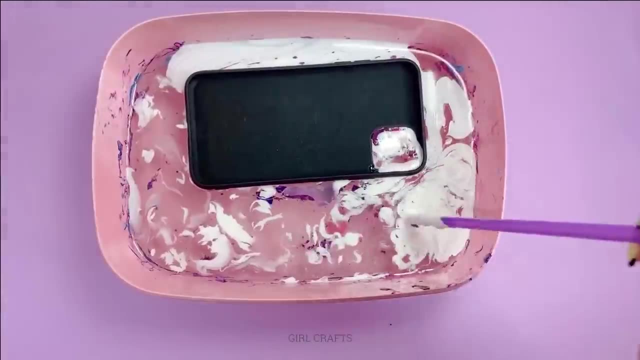 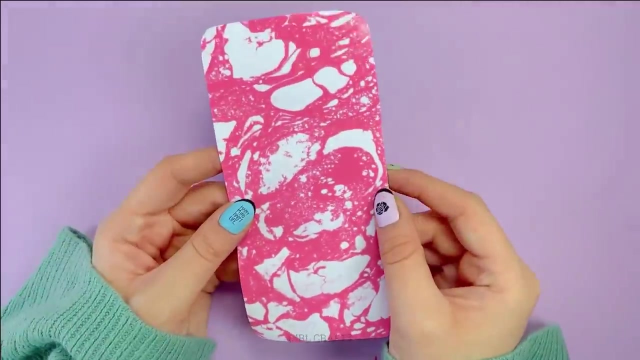 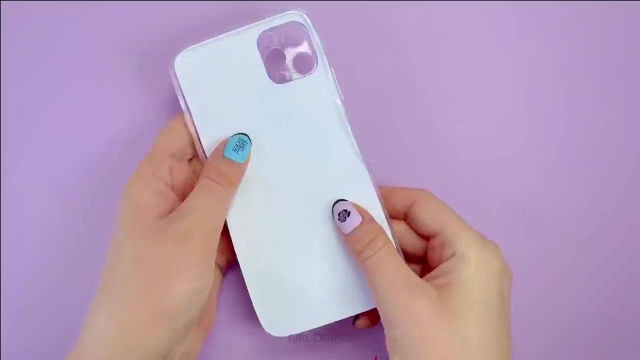 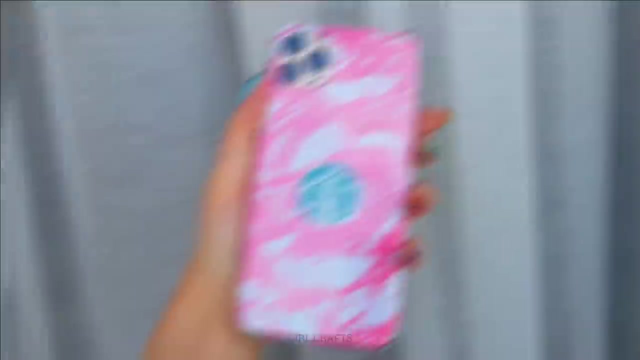 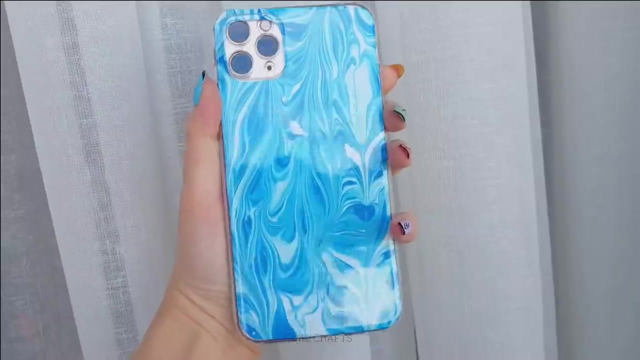 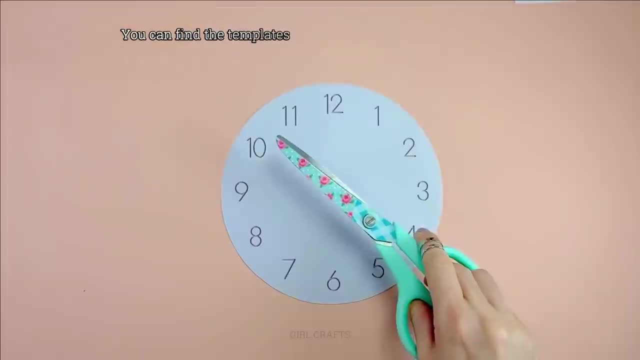 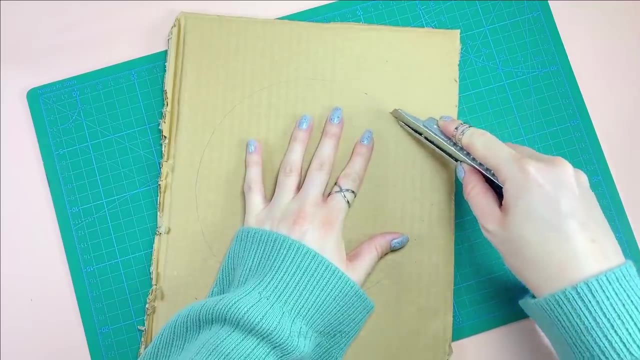 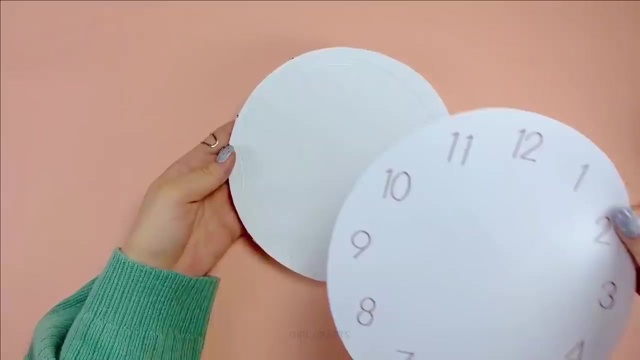 I think I like The way we fight, Not gonna hide Anymore. I got a good good feeling. You got me in a mood. I got a good good feeling And I know you feel it too. I'll take you to my rooftop Let you see the view. 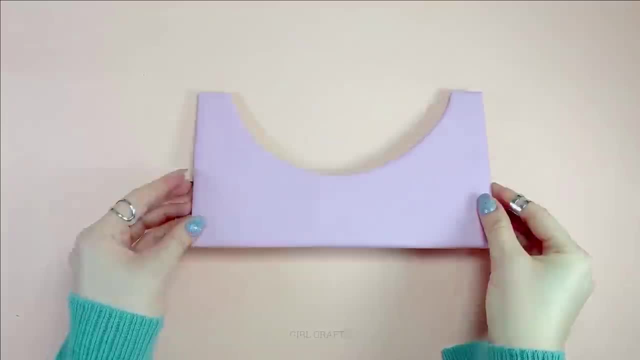 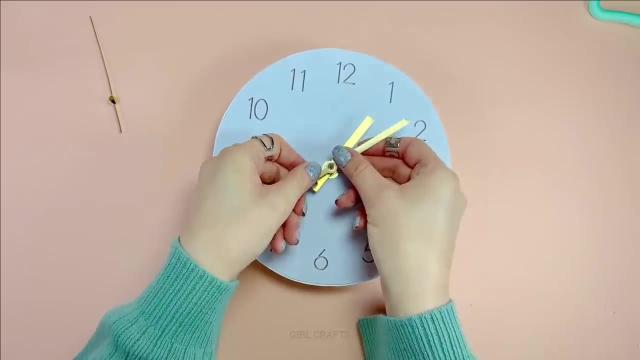 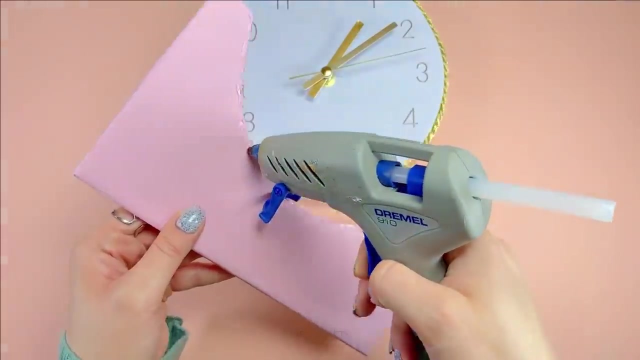 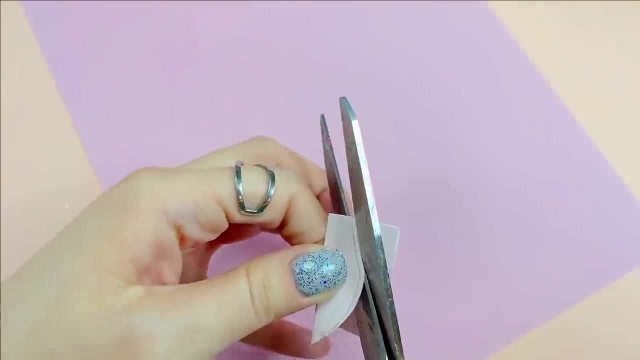 Passing all my levels, baby Making up the rules. I think I like The way we fight, Not gonna hide Anymore. I got a good, good feeling. Good, good feeling. I got a good, good feeling. I'm not gonna hide, hide, hide it anymore. 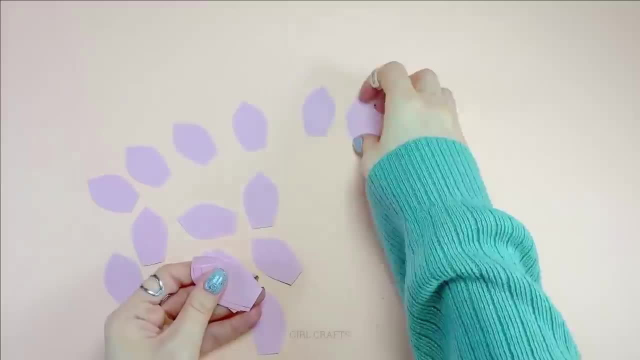 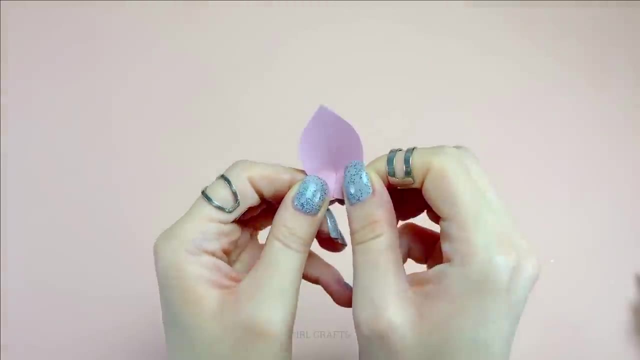 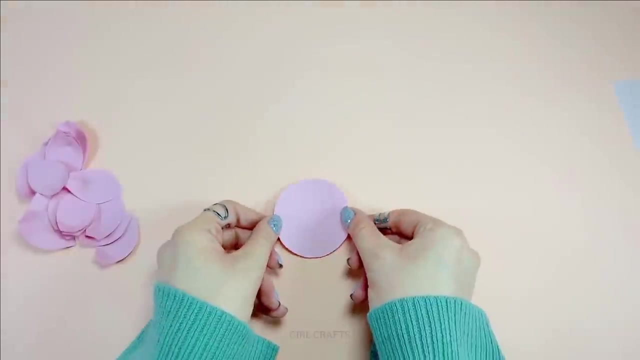 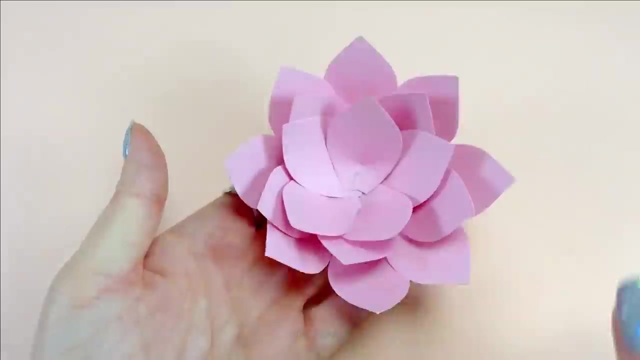 I got a good, good feeling. You got me in the mood. I got a good, good feeling, And I know you feel it too. I know you feel it too. Nothing gonna stop me living it up, Dancing to the backbeat, turning it up. Nothing gonna stop me living it up. 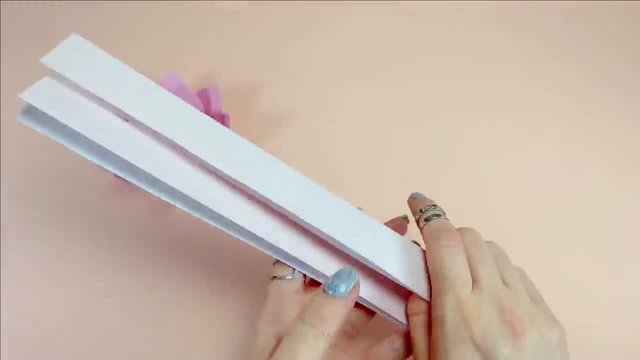 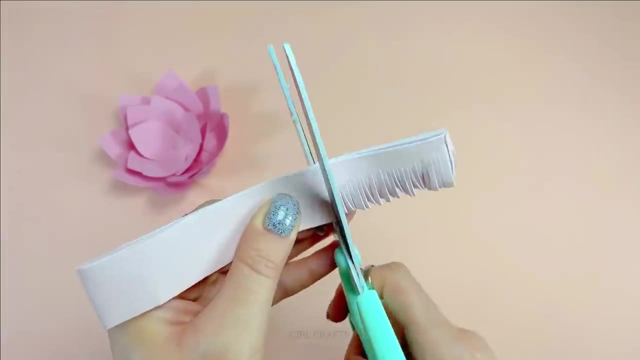 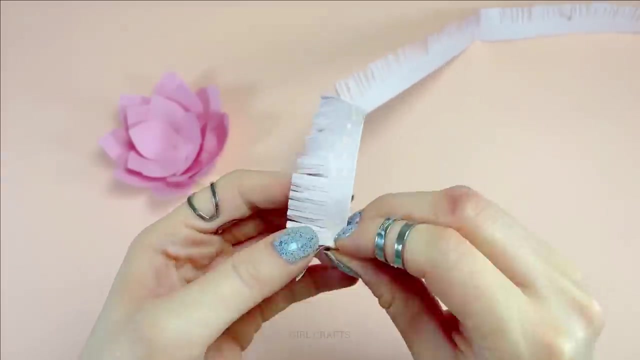 Dancing to the backbeat, turning it up, Nothing gonna stop me living it up. Dancing to the backbeat, turning it up, Nothing gonna stop me living it up. I got a good, good feeling. You got me in the mood. I got a good, good feeling. 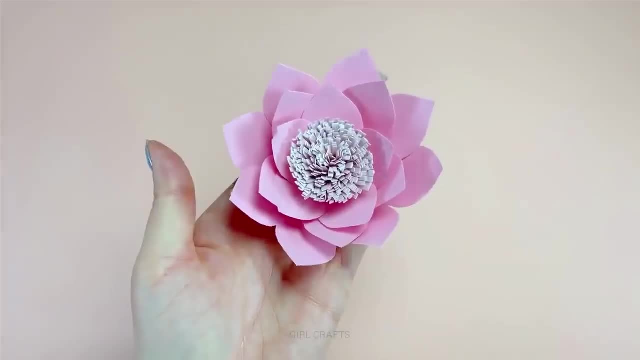 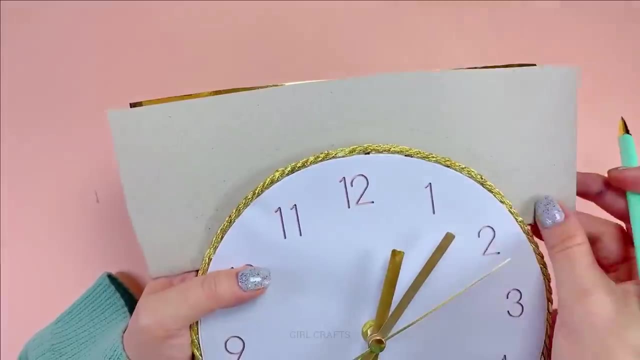 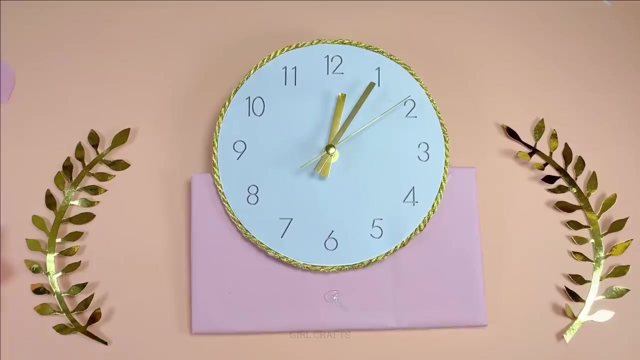 And I know you feel it too. I know you'll feel it too. Nothing's gonna stop me Living it up Dancing to the back beat, Turning it up. Nothing's gonna stop me Living it up Dancing to the back beat. Nothing's gonna stop me Living it up. 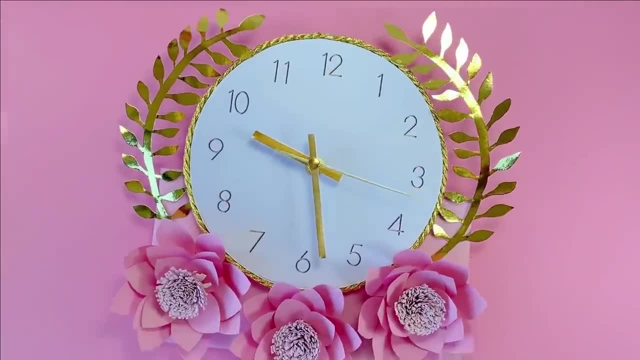 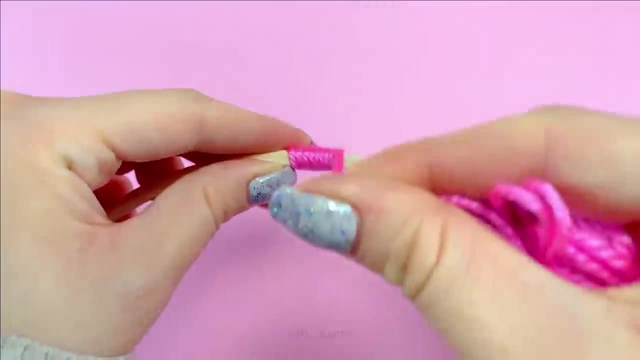 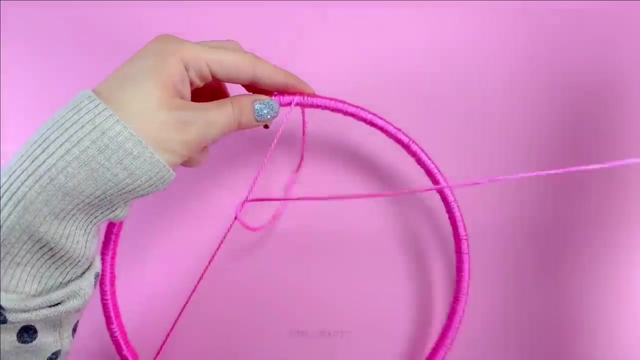 Dancing to the back beat, Turning it up. Nothing's gonna stop me- I know you'll feel it too- Dancing to the back beat, Back beat, back beat. Head's turned when I roll up, Spin around like a donut. Got a feeling that I can't lose. 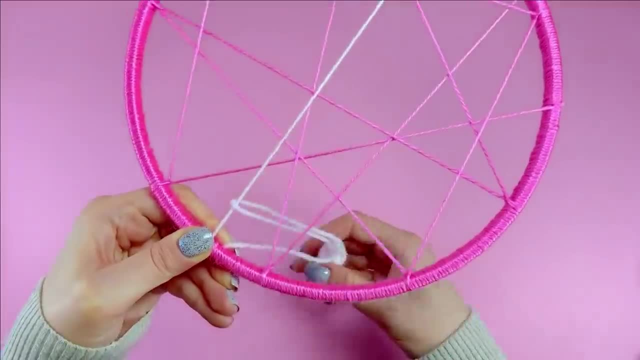 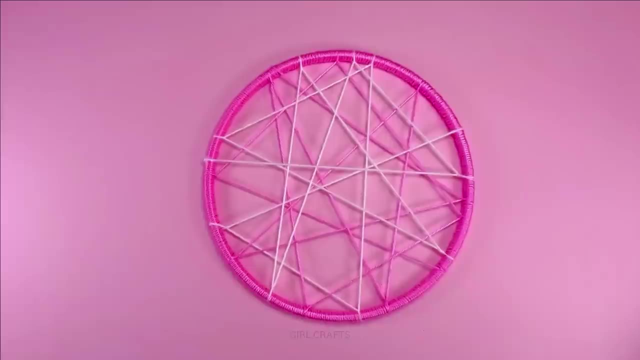 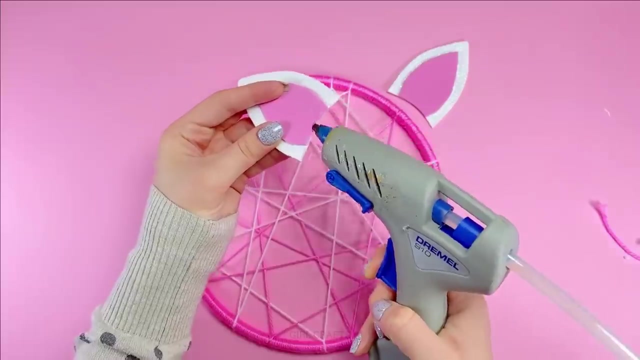 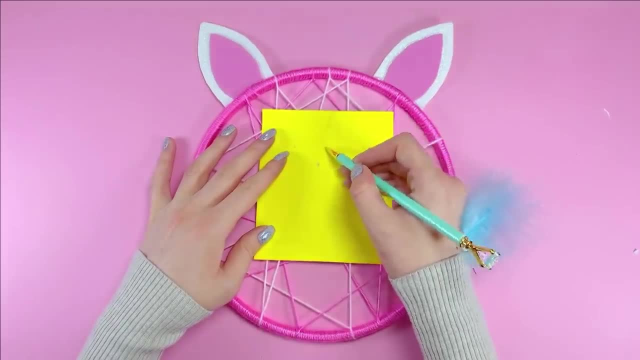 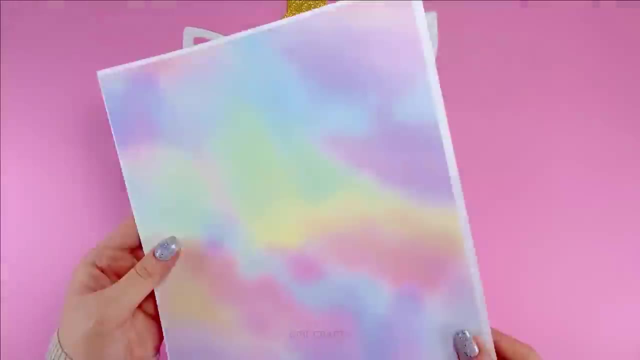 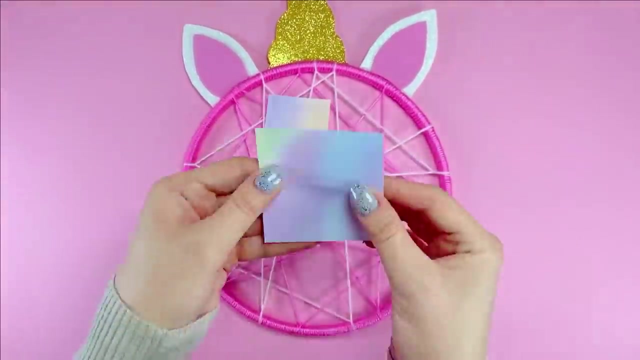 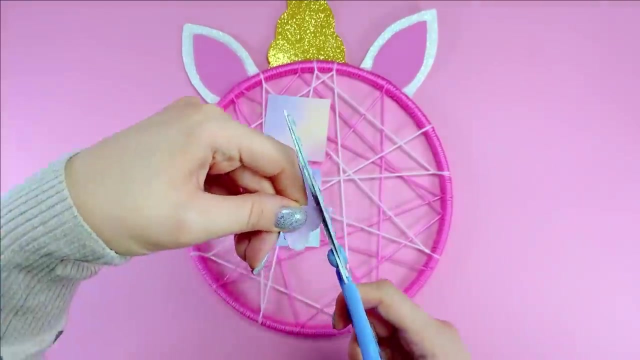 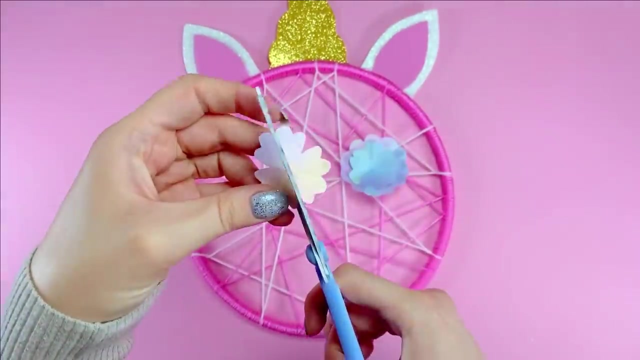 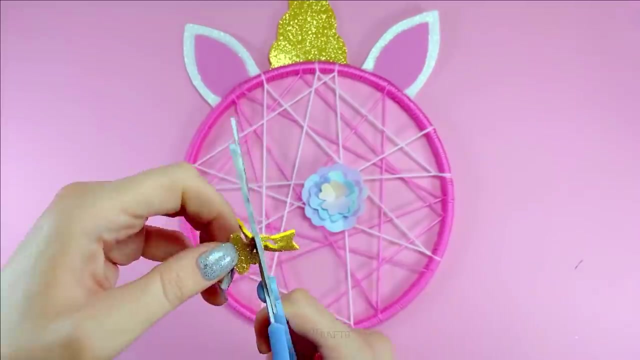 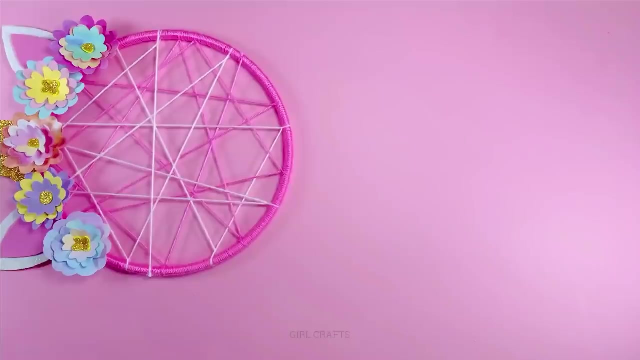 Can you feel it? Can you feel it Sky high on the good vibes Jumping? you can come too. Just tell me what you wanna do. I got something you can't explain In the metaphysical kind of way. There's something magic inside my veins. 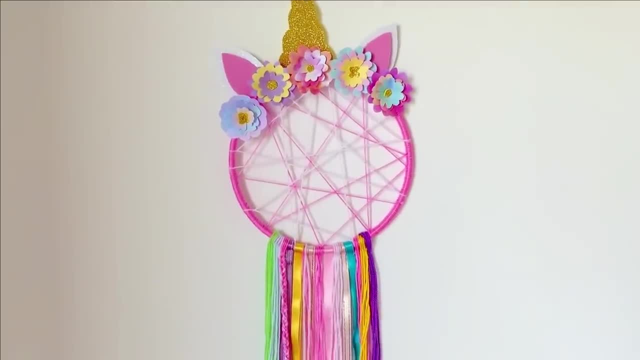 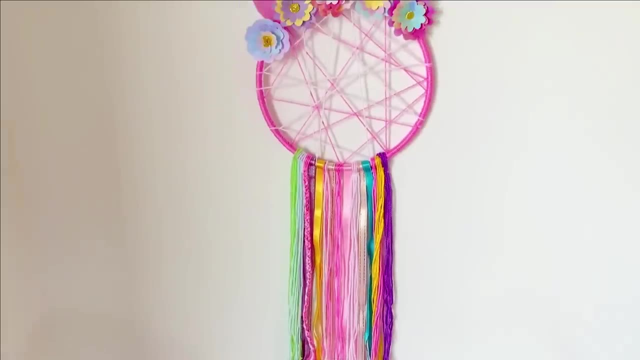 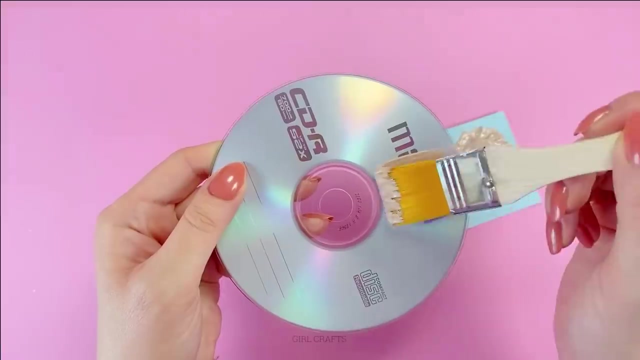 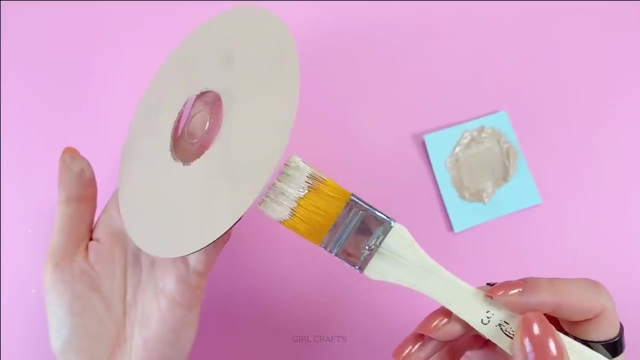 No matter what, I'ma do my thing. I'ma do my thing. Can you feel it? I wanna go high. All I gotta do is I'ma be Viva. I wanna have continue. Can you feel it? I gotta make it. Yeah, can you feel it? 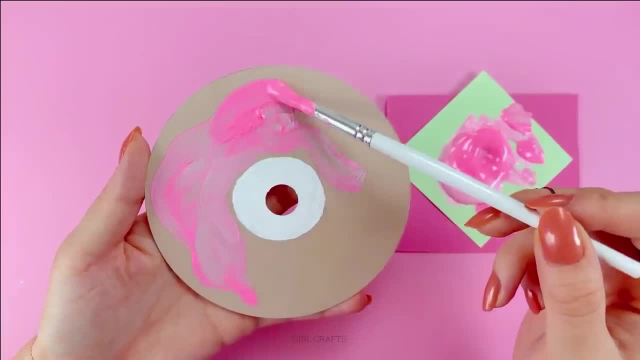 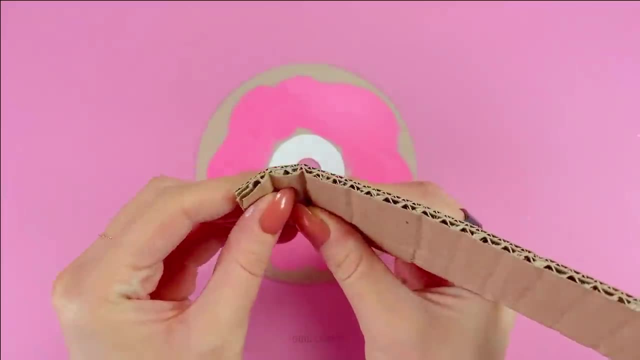 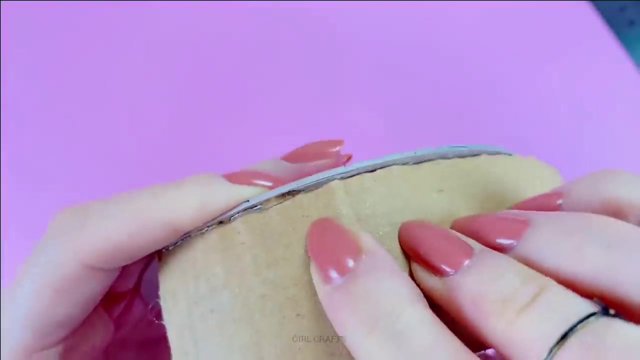 Yeah, can you feel it? Yeah, can you feel it? I'ma do whatever I should. I just need you, I need you, I need you. Can you feel it? Can you feel it? I got something you can't explain. Can you feel it? 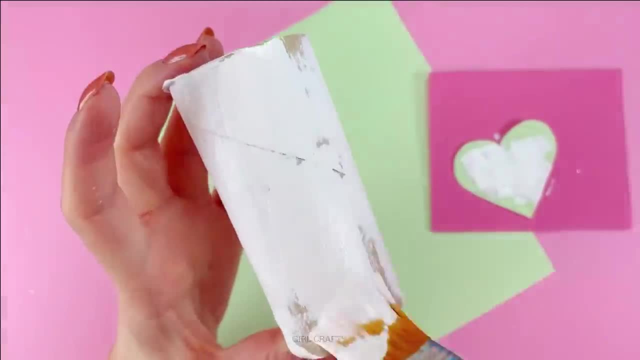 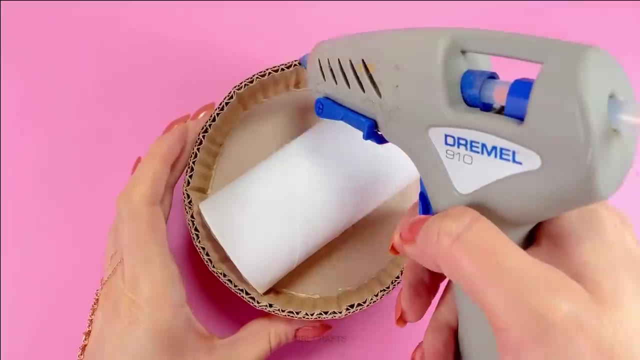 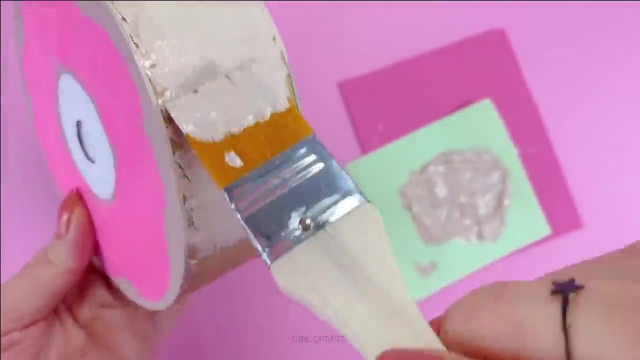 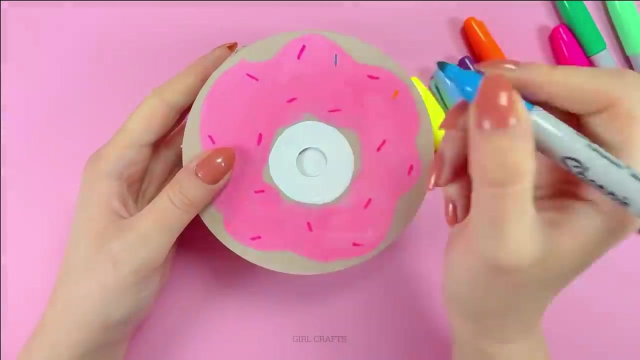 Invisible kind of brain. There's something magic inside my veins. No matter what, I'ma do my thing, I'ma do my thing. Can you feel it? Can you feel it? We got the moon. Can you feel it? We got the moon. Can you feel it? 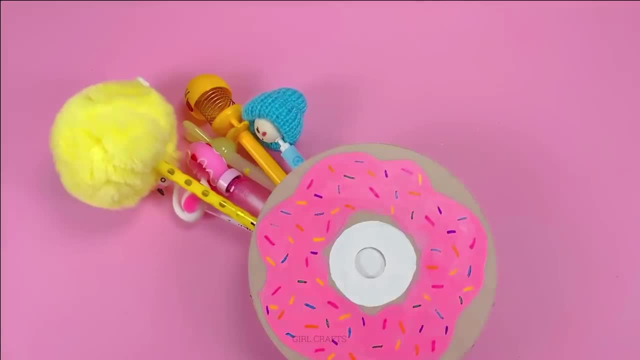 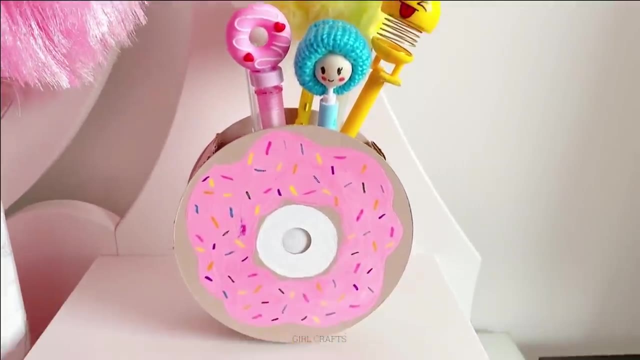 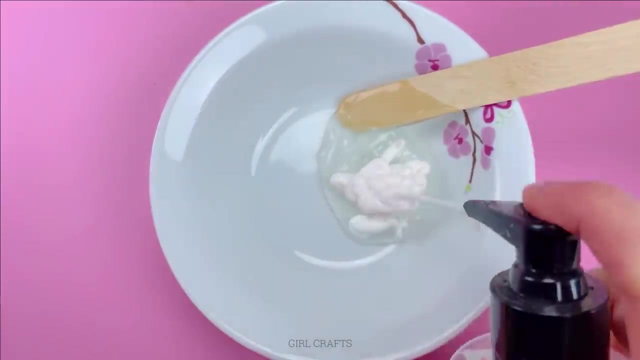 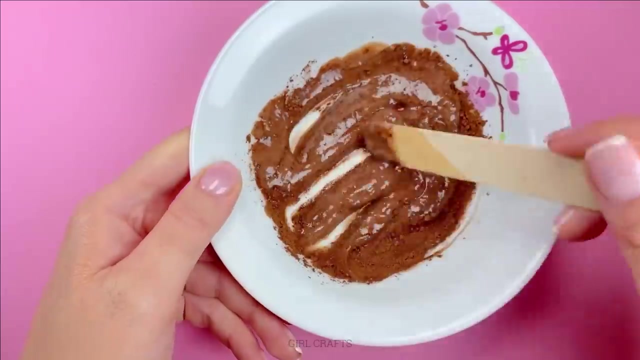 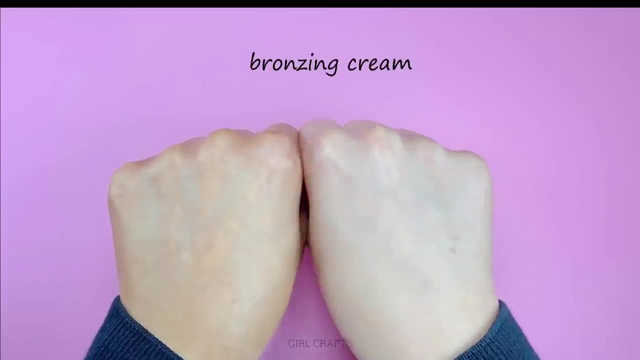 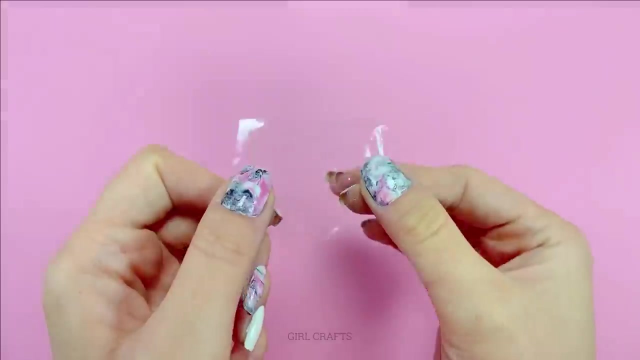 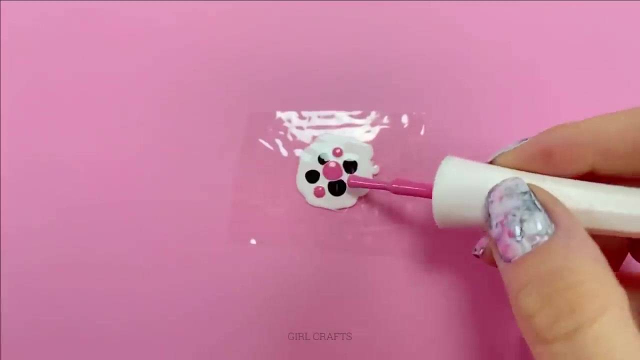 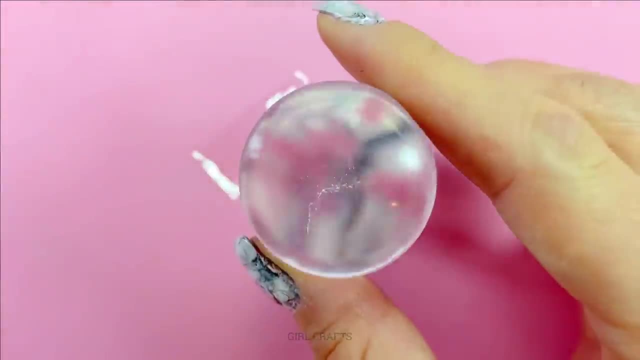 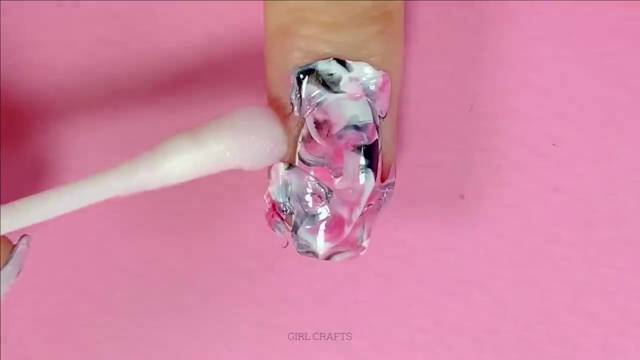 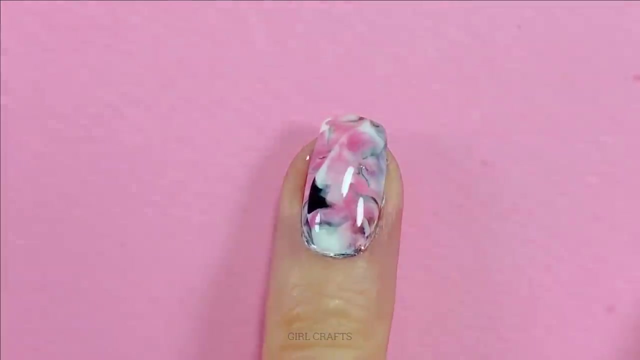 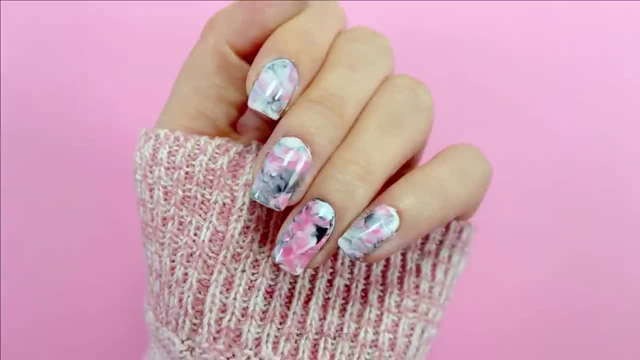 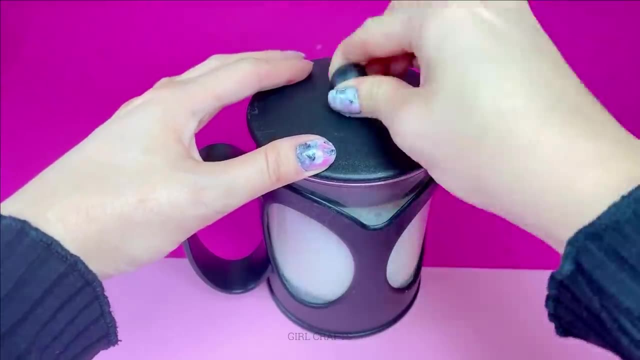 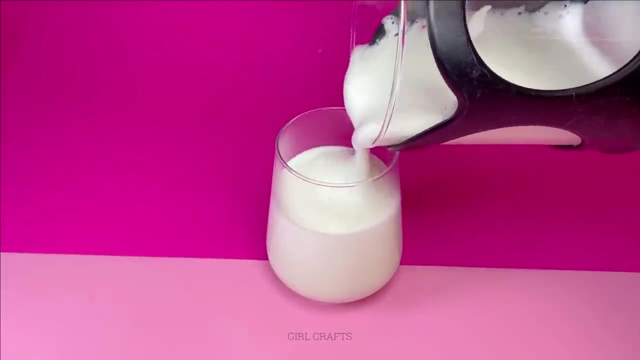 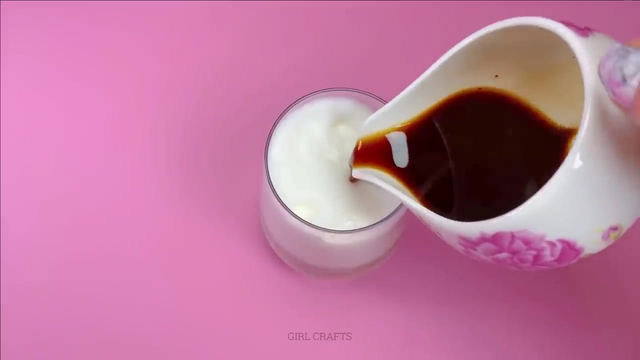 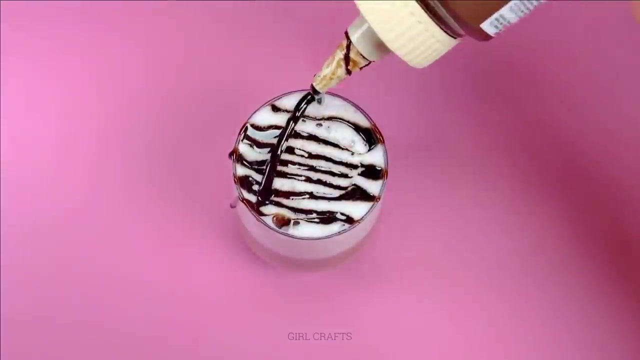 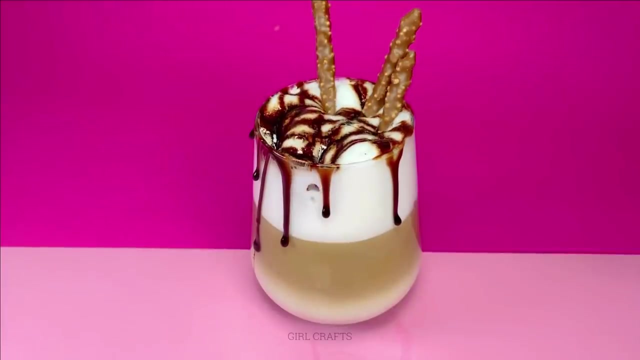 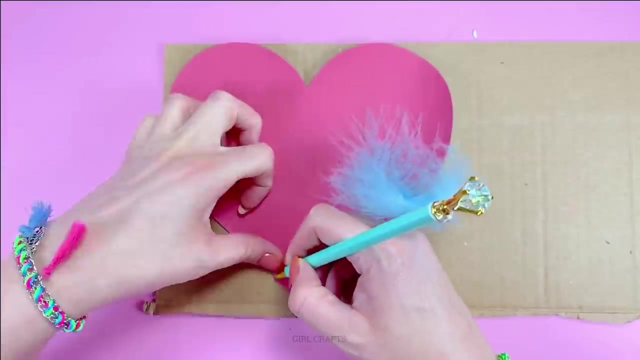 I say, hey, Shine like a star cause. you know that you are Circle through, Free my every kind. I just came to have a good time. Now everybody inside Feels good. on cloud nine: Yeah, everything you see right here, right now I've made look good. 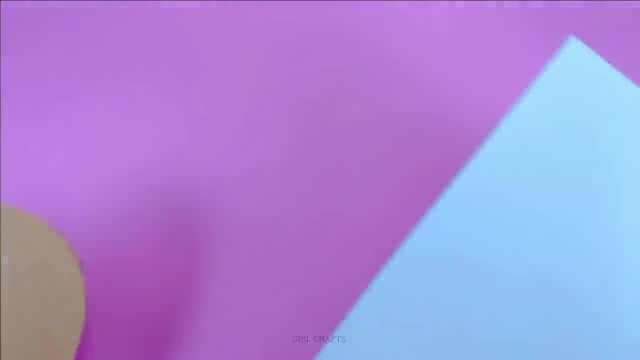 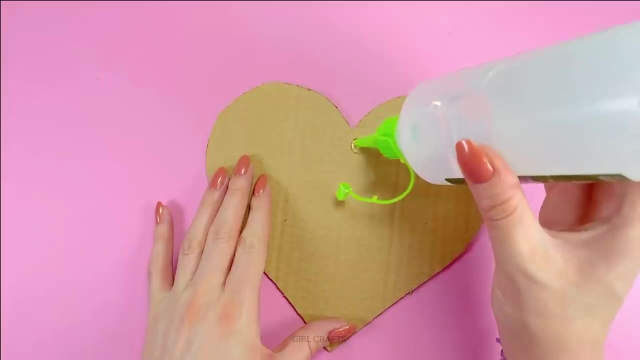 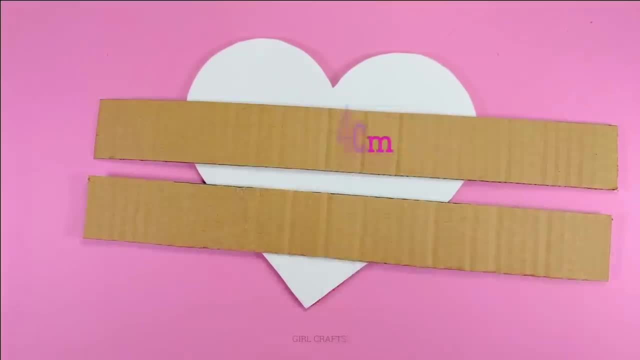 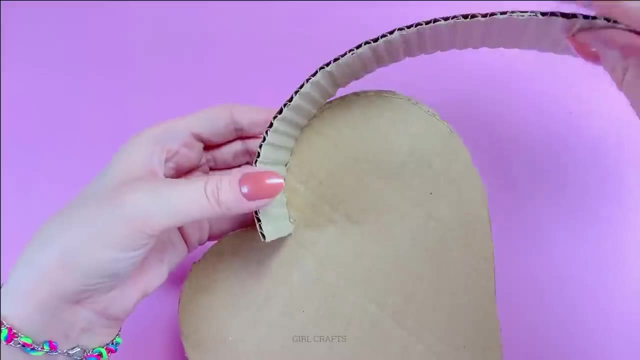 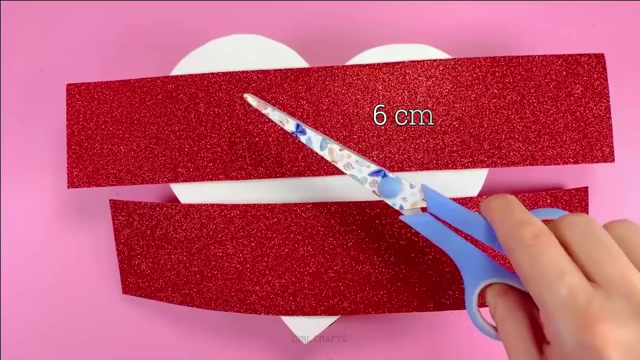 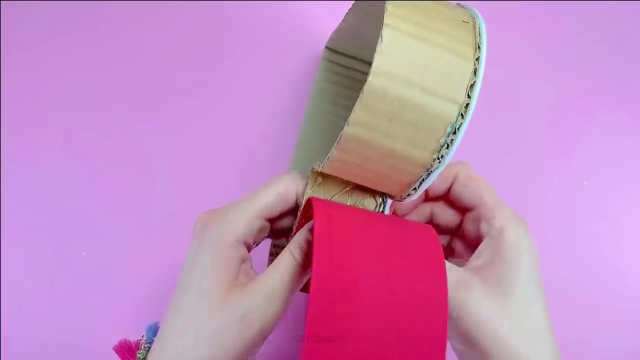 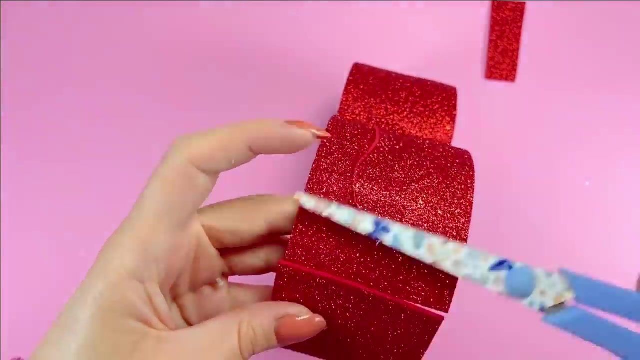 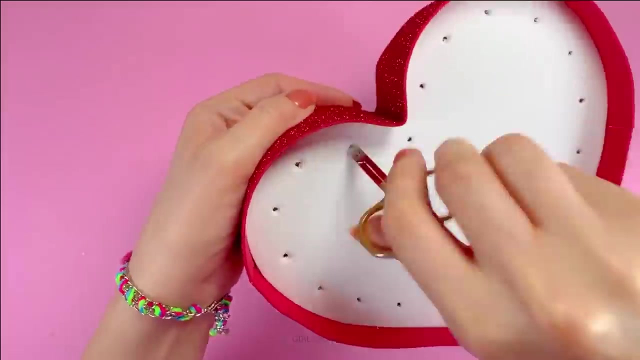 Oh, oh-oh, oh, oh, oh. So here I am, One-off a kind And bottom line. I say, hey, Shine like a star cause. you know that you are, So come through, Free my every kind. I just came to have a good time. Now everybody hands high. 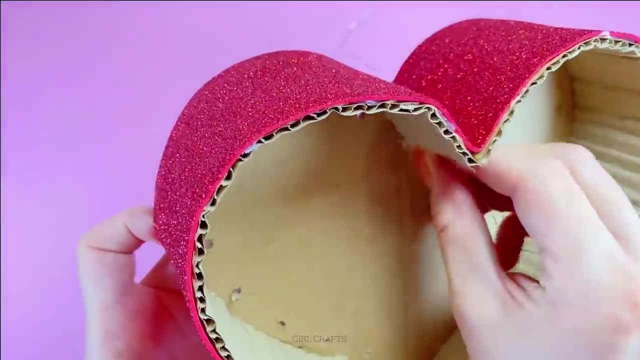 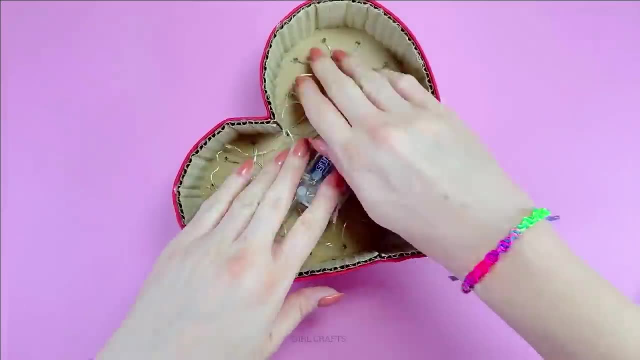 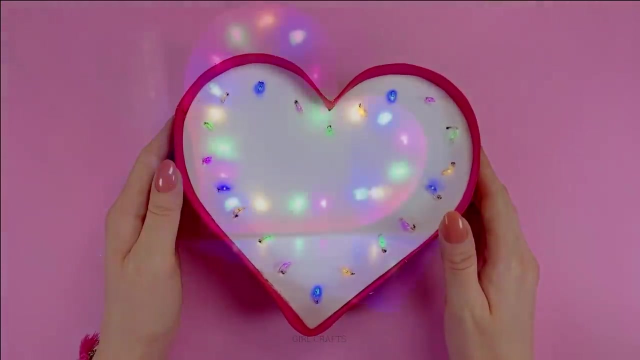 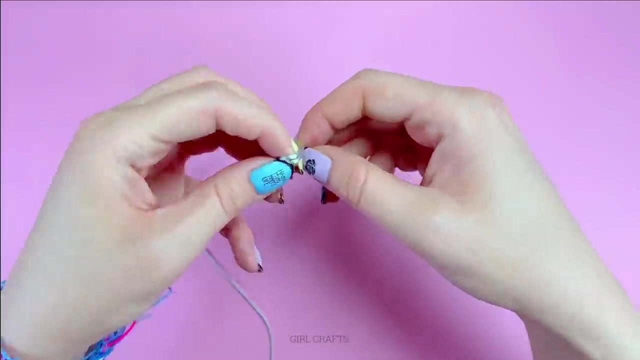 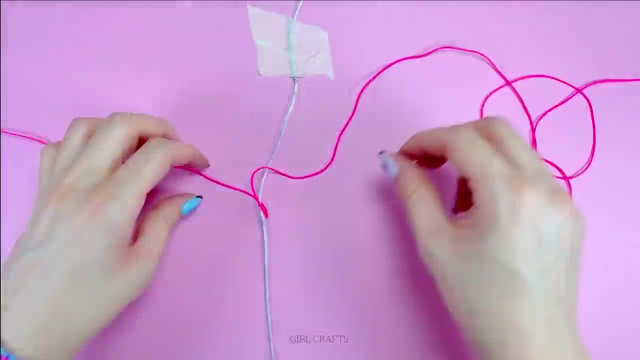 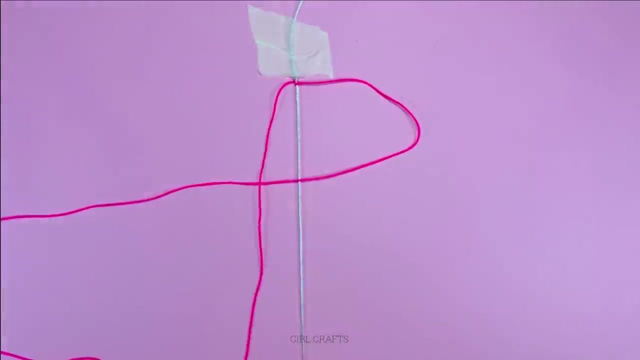 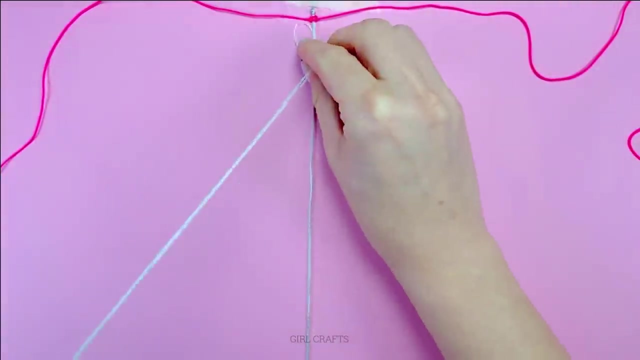 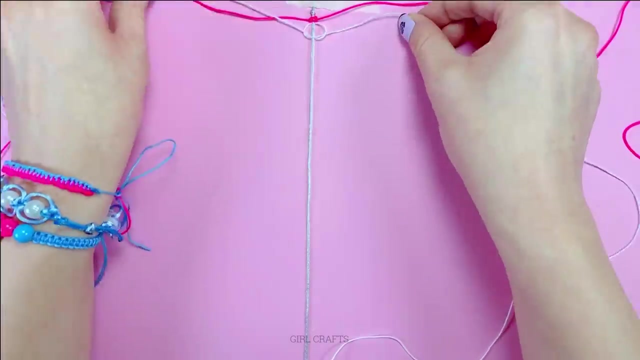 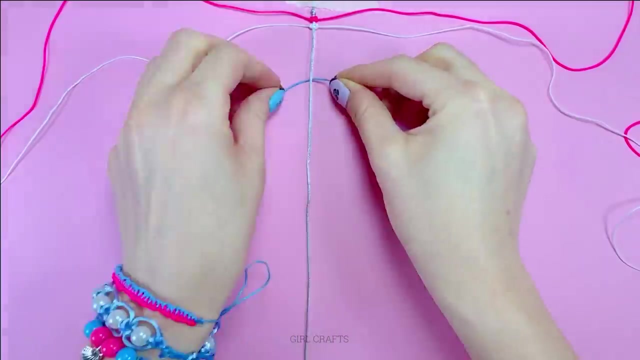 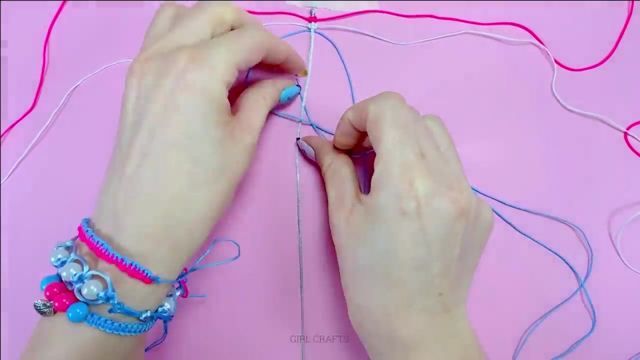 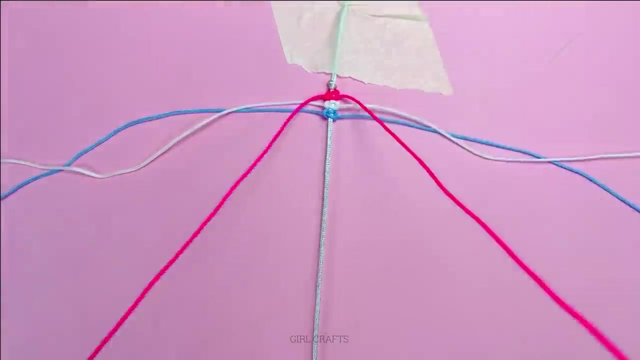 Feels good on a hot night. Everything you see right here right now. I just came to have a good time Now. everybody hands high, Feels good on a hot night. Everything you see right here right now. Woah, oh, Woah, oh, Woah. oh, I know I let love slip away. 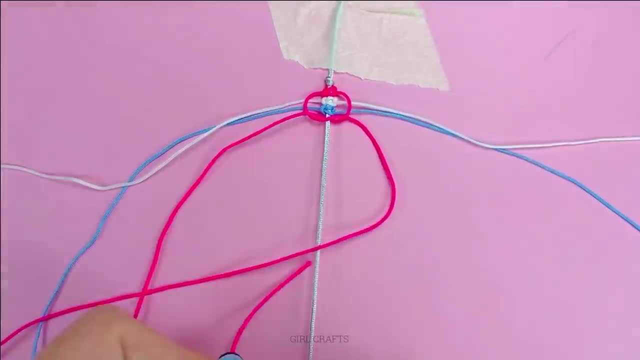 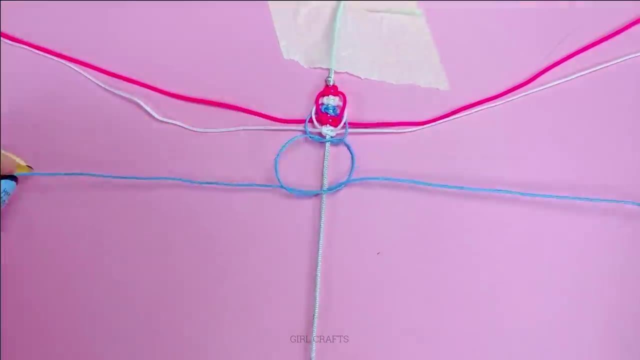 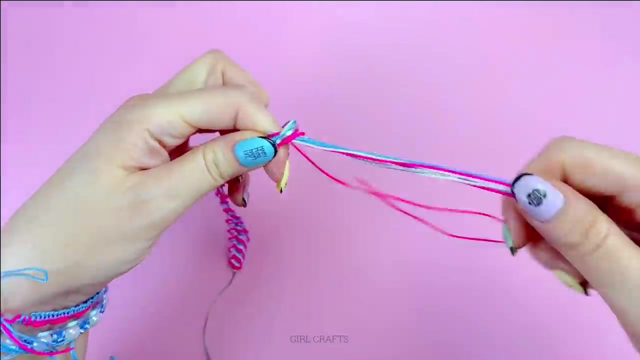 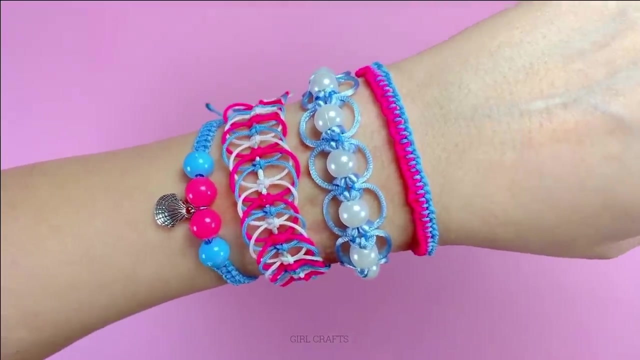 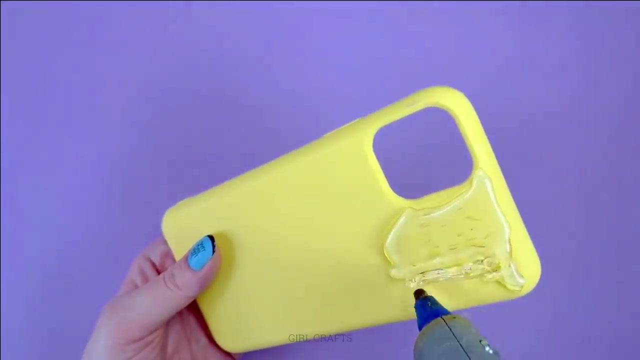 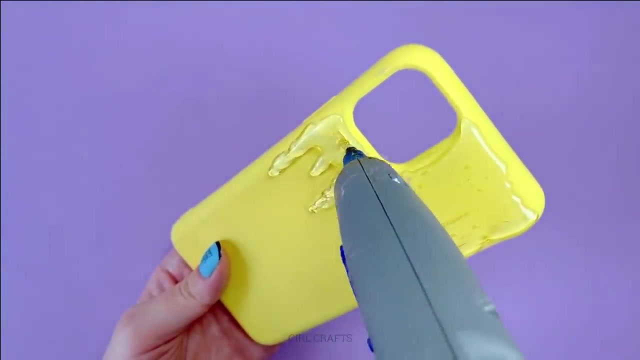 And I know you're done with me, But when I see your pretty face I can barely breathe. We talk as if we never met And you know that's fine with me. I just pretend I'm innocent Till I watch you leave, Cause you're my enemy, You're my habit. 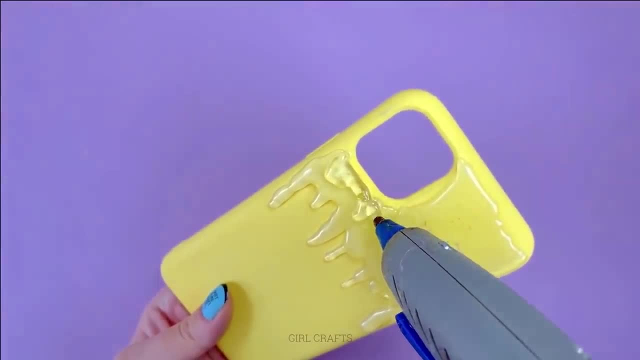 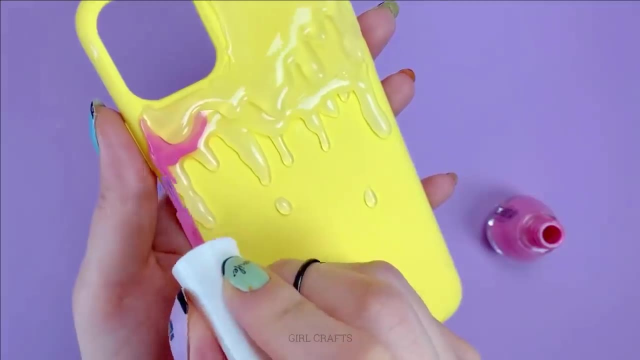 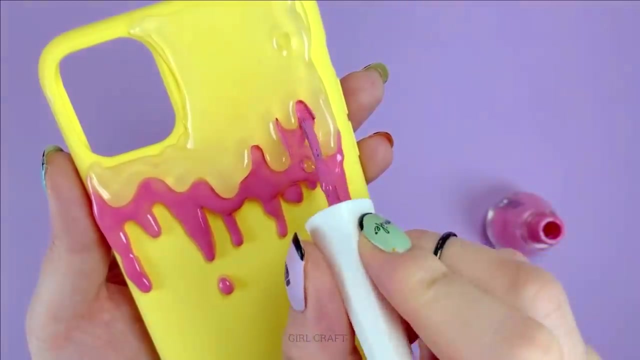 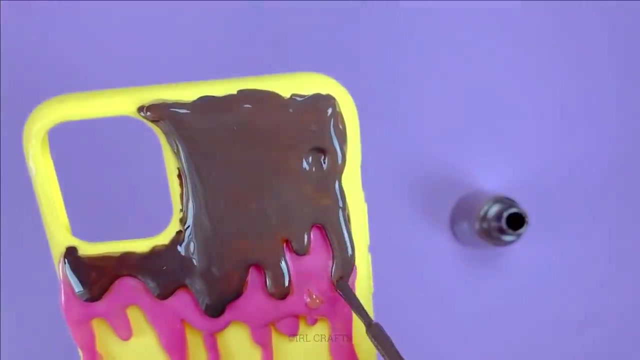 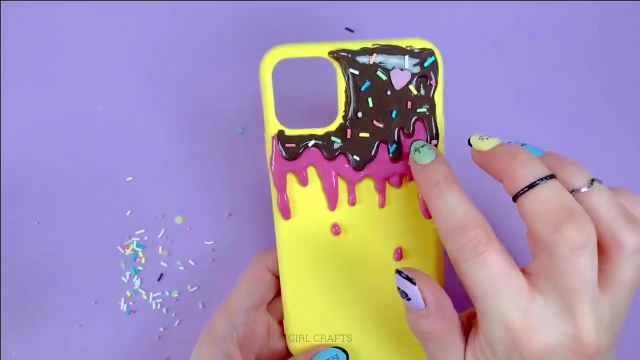 I can't let you go. You're my habit. Yeah, you feel like home. I know you mean it When you say goodbye, But I don't feel it. Looking in your eyes, I know you're done with me. Never ask how long it's been And you never say his name. 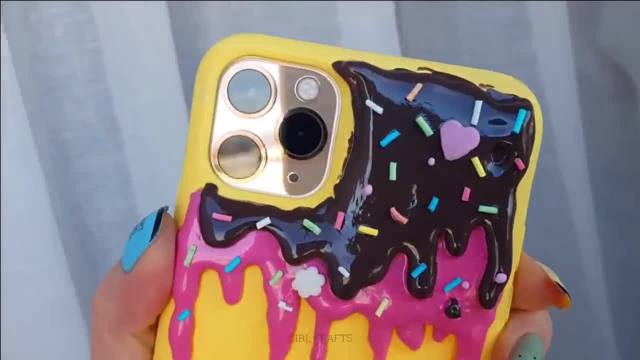 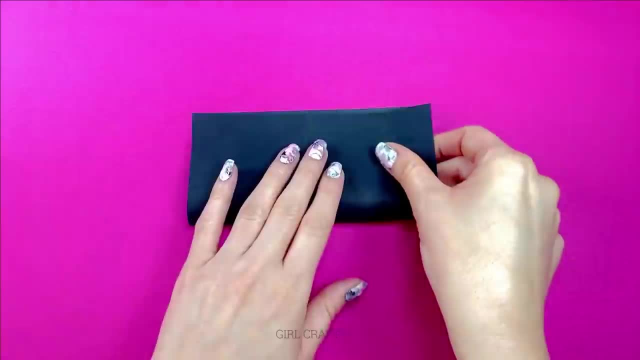 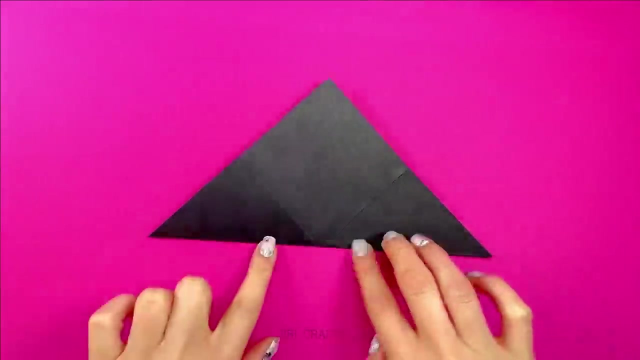 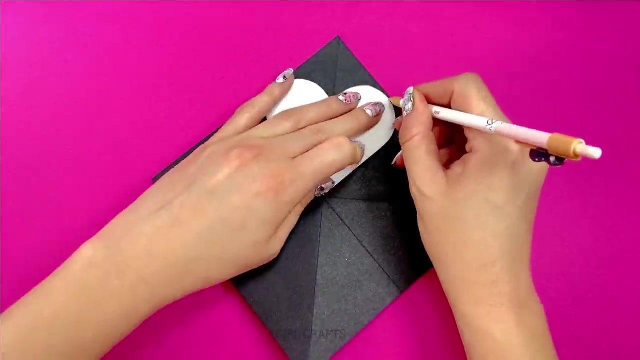 You know it leaves me wondering If he's gone away. I know it's all inside my head, These mixed up memories, But I'm happiest when we forget. You don't belong to me, Cause you're my habit. Yeah, you're done with me. I can't let you go. 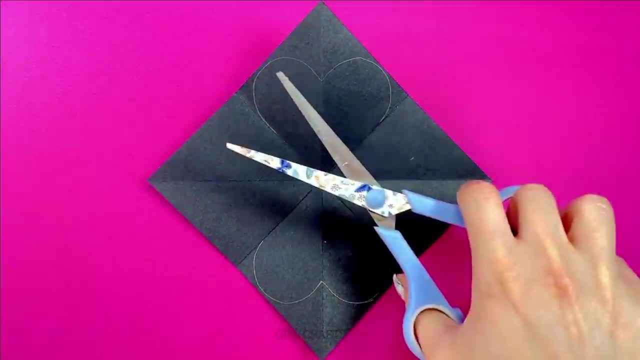 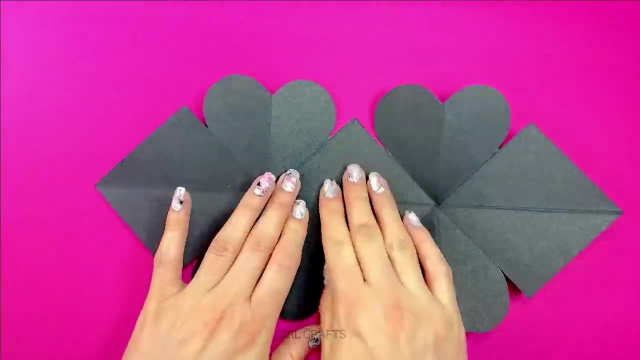 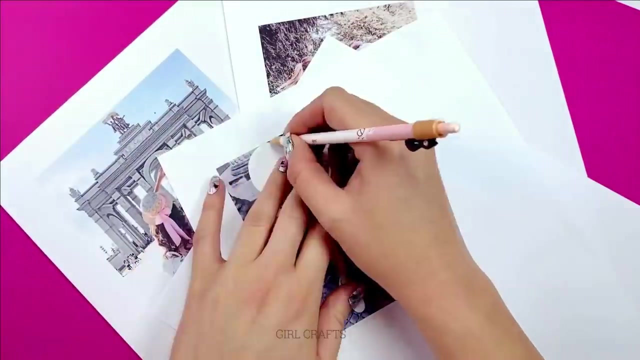 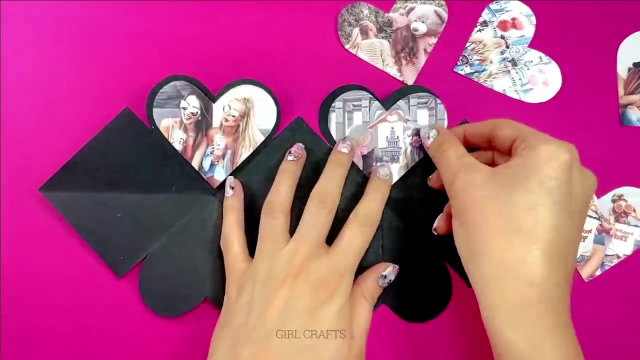 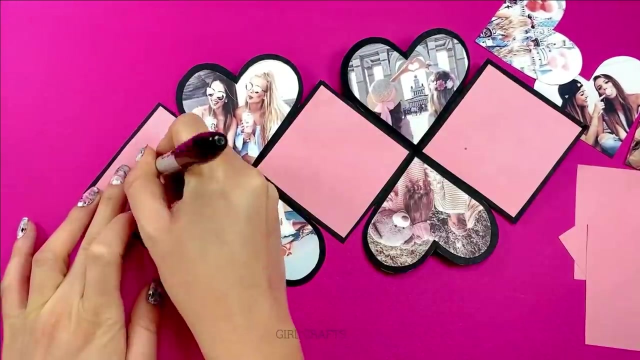 You're my habit. Yeah, you feel like home. I know you mean it When you say goodbye, But I don't feel it Looking in your eyes. I know you mean it. I know you mean it When you say goodbye. I know you mean it When you say goodbye. 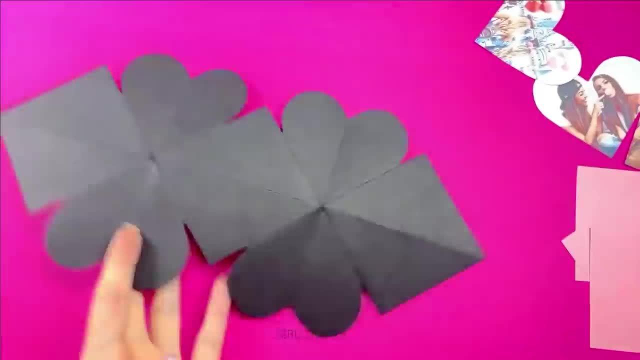 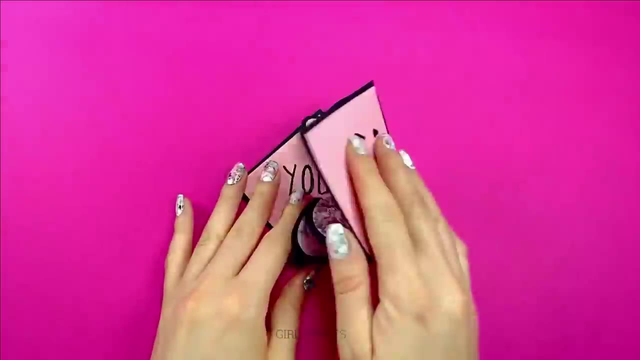 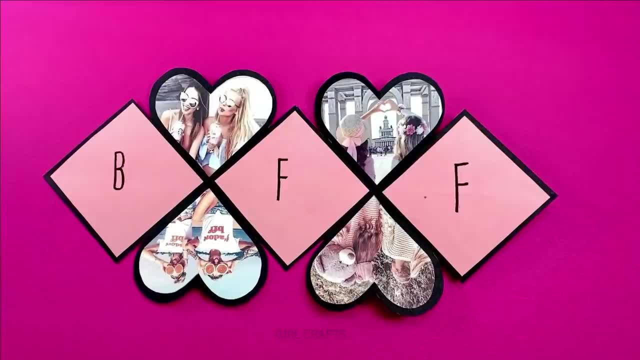 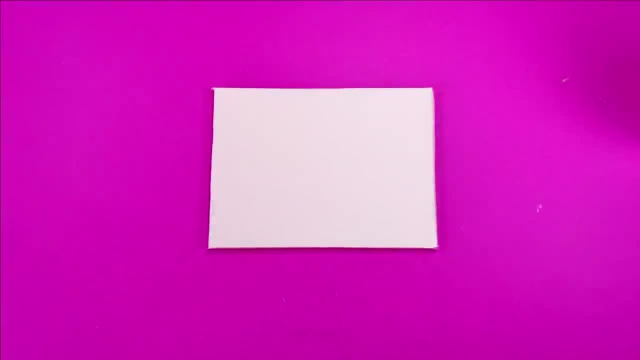 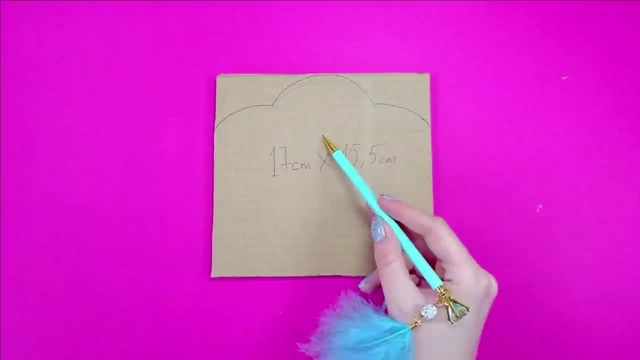 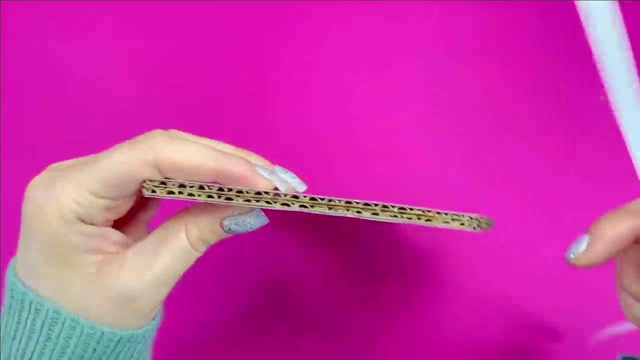 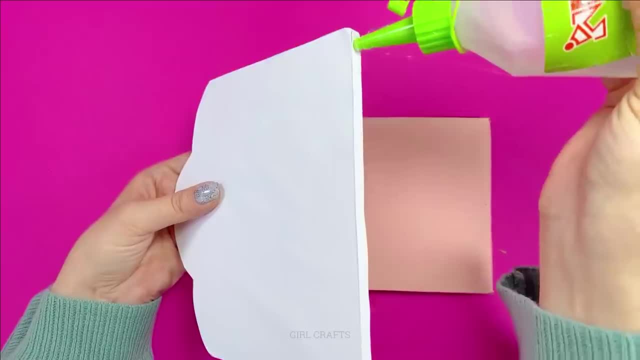 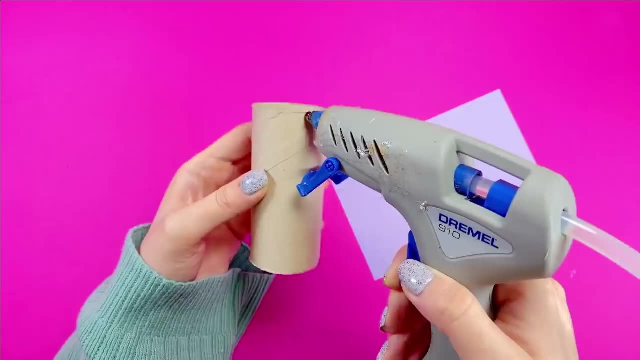 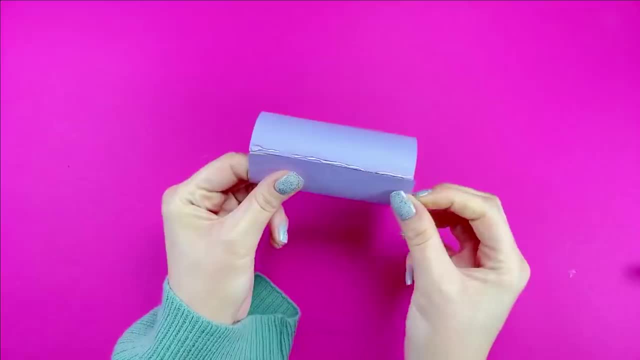 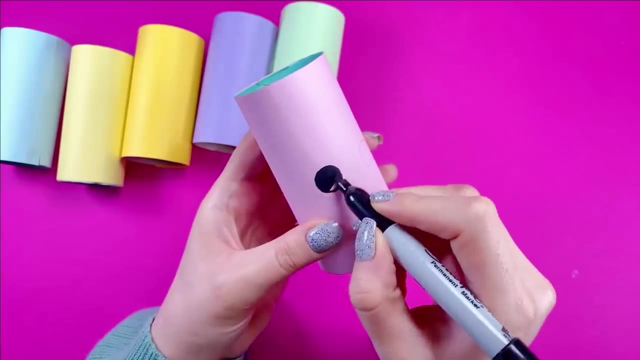 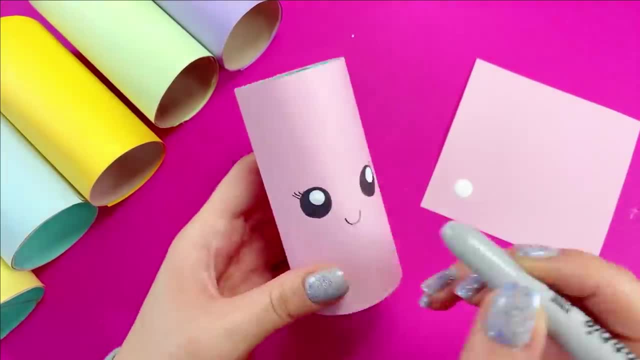 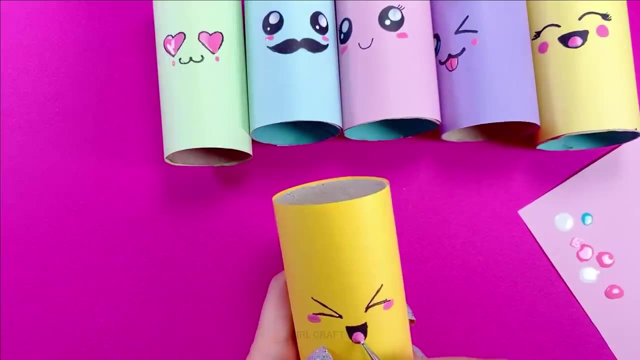 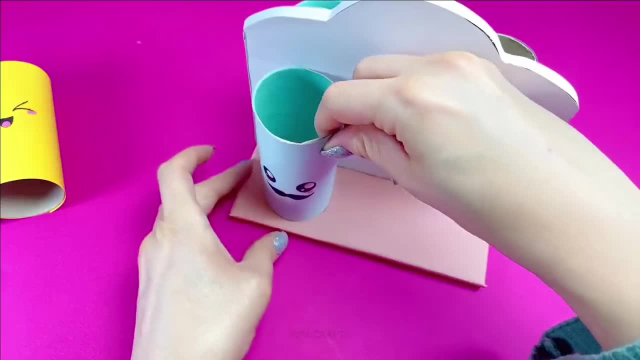 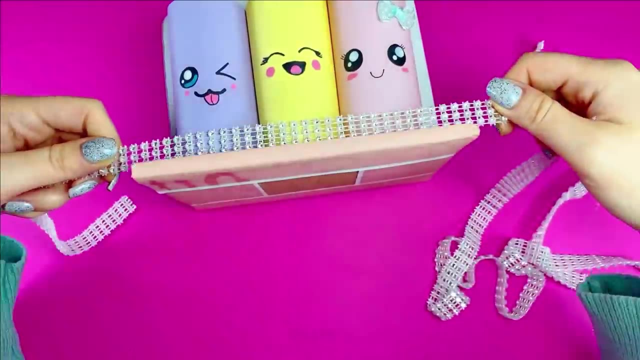 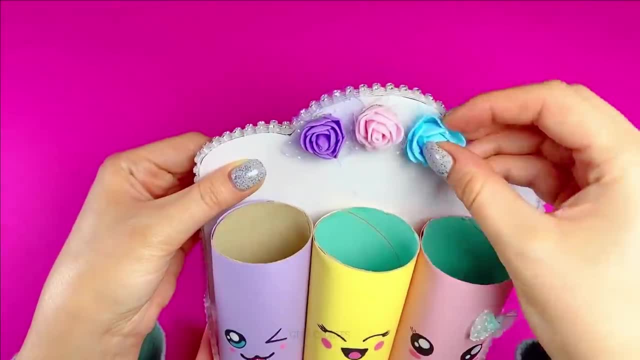 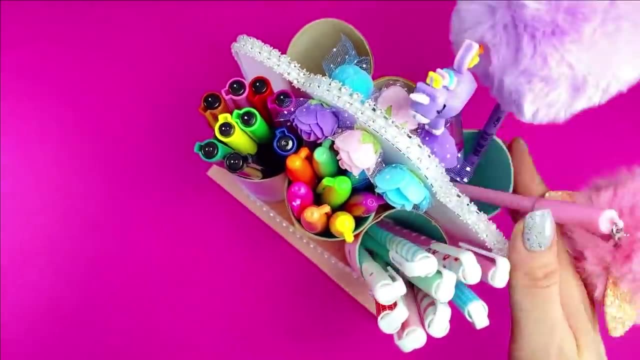 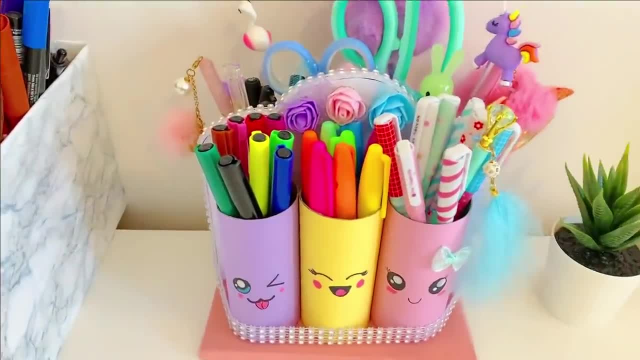 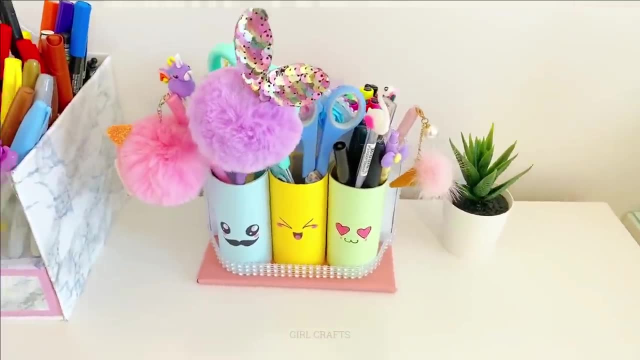 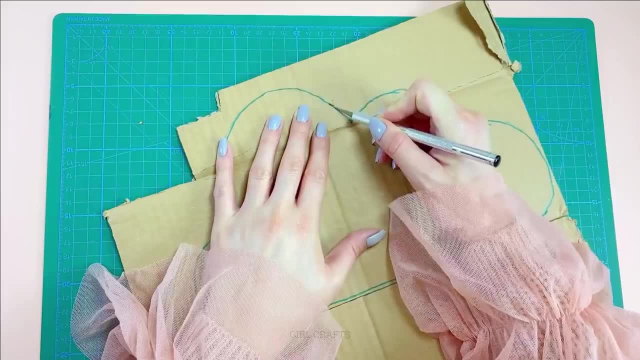 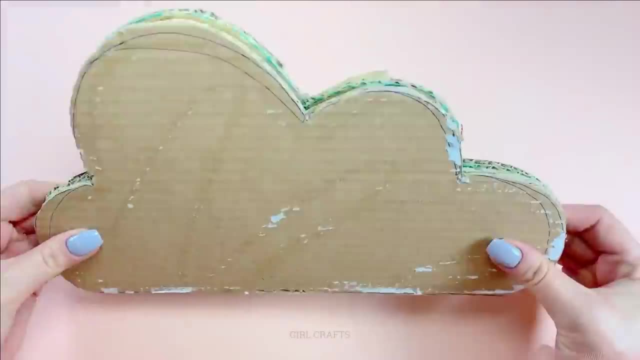 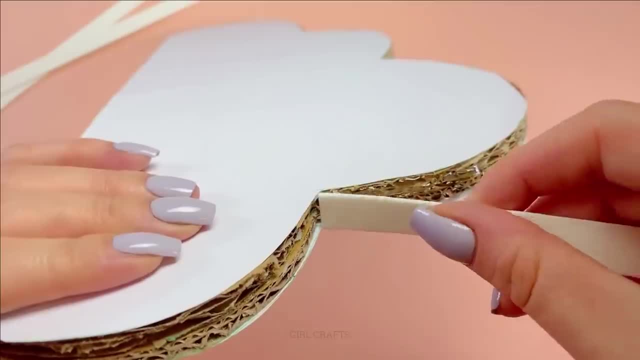 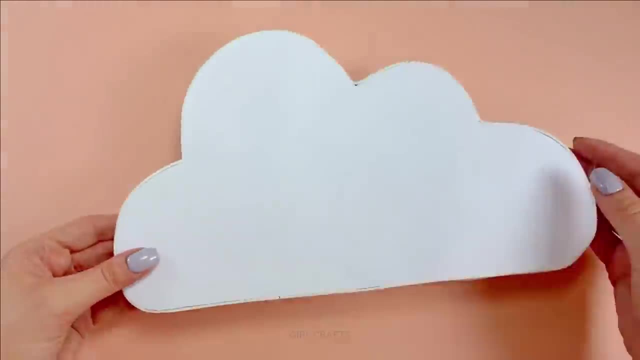 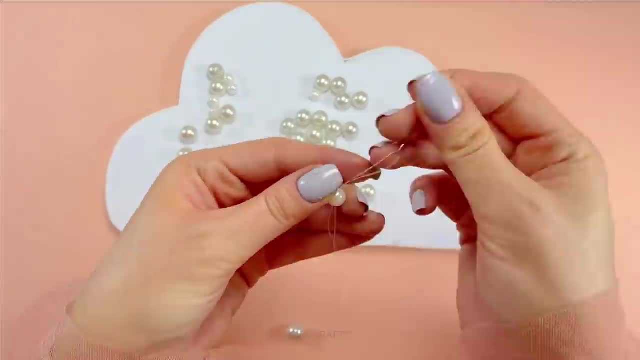 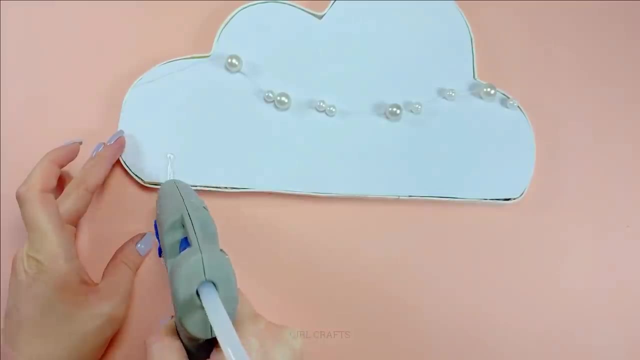 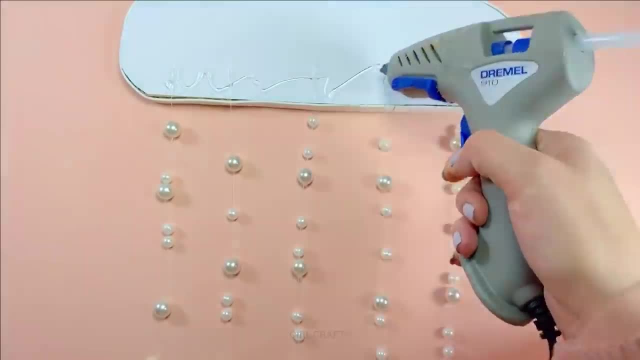 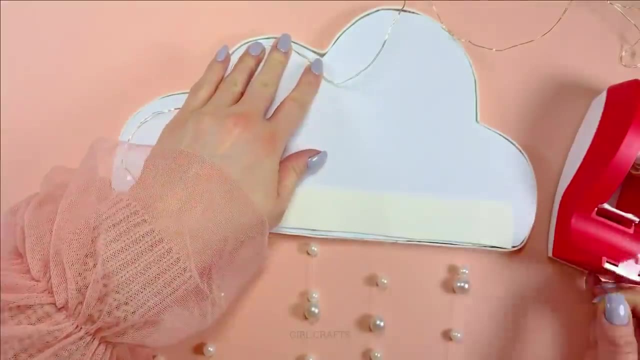 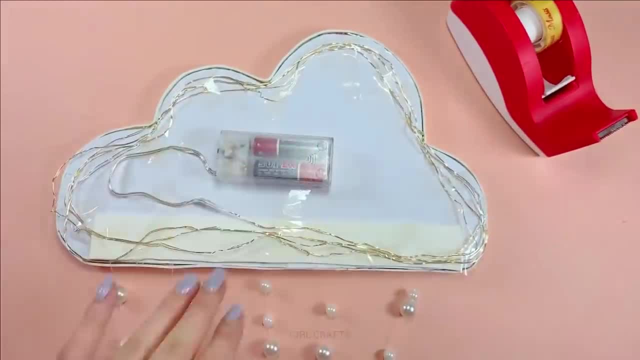 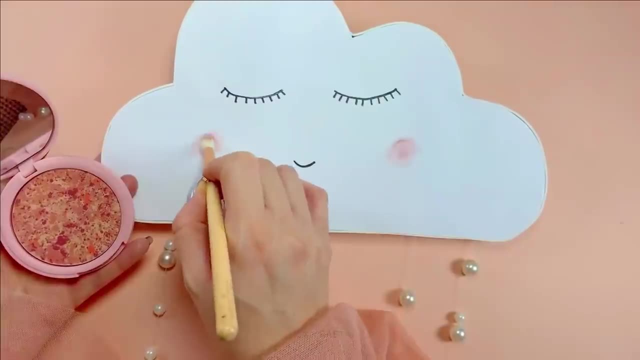 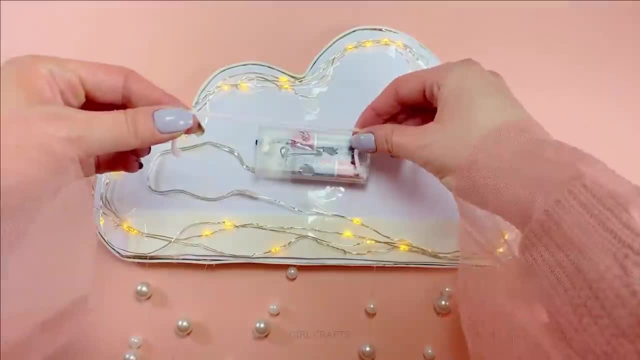 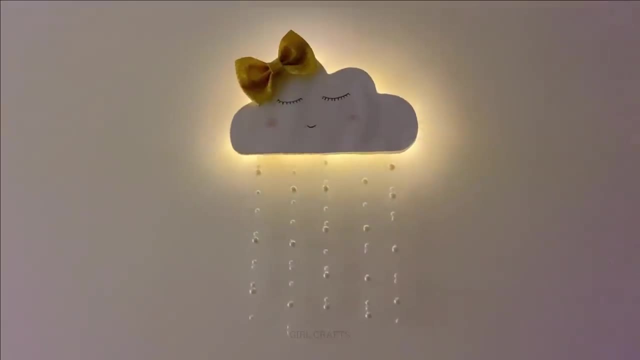 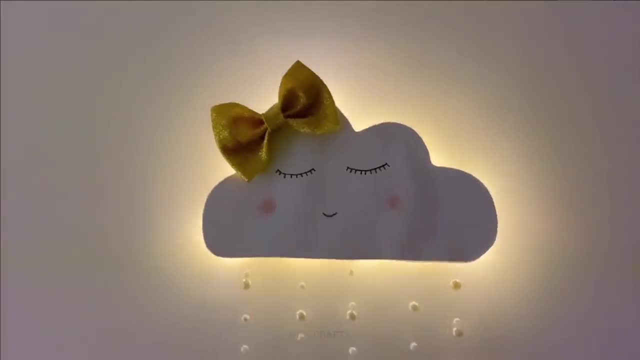 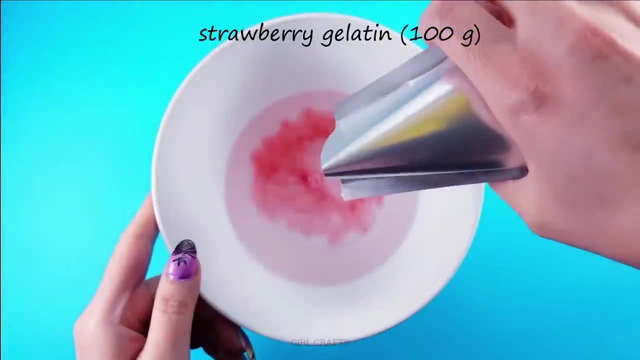 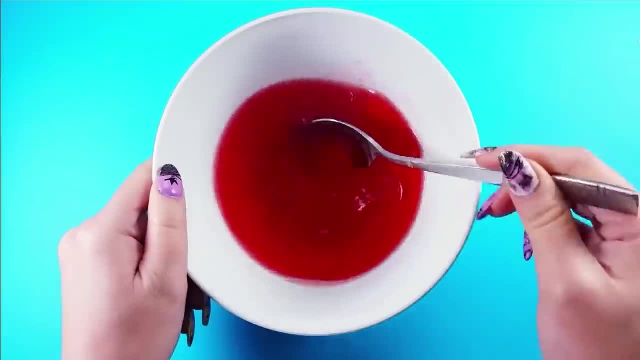 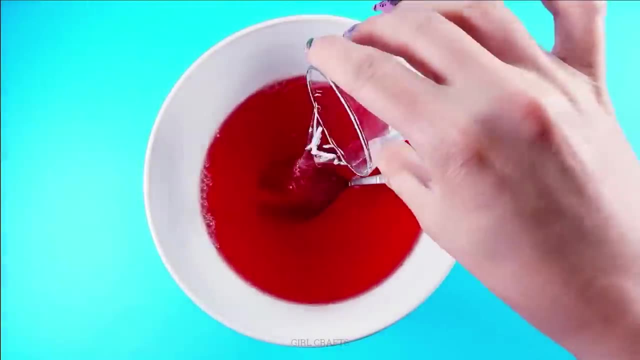 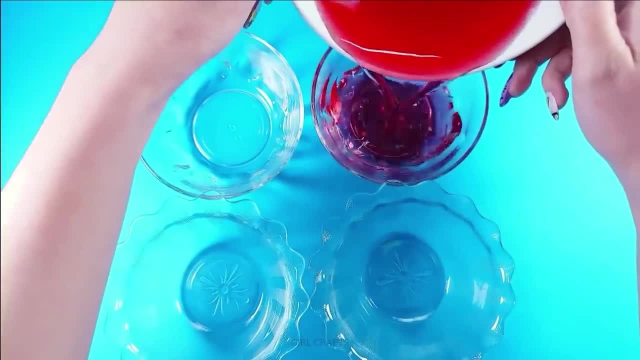 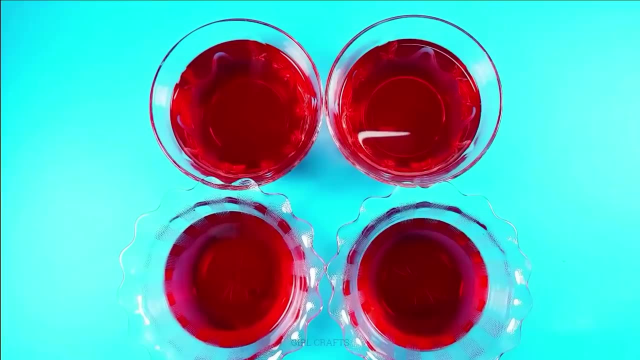 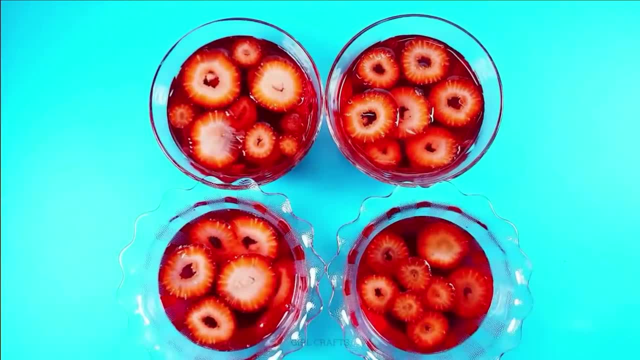 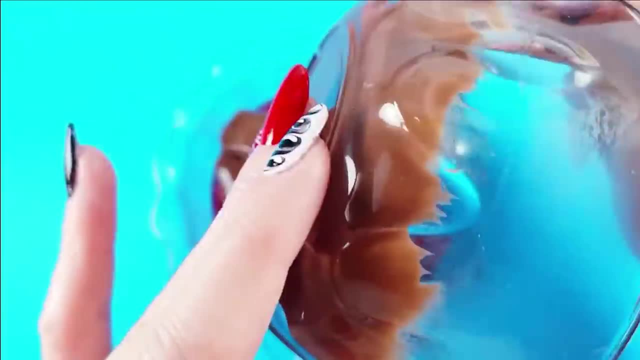 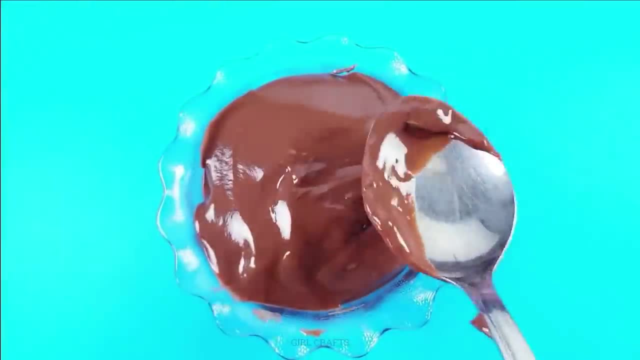 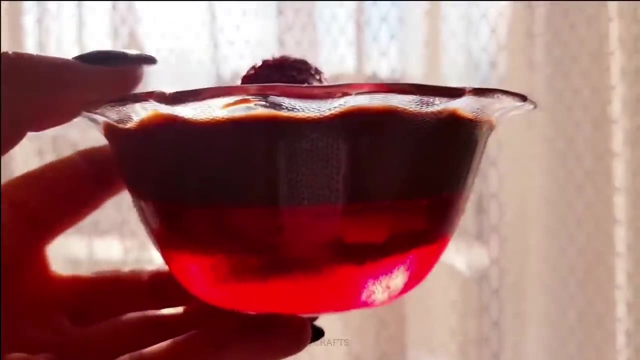 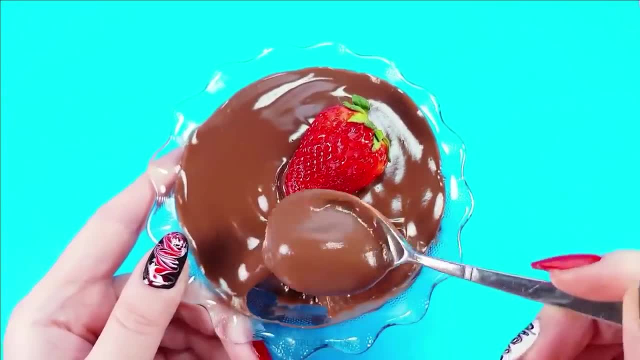 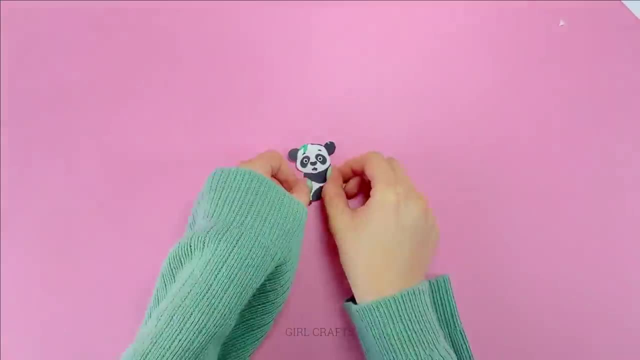 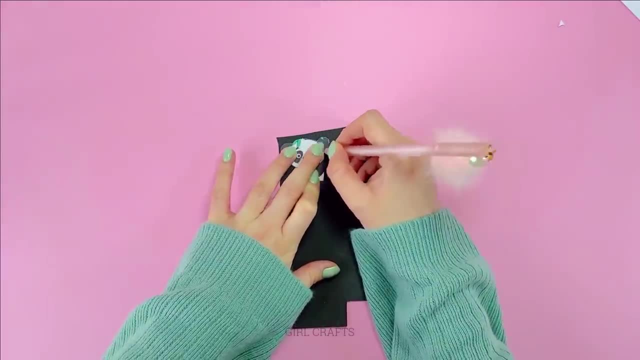 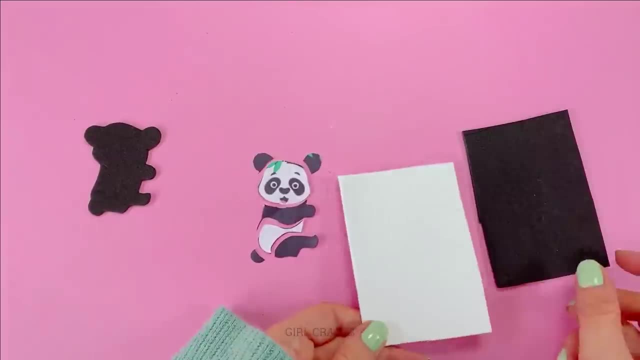 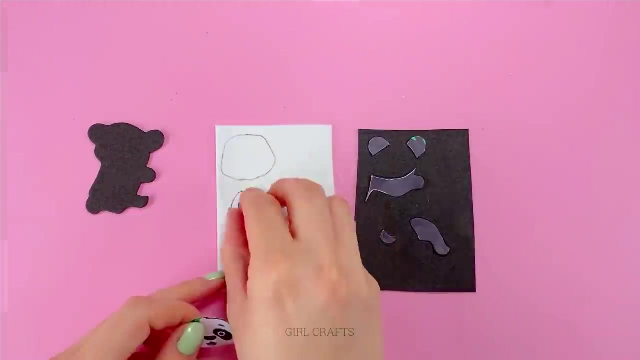 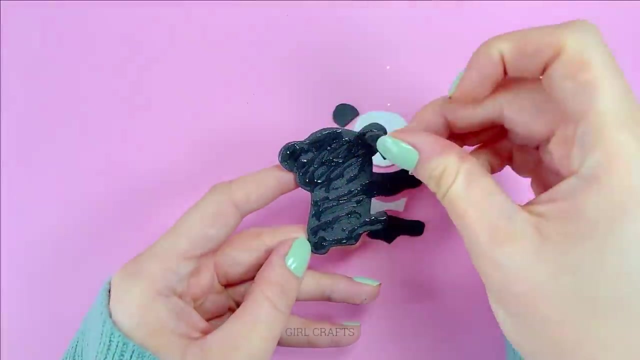 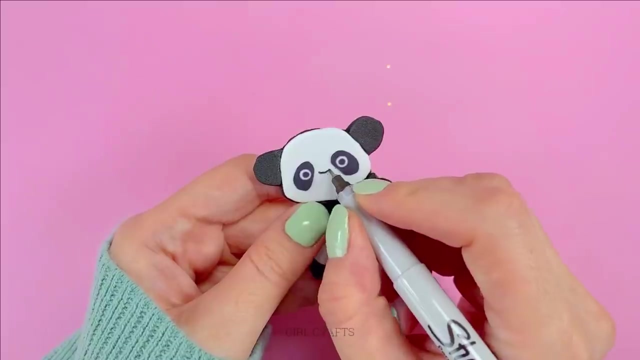 Me tonight. So just break Your life. We'll steal back your heart Tonight And win a way. Arrive With guns on your very tight. We'll take them all down My back Against the wall. now I go down In a hill of fire For you to love tonight. 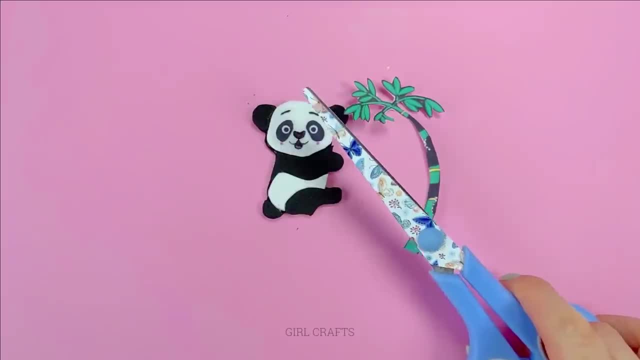 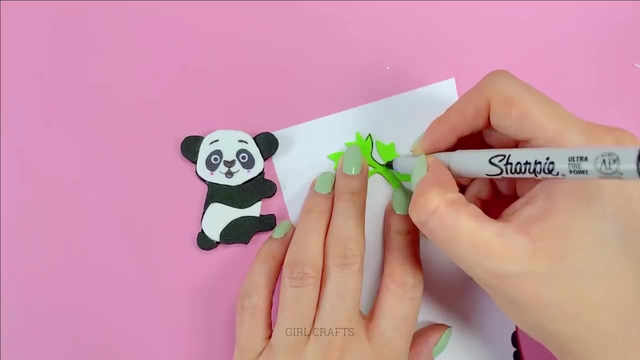 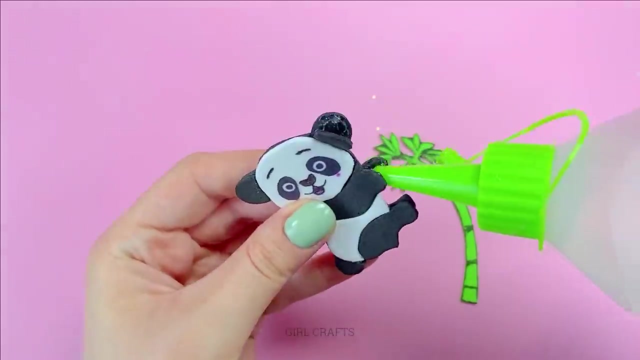 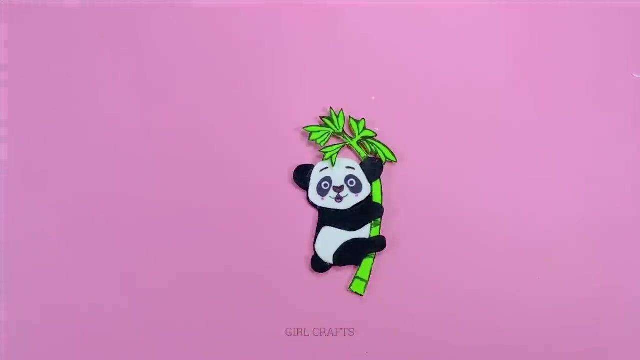 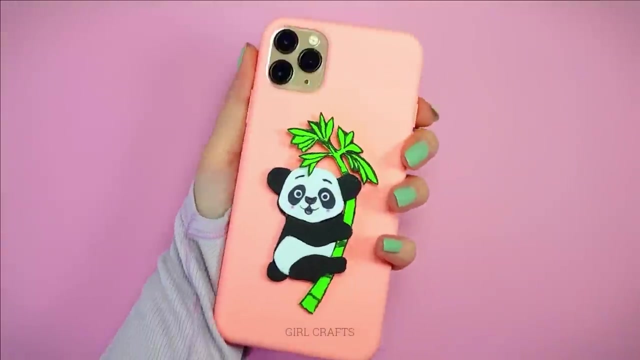 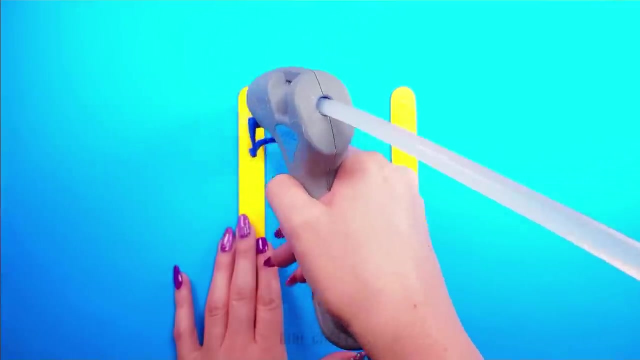 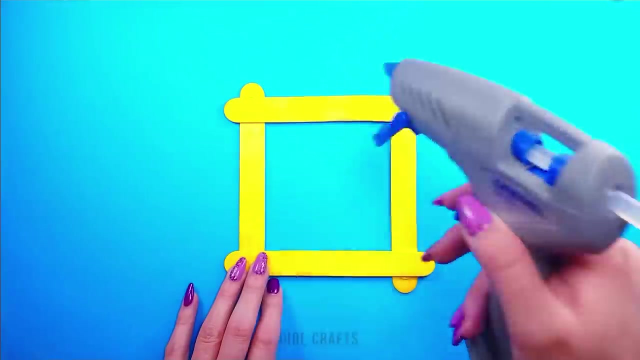 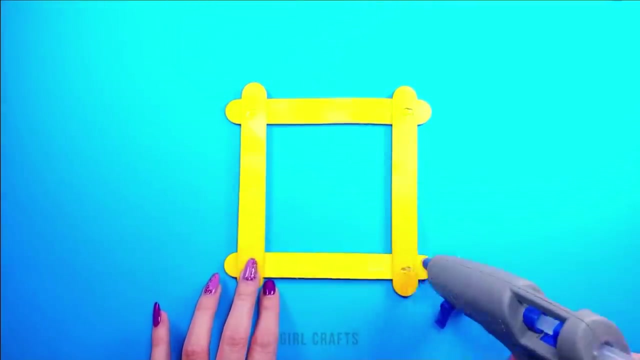 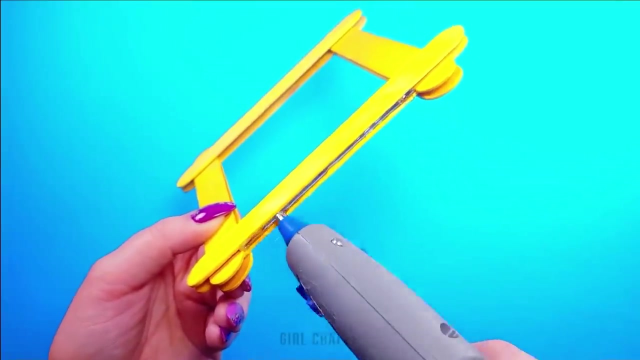 I'll take the fall now. I think we gotta run now. They're coming, So let's hide away Into the light Tonight, So just Break Your life. We'll steal back your heart Tonight And win a way. Arrive With guns on your very tight, So just break. 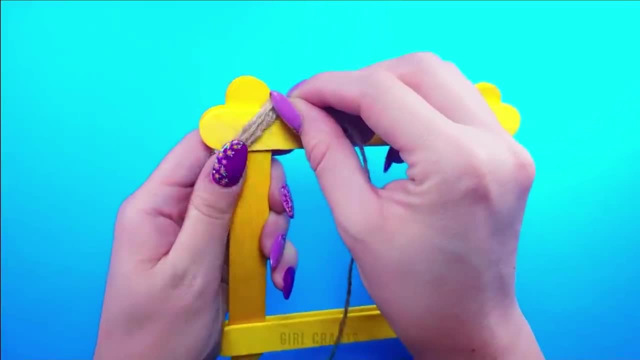 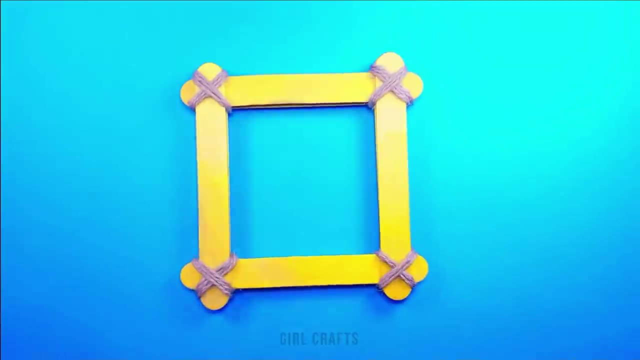 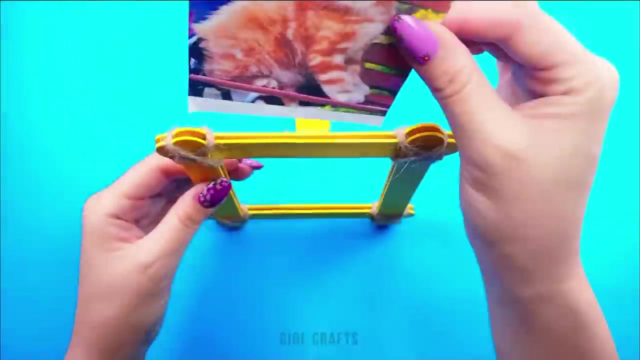 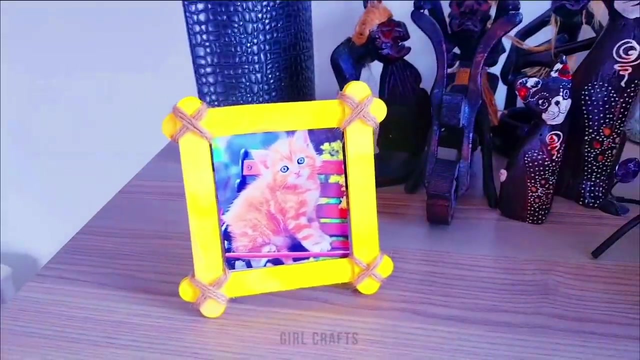 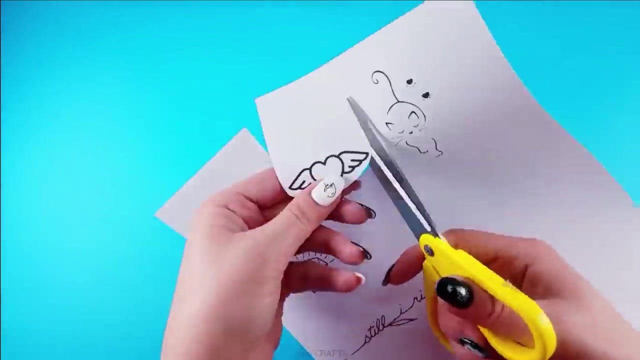 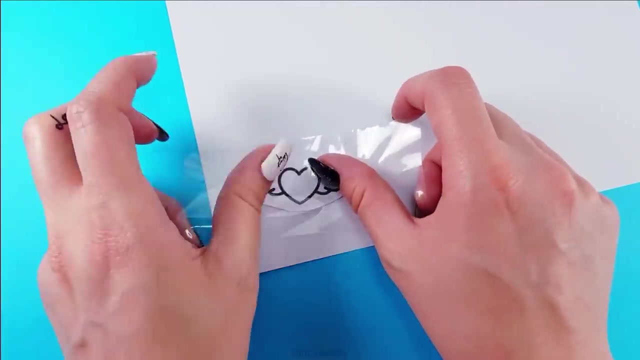 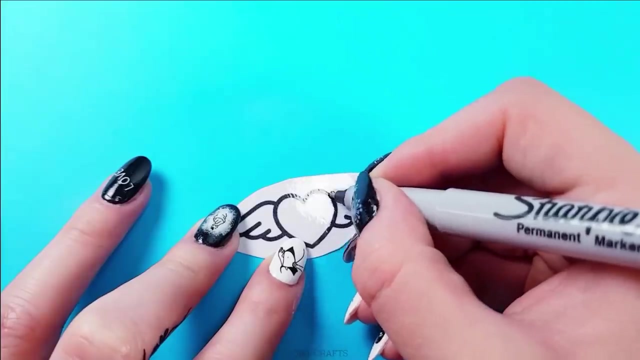 Your life. We'll steal back your heart Tonight And win a way: Arrive With guns on your very tight. Just break Your life. We'll steal back your heart Tonight And win a way: Arrive With guns on your very tight- I'm being honest- With guns on your very tight. 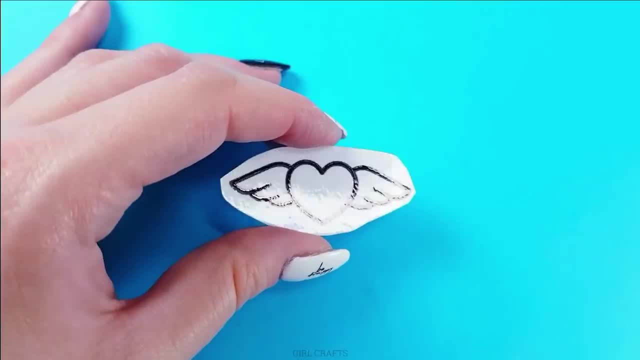 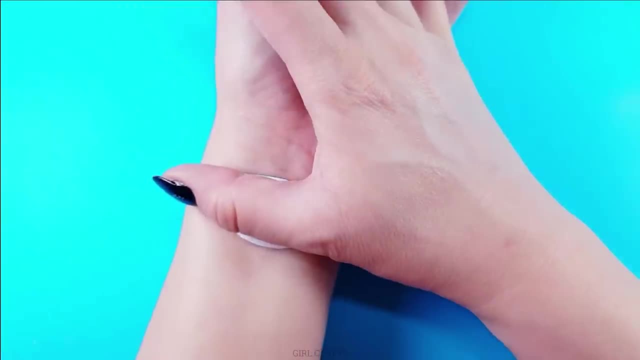 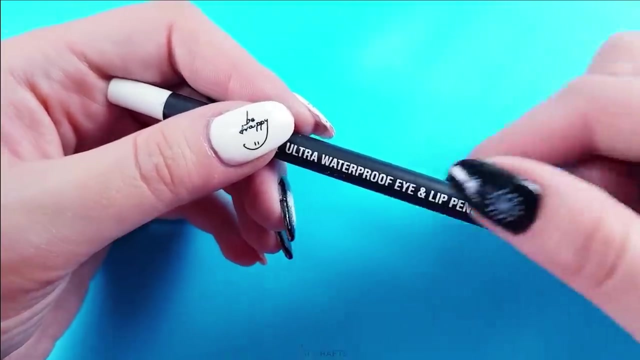 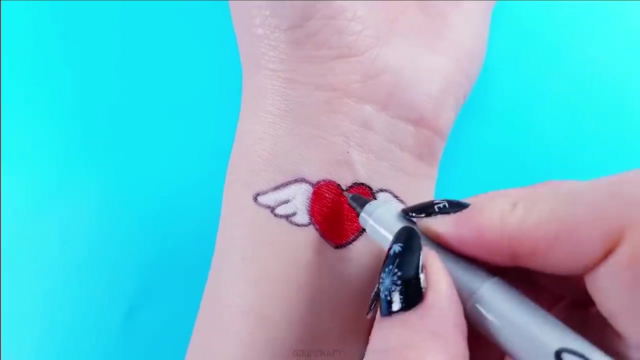 We'll steal back your heart. We'll steal back your heart. You take my breath away. I'm hashtag: blessed, You're the beat. beat to my jade The way you move, move, The way you shake, shake, So hard, so hard, So cool. can't help but say: 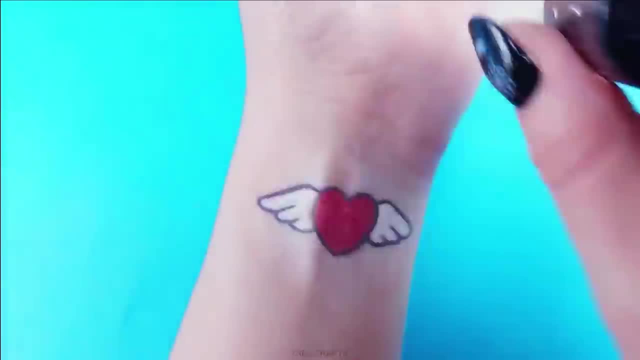 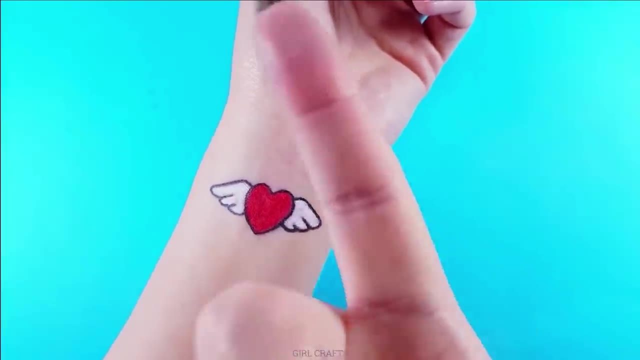 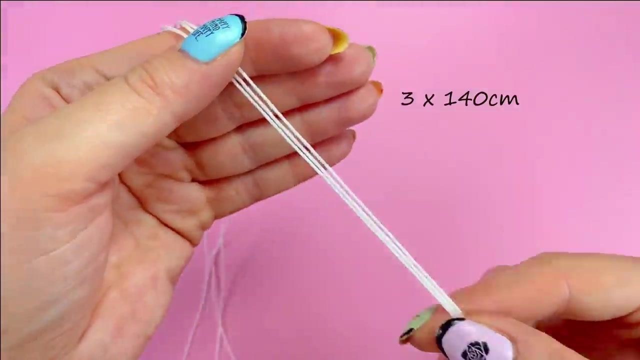 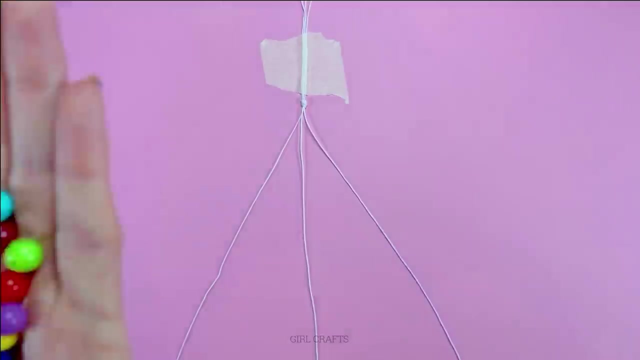 I freaking love you, love you. Something about you, about you, Cause all of it feels it's magic for real. I freaking love you, love you. I freaking love you, love you. Your kisses are electric. Your touch is dynamite. You must be tired. 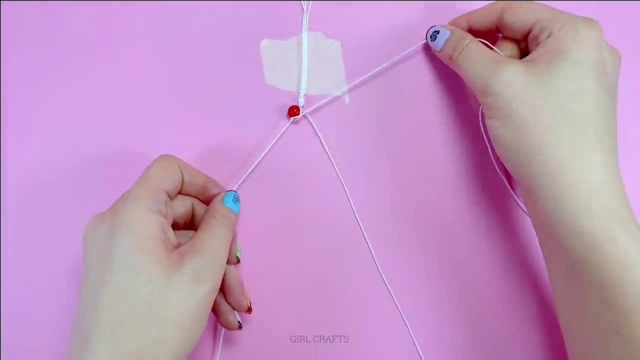 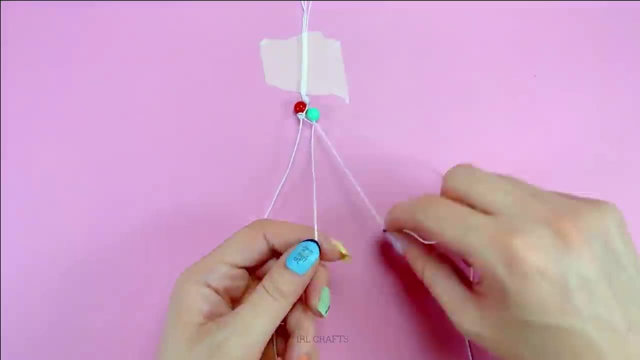 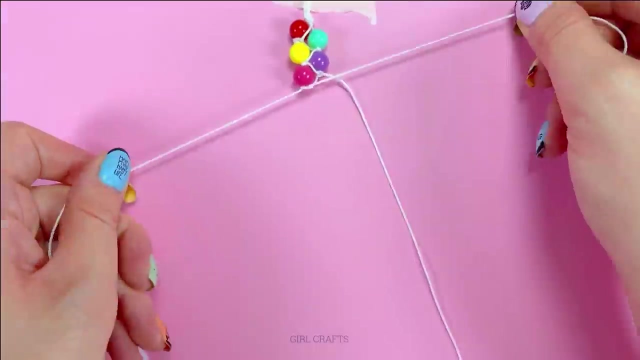 If I'm always gonna do my mind The way you move, move, The way you shake, shake, So hot and so cool, Can't help but say I freaking love you, love you, Something about you, about you, Cause all of it feels it's magic for real. 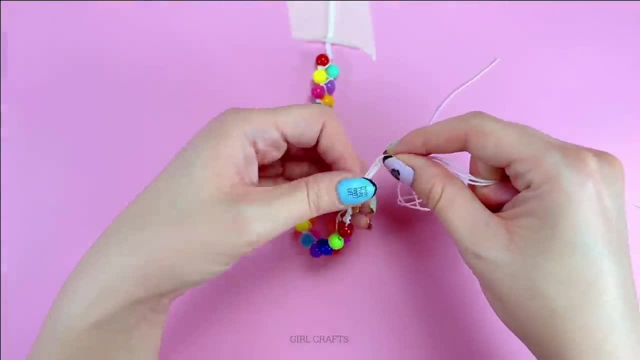 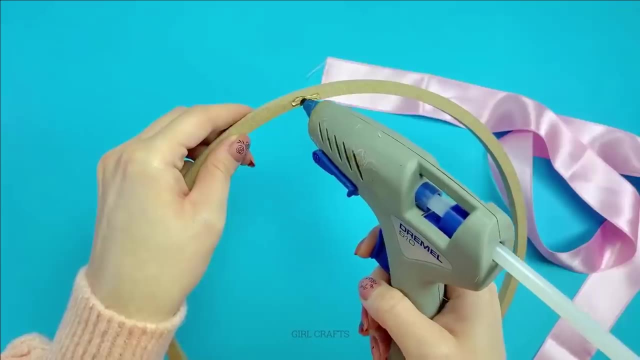 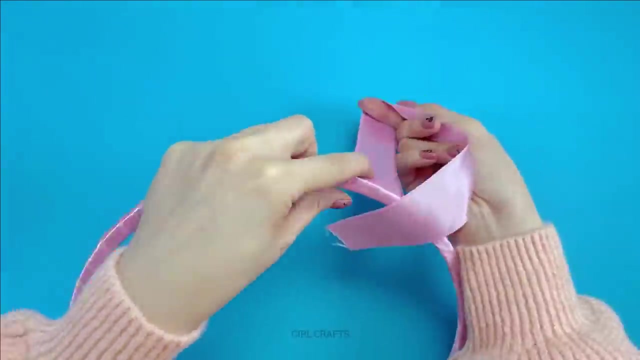 I freaking love you, love you. I freaking love you, love you. The way you move, move The way you shake, shake So hot, so cool, Too much to taste. The way you move, The way you shake, shake So hot, so cool, Can't help but say: 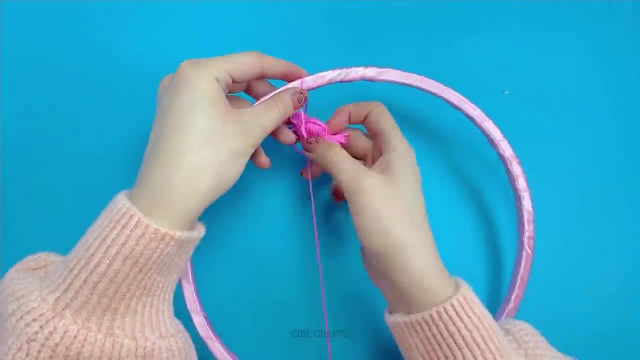 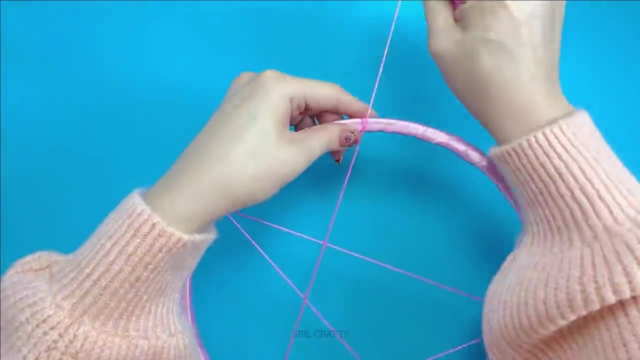 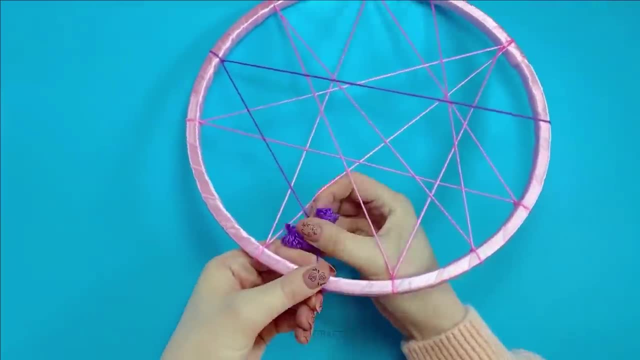 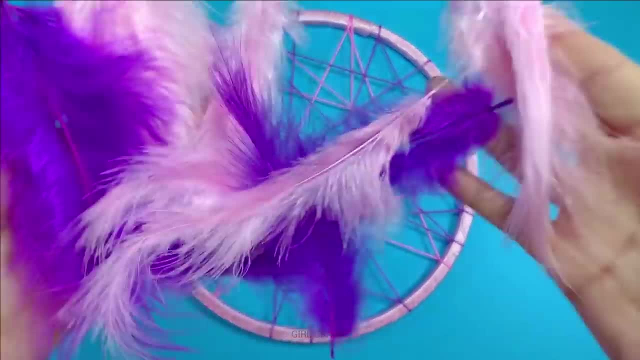 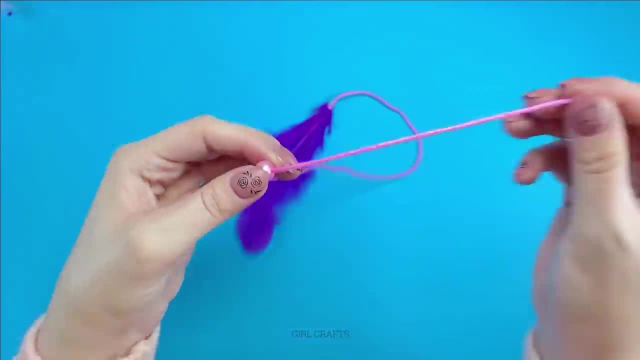 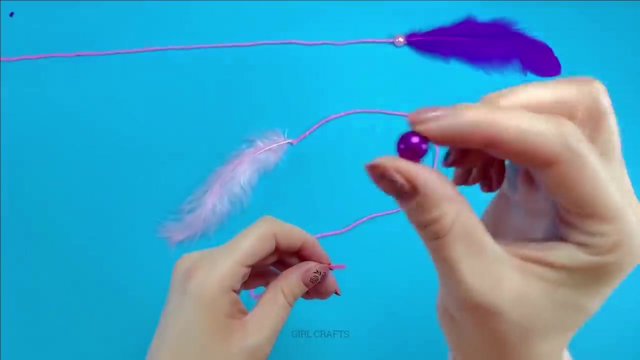 Cause all of it feels it's magic for real. I freaking love you, love you. I freaking love you, love you, I freaking love you, love you, Something about you, about you, Cause all of it feels it's magic for real. I freaking love you, love you. 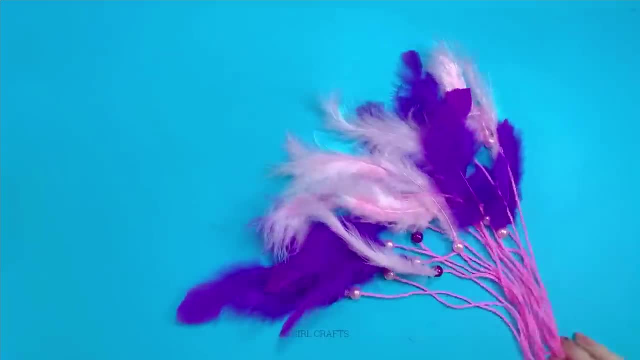 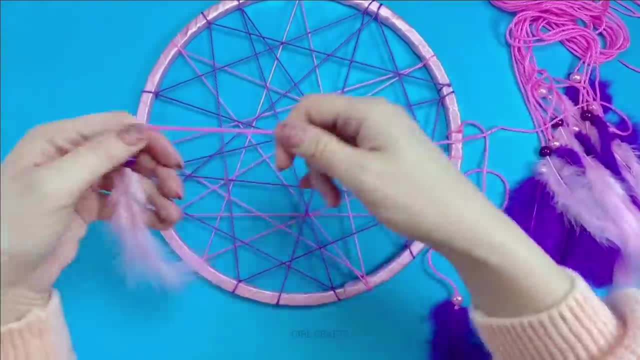 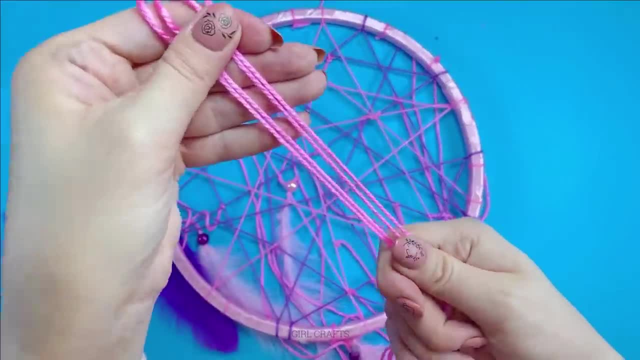 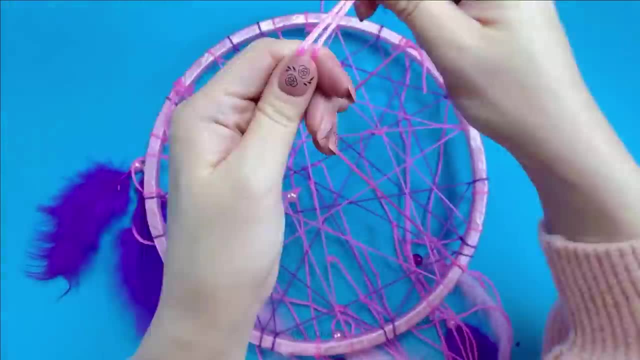 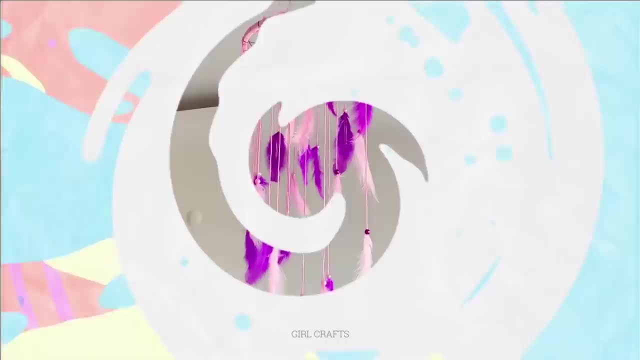 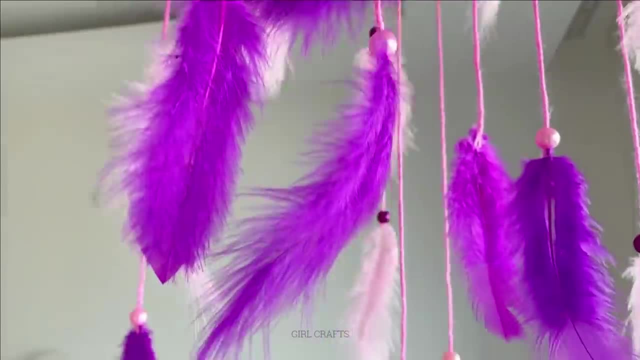 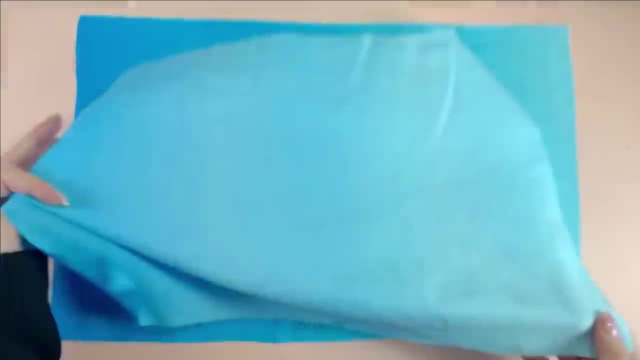 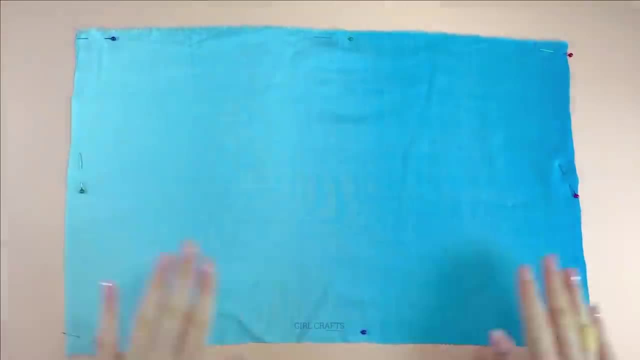 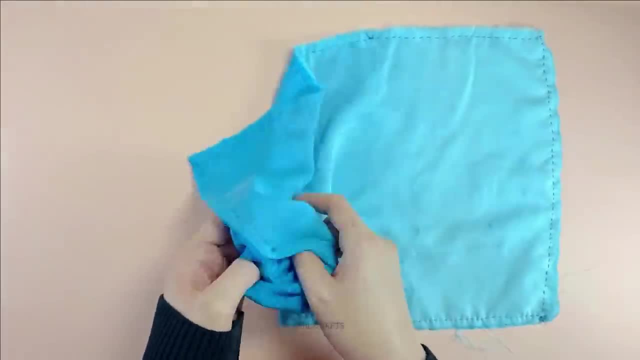 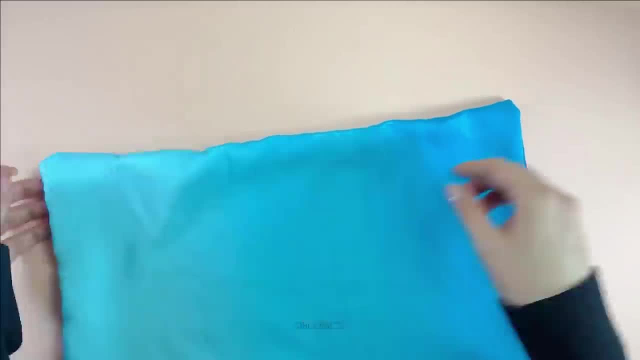 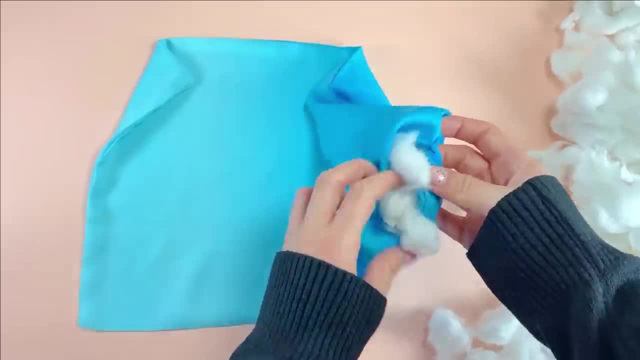 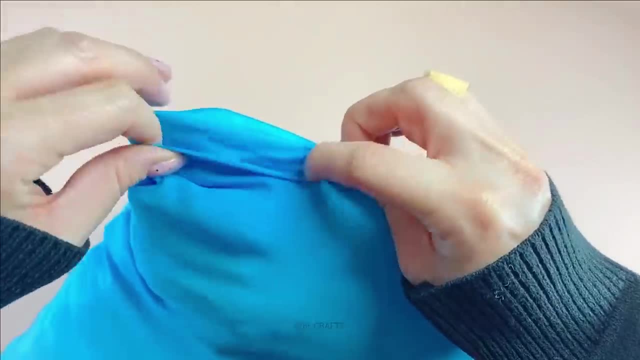 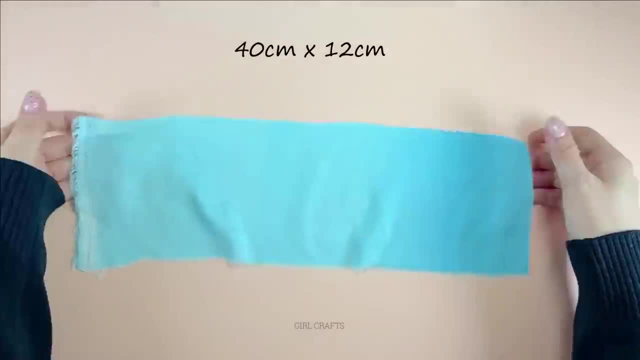 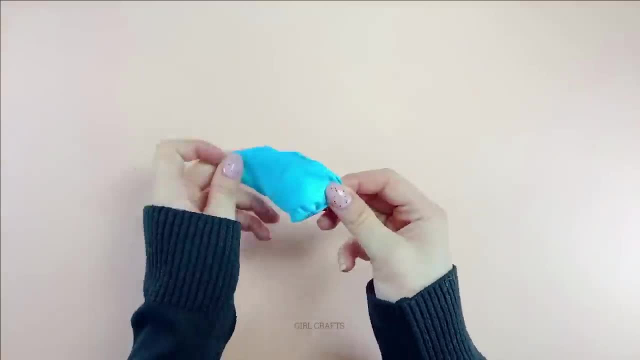 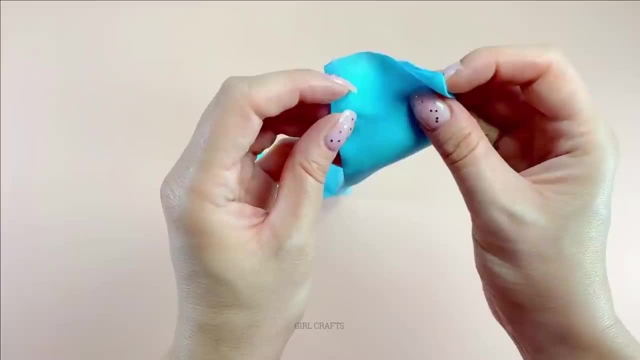 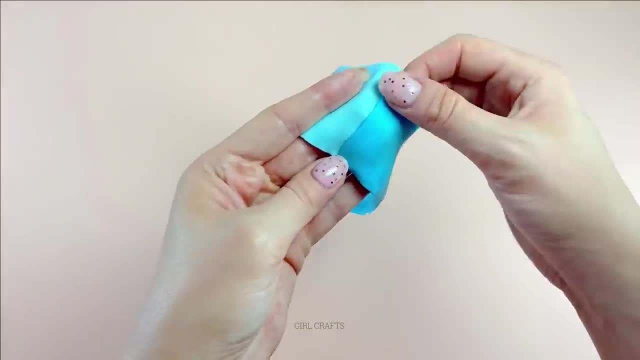 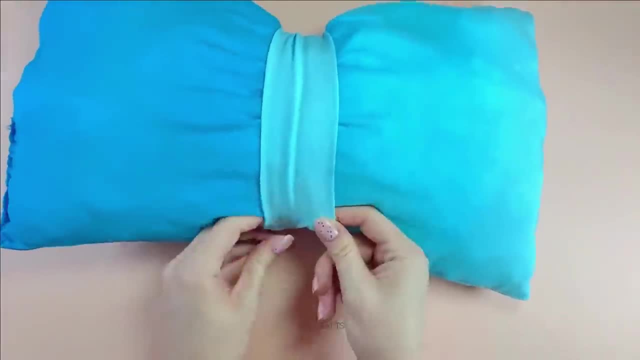 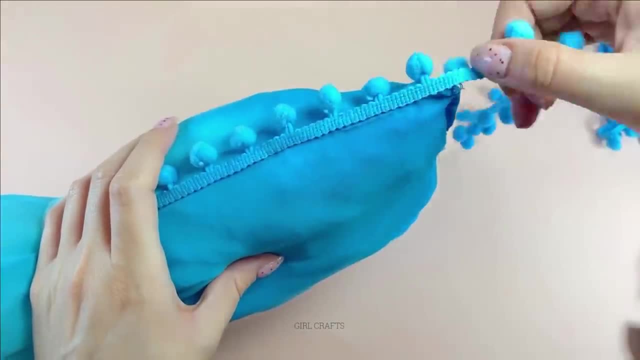 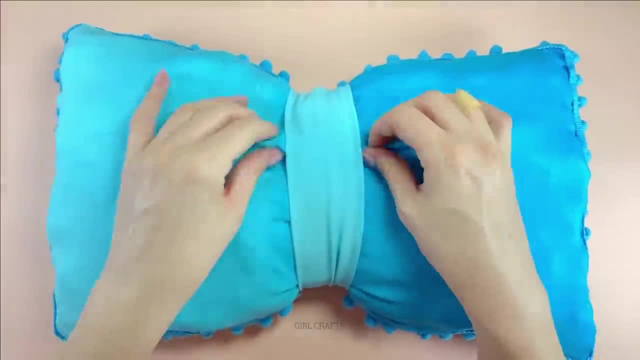 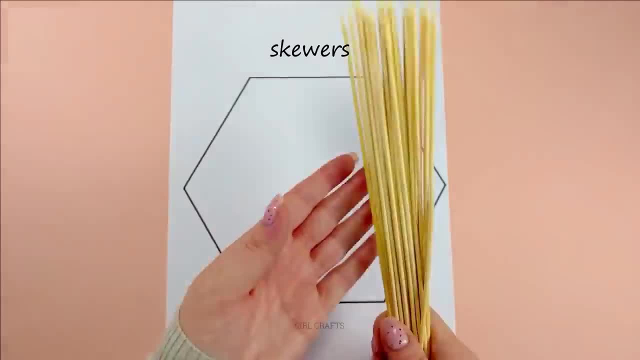 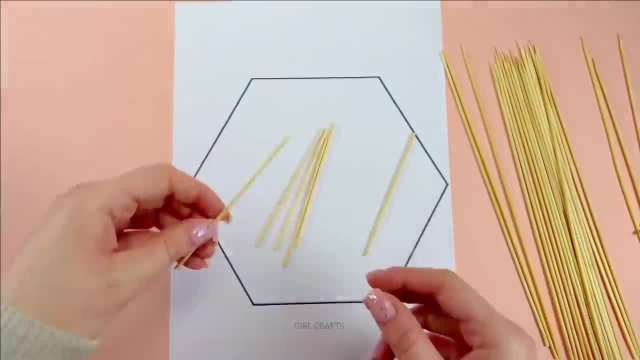 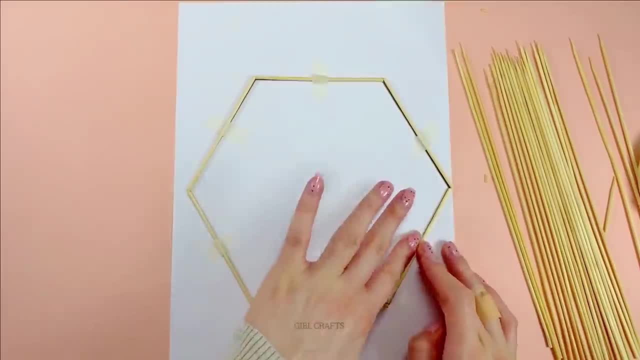 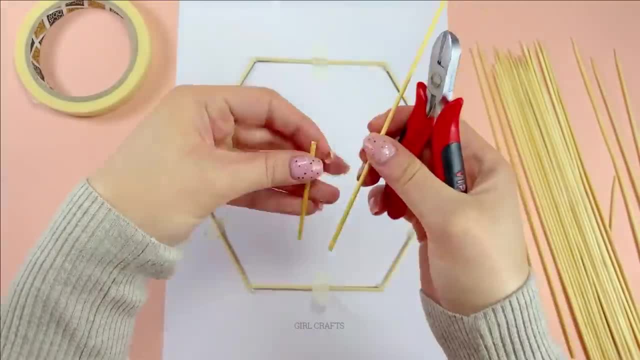 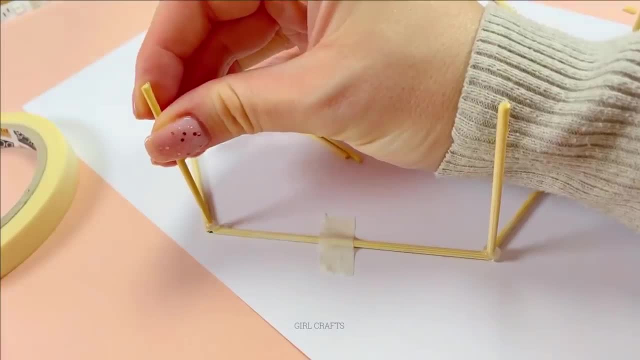 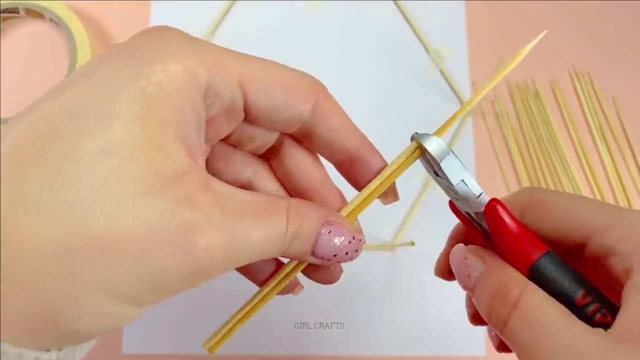 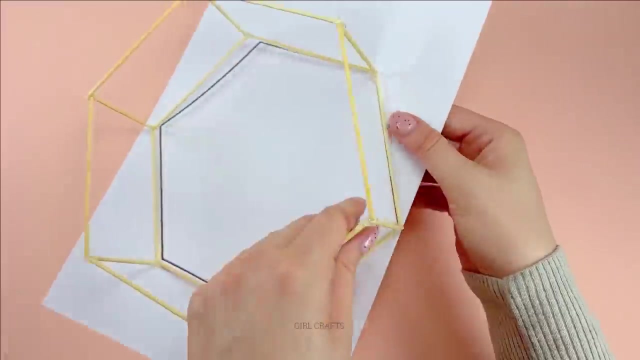 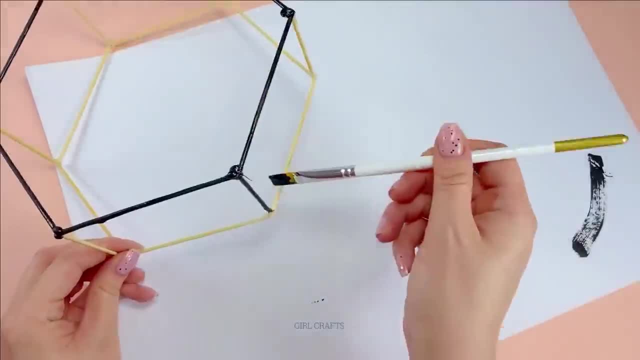 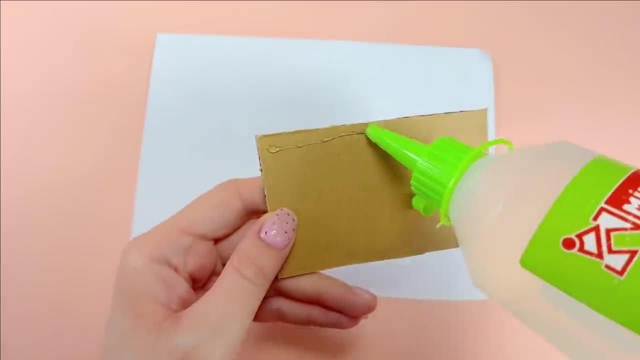 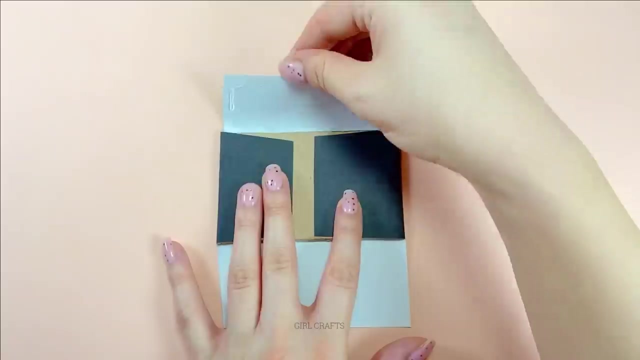 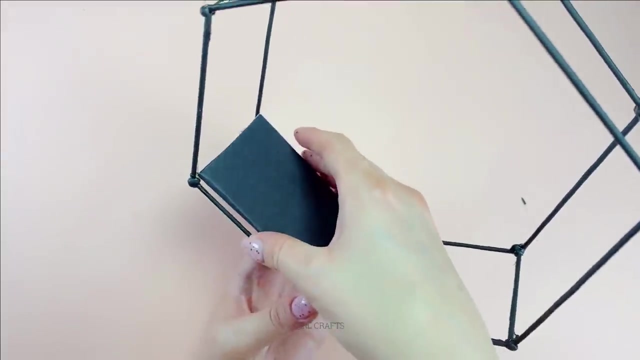 You, I'll never fully know How deep your heart can go, Or the beauty of your soul. Oh you, where were you all along? Every other one was wrong And I found where I belong. Oh, the day I met you, I think I met myself. 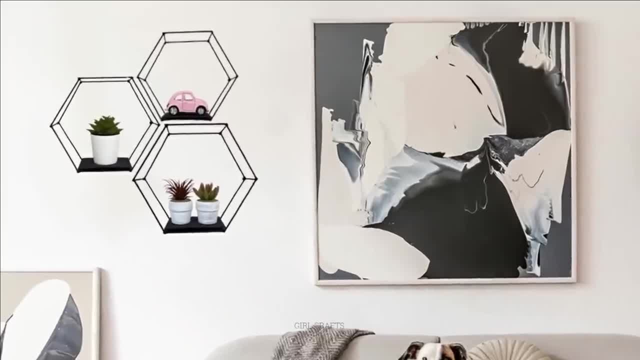 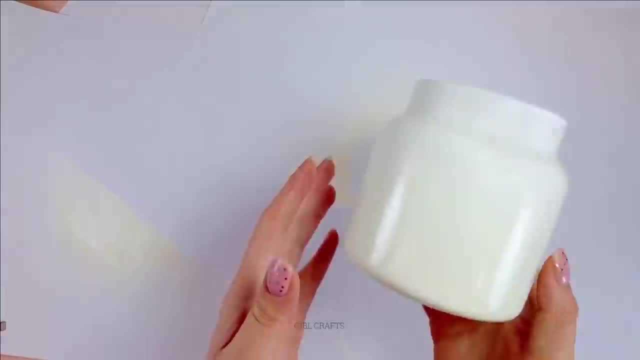 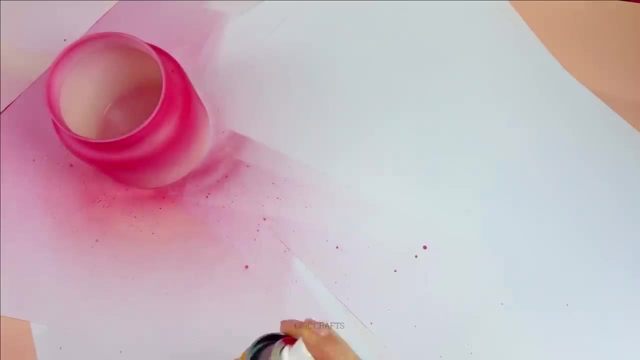 I don't ever wanna be with anyone else. We got the kind of story that the stories would tell Different than I've ever felt, And I Know we've got our whole lives. No indignis inside. darling, all I wanna do Is be with you And I. 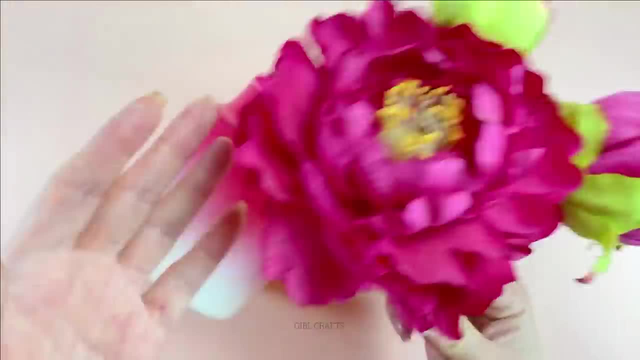 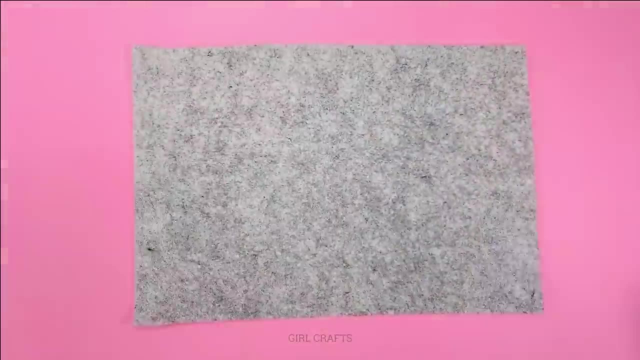 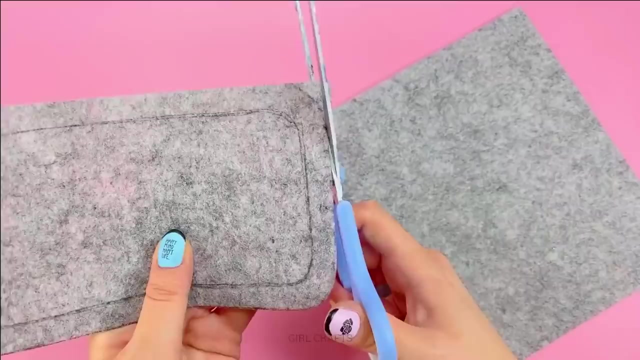 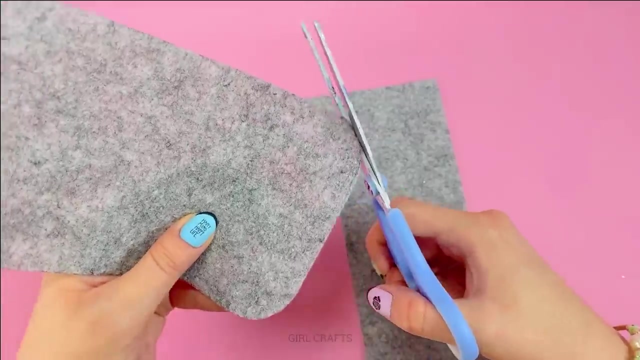 Know we've got our whole lives, No indignis inside. darling, all I wanna do Is be with you tonight. Yeah, yeah, be with you tonight. Yeah, Yeah, yeah, be with you tonight. We're not in a rush, we're not gonna leave, But I can't get enough of what you do to me. 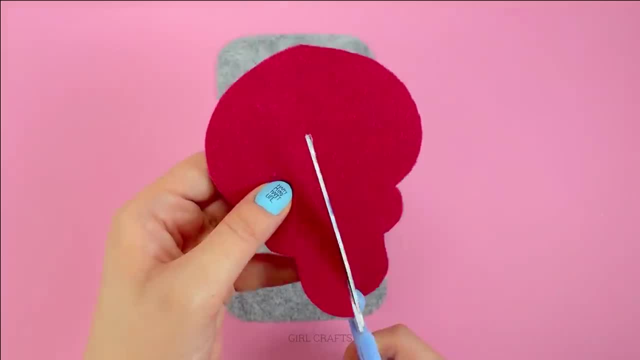 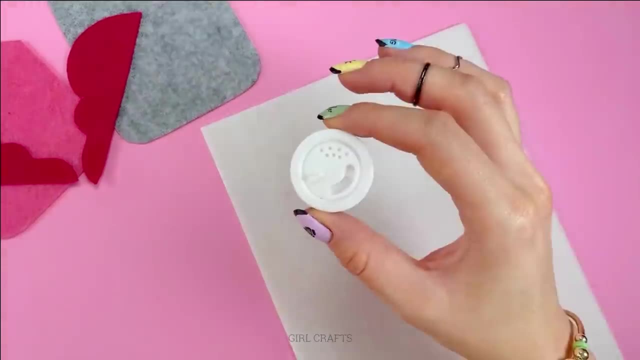 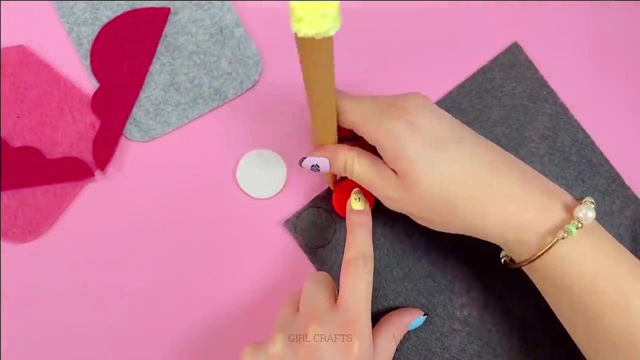 We're not in a rush, we're not gonna leave, But I can't get enough of what you do to me And I Know we've got our whole lives. No indignis inside, darling, all I wanna do Is be with you And I, No, we've got our whole lives. 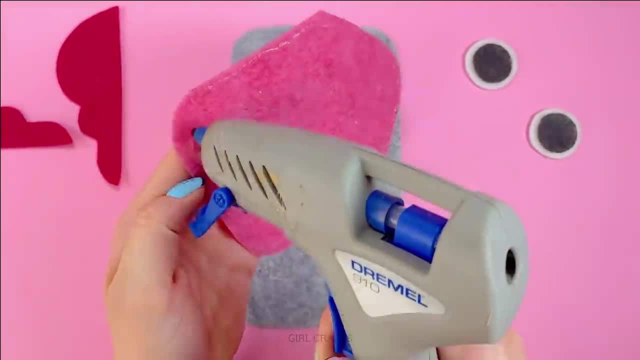 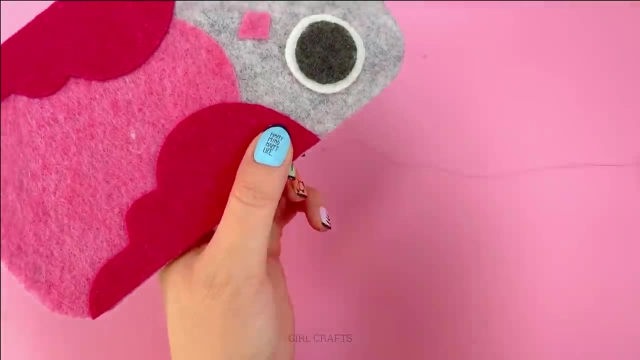 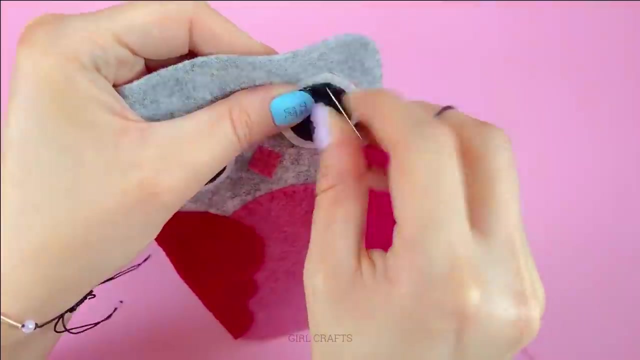 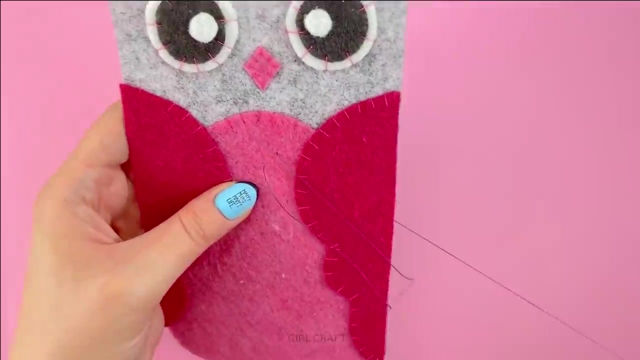 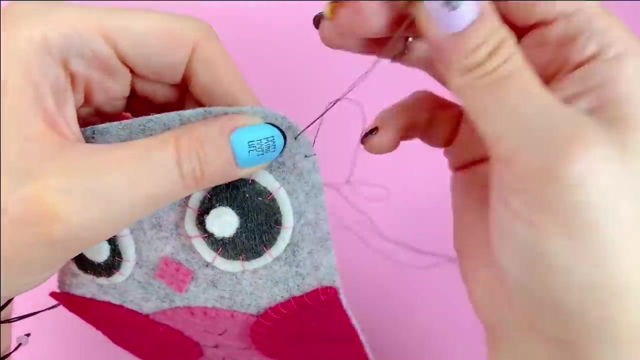 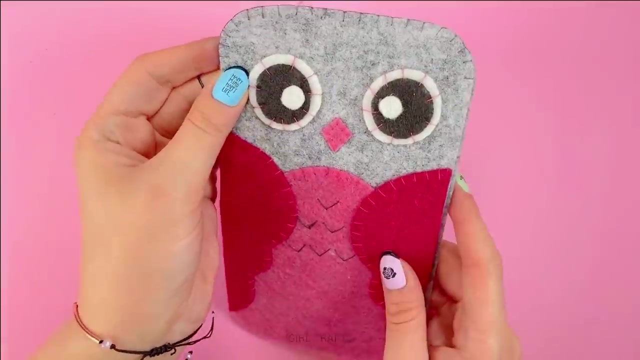 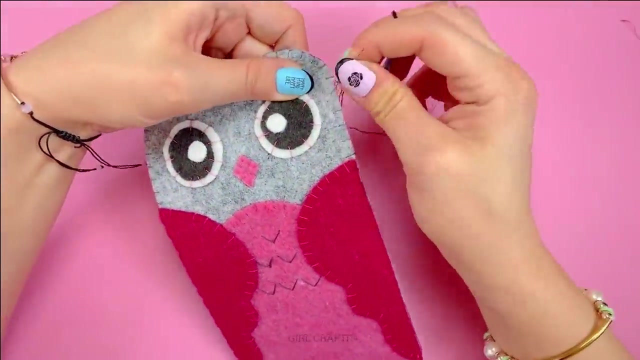 No ending this inside, Darling. all I wanna do Is be with you tonight. Yeah, yeah, Be with you tonight. Hey, hey, Be with you tonight. Hey, yeah, Be with you tonight. Just be with you tonight. What if we walked into the airport And bought a ticket at the counter? 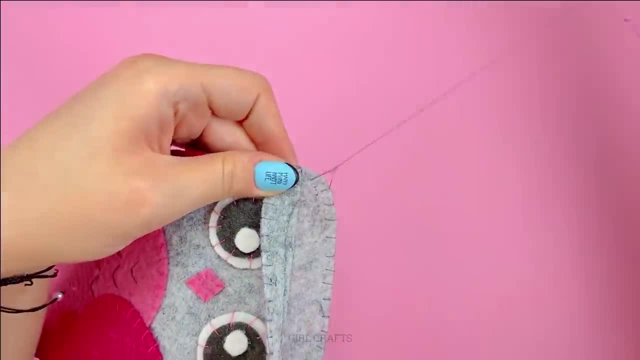 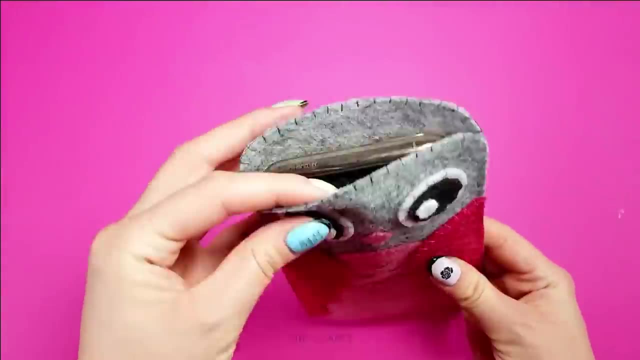 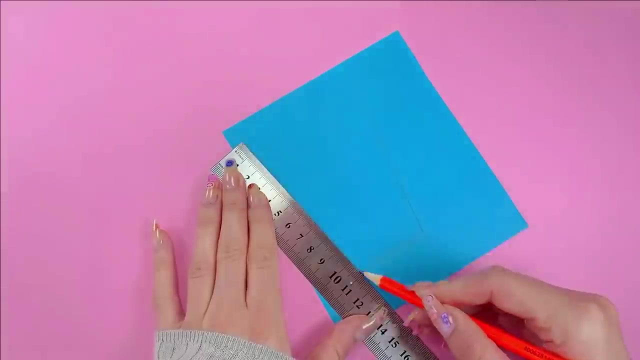 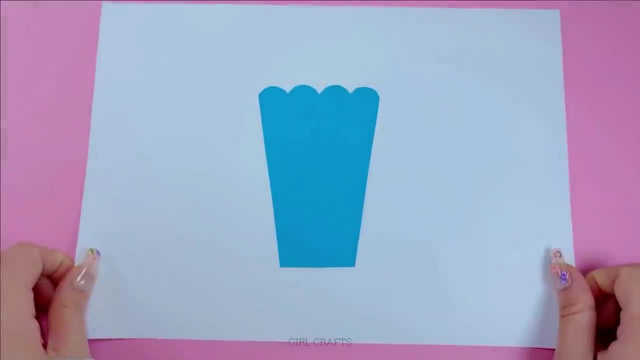 And just flew, Spin the globe and close your eyes. I'll go anywhere Where it lands With you. Let's stop thinking about it. The world will go on without us. We'll disappear somewhere. If it's you and me, I'll be there. Let's drive to Vegas. Your old Mercedes Just wander aimless. Take this freeway Until it ends. I know I'm crazy, But so are you. Let's drive to Vegas, Baby, right now. Let's drive to Vegas. Let's drive to Vegas. You've got that iPod from 06 With all the songs we know. 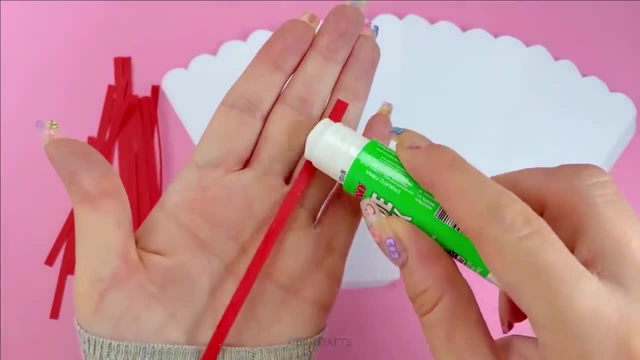 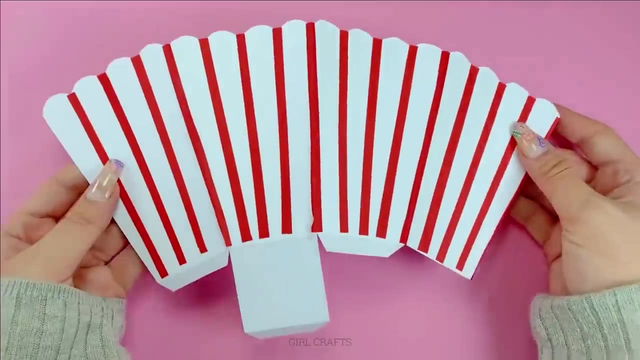 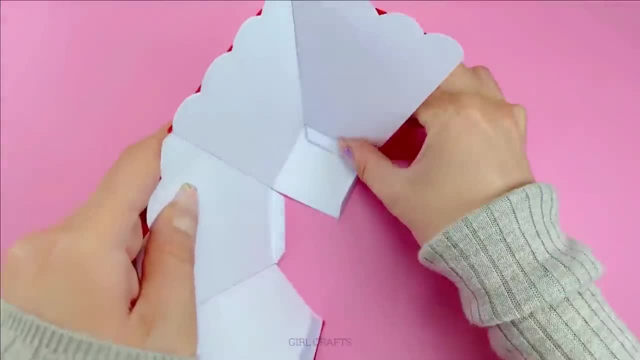 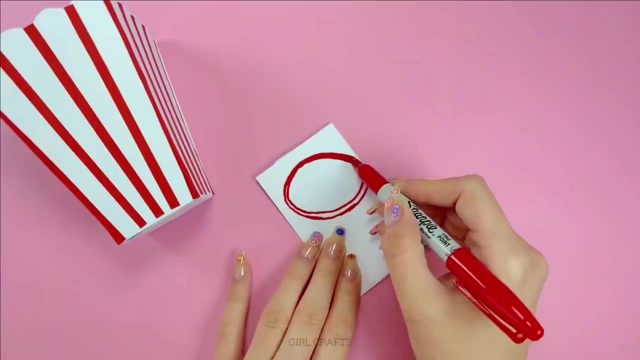 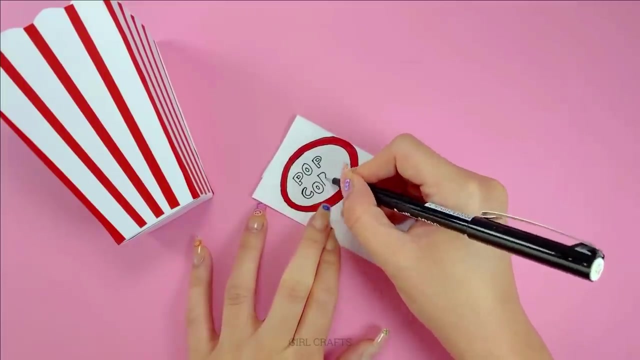 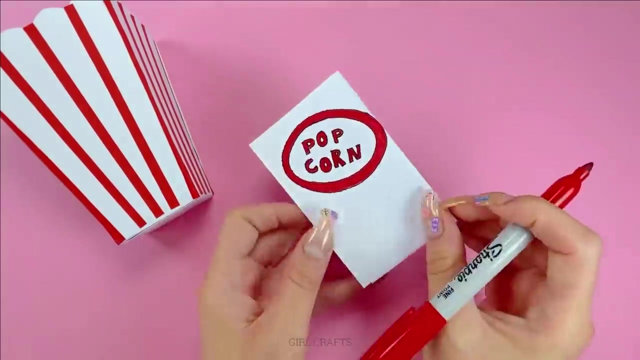 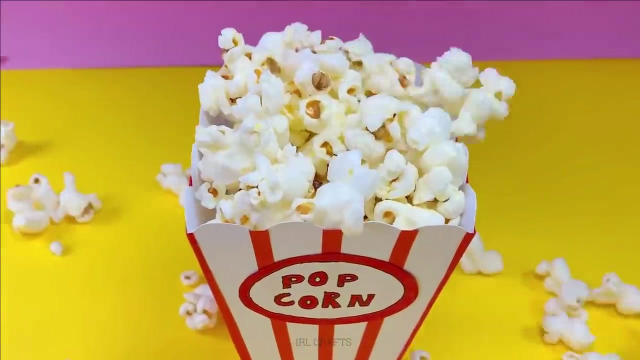 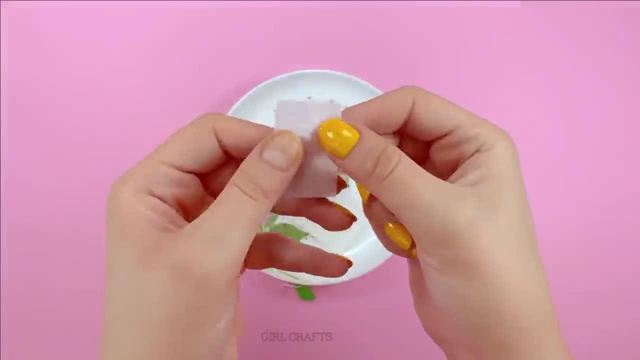 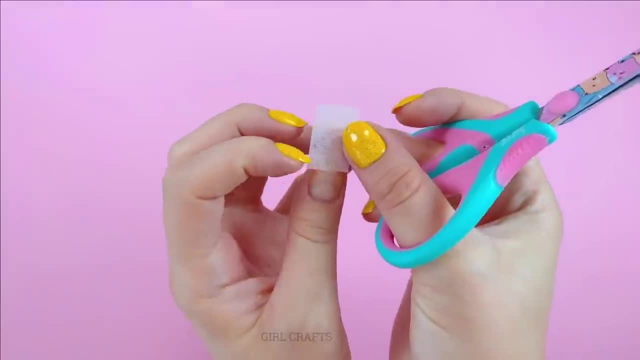 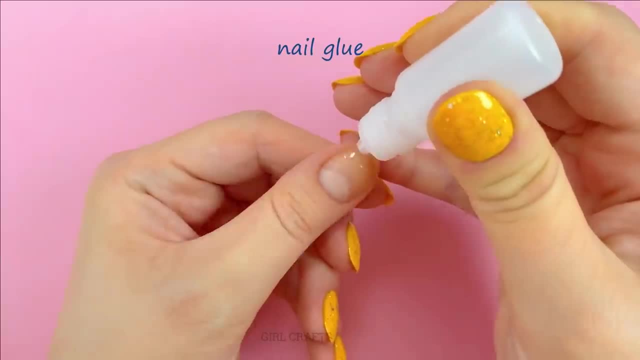 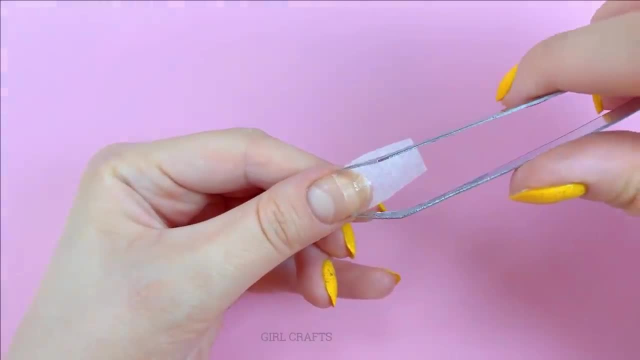 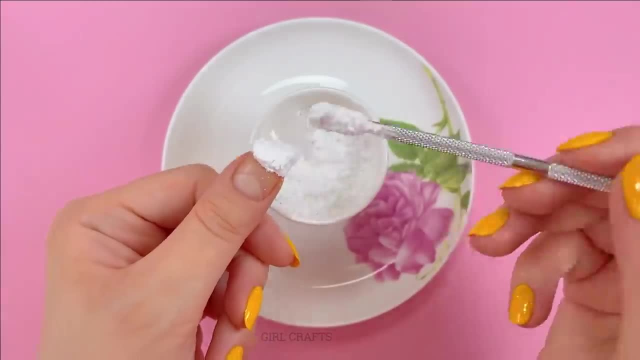 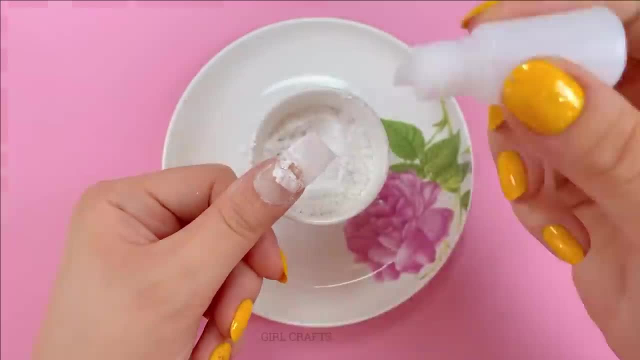 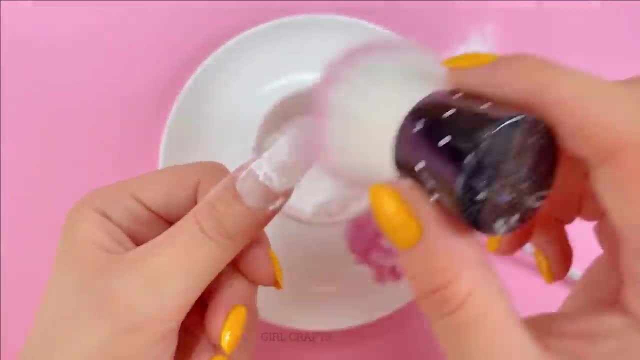 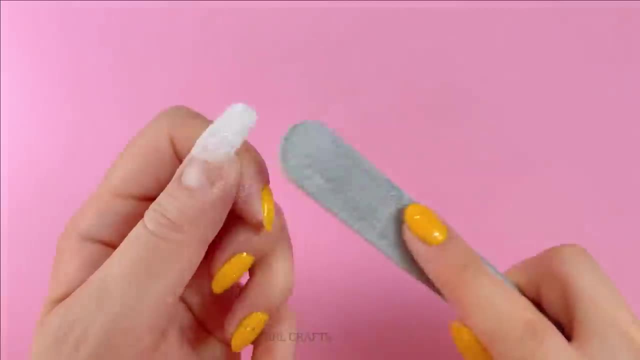 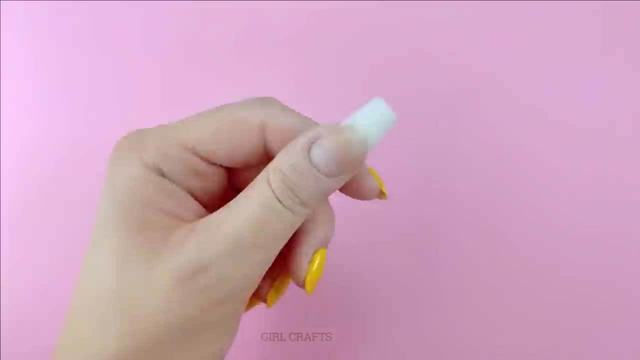 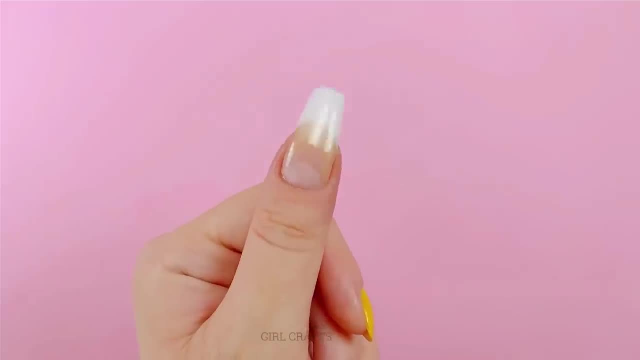 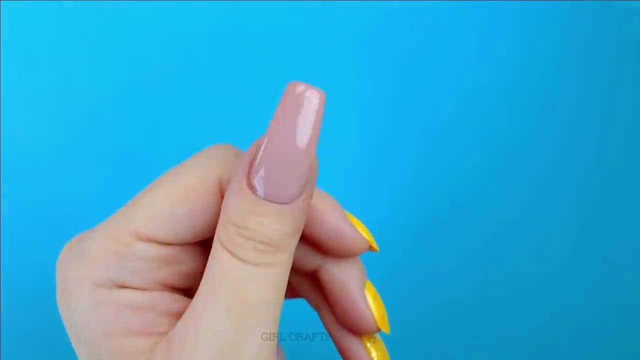 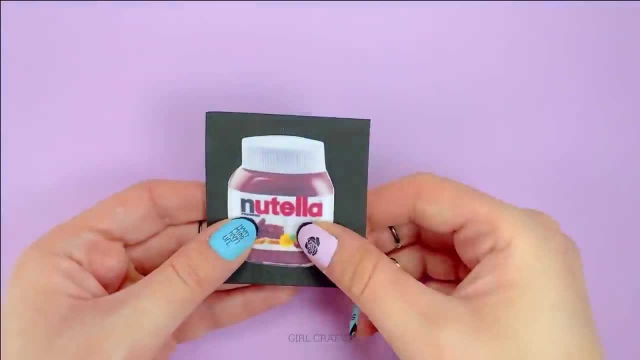 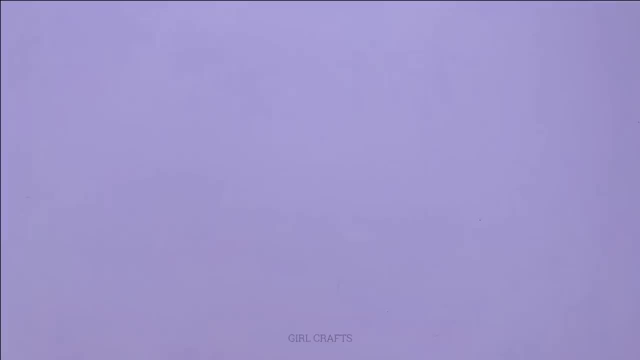 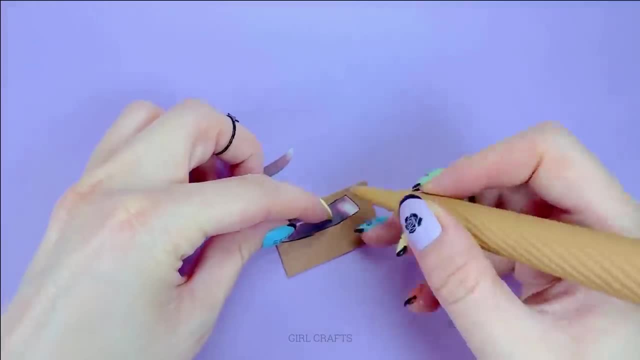 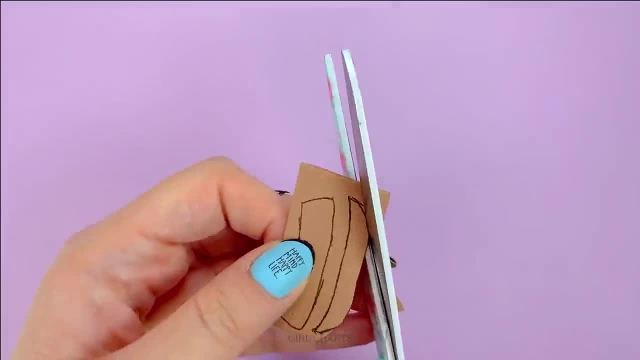 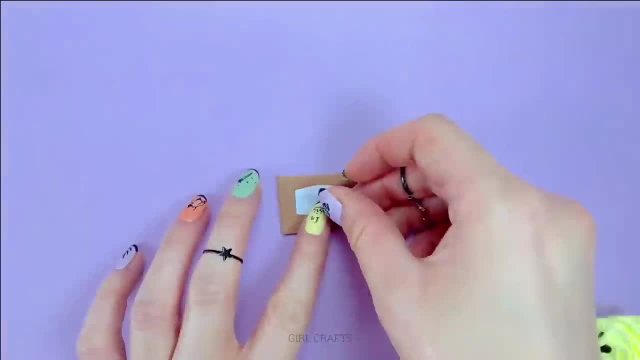 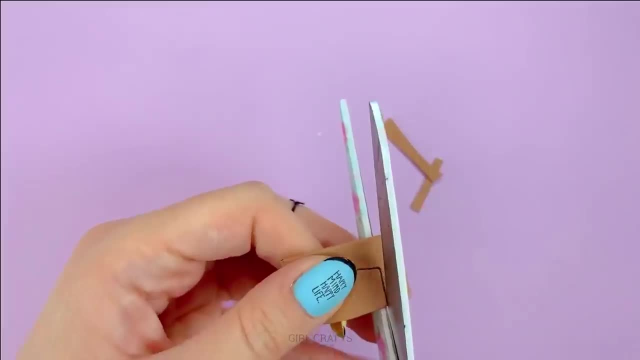 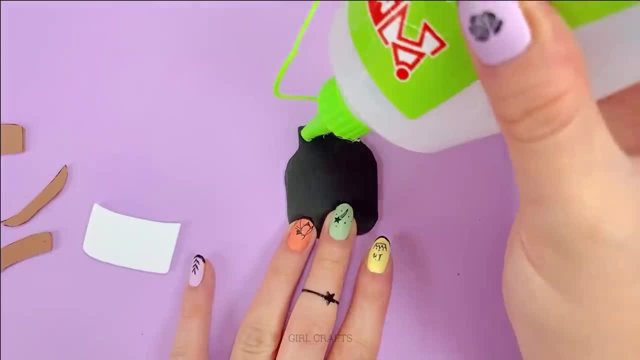 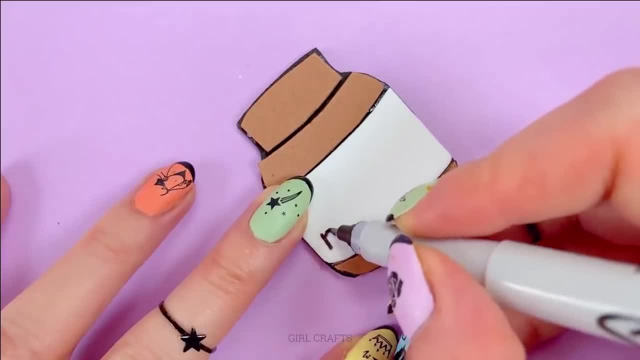 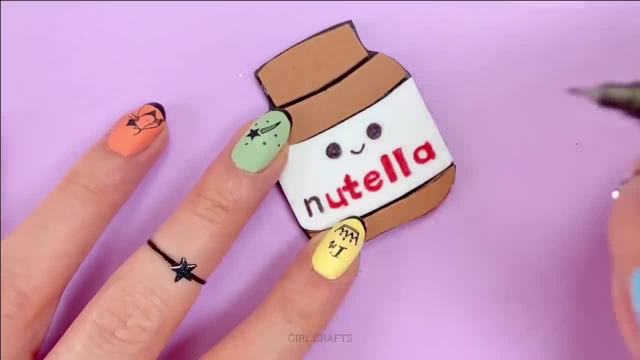 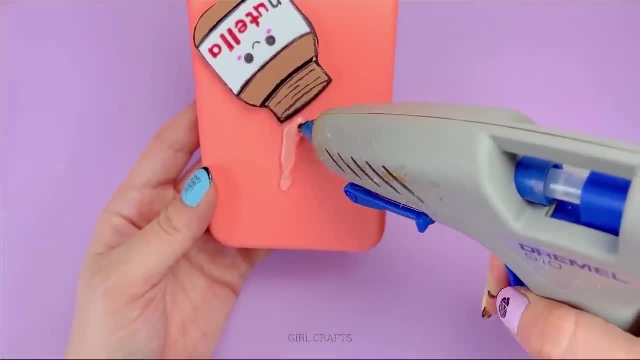 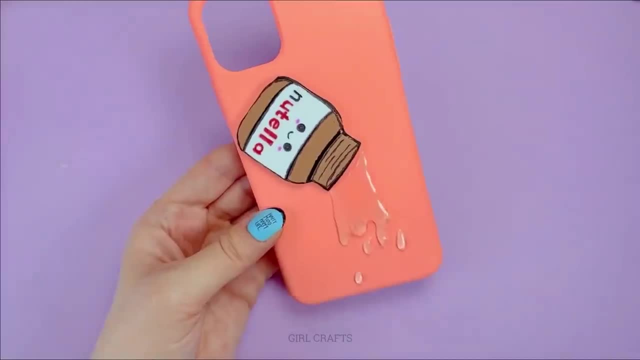 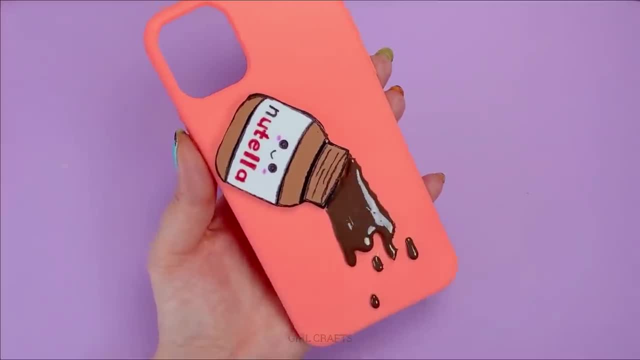 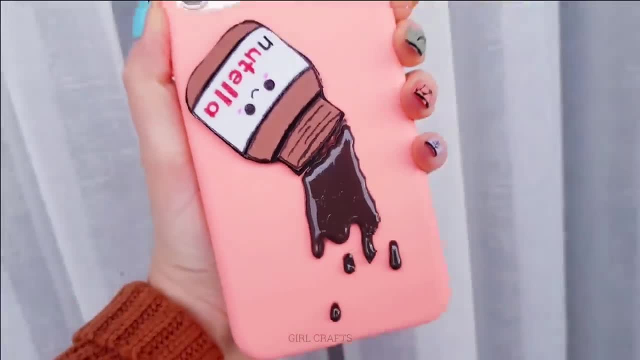 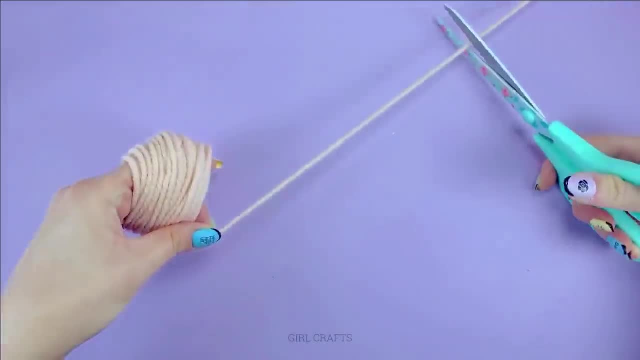 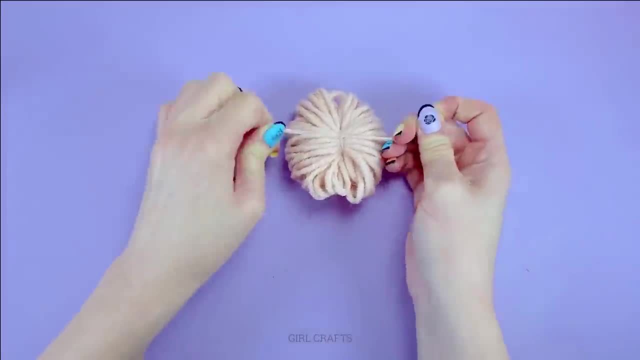 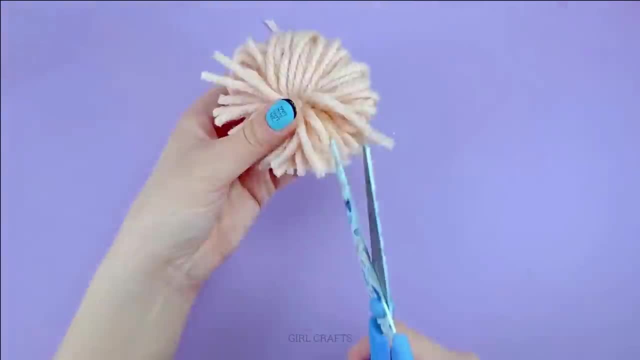 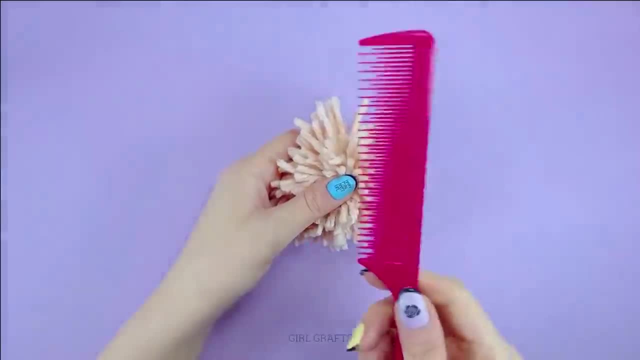 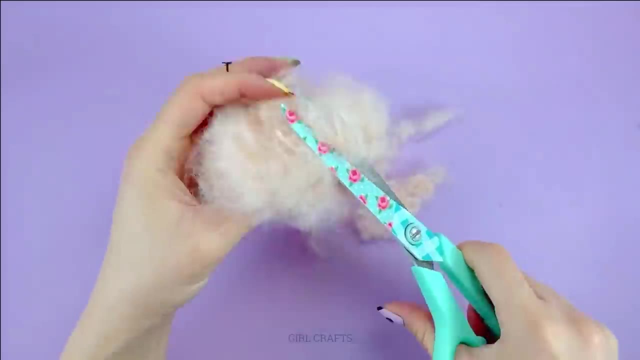 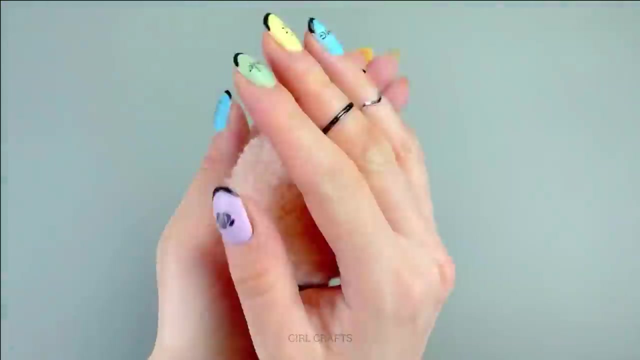 Readin' issues at PEAS For you. you for me, Haven't got to care. Whatever comes, we have all we need. Like a puzzle, every piece Comes together perfectly. What a picture, what a scene. Oh, we were made to go together. 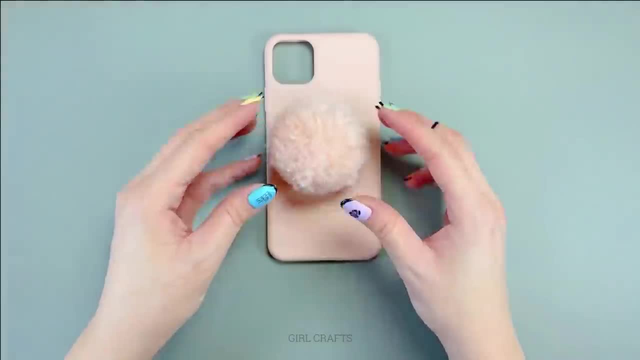 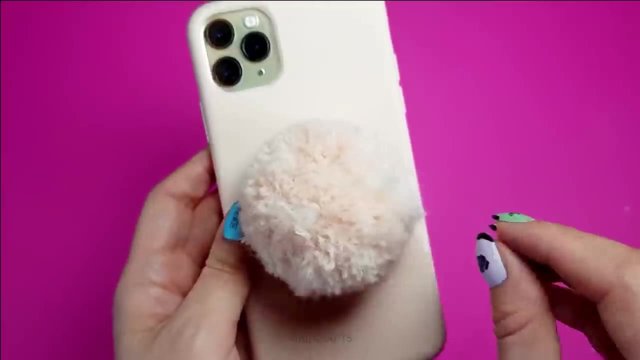 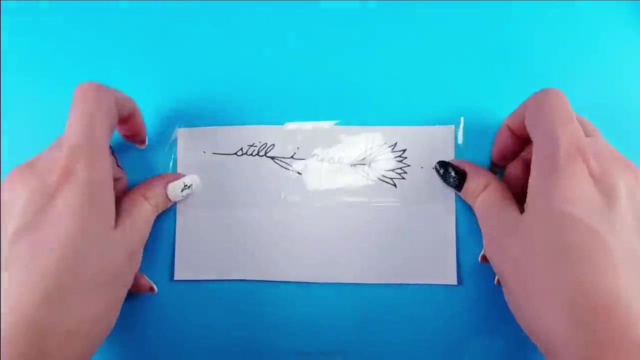 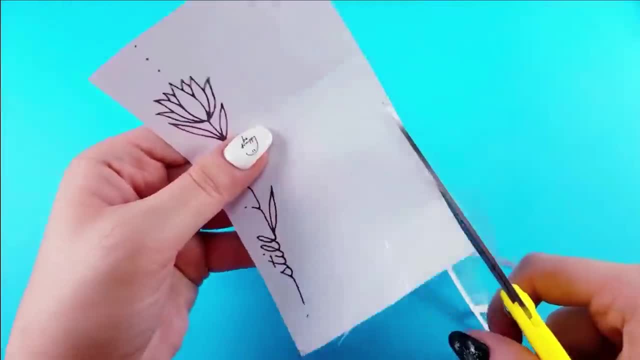 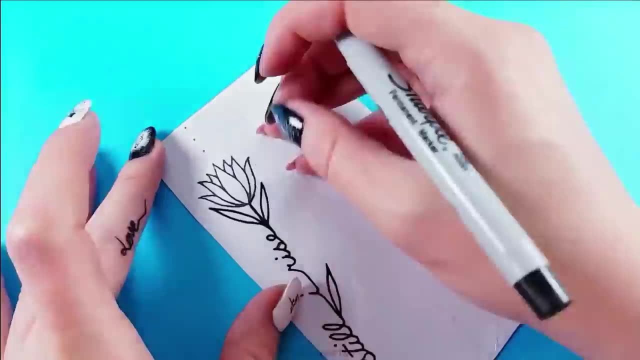 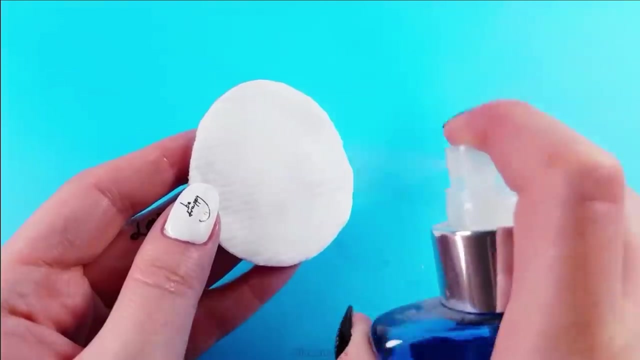 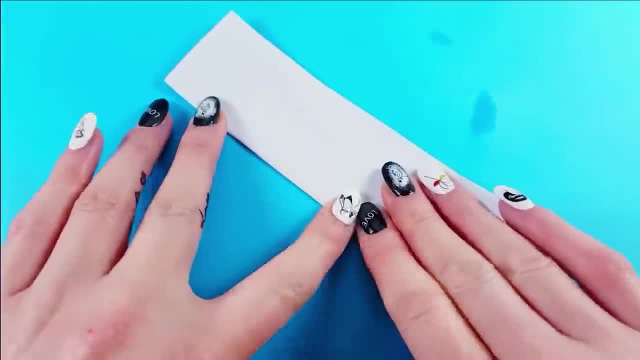 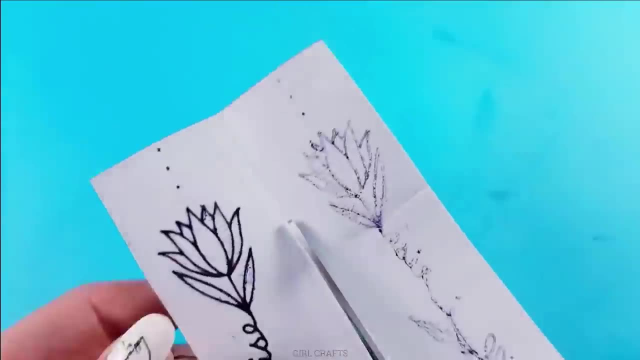 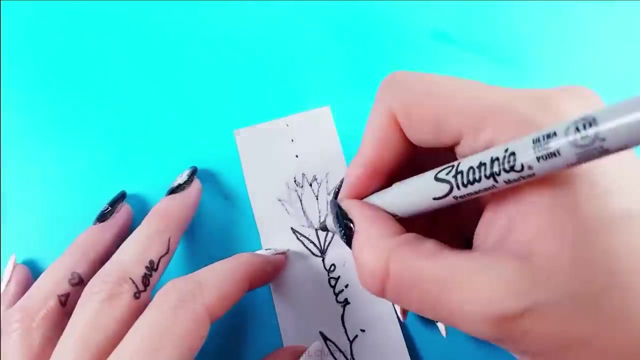 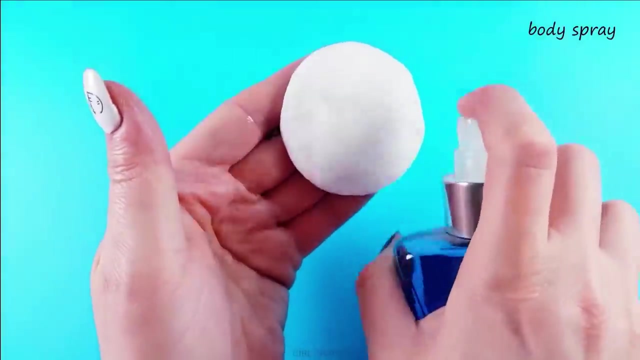 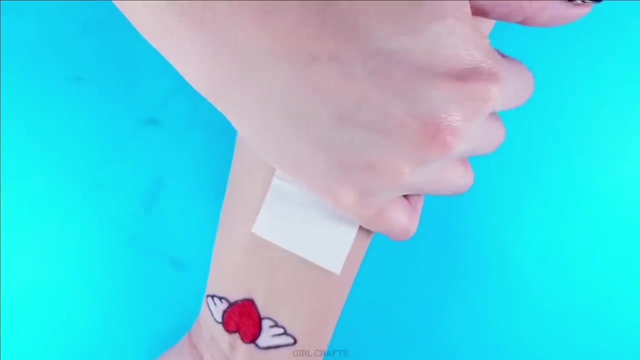 Like a puzzle. every piece Comes together perfectly. What a picture, what a scene. I've got music. I've got fire. I've got magic, Magic love. I've got music. I've got something. I've got color. This is magic, Magic love. I've got a feeling. 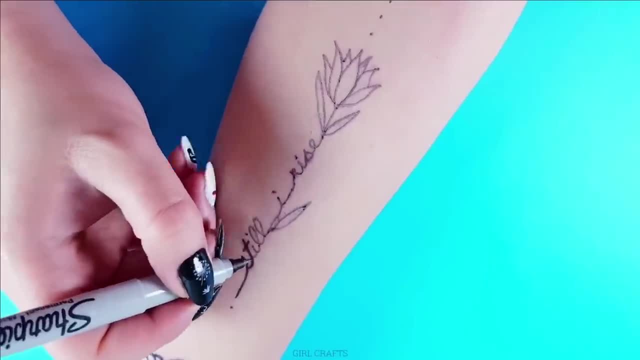 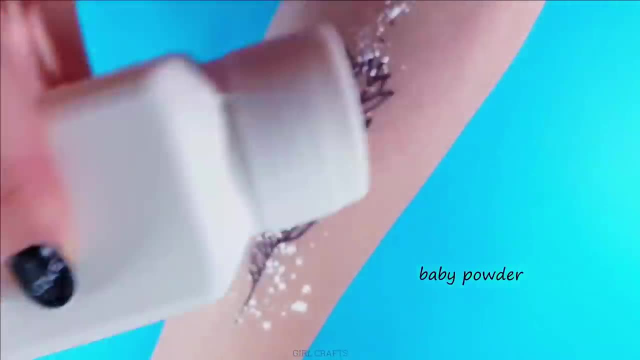 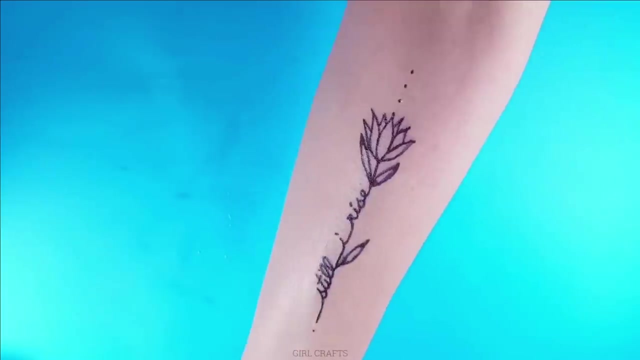 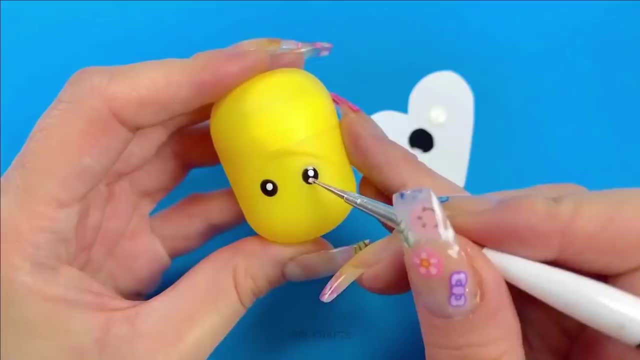 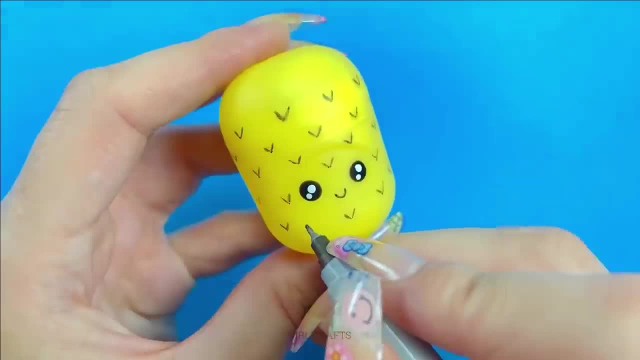 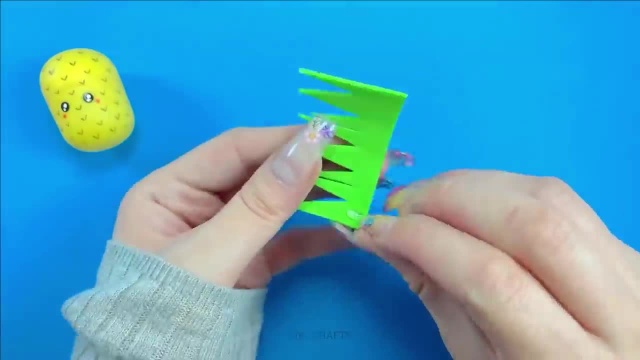 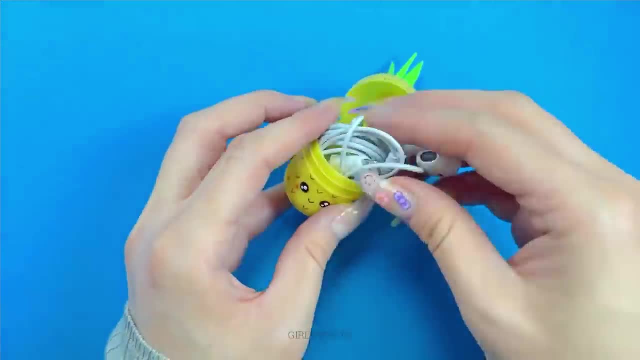 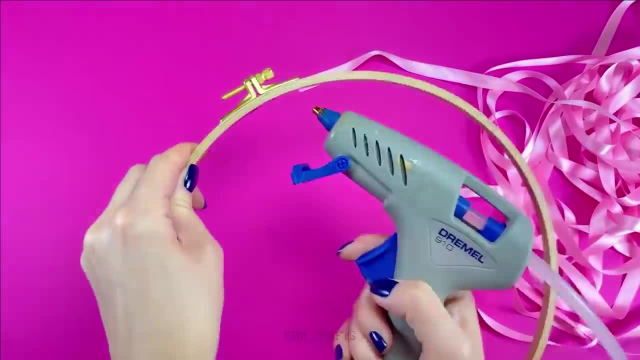 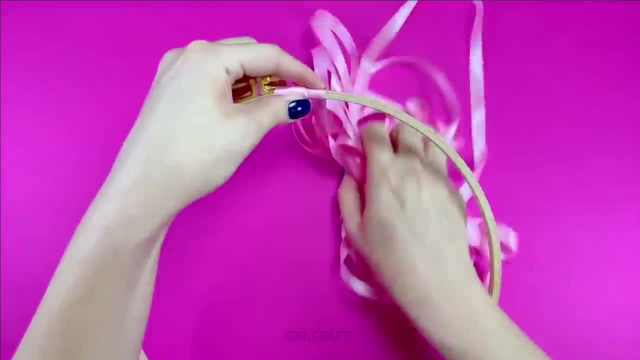 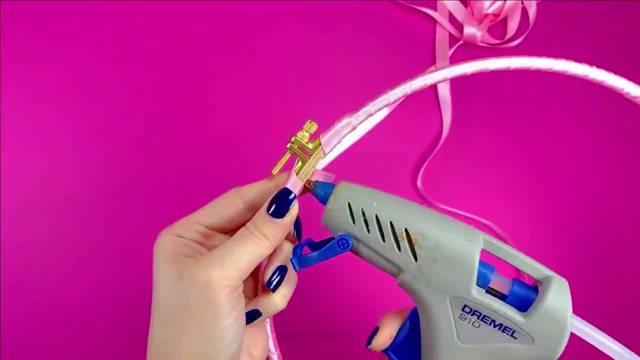 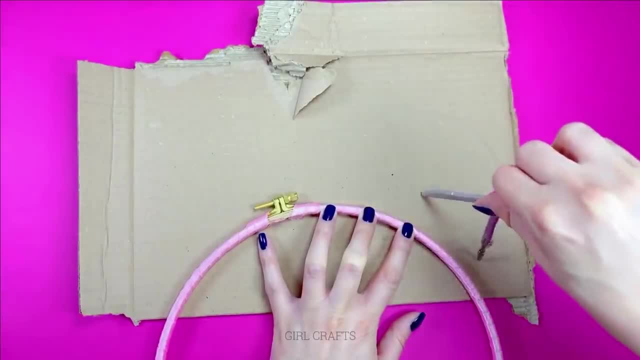 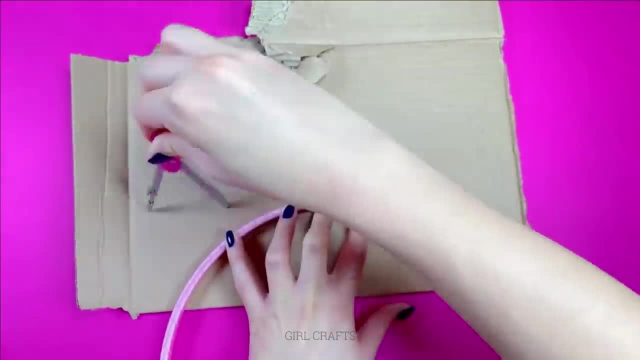 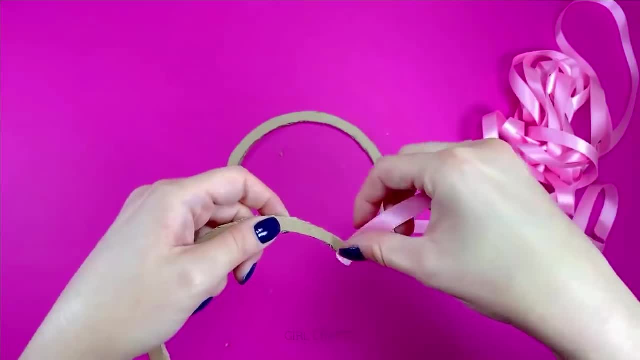 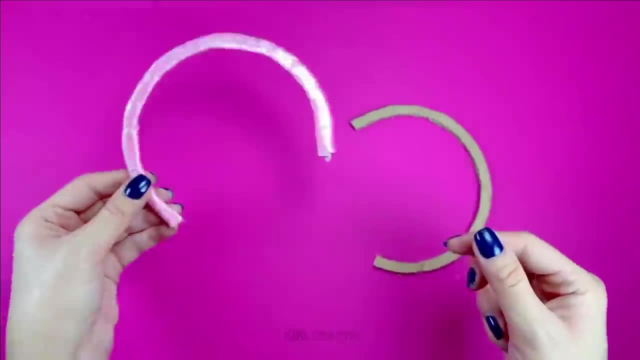 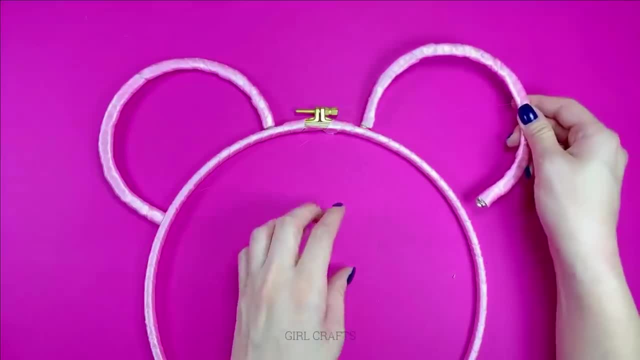 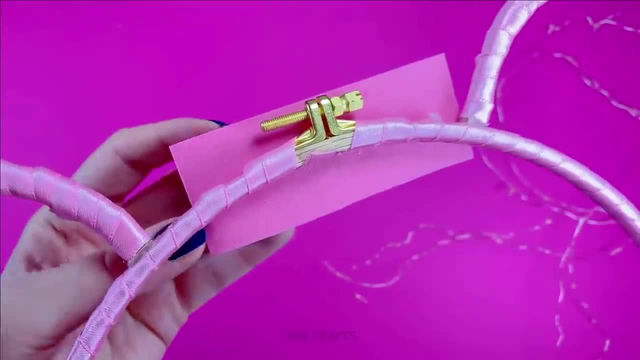 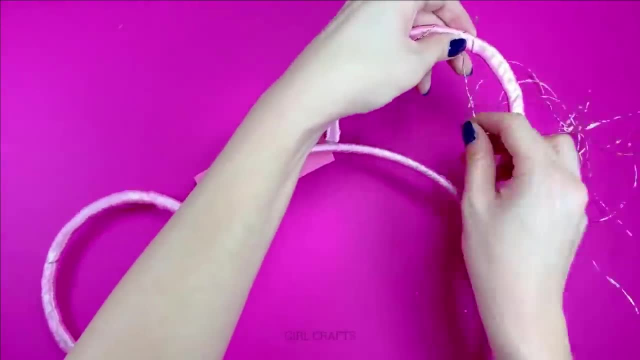 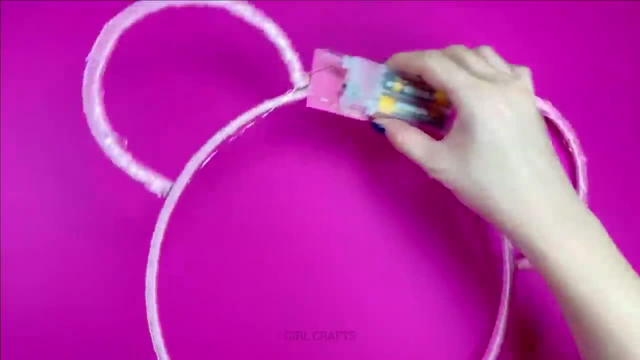 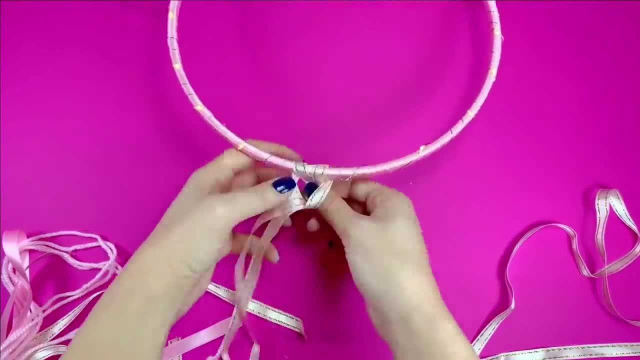 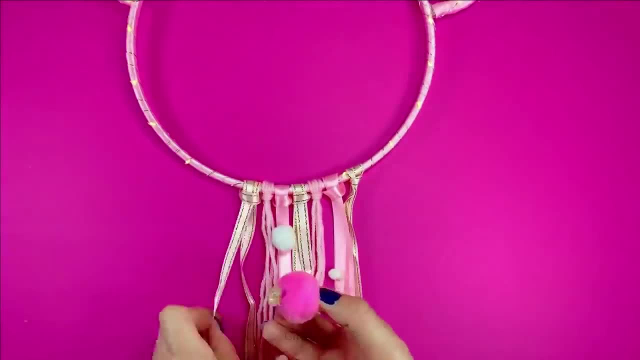 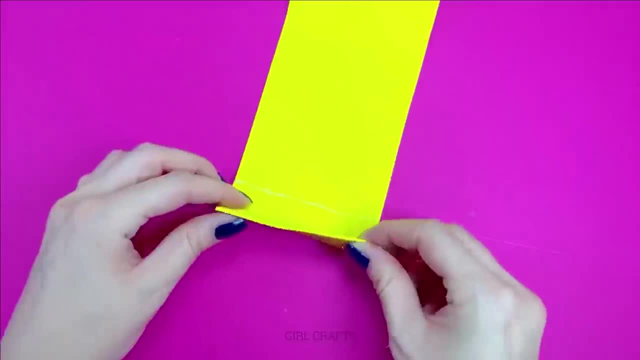 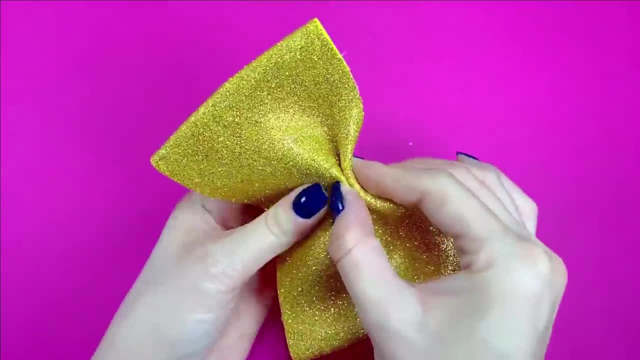 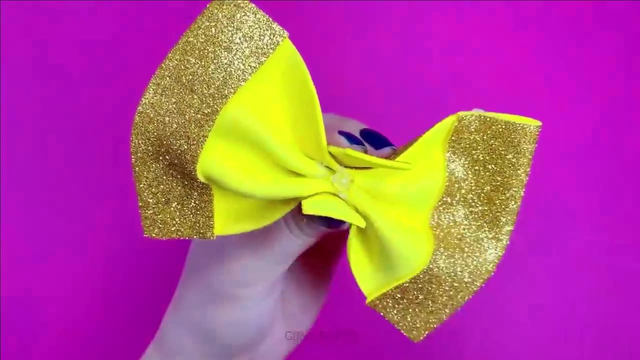 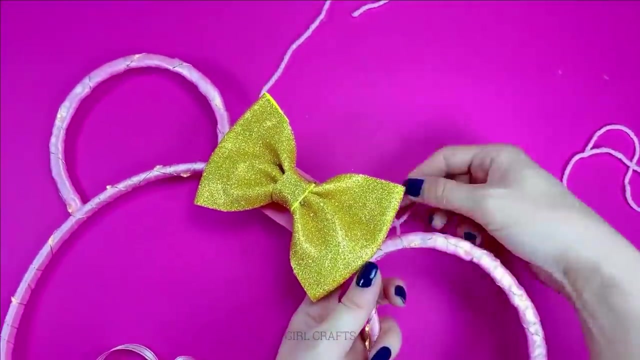 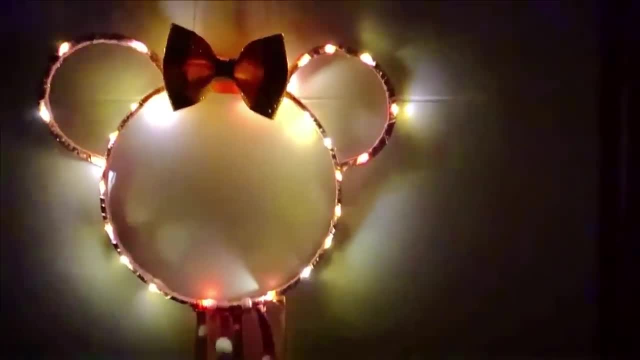 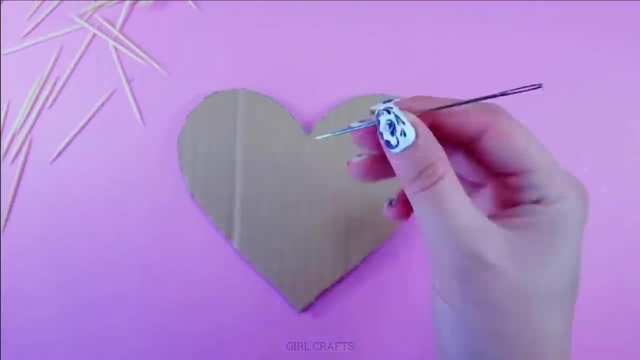 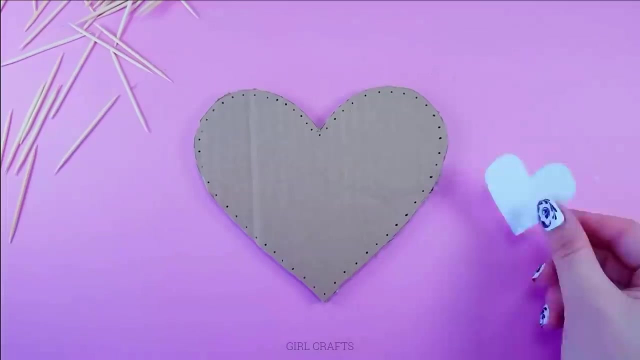 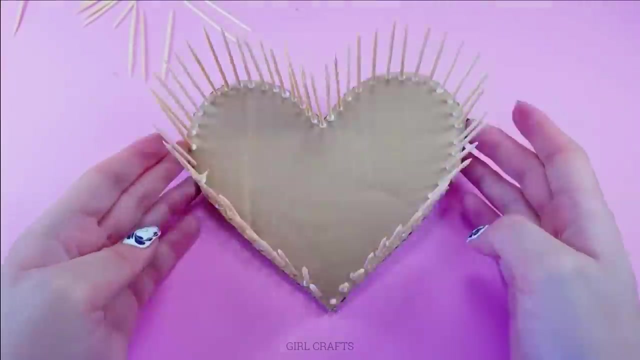 Your love takes me to the other side When I'm paralyzed and can't decide. Your love takes me to the other side When I'm stranded and I need a guide. Your love takes me to the other side When I'm catching up but still behind. Your love takes me to the other side. 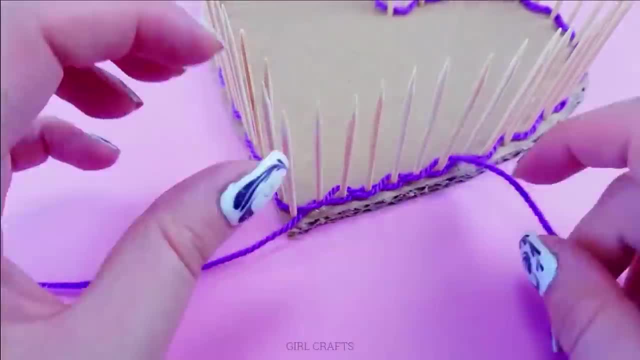 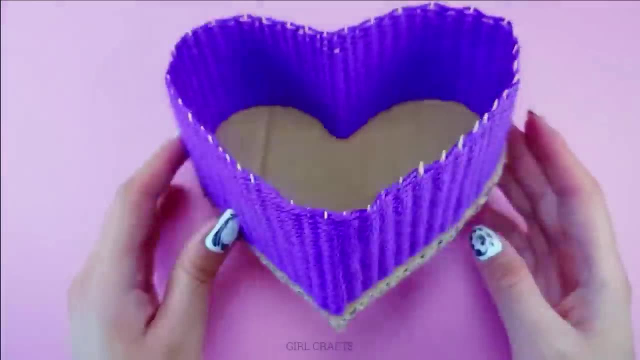 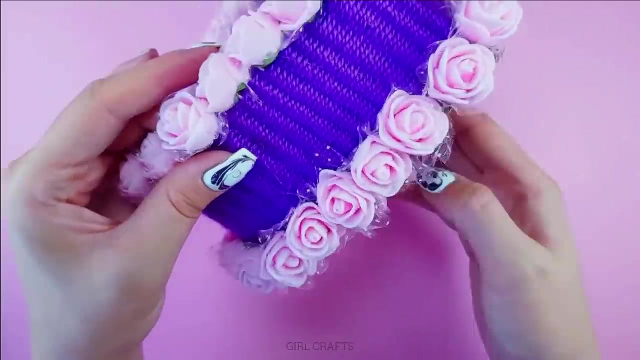 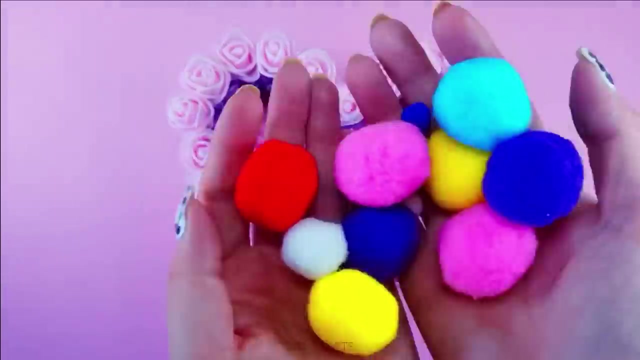 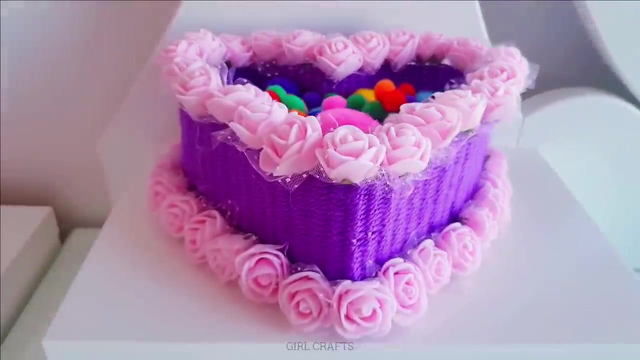 Your love, your love. It takes me to the other side. Your love, your love, Your love takes me to the other side. Your love takes me to the other side When I don't think that I can survive, When there's nothing but about goodbye, When life decides to be unkind. 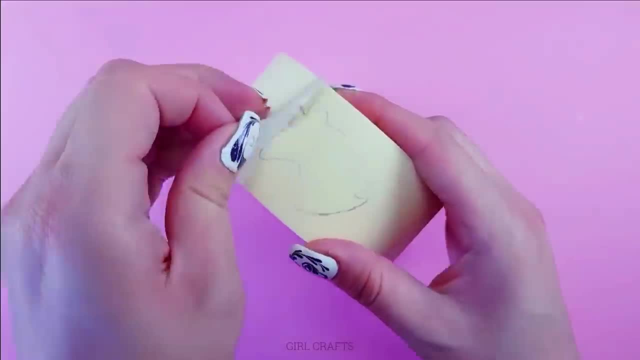 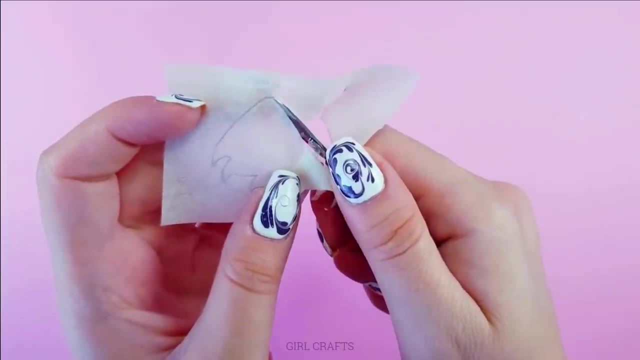 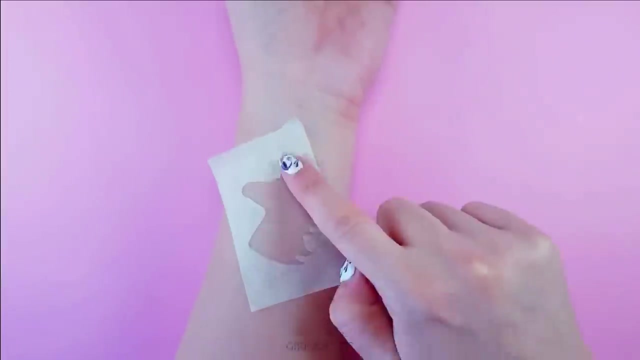 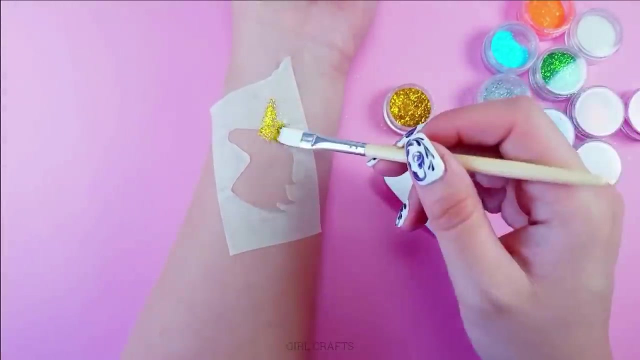 Your love takes me to the other side. When there's nothing but about goodbye, When I keep wandering but don't arrive, When the sun is hiding from the sky, When I'm feeling like I lost my mind, Your love takes me to the other side. Your love, your love. 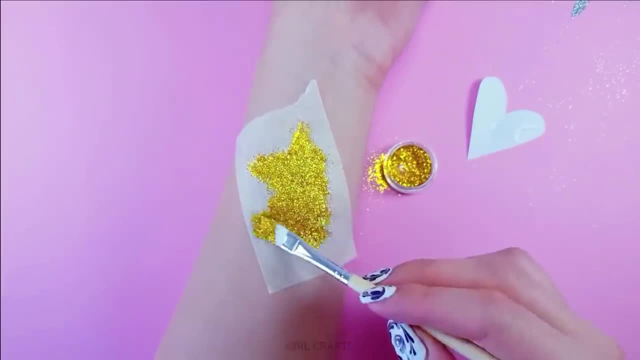 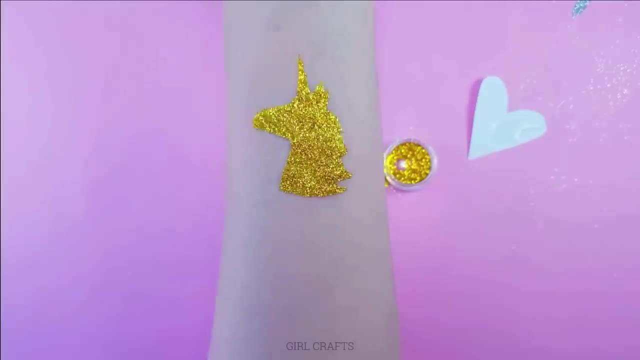 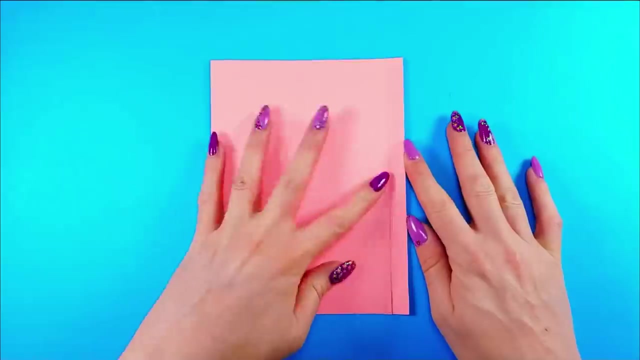 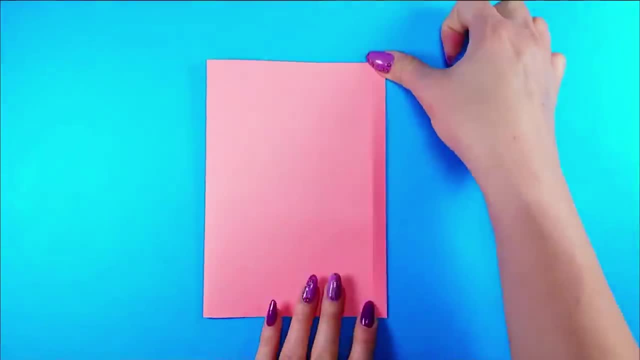 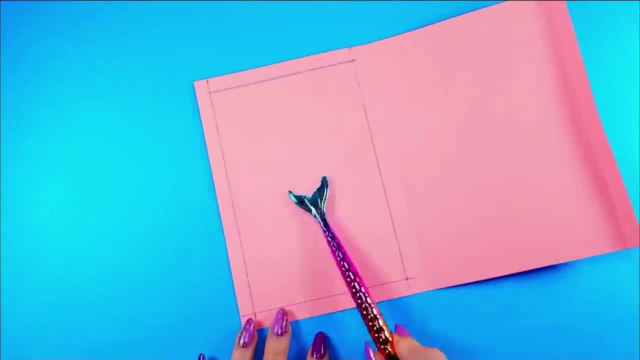 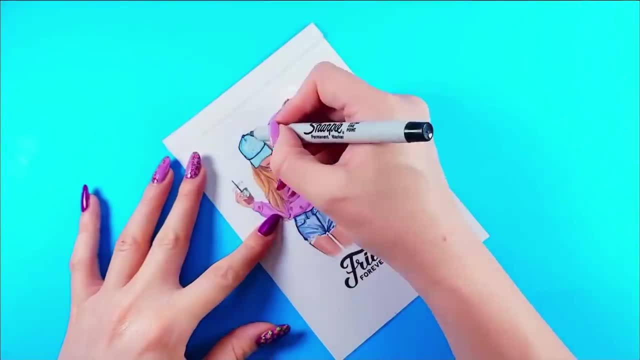 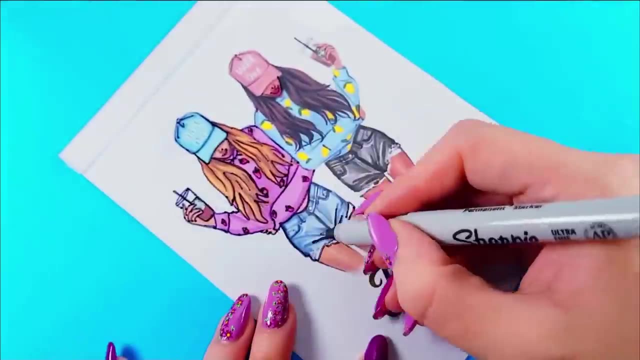 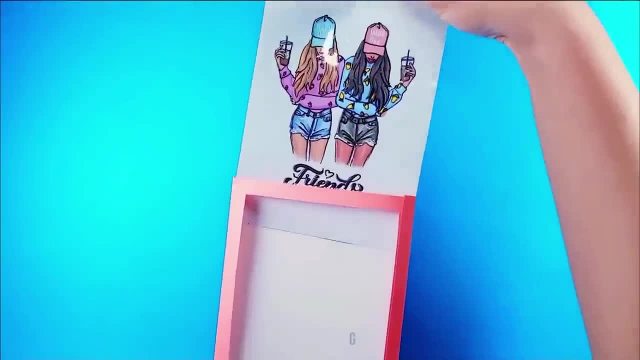 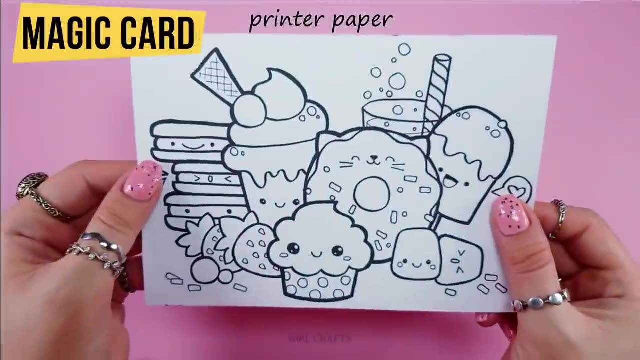 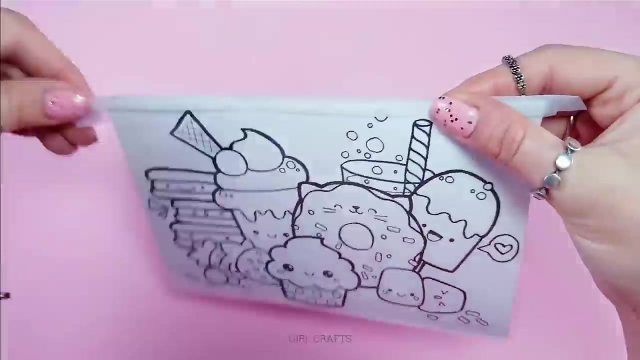 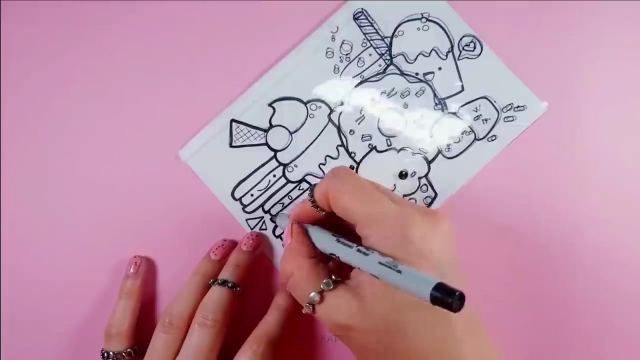 I'm wearing out my shoes. I can't make my mind up. I've got too much to lose. I'm old enough to leave home, Way too young to know what I should do. I'm trapped And in the water. I'm trying to keep my head above the ground. 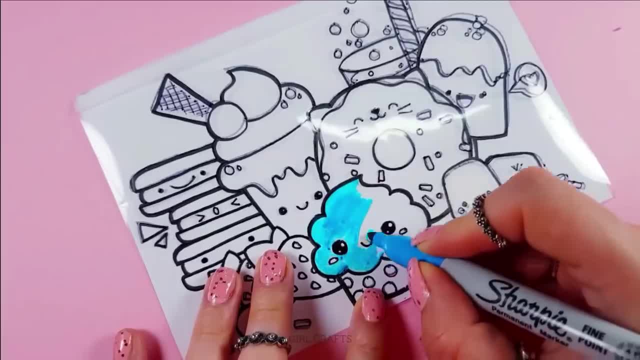 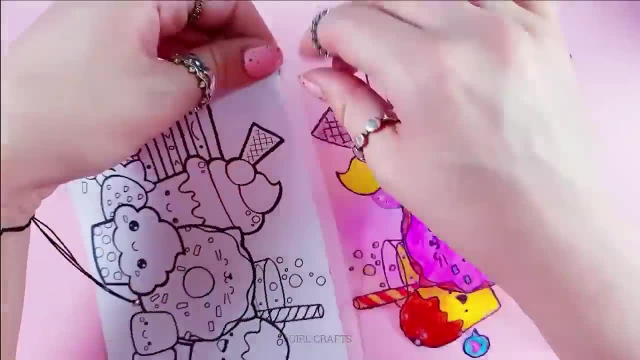 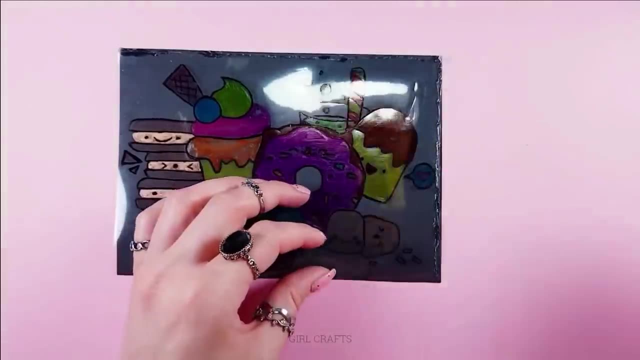 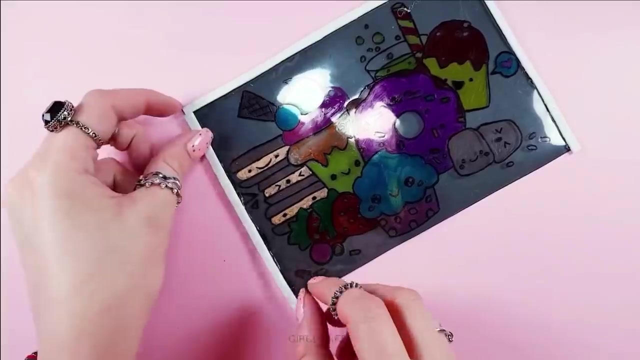 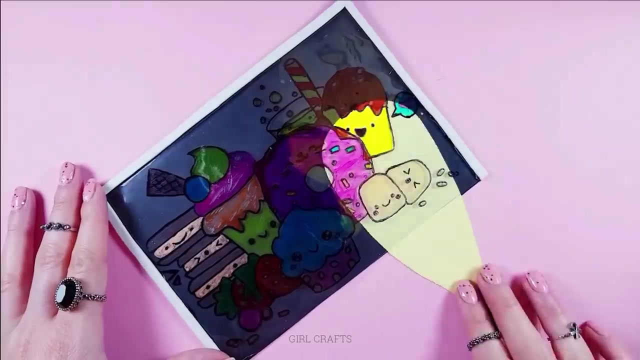 So would you come with me up to the oak tree. Time will stop for us again. Look back, remember, when, Yeah, we were just 18 under the oak tree. Safer than made open. Hold on to innocence. Where has the time gone? I'm feeling old and gray. 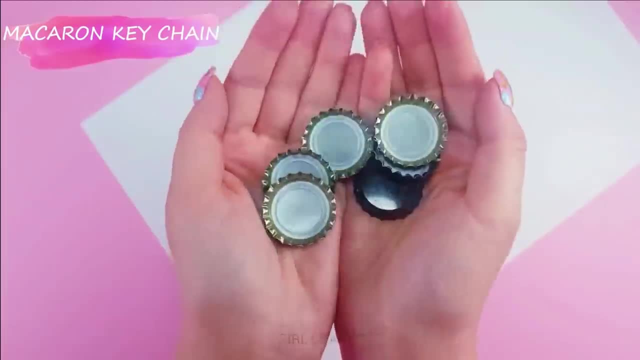 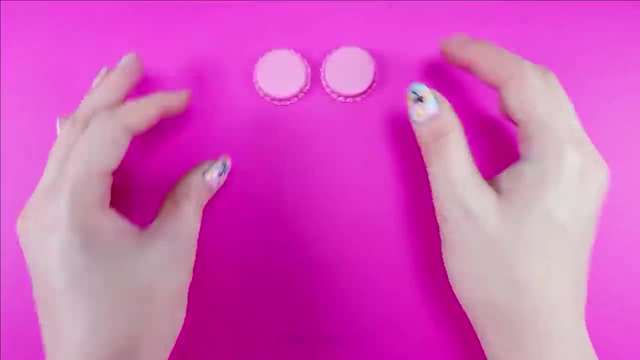 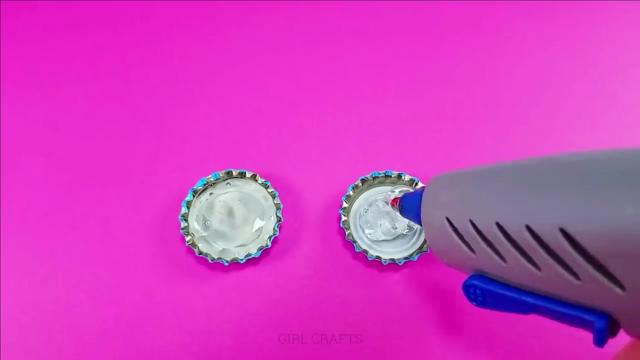 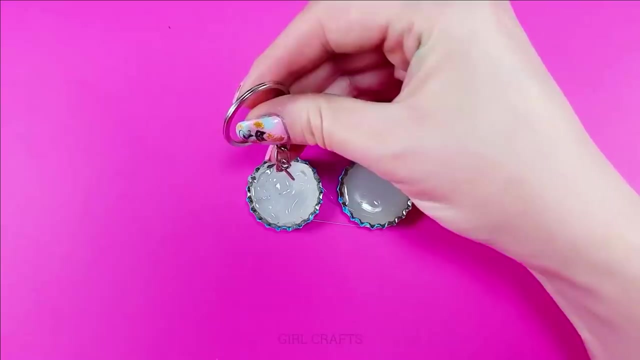 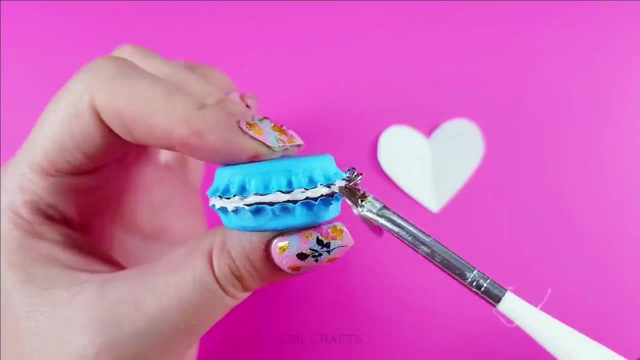 Trying to breathe revival into my broken ways. I'm old enough to leave home, But way too young to carry all the blame. I'm not alone, I'm not alone, And in the water I'm trying to keep my head above the ground. So would you come with me up to the oak tree. 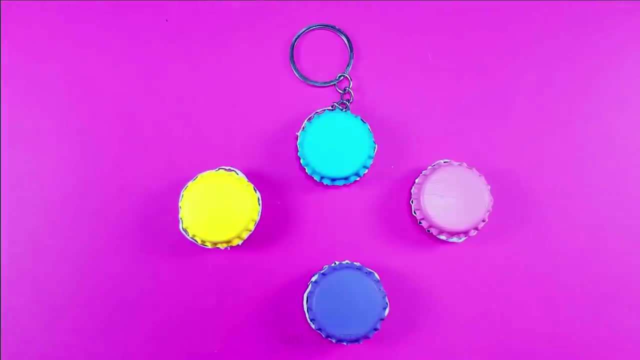 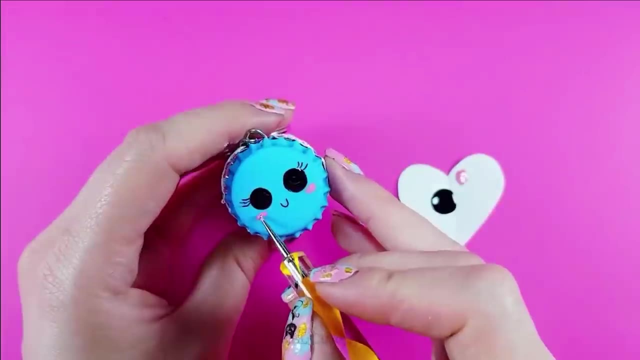 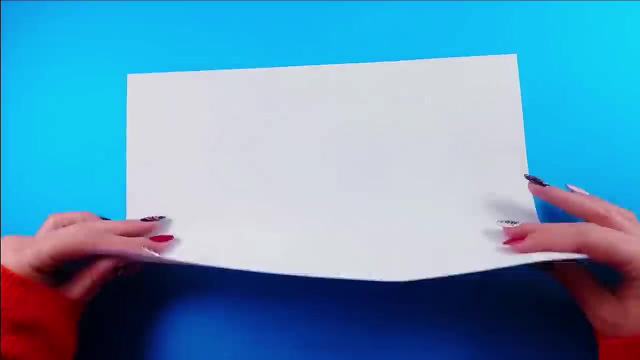 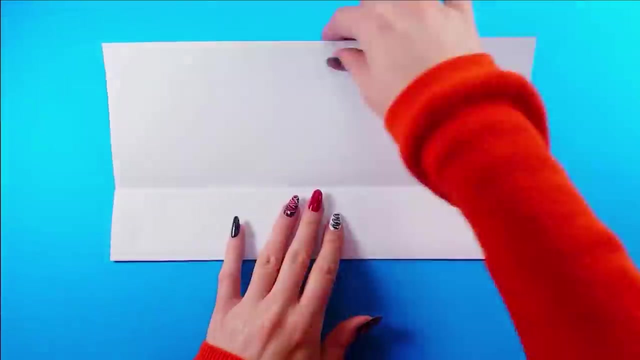 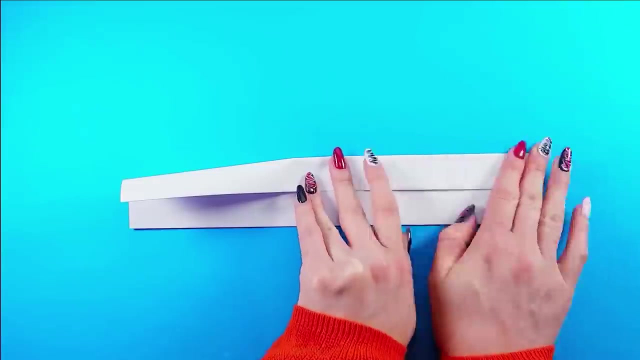 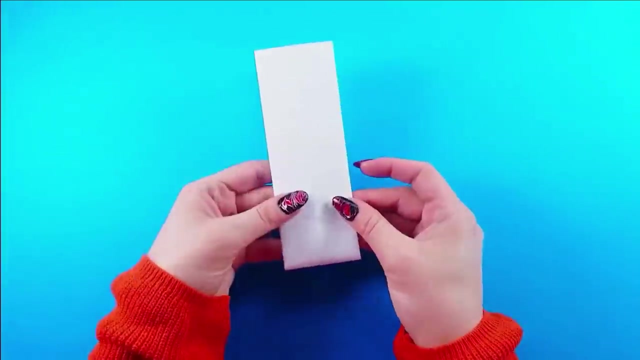 Time will stop for us again. Look back, remember when, Yeah, we were just 18 under the oak tree. Safer than made open. Hold on to innocence. We were young. Oh, we were young And we had time. How I hate the feeling that time It keeps slipping. 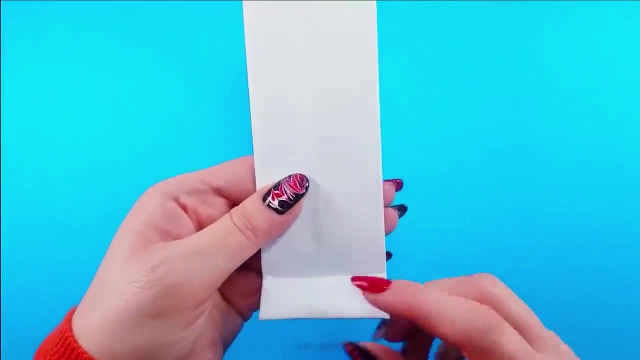 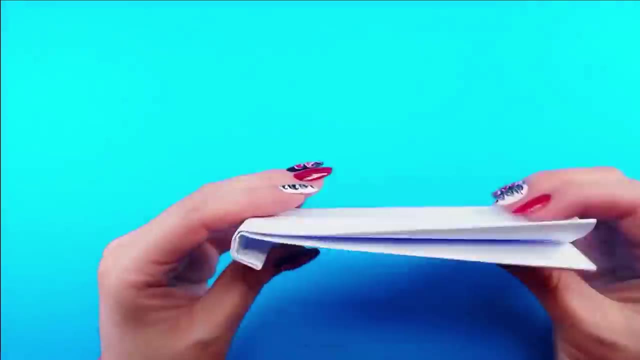 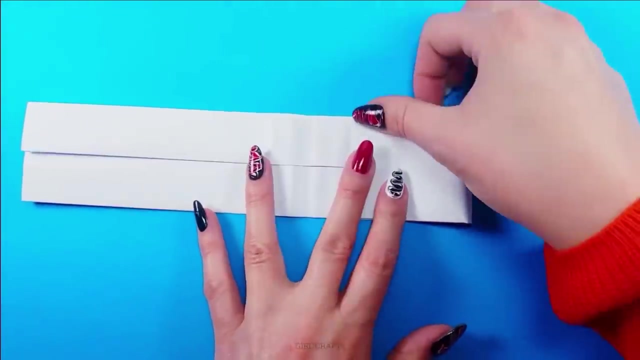 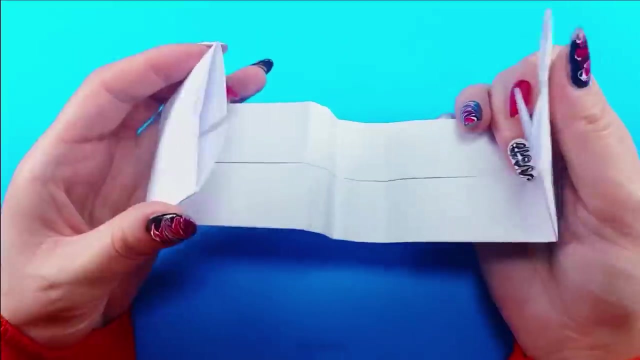 And it keeps slipping Away. The child in me is kicking. Don't let a moment pass, Cause I can't bear to witness My parents age so fast. They're way too young to fly home, And I can't stand to watch the hourglass. I'm treading water. 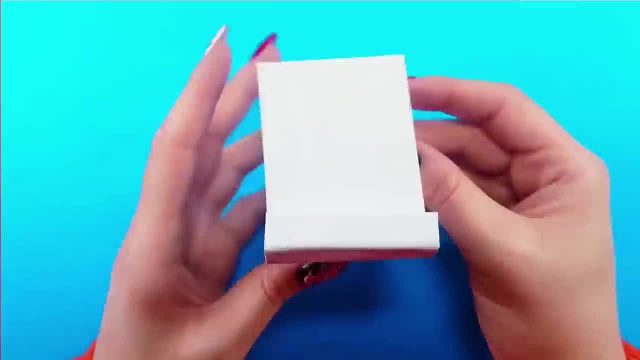 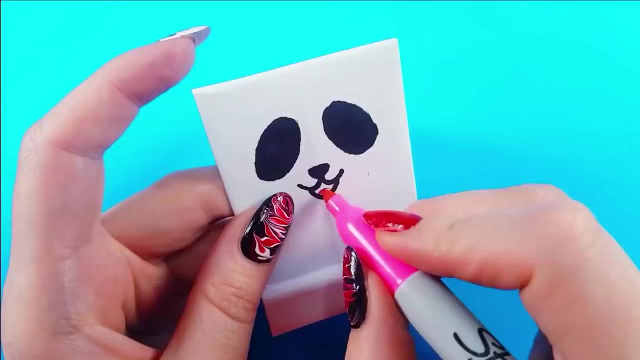 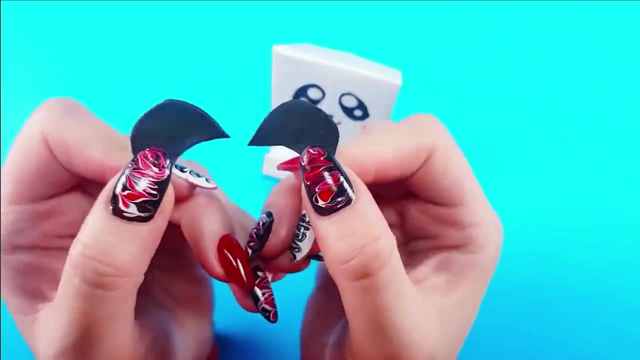 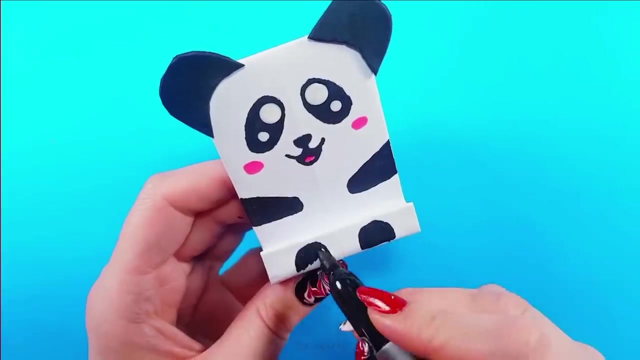 I'm trying to keep my head above the ground. I'm treading water. I'm trying to keep time from running out. So would you come with me up to the oak tree. Time will stop for us again. Look back, remember when- Yeah, we were just 18 under the oak tree. 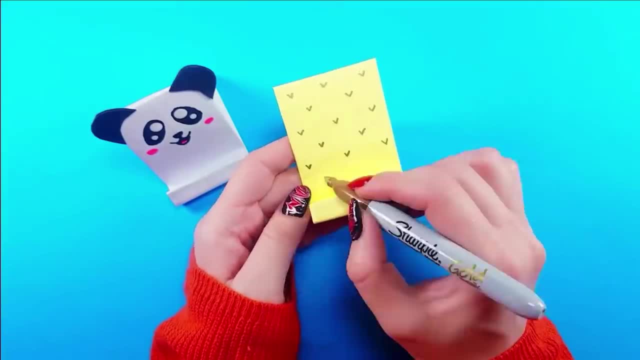 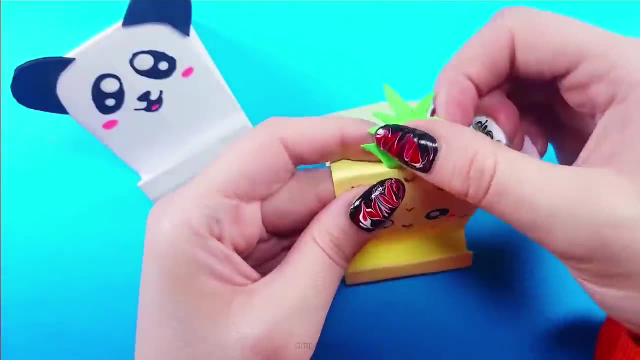 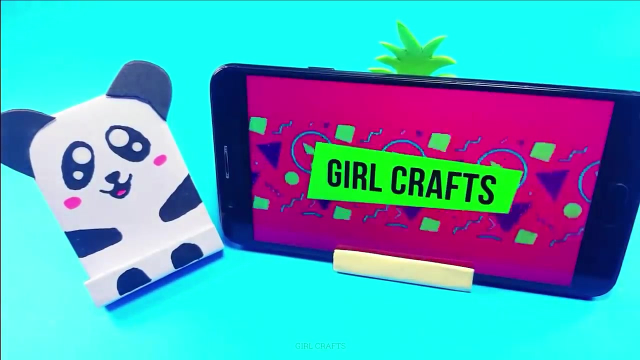 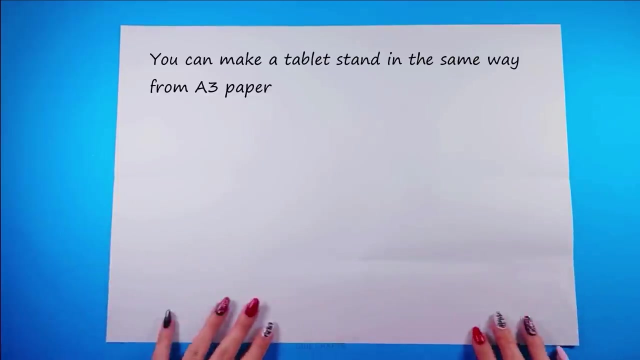 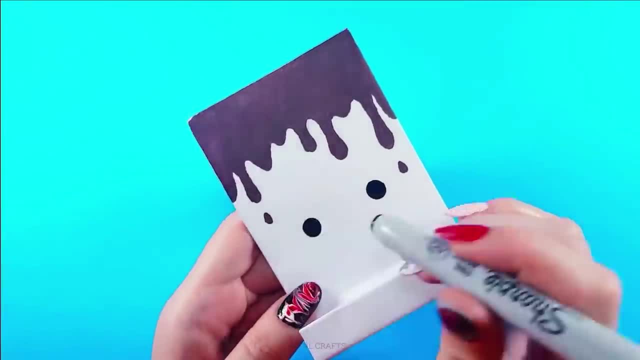 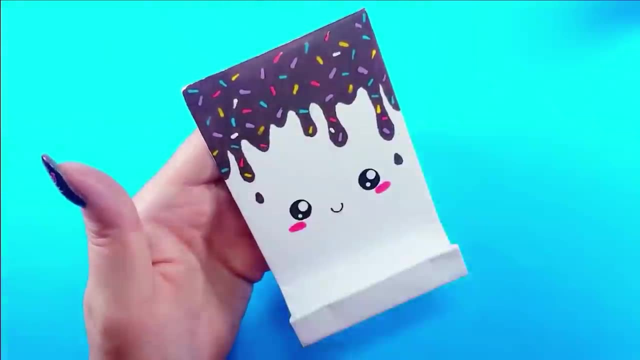 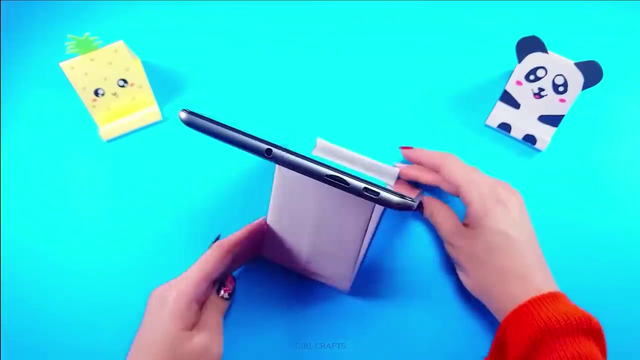 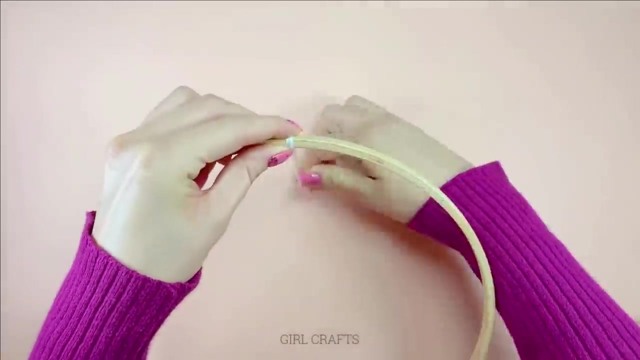 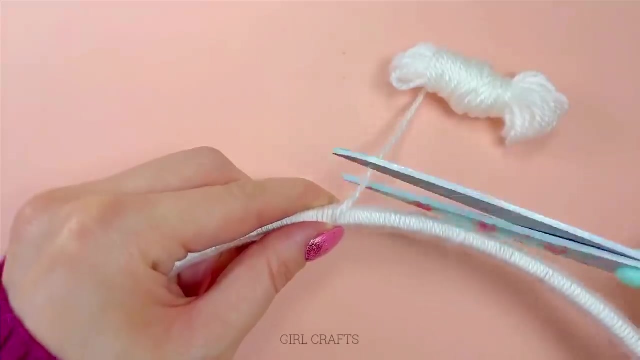 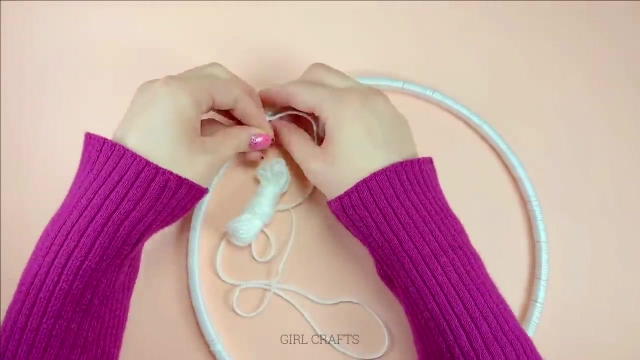 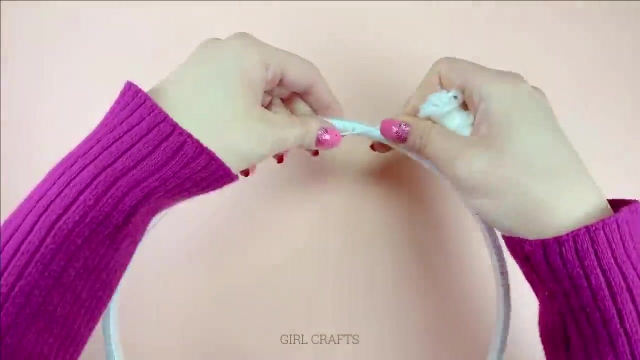 And to have time. There's no better day. it's time to get away. I want to see it all. The world is open wide. I want to feel alive. I hear adventure call. 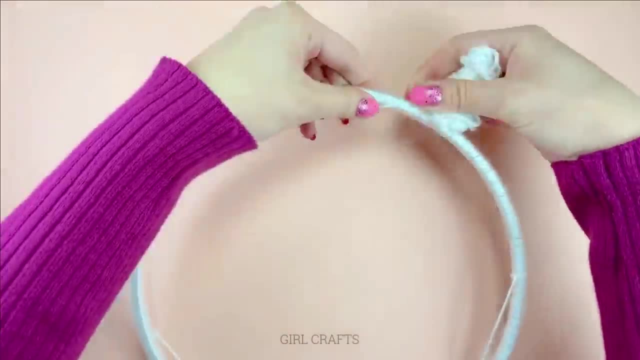 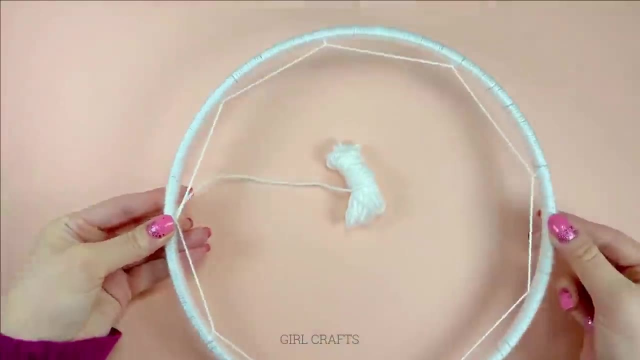 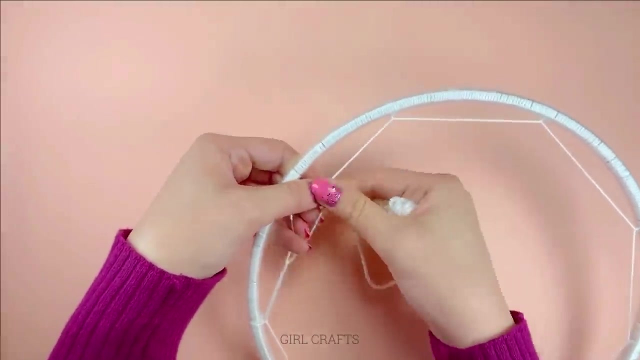 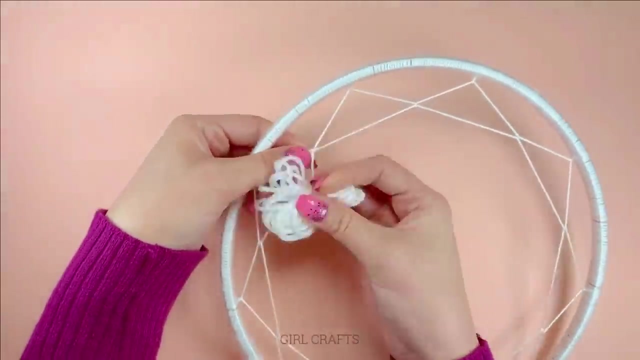 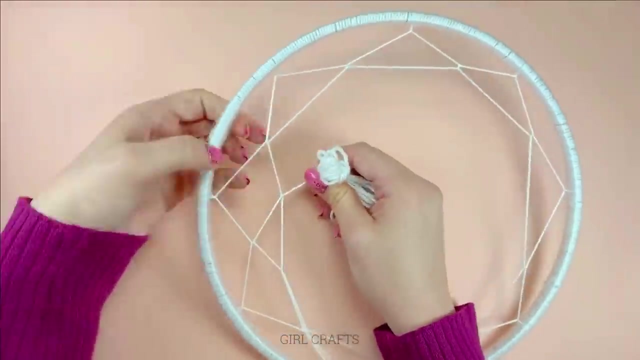 Hey, hey, what are you saying? Feels like a perfect day to get lost and find our way. We'll camp out in our cars, sleep under the stars. it's like the world is ours. oh yeah, This is the good life. This is the good life. 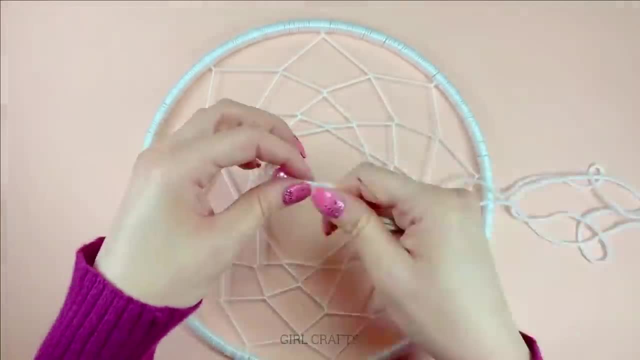 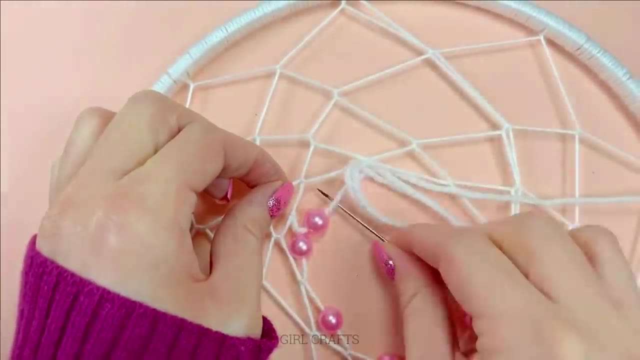 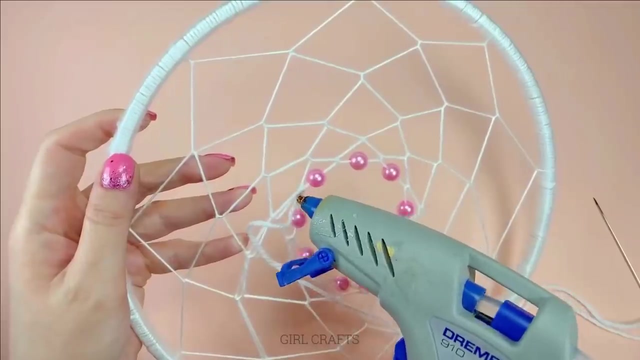 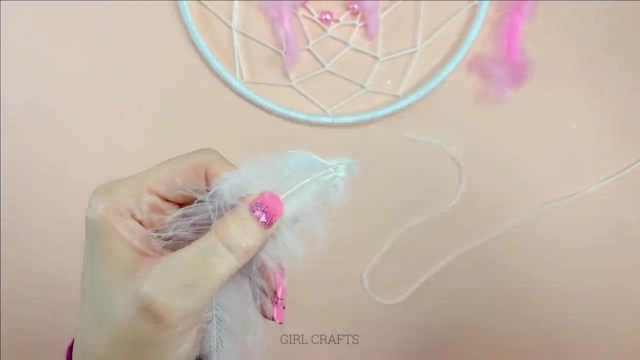 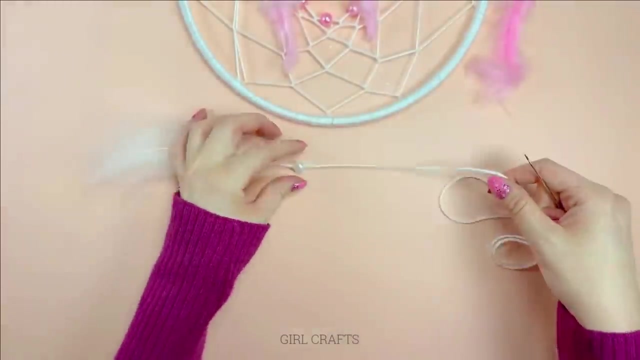 This is the good life. Follow the desert roads to where no man goes. we can see it all. Drive on through the night and look up at the brighter sky. can you hear adventure call? Hey, hey, what are you saying? Feels like a perfect day to get lost and find our way. 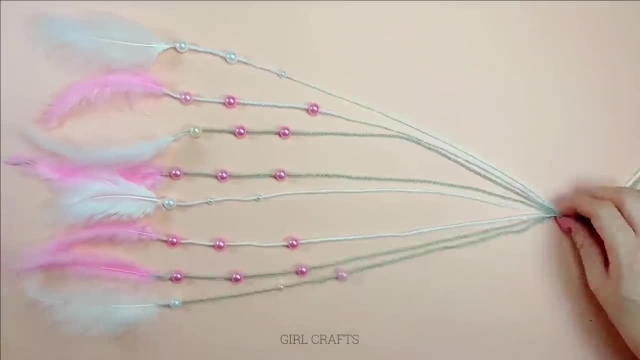 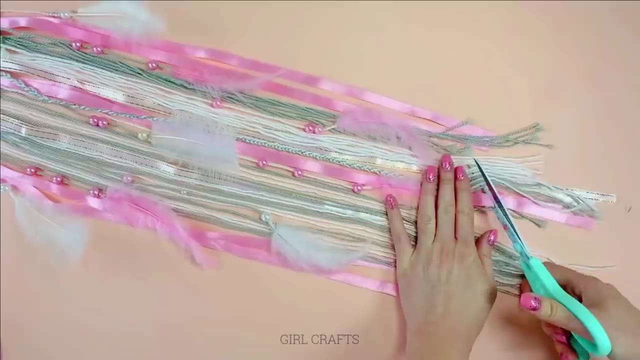 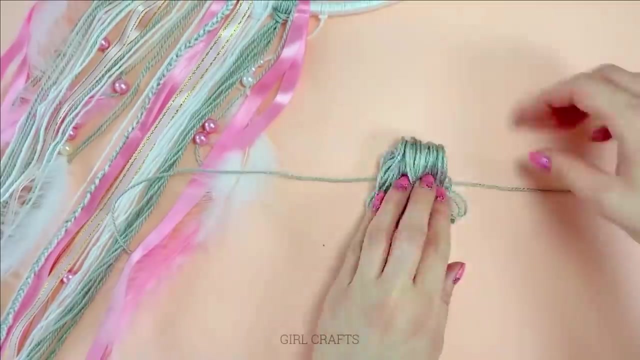 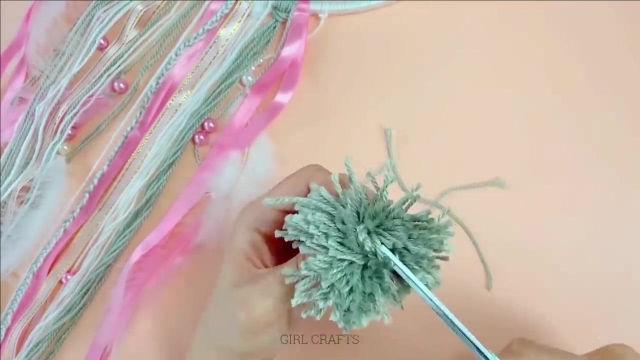 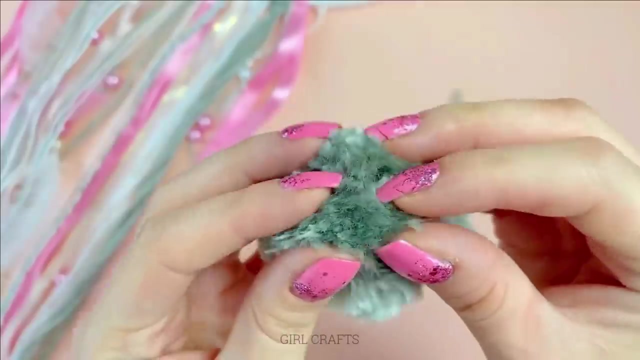 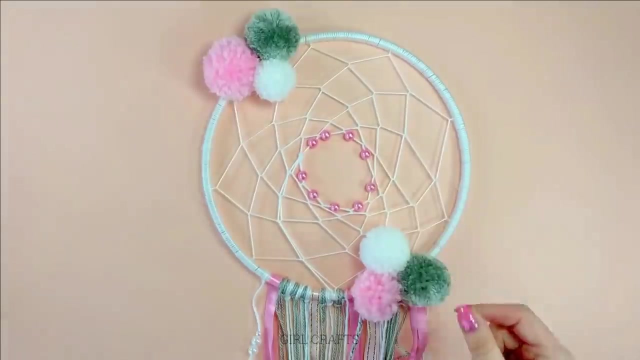 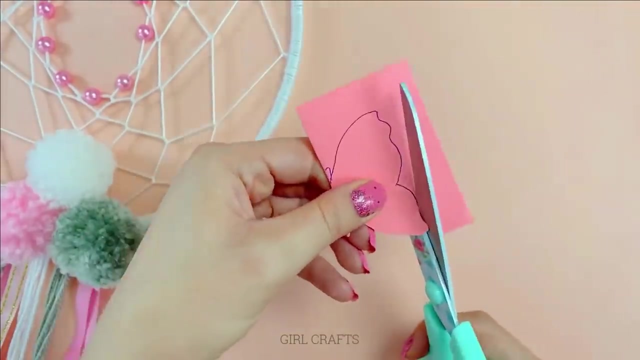 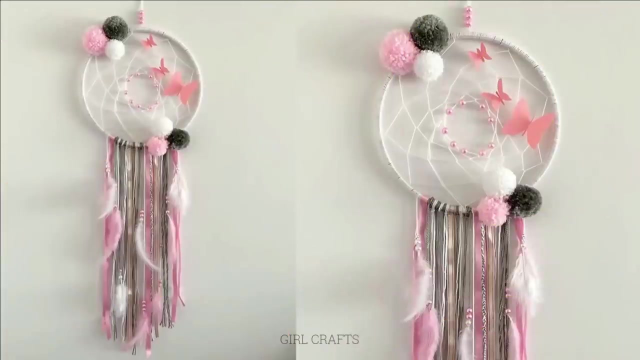 We'll camp out in our cars, sleep under the stars. it's like the world is ours. oh yeah, This is the good life. This is the good life. There's no better day. it's time to get away. I hear adventure call. now the world is ours. 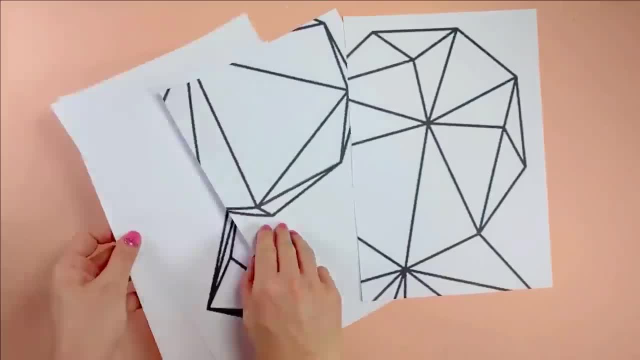 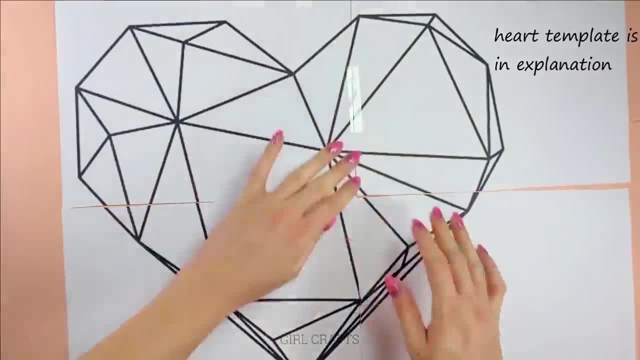 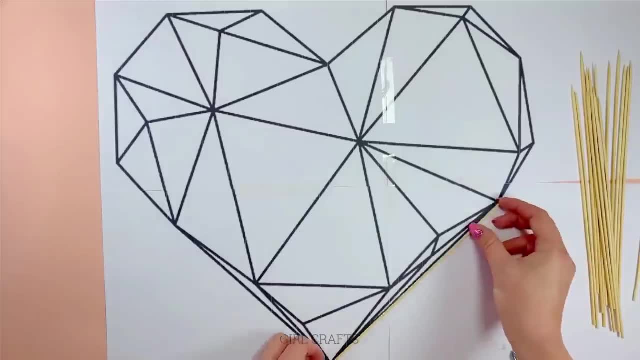 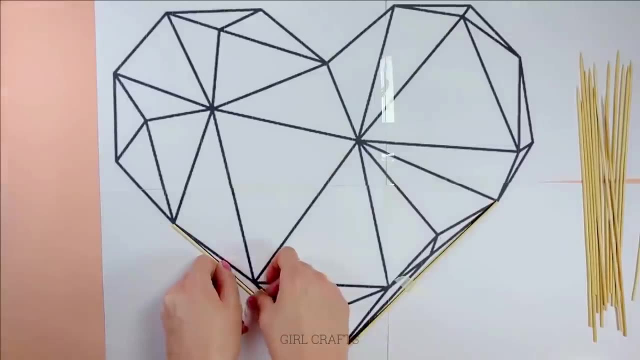 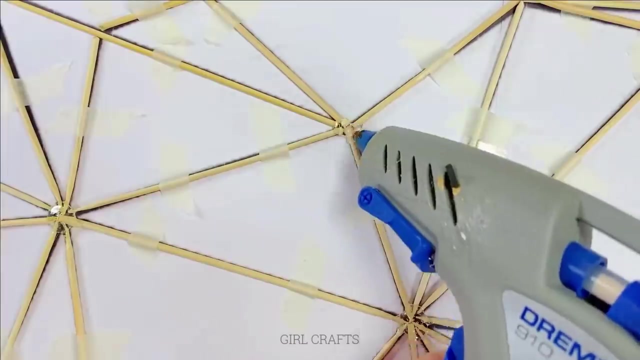 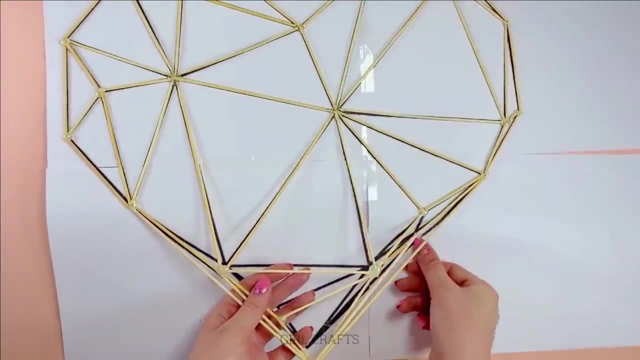 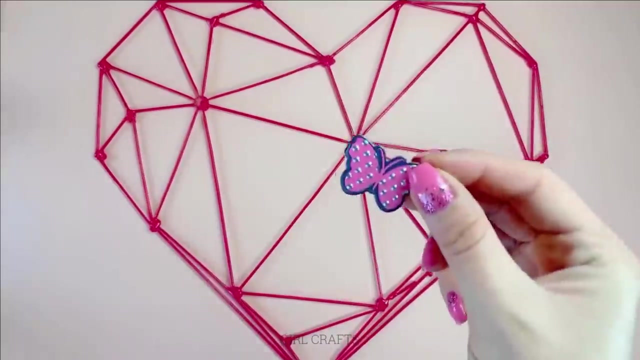 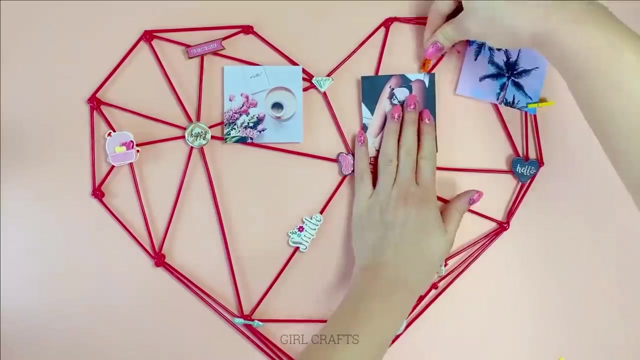 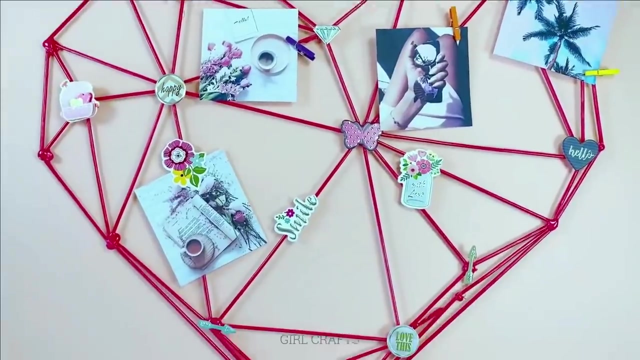 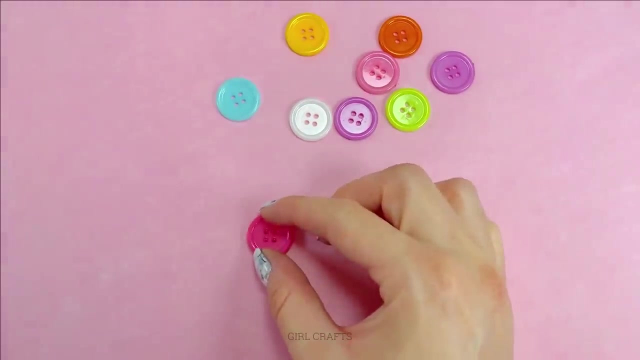 We'll camp out in our cars, sleep under the stars. it's time to get away. This is the good life. This is the good life. This is the good life. It's like running through an open door. It's like finding what you're looking for. 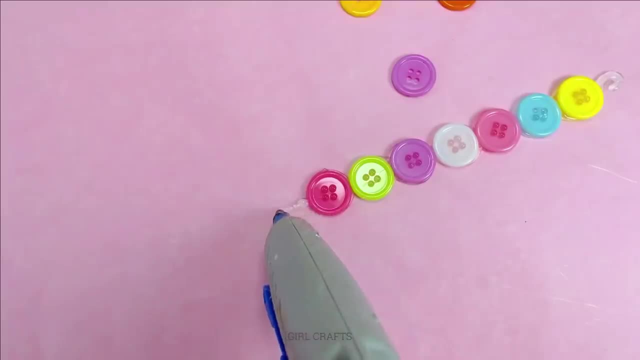 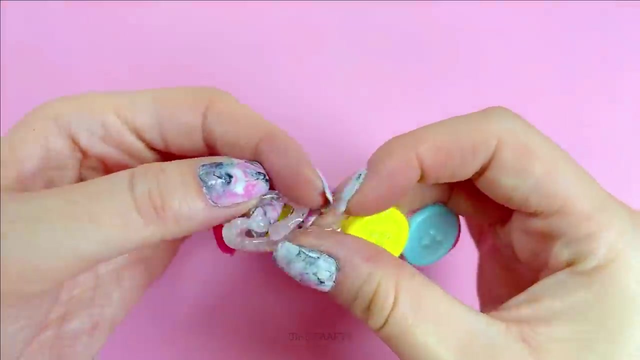 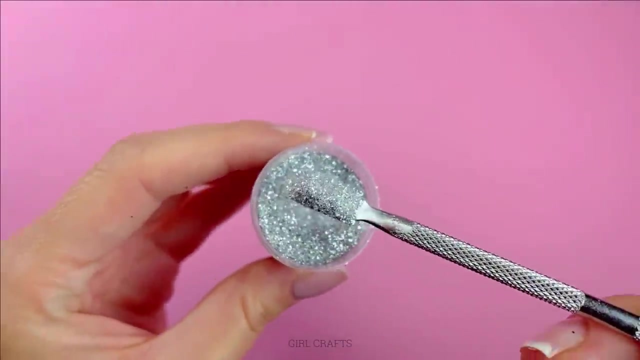 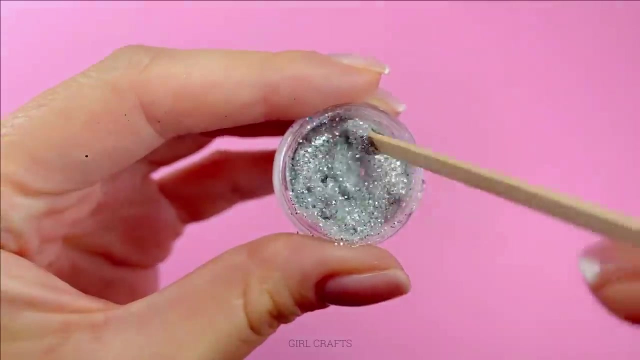 We've been waiting. we won't wait no more. Every season, every memory made All the dreaming, that is here today. Can you see it? We got a beautiful story Every moment, on and on. We got a beautiful story And we've only just begun. 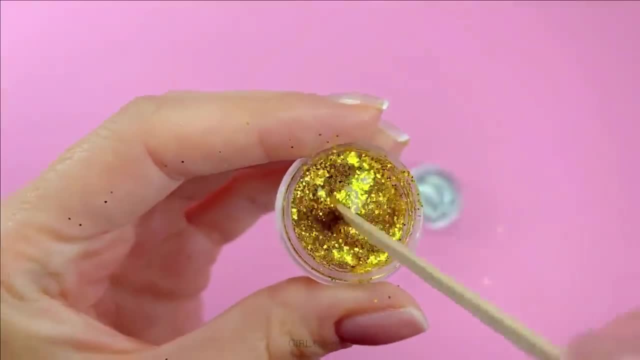 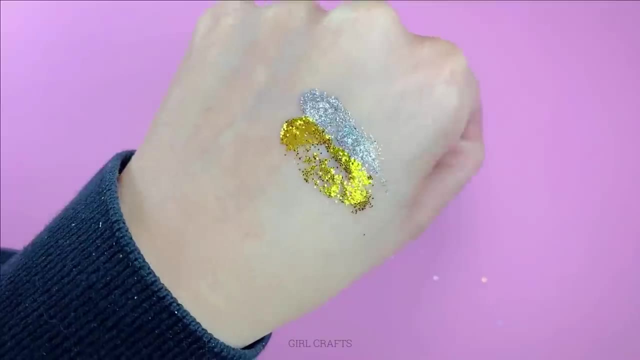 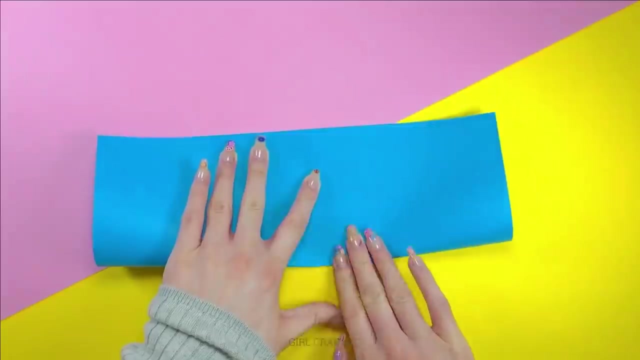 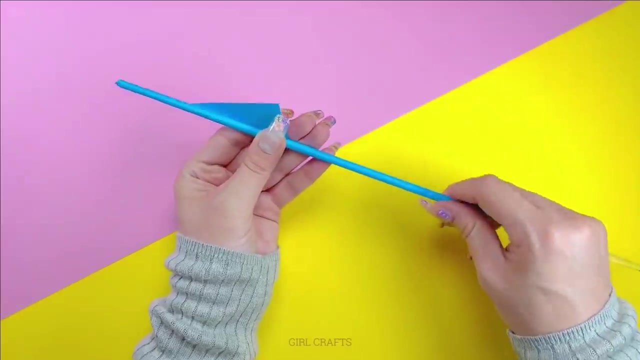 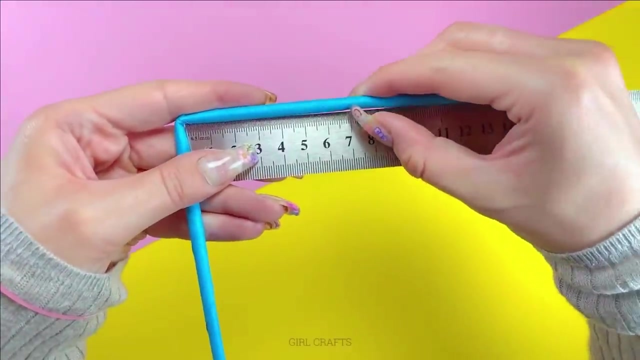 The best is yet to come. We got a beautiful story. The best is yet to come. Never felt my heart beat so wild While the sunset sets the night on fire, You and me here, and it feels so right. We got a beautiful story Every moment on and on. 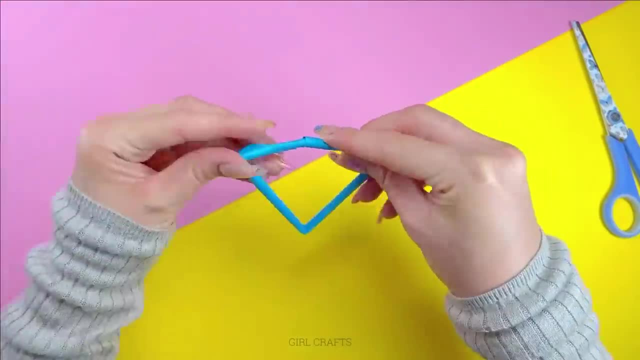 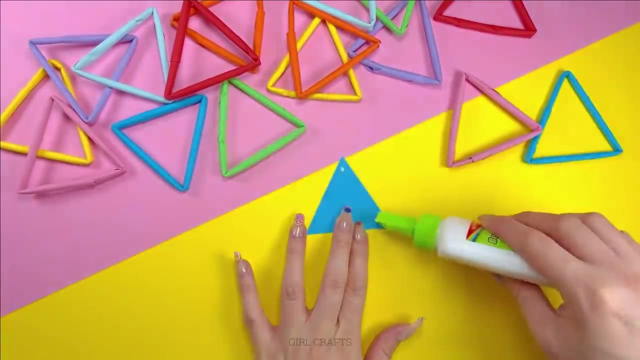 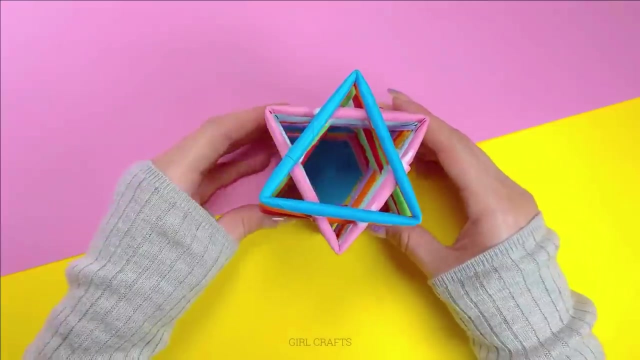 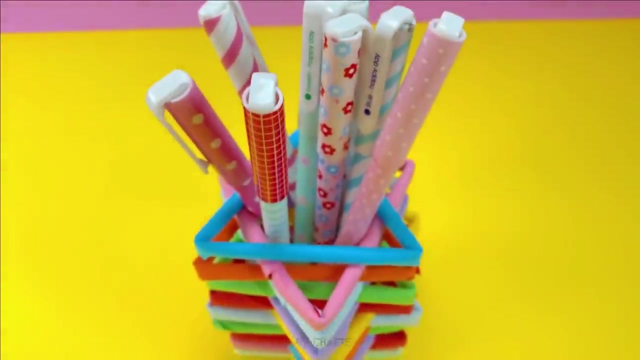 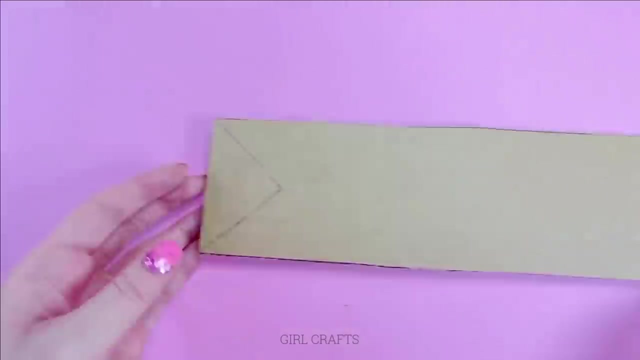 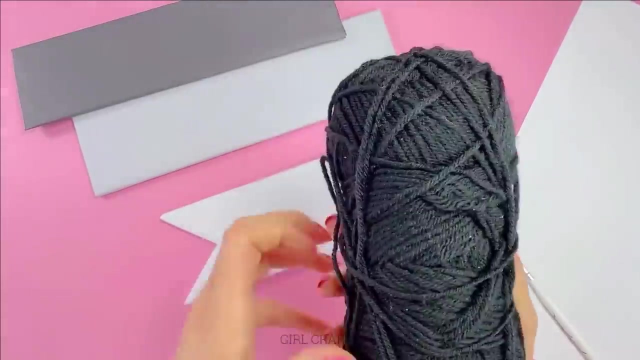 Every moment, on and on. We got a beautiful story, And we've only just begun. The best is yet to come. The best is yet to come. It's like running through an open door. It's like finding what you're looking for. We got a beautiful story. 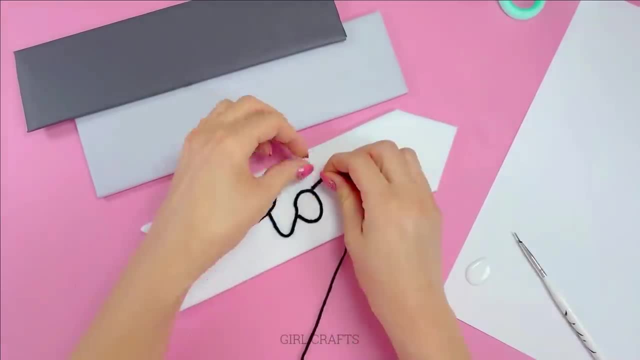 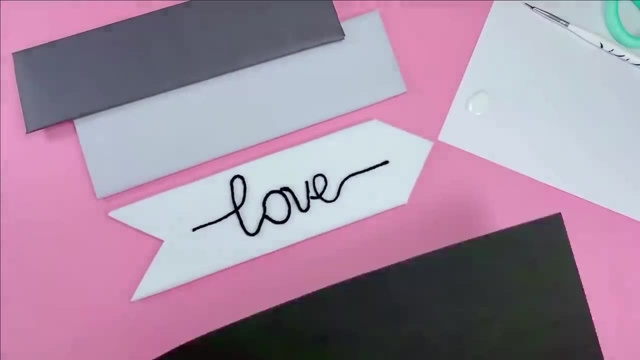 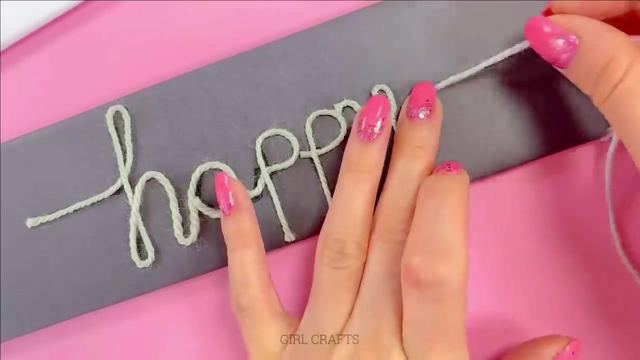 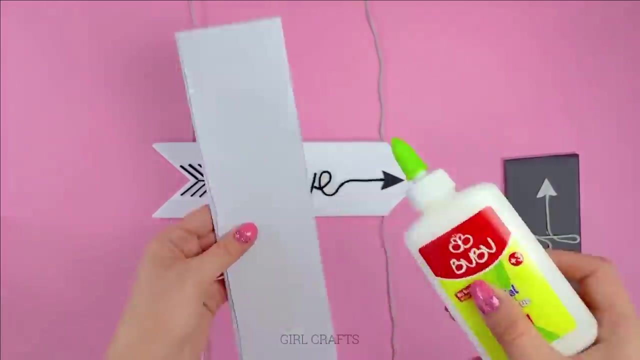 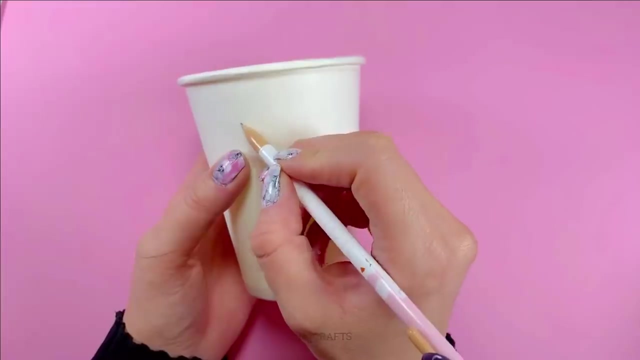 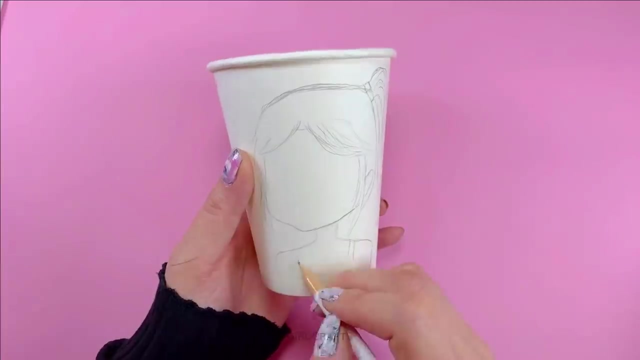 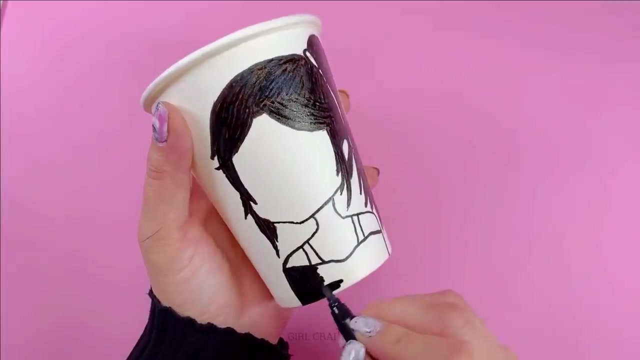 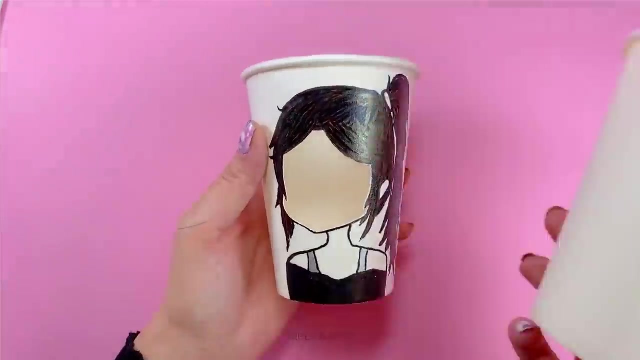 Every moment, on and on. We got a beautiful story, And we've only just begun. The best is yet to come. We got a beautiful story. The best is yet to. the best is yet to come. The best is yet to come. What has gotten into me? it's like I'm in some dream. 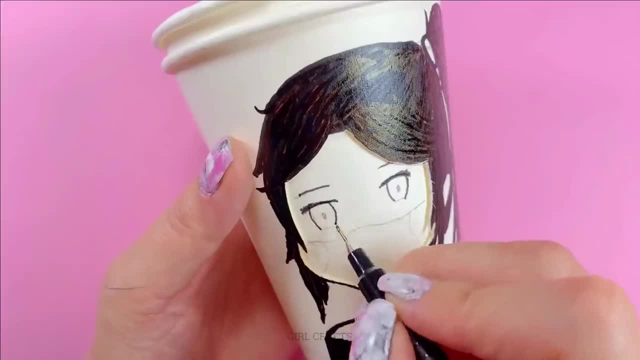 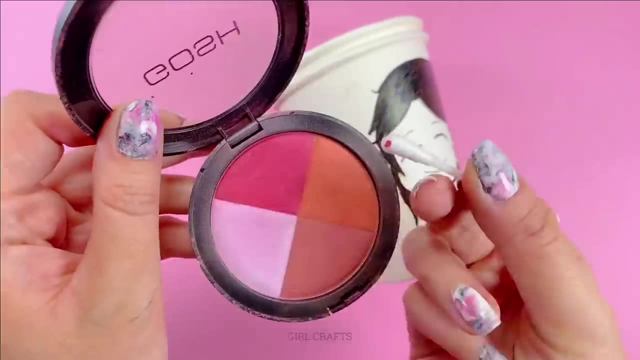 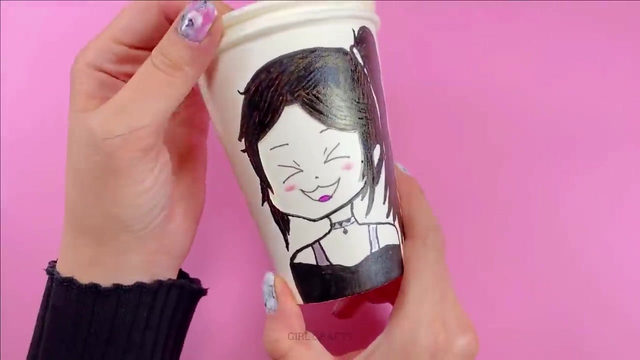 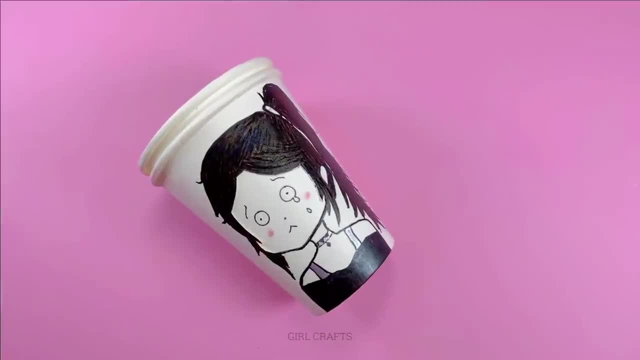 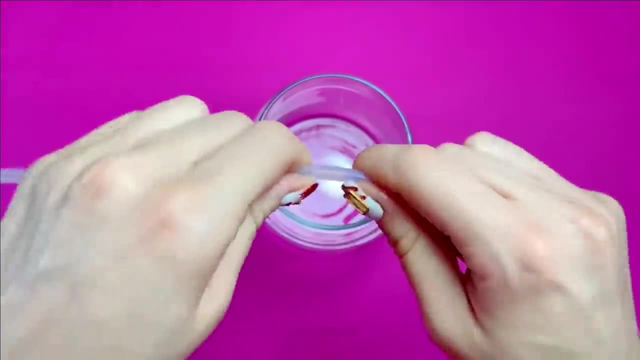 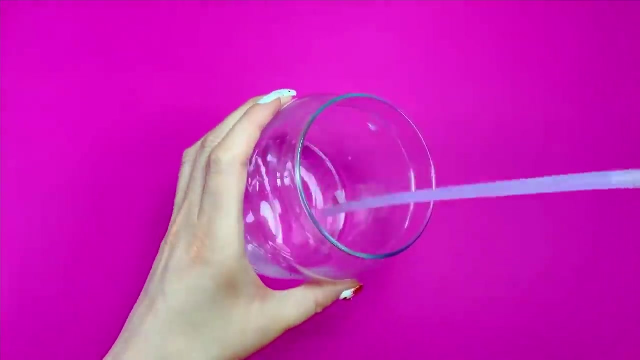 I just know I want it, that thing. Give me that thing that you do. Give me that right next to you. Give me that buzzing underneath my skin again. Show me that, look in your eye And, baby, I think I can fly. Give me you that thing that you do. 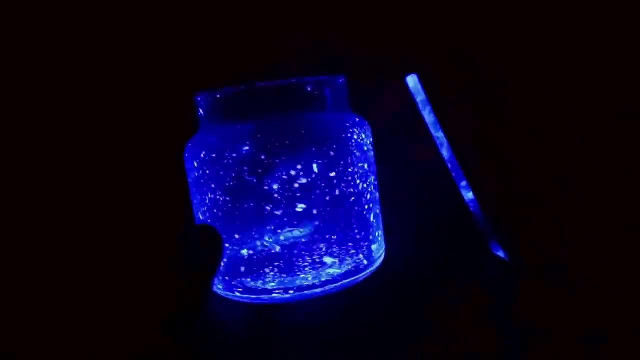 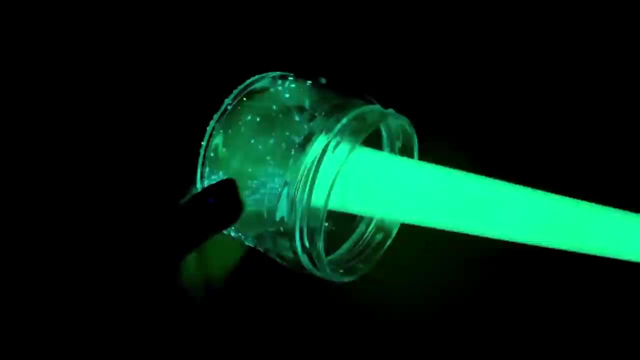 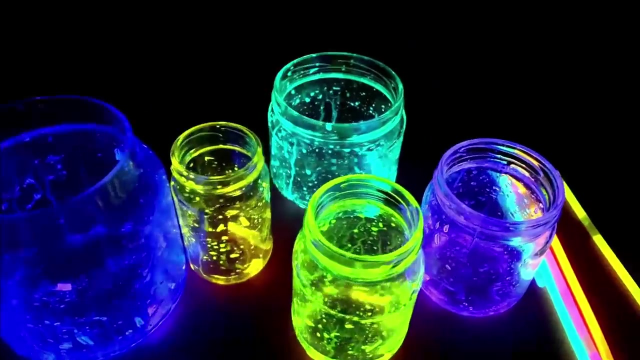 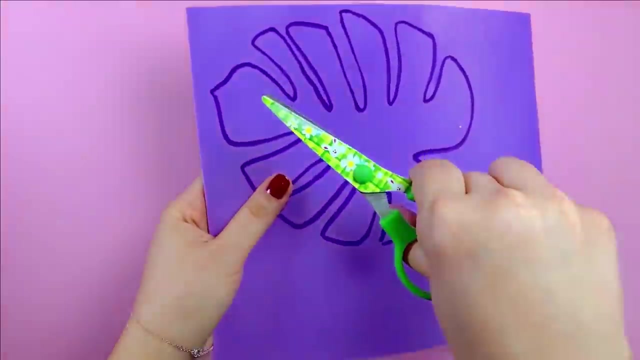 That thing that you do? Whoa-oh-oh-oh-oh-oh, Whoa-oh-oh-oh-oh-oh, That thing that you do. People think we've lost our minds, But we just can't hide. We're a little crazy. 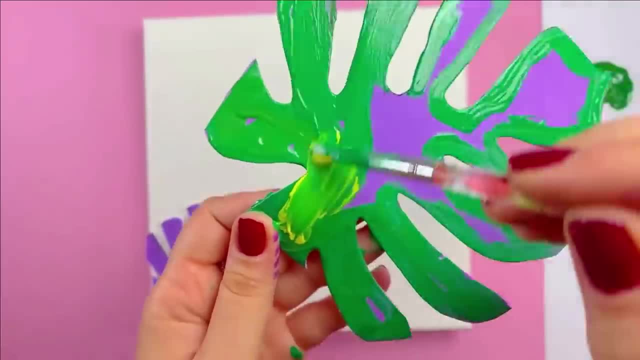 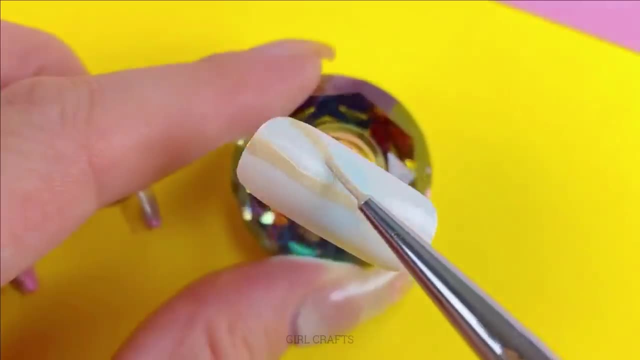 And I swear to you that I'm not high. I'm just high on life And a little love drunk. Can't put my finger on it, Will no one understand That I'm just gonna lose it? Can't put my finger on it Or find the words to explain. 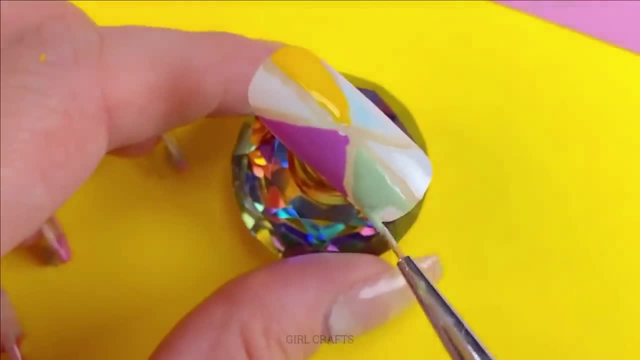 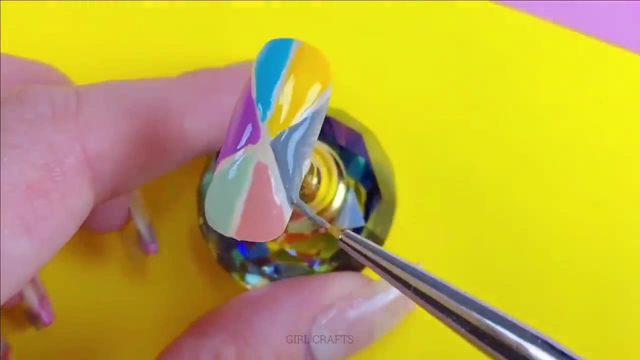 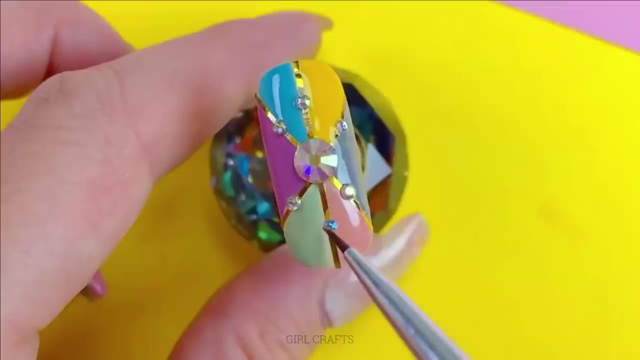 I just know I want it, that thing. Give me that thing that you do. Give me that right next to you. Give me that buzzing underneath my skin again. Show me that, look in your eye And, baby, I think I can fly. Give me you that thing that you do. 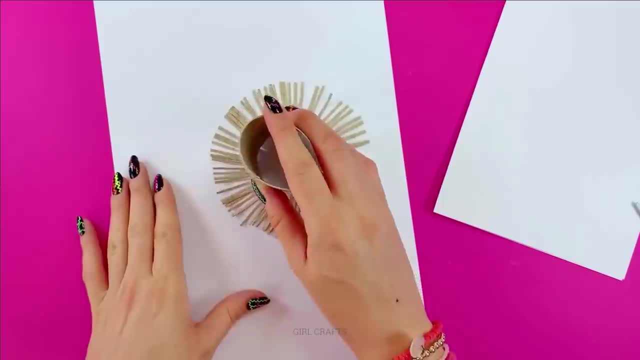 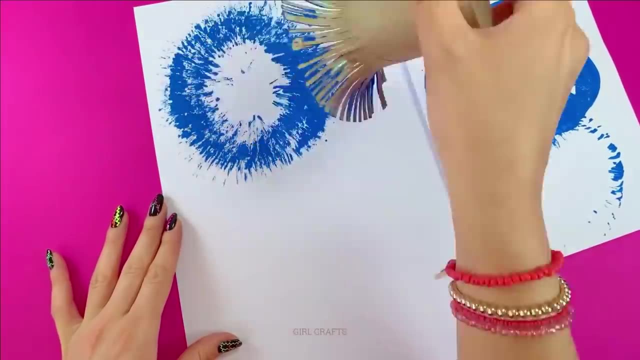 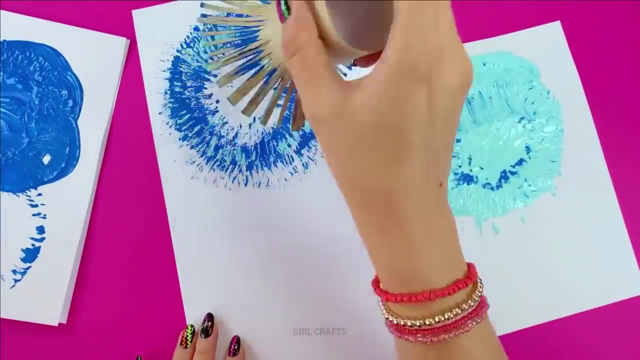 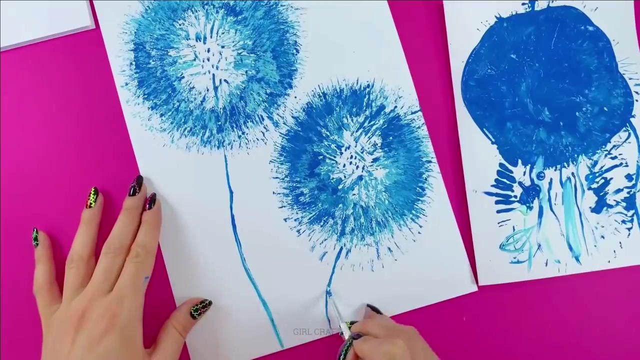 Well, whoa-oh-oh-oh-oh-oh, That thing that you do, That thing that you do. Somewhere along the line, Someone will say that you'd be better if you were somebody else. Hey, then don't mind, I promise. there is no one better than you at being yourself. 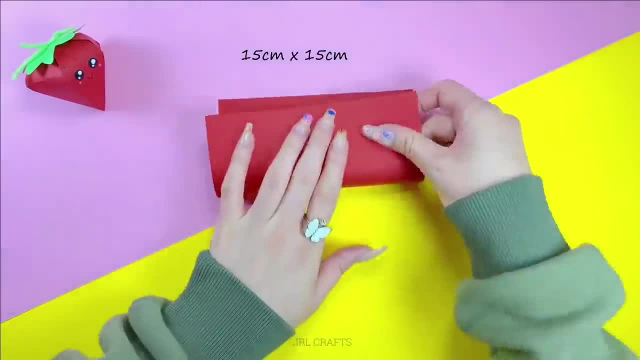 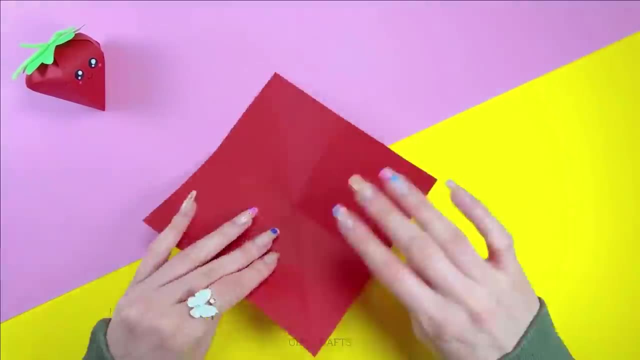 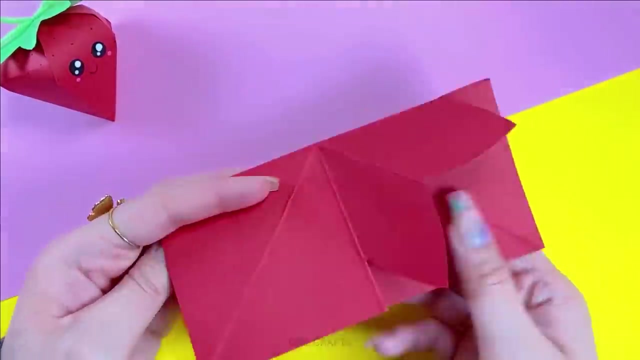 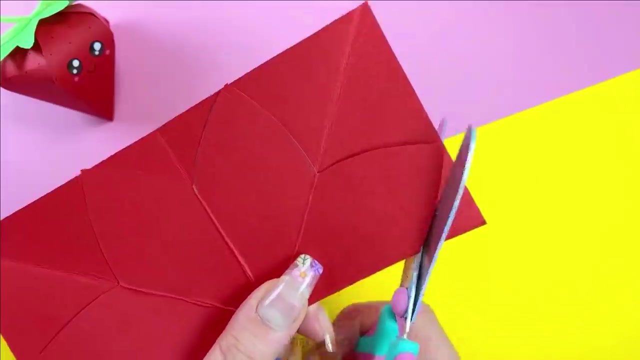 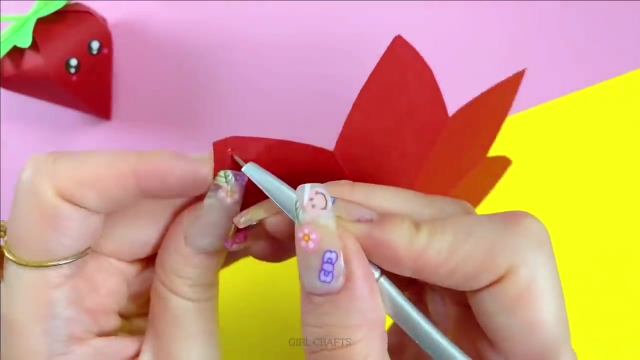 So, come on, just be you. Do that thing, you do That thing that you do. Give me that thing that you do. Give me that right next to you. Give me that below That thing that you do, Is it underneath my skin again? Show me that. look in your eyes. 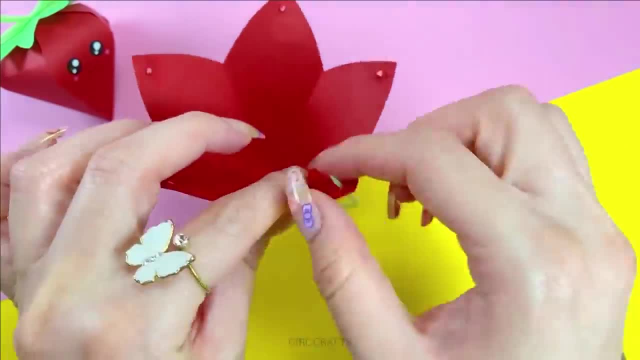 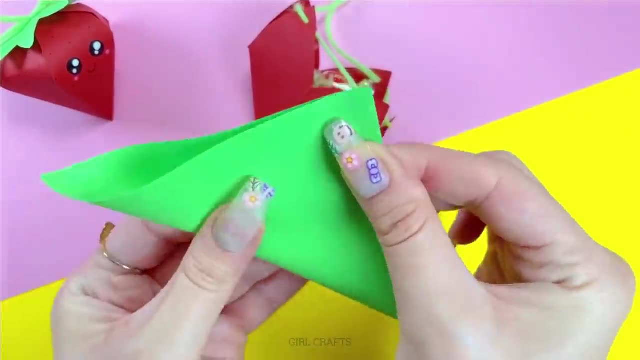 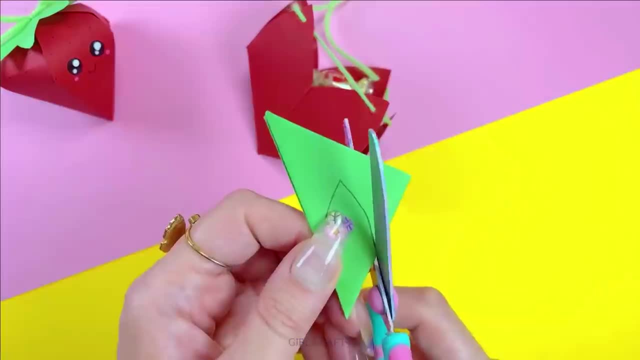 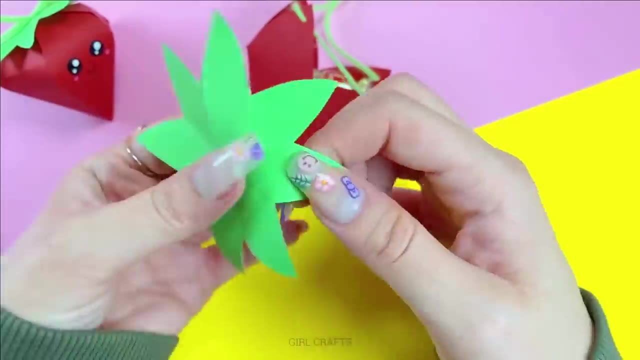 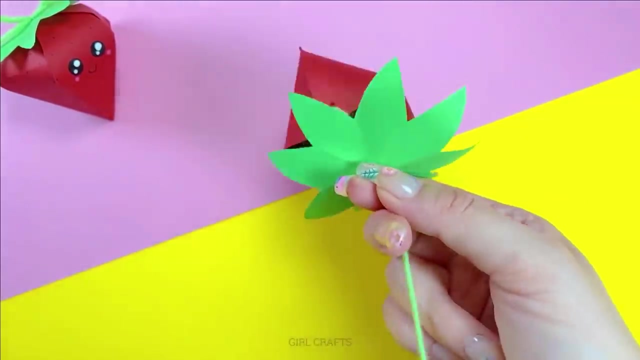 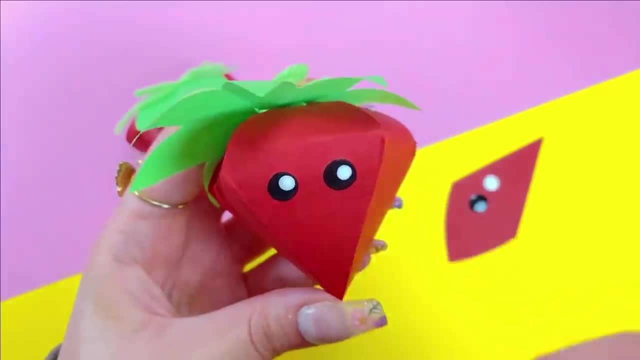 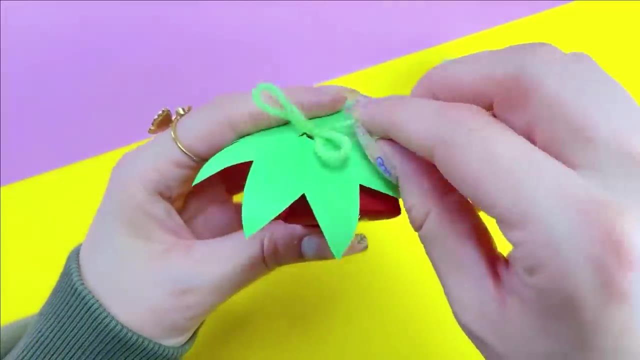 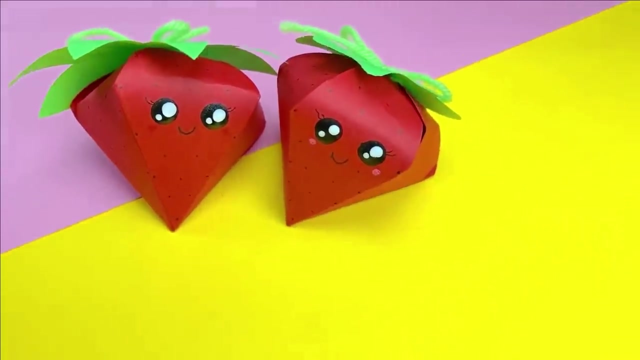 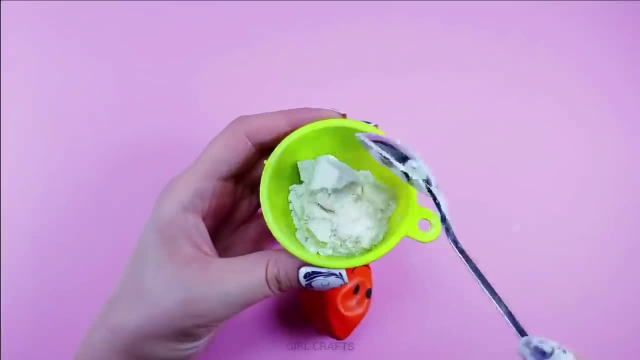 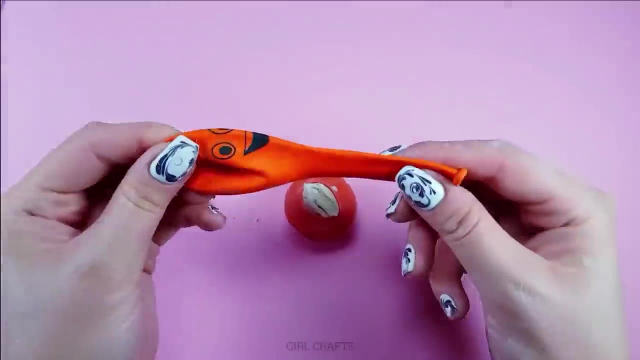 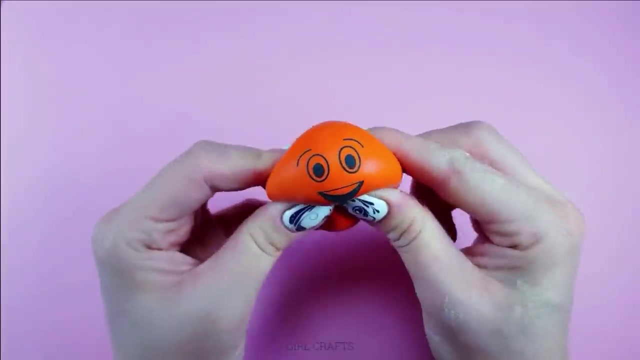 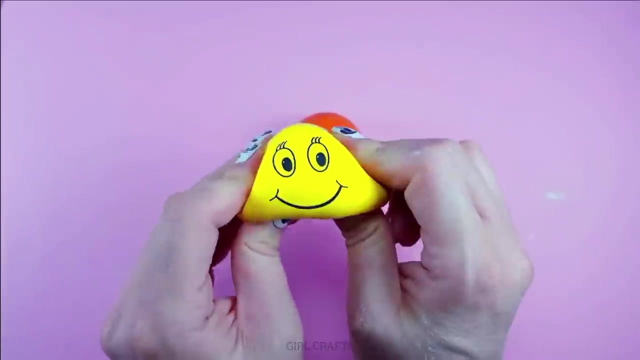 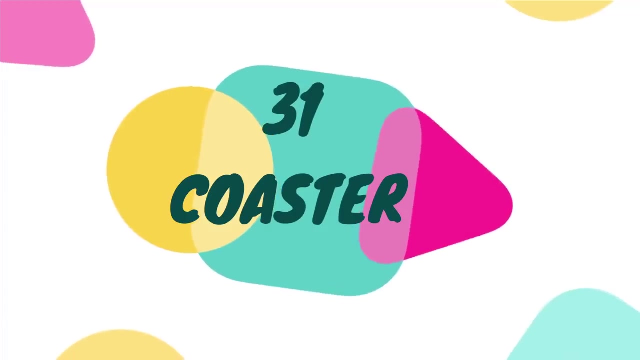 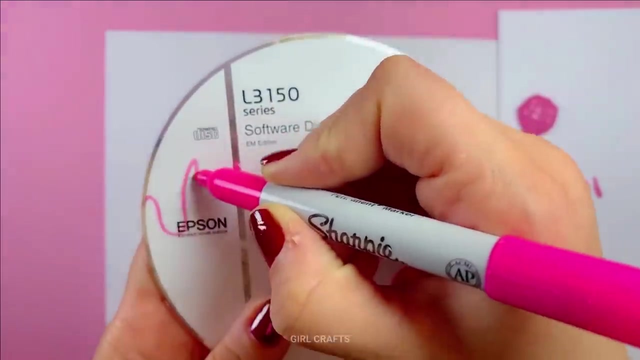 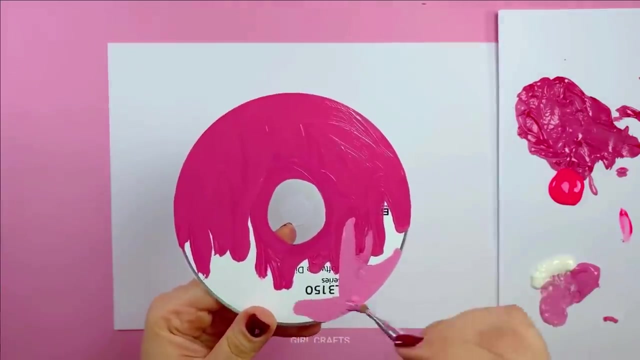 Way to spend the day just dreaming. Way to spend the day just hoping You'll feel the same Way to spend the day just dreaming. Way to spend the day just dreaming. Way to spend the day just dreaming. But I'm boom, boom, boom. I got the birds in the air. 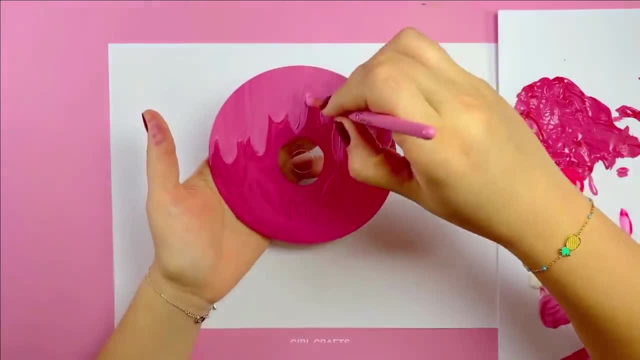 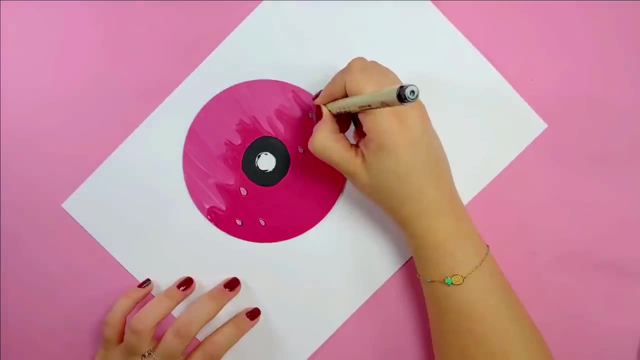 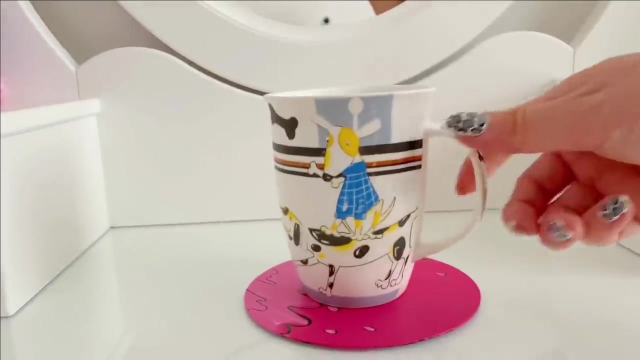 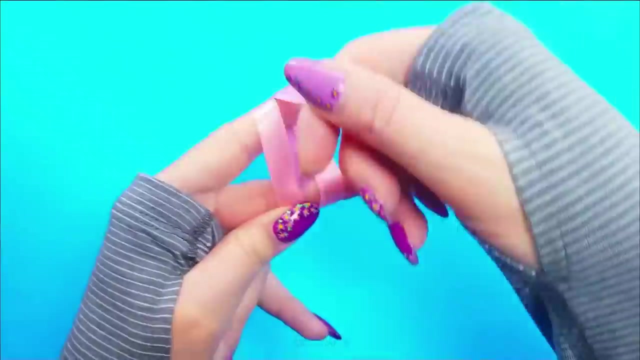 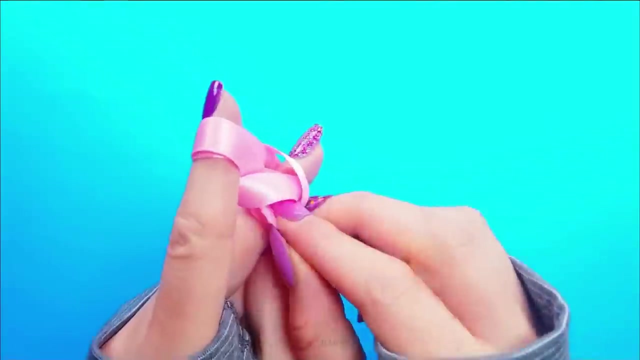 Singing love is everywhere. I got the birds in the air. I got the kids drum heart beat, pounding Breath short of air. What a perfect. what a perfect way To spend the day- just dreaming Way to spend the day just dreaming Way to spend the day just hoping. 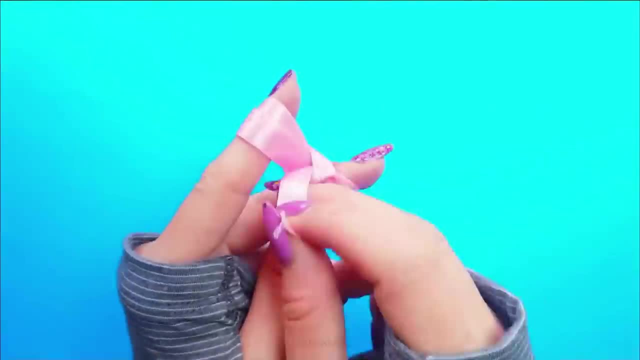 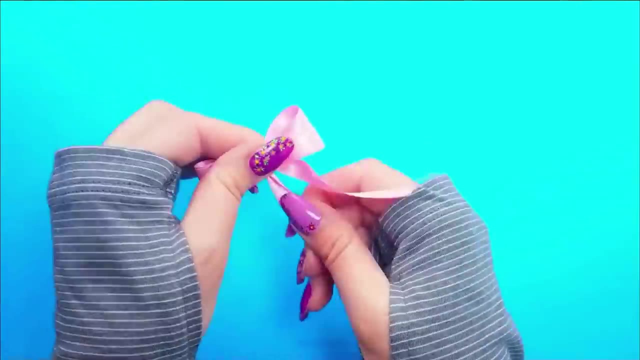 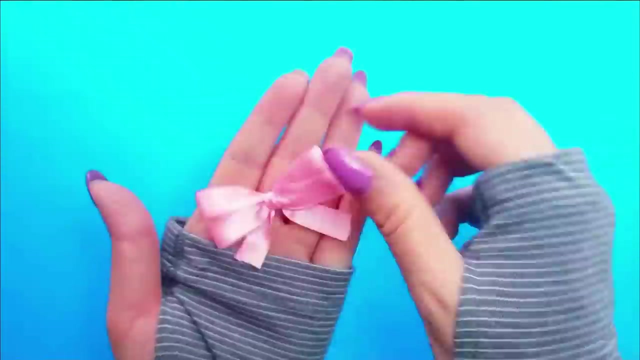 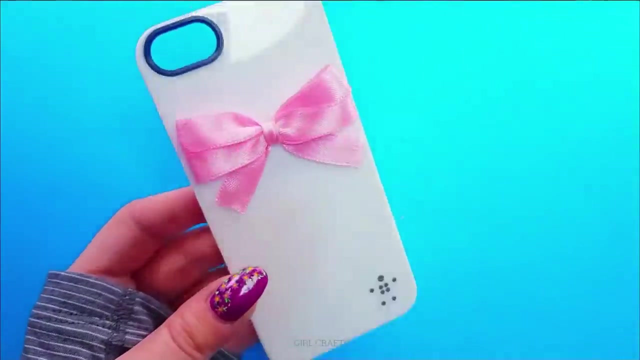 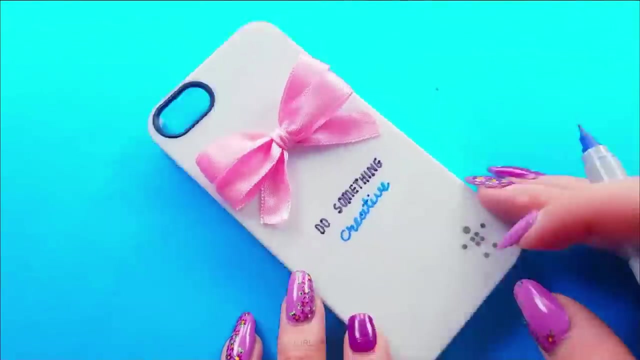 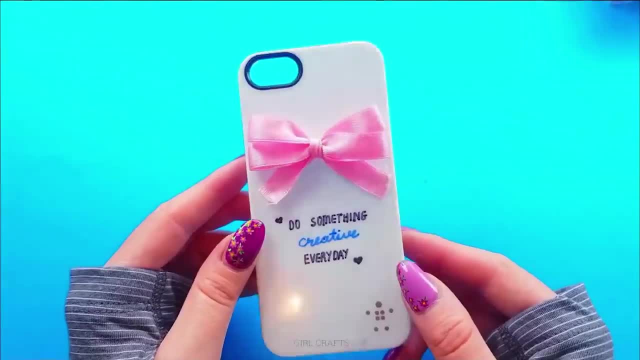 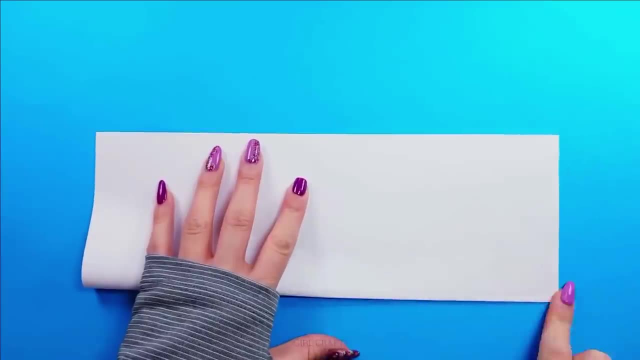 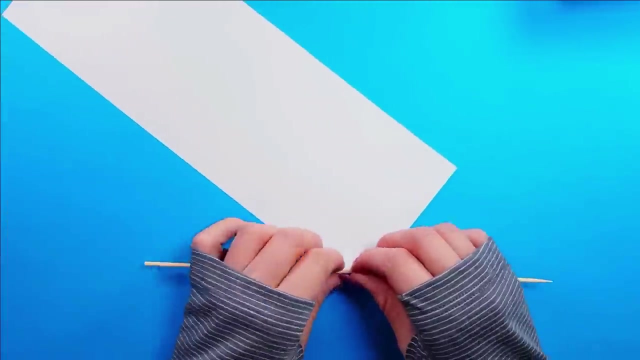 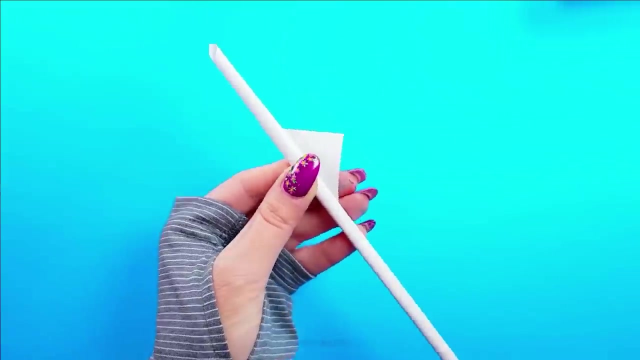 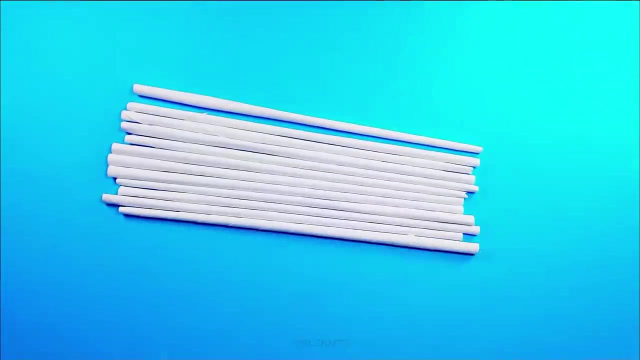 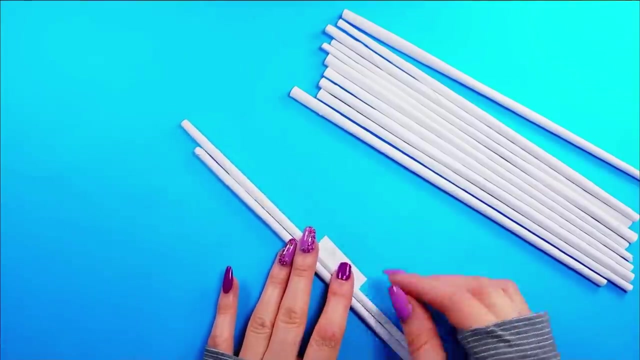 Oh, oh, oh, oh, oh, oh oh. I know we've seen better days. Life is just a game we play. You hold tight to the world. you know The hardest part is letting go. Follow me to the sunshine, Come and see what it feels like. 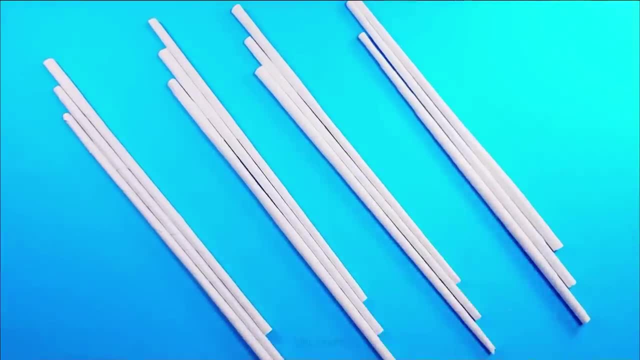 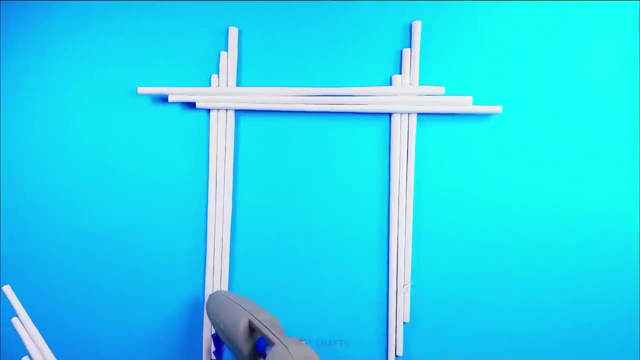 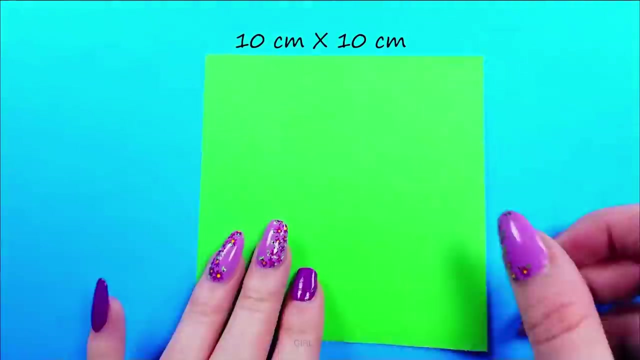 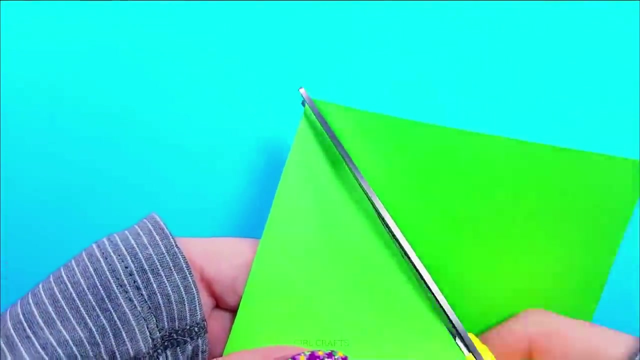 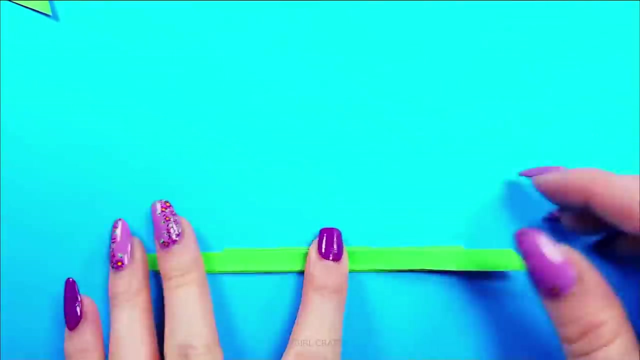 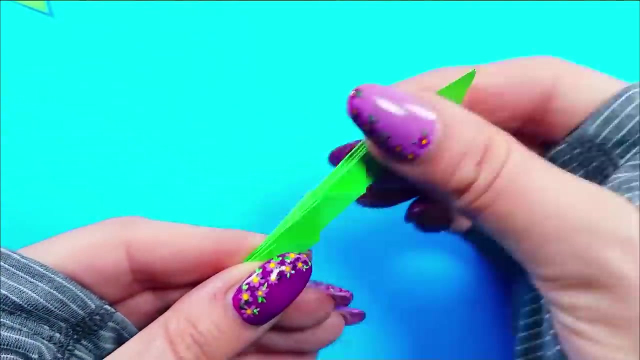 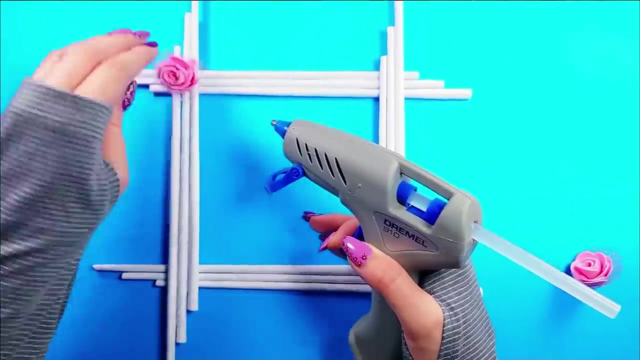 Higher, higher that we climb. I know somewhere that you and I, We could stay wild, wild, We could stay wild. wild, We could stay wild, We could stay wild. Wake up, don't miss your chance. Take off, get lost again. Young enough to change our love, Laugh it off when times get tough. 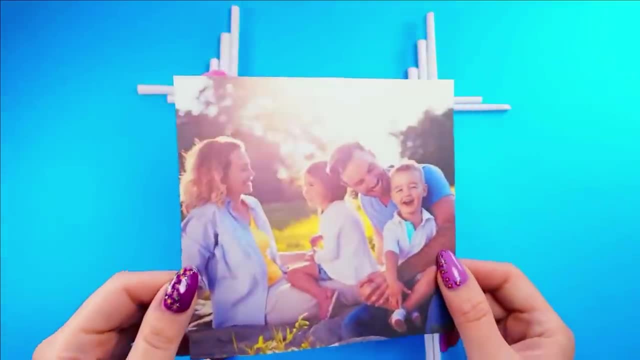 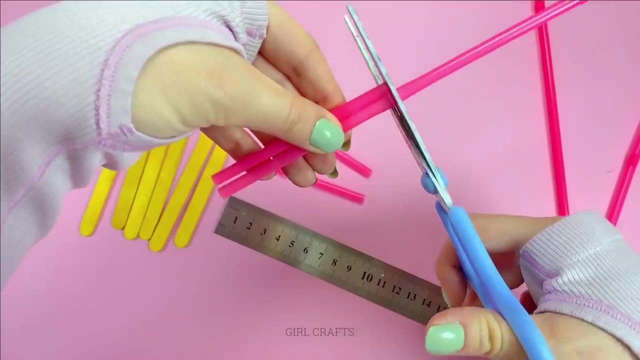 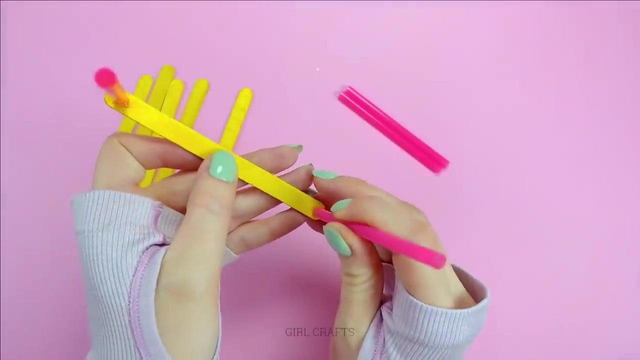 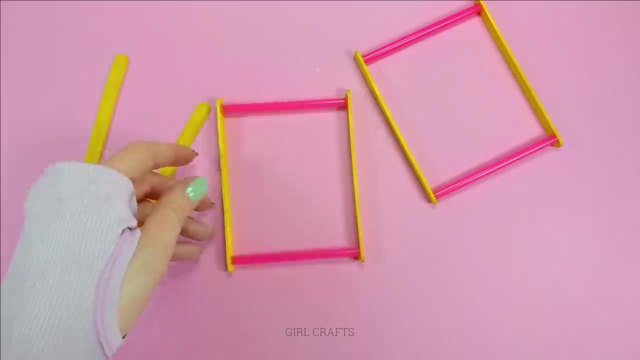 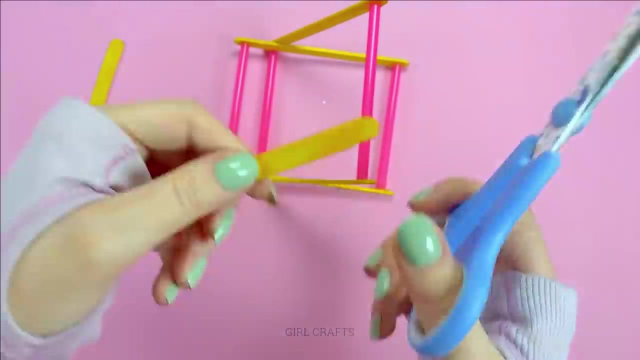 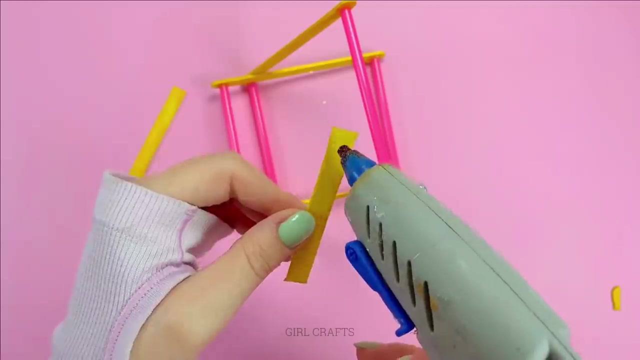 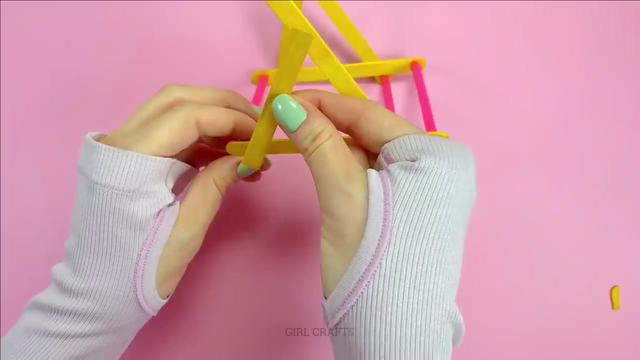 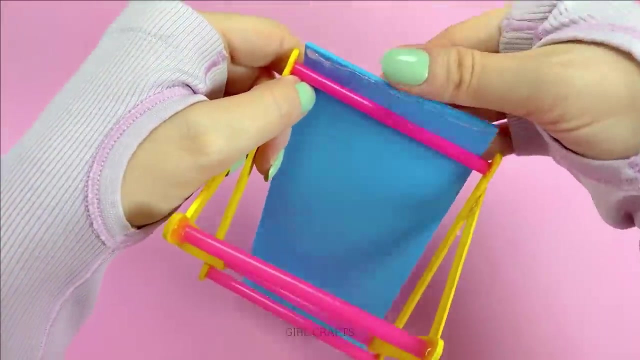 Follow me to the sunshine, Come and see what it feels like Higher, higher, that we climb. I know somewhere that you and I, We could stay wild, wild, We could stay wild, wild, We could stay wild, We could stay wild, Away where we go, Away where we go. 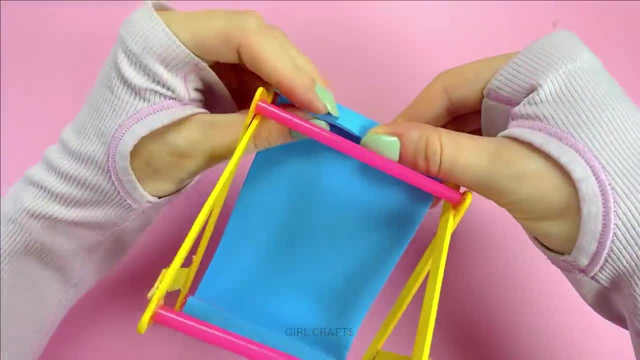 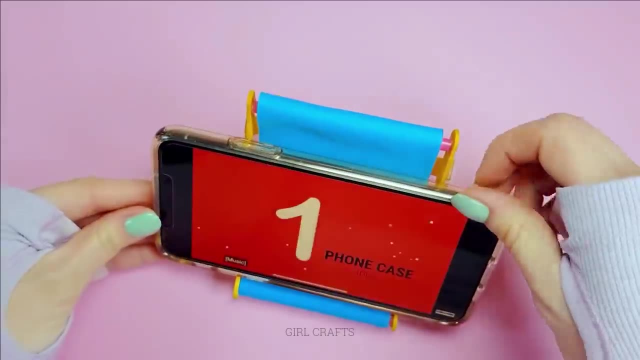 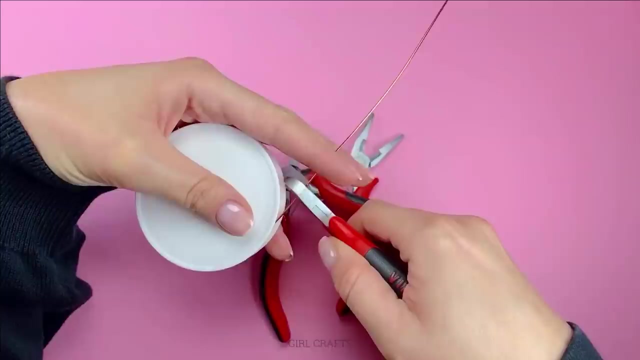 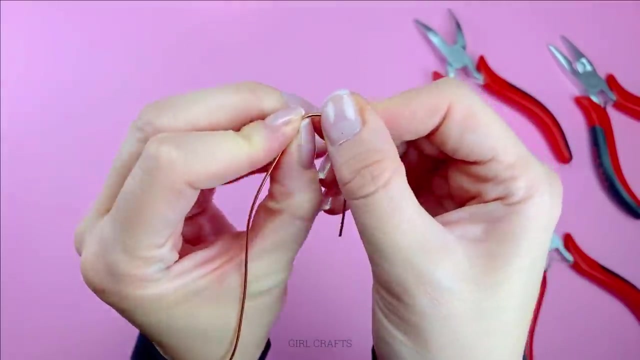 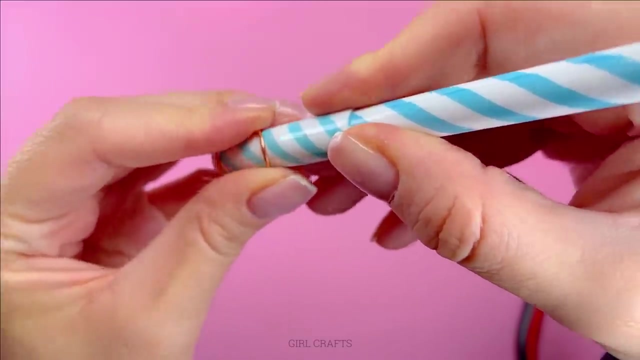 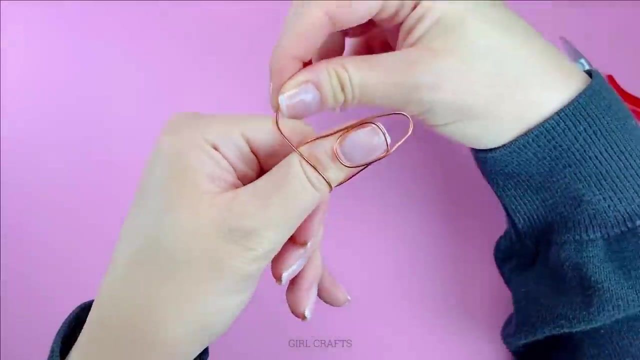 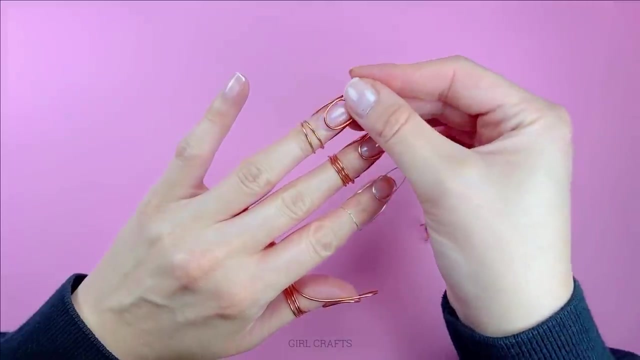 Don't think twice. Away where we go, away, where we go, Don't think twice. Follow me to the sunshine. Come and see what it feels like. Higher, higher did we climb? I know somewhere that you and I, We could stay wild. We could stay wild, We could stay wild. 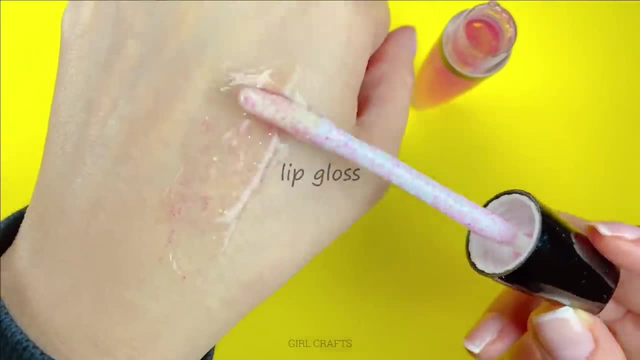 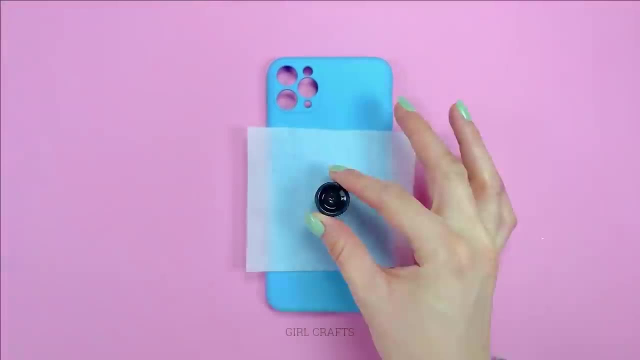 Ooh, no, no, let's slow down the speed. We got time. time time. Oh, you get to where you need to be: Good time, time time. Oh, no, not me, I'm in no hurry, I'm a slow and steady man. 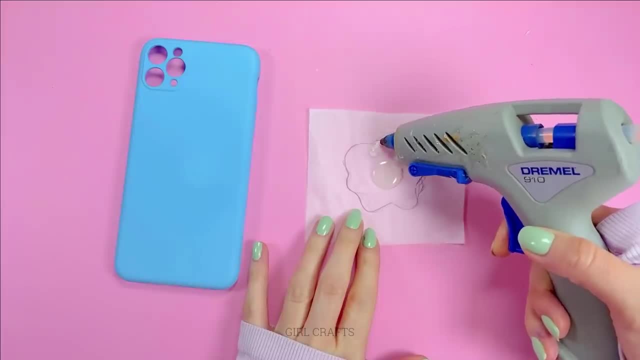 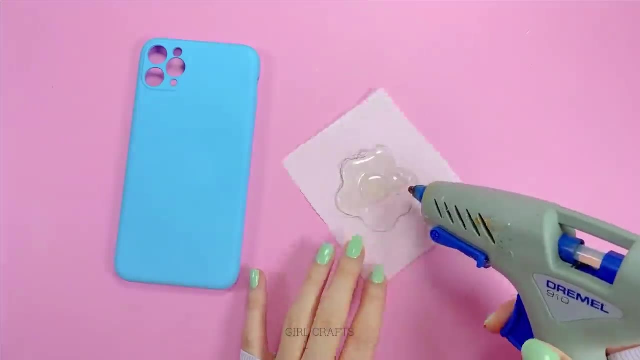 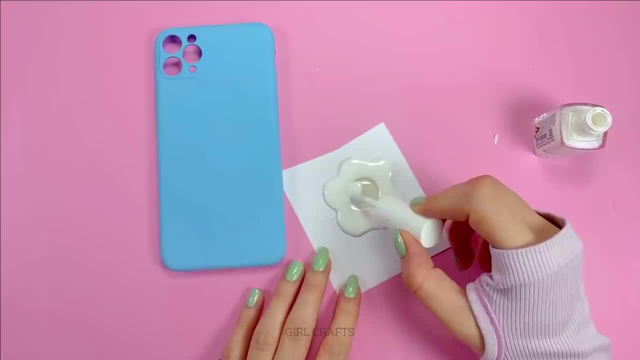 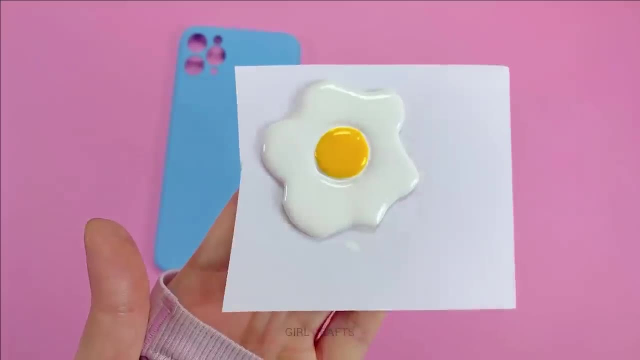 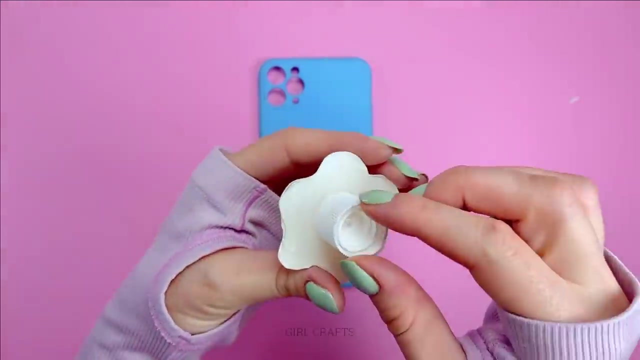 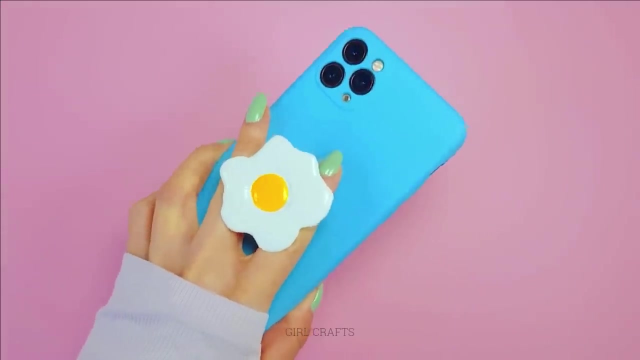 Ooh, if you wanna make something last, It takes time, time, time Overheat and you'll burn out fast In no time time time, Oh, no, not me, I'm in no hurry, I'm a slow and steady ride. Oh, don't you see, it's still so early. 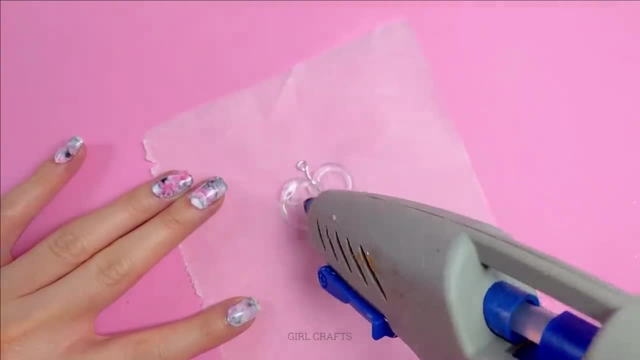 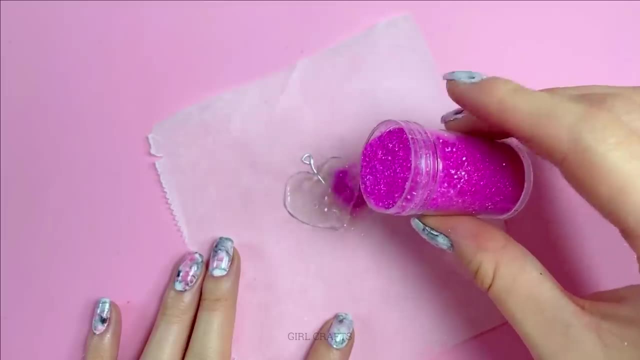 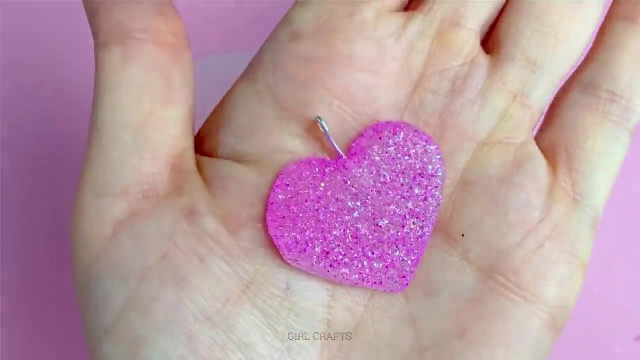 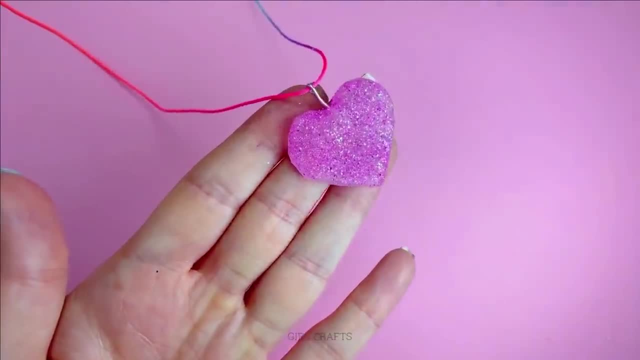 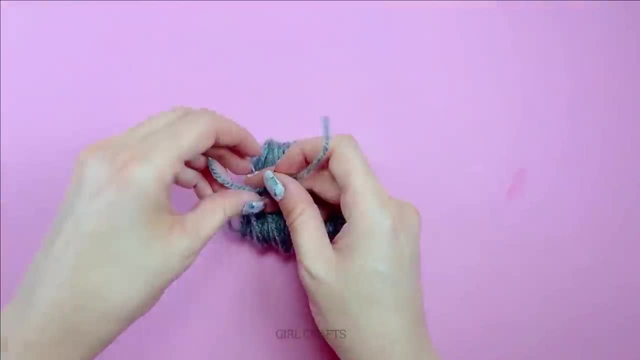 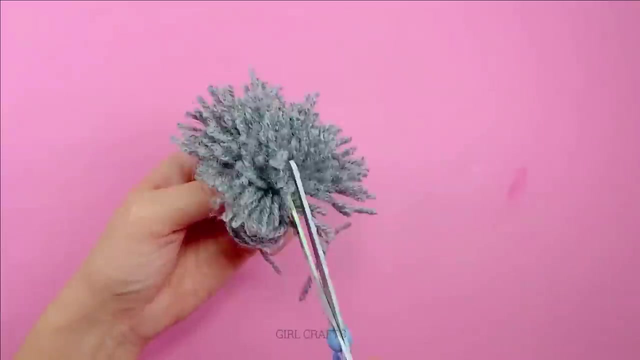 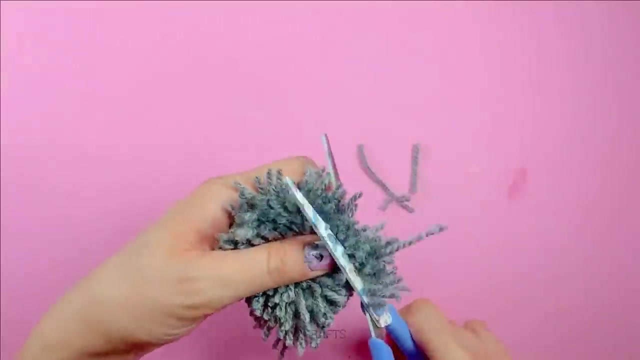 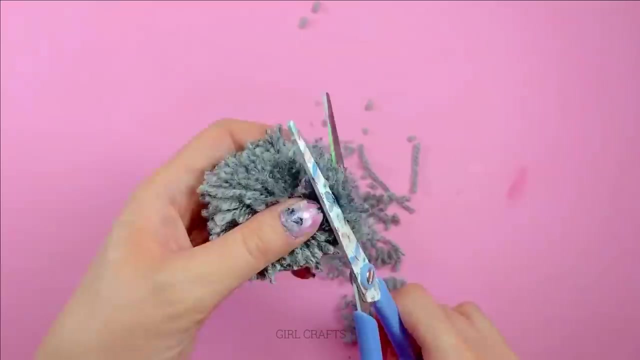 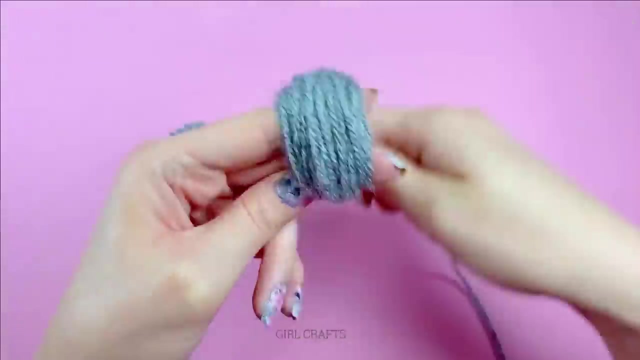 Burn. ooh yeah, ooh yeah. Turn the heat down and cool it. I'm not gonna be a flash in the pan Or a flavor of the week. No, no, no, no, no, no, no. Not gonna be a one-night stand. 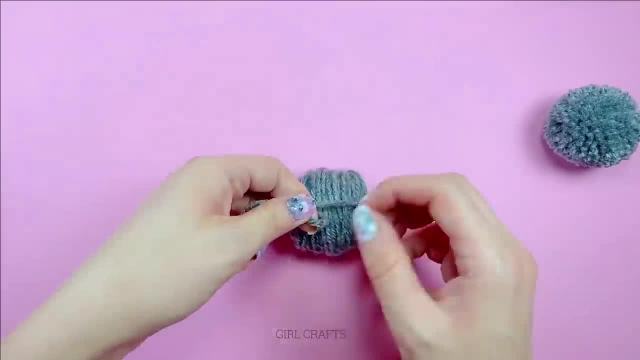 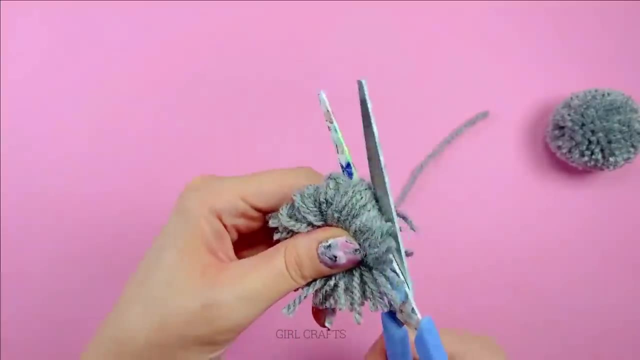 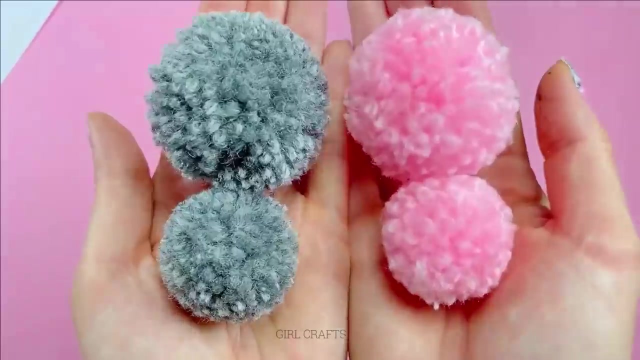 I wanna be around the long, long line. Ooh yeah, ooh yeah, Turn the heat down and cool it. Ooh yeah, ooh yeah, Turn the heat down and cool it. Slow, no, no, slow, no, no. 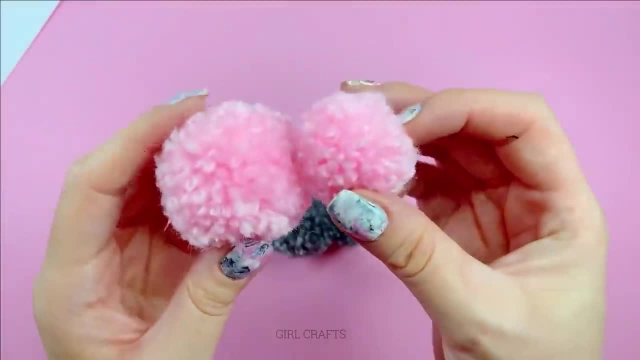 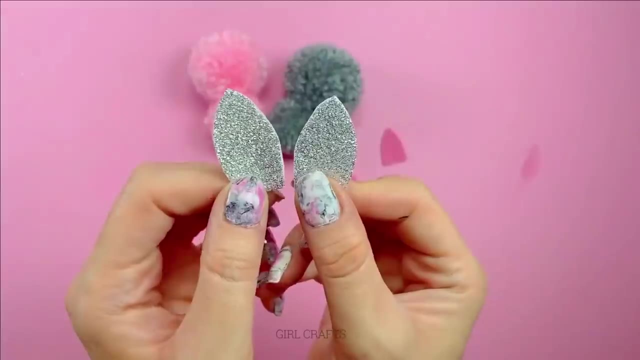 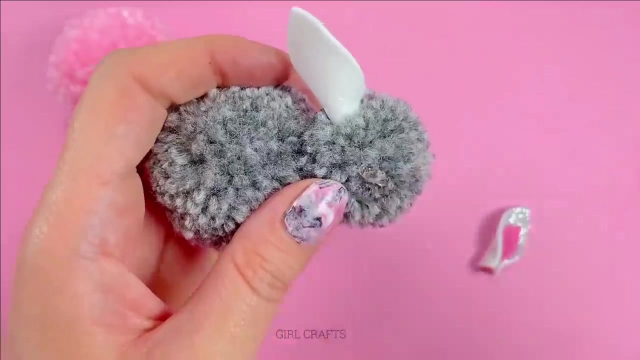 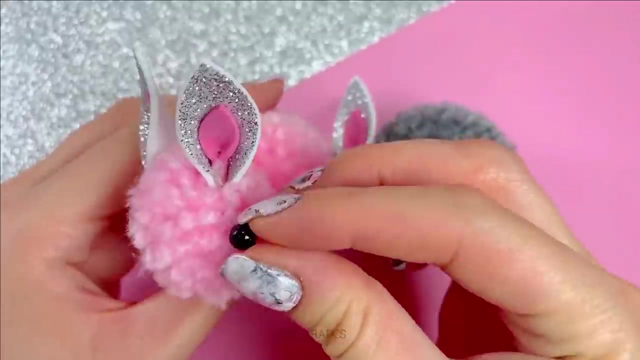 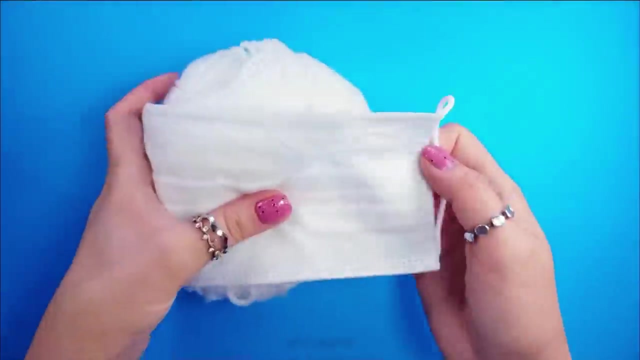 Slow. no, no, no, no, no, no. Burn. ooh yeah, ooh yeah. Turn the heat down and cool it. I'm talking about something they can't capture on a camera. I'm talking about your life, babe. 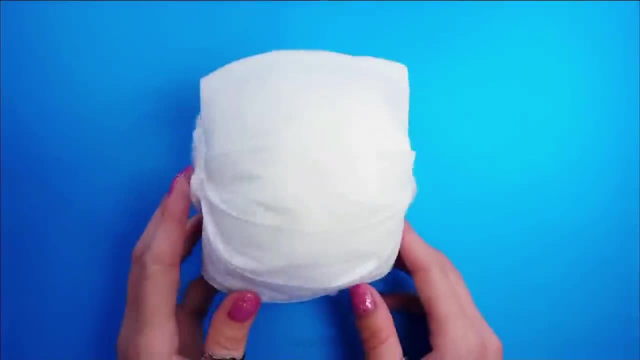 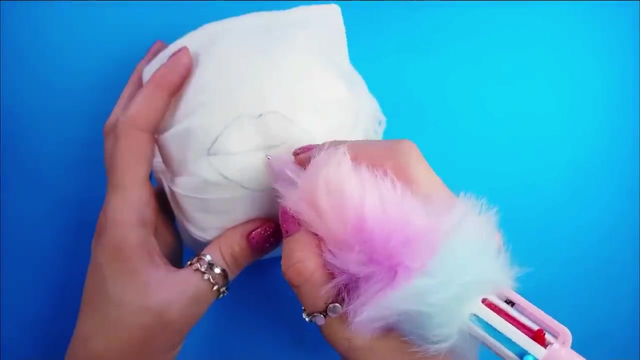 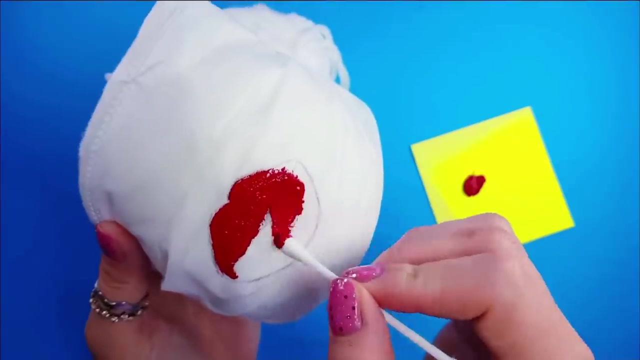 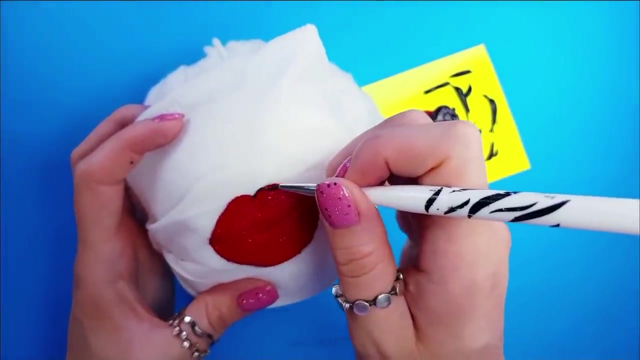 Your character. You're driving and they cut you off. The stranger spills your coffee cup And it's hot. babe, Tell me what's your heart. say, Maybe we got it all wrong. It ain't about what you like, Yeah, it's about what you're made of. 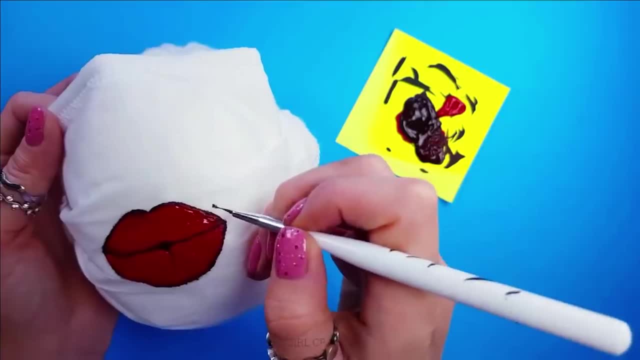 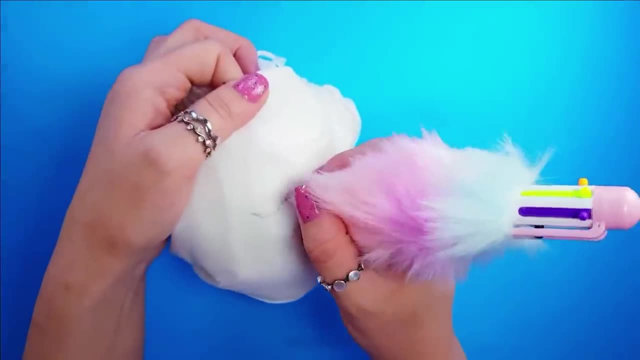 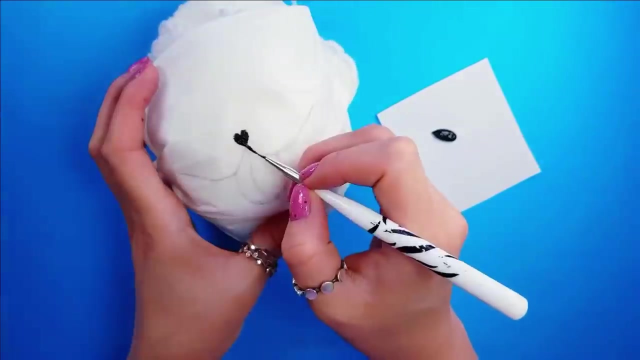 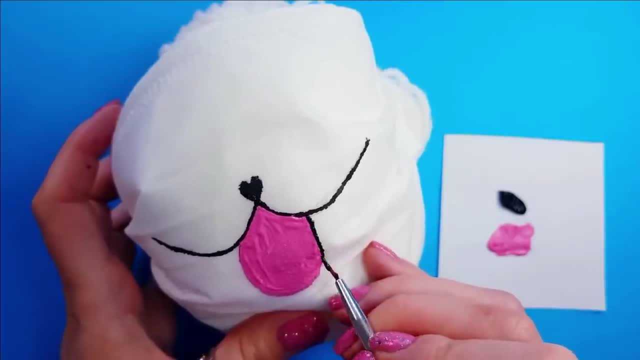 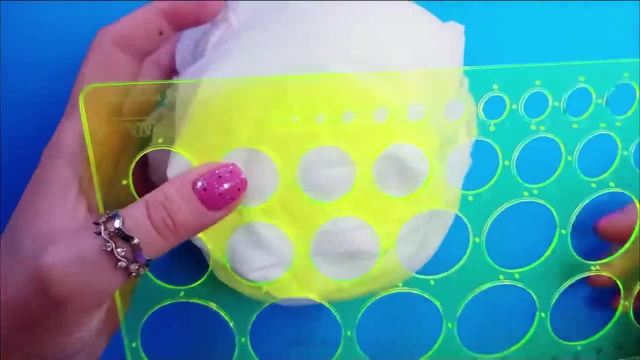 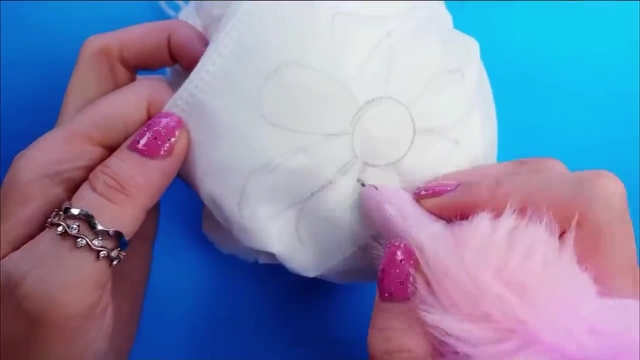 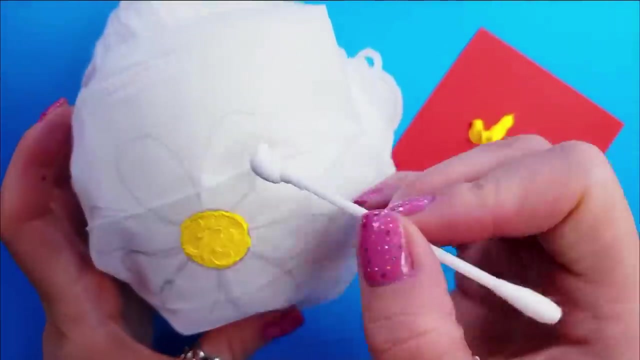 Humble and strong, Secure in my bones. I'm talking about even when no one. But it seems I'm trying to be the best of me And it's hot, babe, And I've had a rough day. Maybe we got it all wrong. It ain't about what you like. 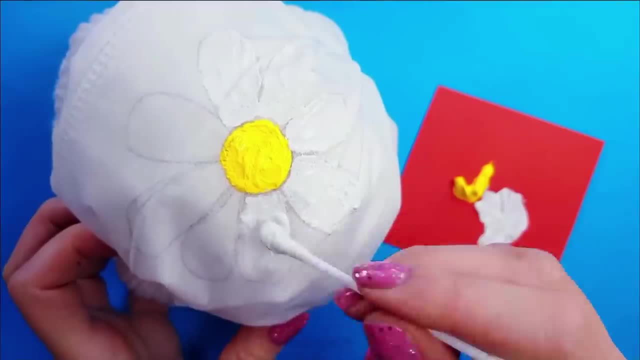 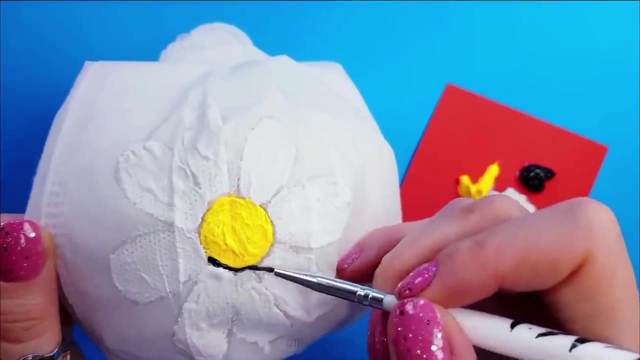 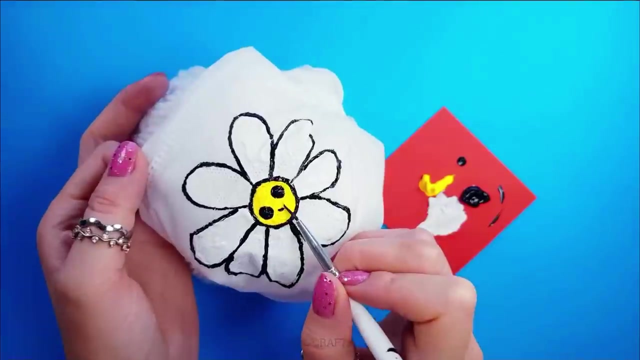 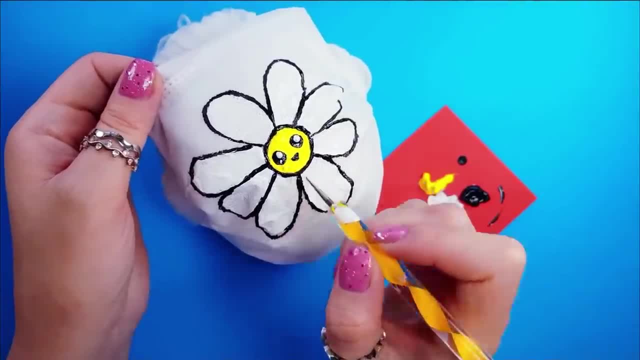 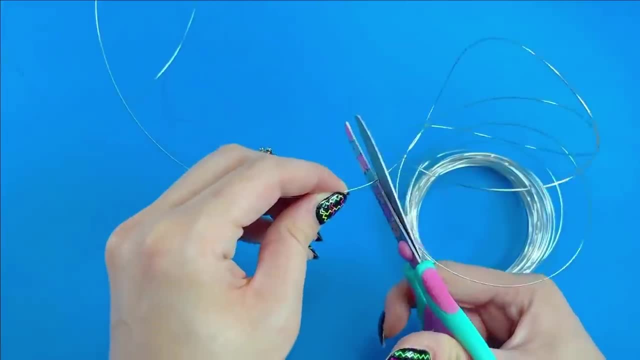 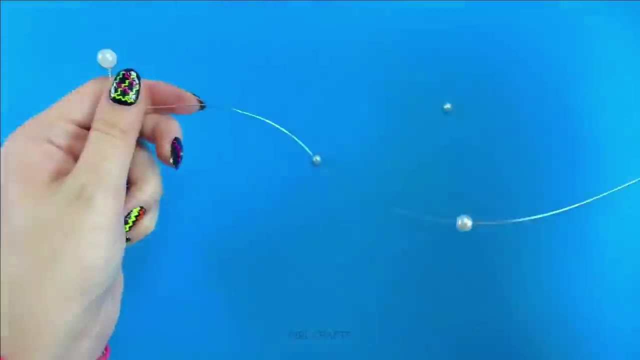 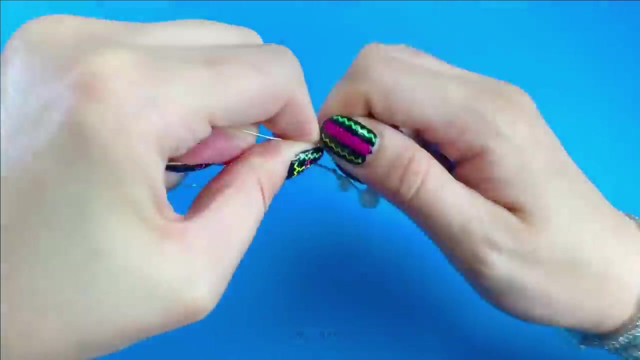 It's in your nature, It's how he creates you, And I ain't no preacher, But I'll tell you like it is. It's in your nature, It's how he creates you, And I ain't no preacher, But I'll tell you like it is And it's how he creates you. 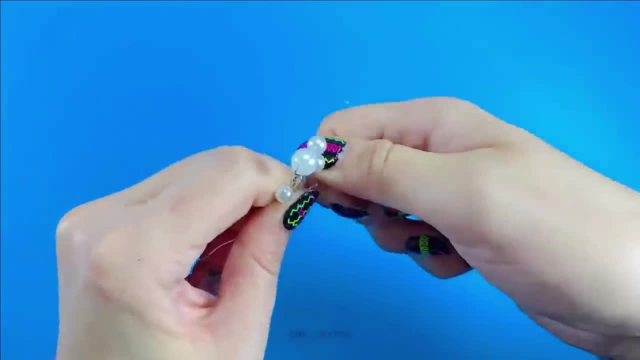 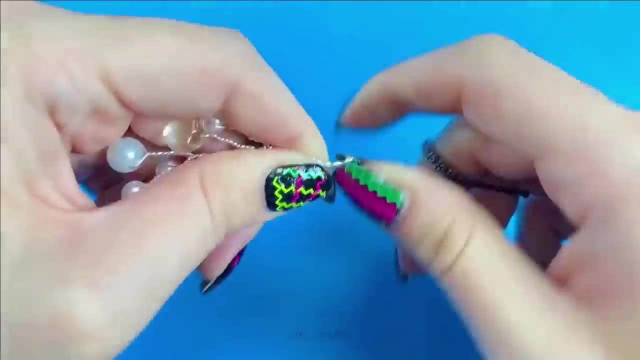 It's in your nature, It's how he creates you. But it's hot, babe, And I was hoping. Ooh, what disgrace. I said this ain't how it should feel Her smile, what she puts on Her floats. This ain't about who she is. 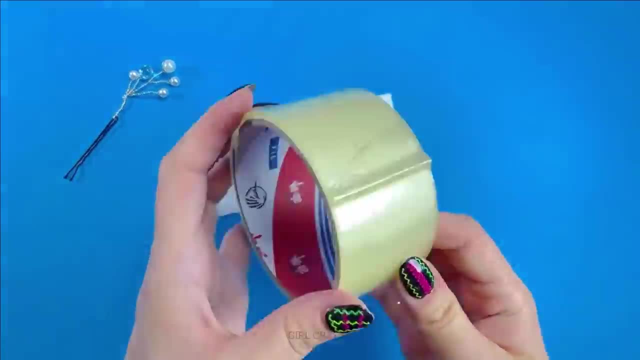 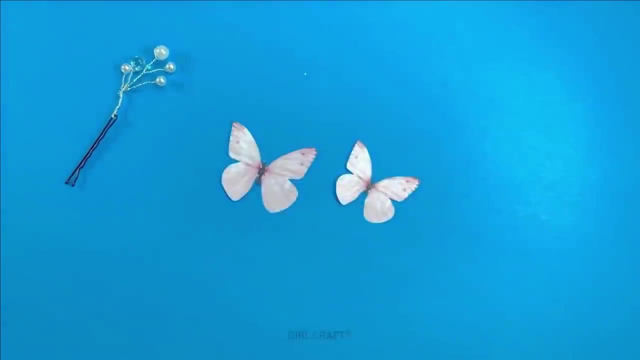 This ain't about where she goes, And I ain't no metallurgist. I'm talking about your love. I'm talking about your character. I'm talking about your character. I'm talking about you. I ain't no preacher. This ain't about who you like. It's in your nature. 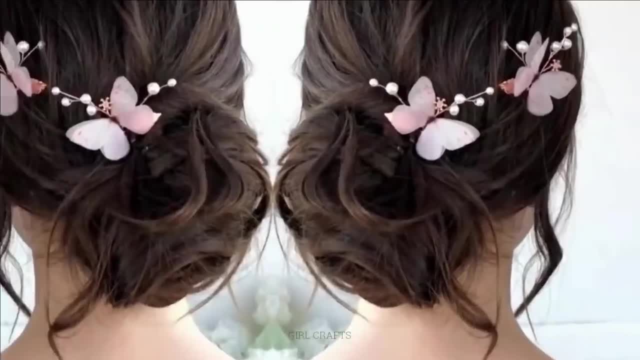 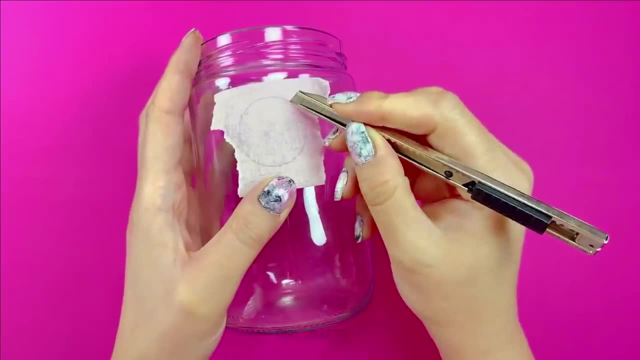 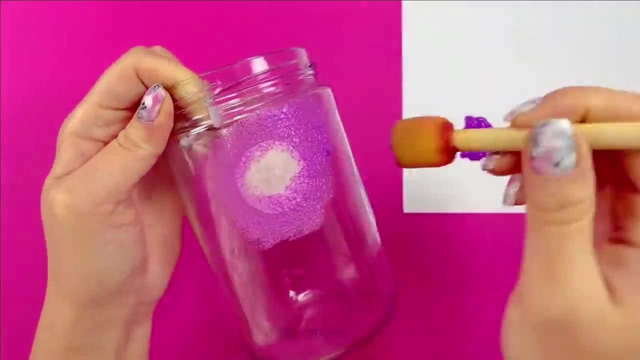 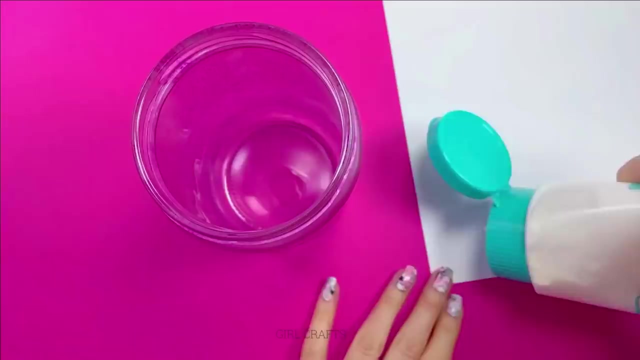 It's how he creates you. Well, I'll sing, sing like a bird, Singing your song all day till it gets dark, And then speak, speak like an owl, Saying who, who, who is that in my heart? Well, it's you, baby, it's true. 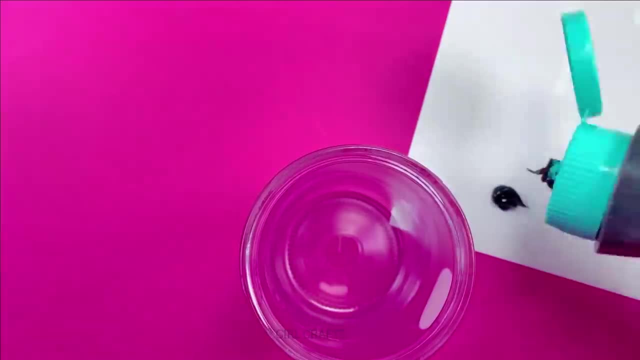 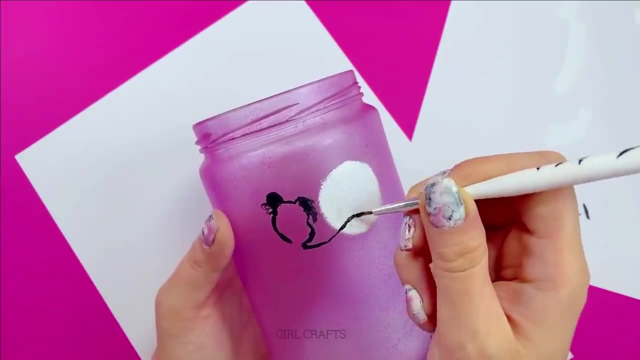 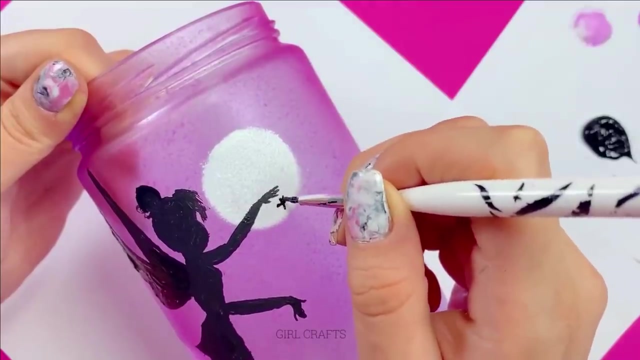 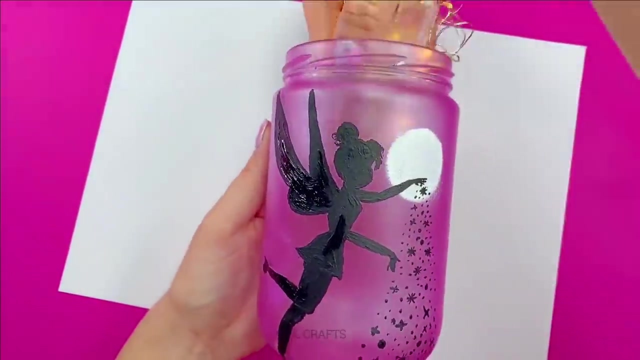 All of my life I've waited for you. I'm taking flight and sailing the world, But you love me too. Oh baby, when you walk into the room, Everybody turns to staring at you As they all pick their jaws off the floor. It's plain to see, girl, it's you they adore. 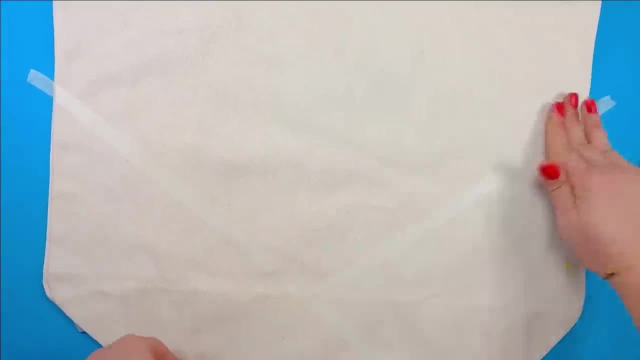 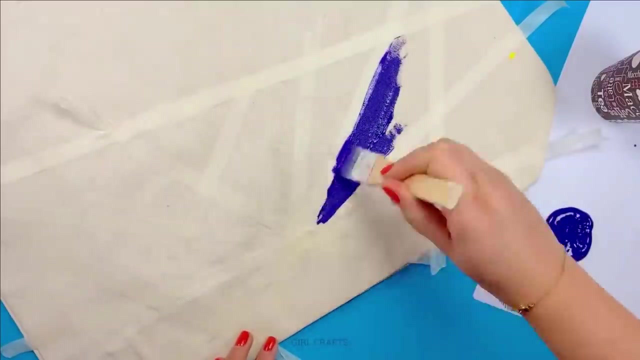 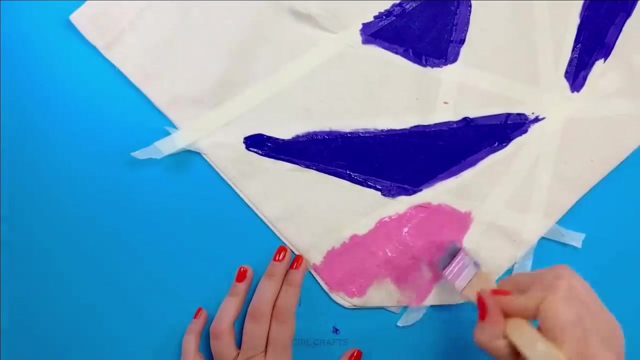 And I can't help but sing, sing, Oh, Oh. Well, I'll sing, sing like a bird, Singing your song all day till it gets dark, And then speak, speak like an owl, Saying who, who, who is that in my heart? Well, it's you, baby, it's true. 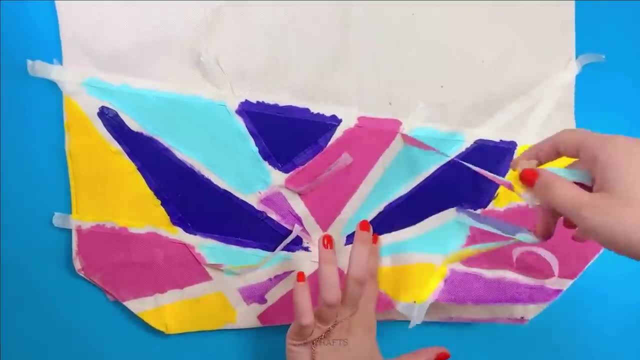 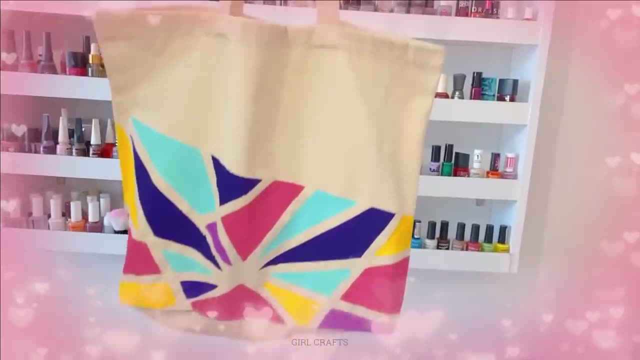 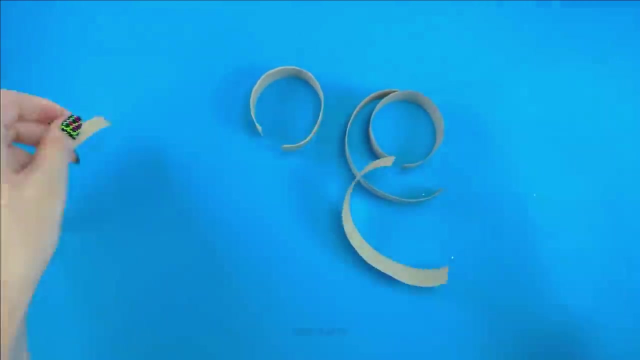 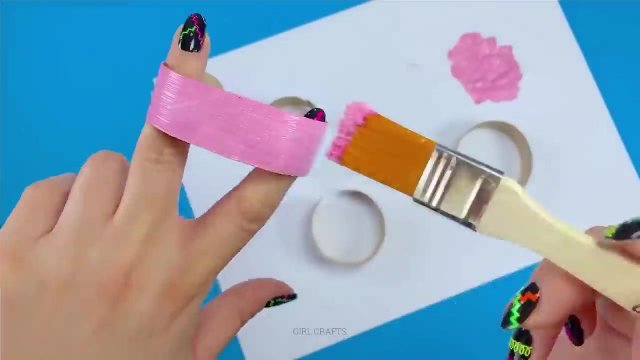 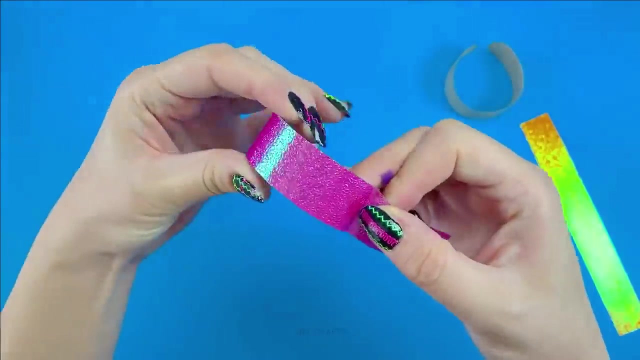 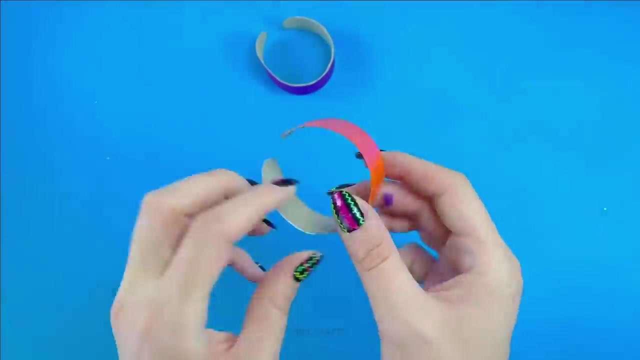 All of my life I've waited for you. I'm taking flight and sailing the world, But you love me too. Oh baby, when you're walking by my side, Everybody turns as we pass by And you've got those angel eyes And you flash that starry smile. 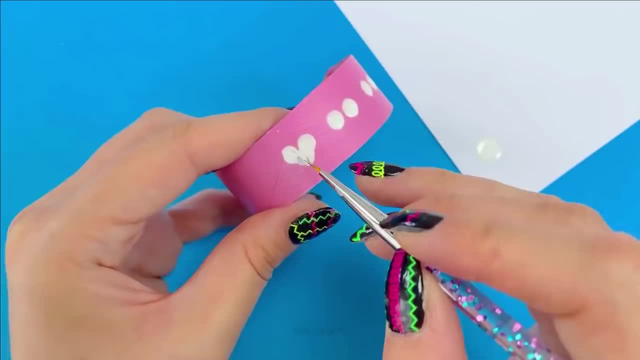 And I think this is the end of the world. And I think this is the end of the world, And I think this is what flying feels like. Oh whoa, And I'll sing, sing like a bird, Singing your song all day, till it gets dark. 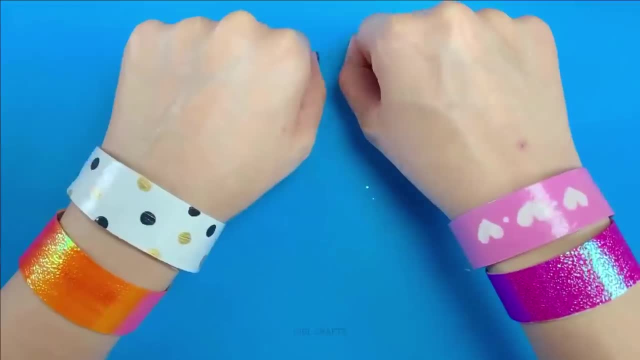 And then speak, speak like an owl, Saying who, who. who is that in my heart? Well, it's you, baby. it's true. All of my life I've waited for you. I'm taking flight and sailing the world, And you love me too. 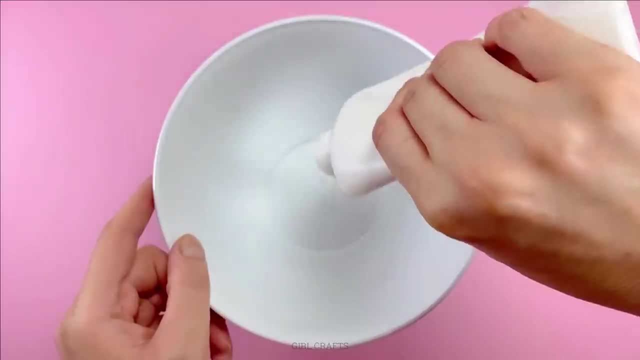 Oh baby, when you walk into the room, Everybody turns to staring at you. As they all pick their jaws off the floor, Everybody turns to staring at you. I'm taking flight and sailing the world, But you love me too. Oh baby, when you're walking by my side. 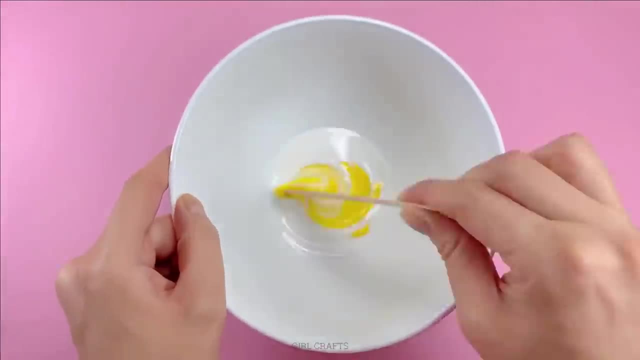 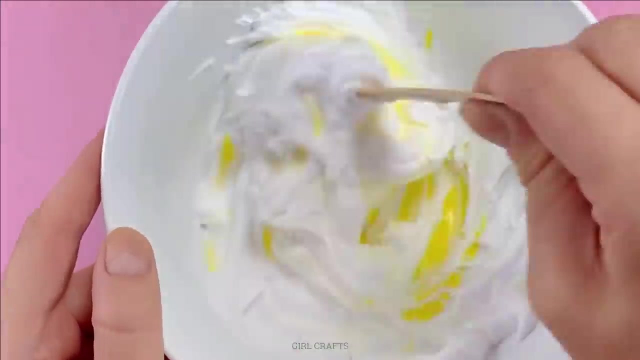 Everybody turns as we pass by my side And you flash that starry smile And I think this is the end of the world. When you're walking by my side, Everybody turns as we pass by my side. Well, it's you, baby, it's true. 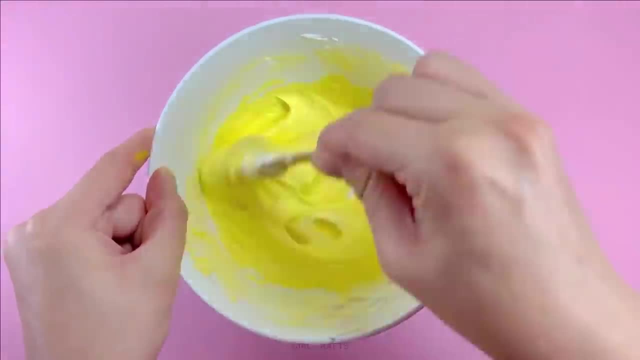 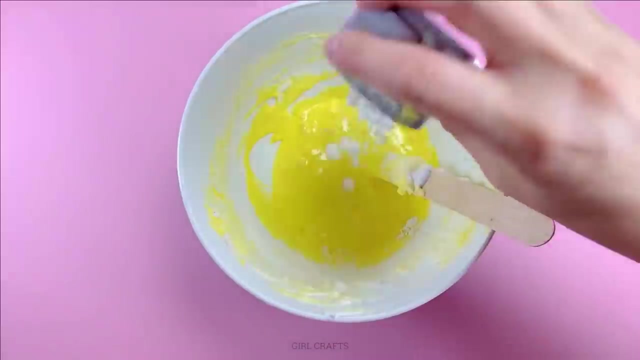 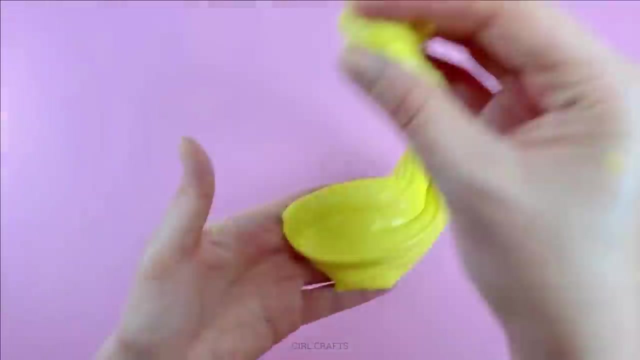 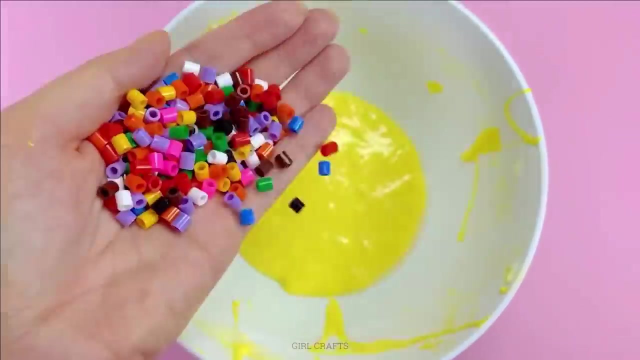 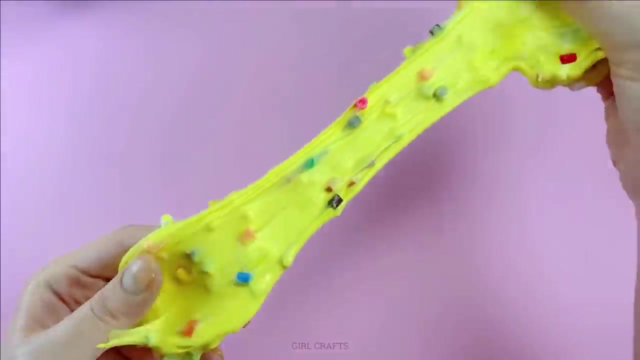 All of my life I've waited for you. I'm taking flight and sailing the world, And you love me too. I'm taking flight and sailing the world. so long that I crumbled. I can't believe that this could come. I worked so hard in the evening. 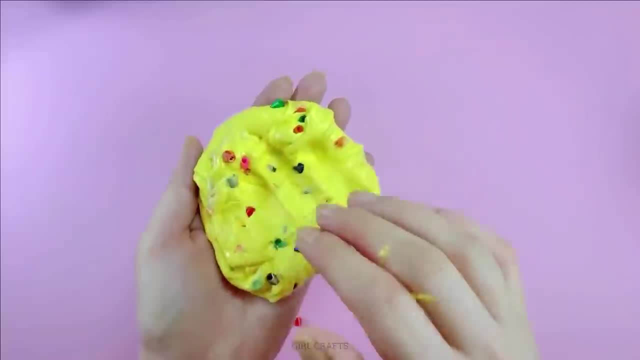 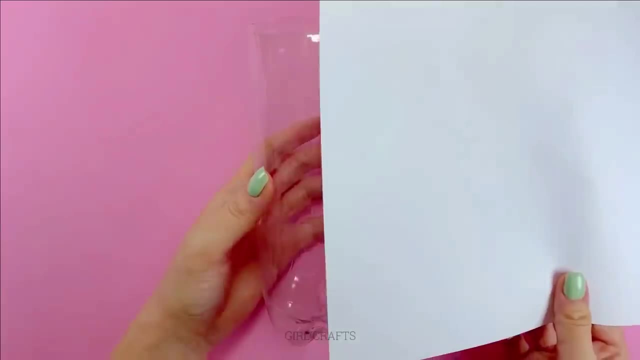 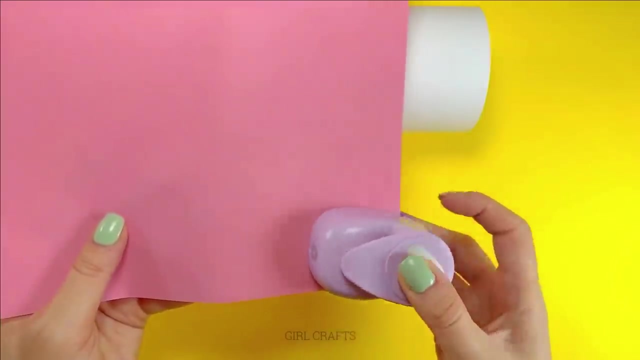 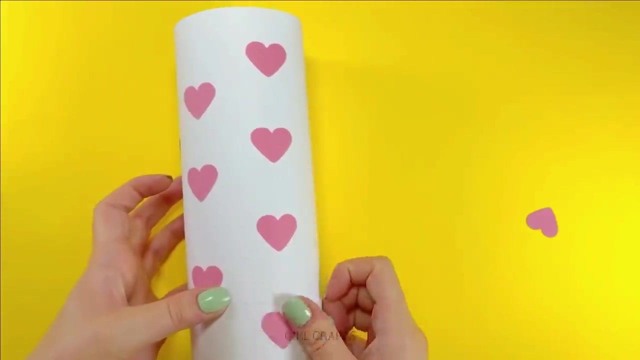 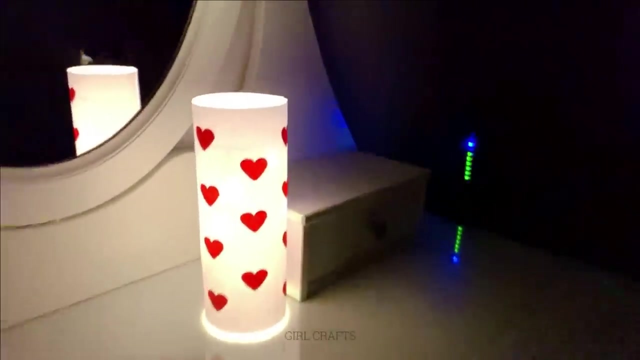 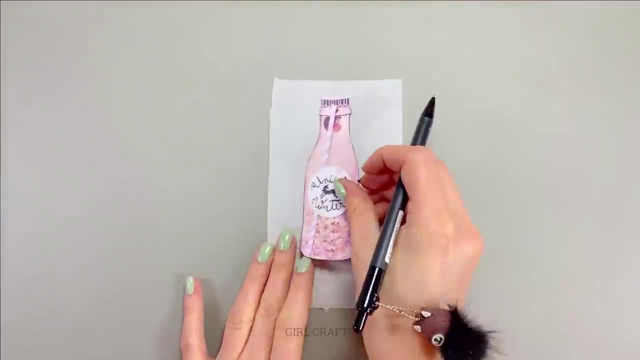 that I stumbled. Oh, I can't believe that this could come. Oh, now, how do I get to sleep at night? and knowing I'm in a recession, suit to be depression? It ain't my fault. Who robbed me? Who robbed me? Why rob me? Give me back my money. My fingers bleed. I can't afford food. 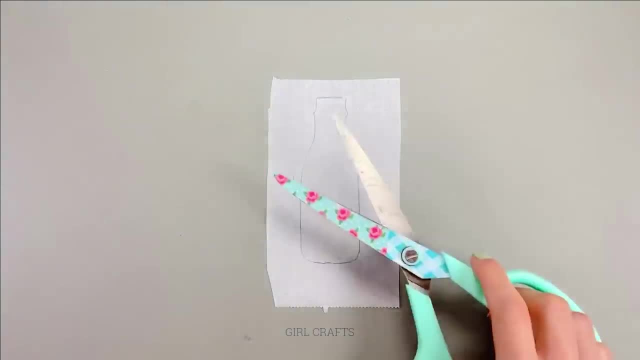 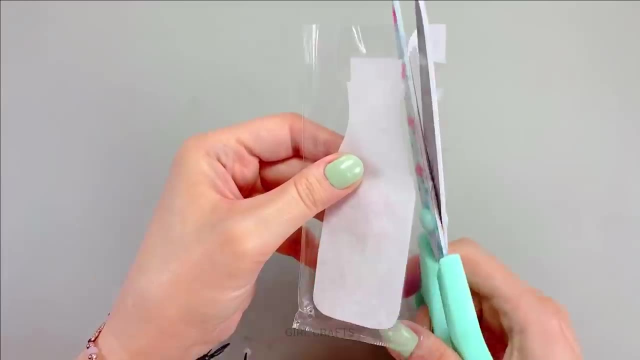 for my family And you. you're out wasting time on vacations, jets and fancy wine. Well, what's a little bit of money to you? Well, how about I sell the fuel? We're sleeping on. we're sleeping on screen. 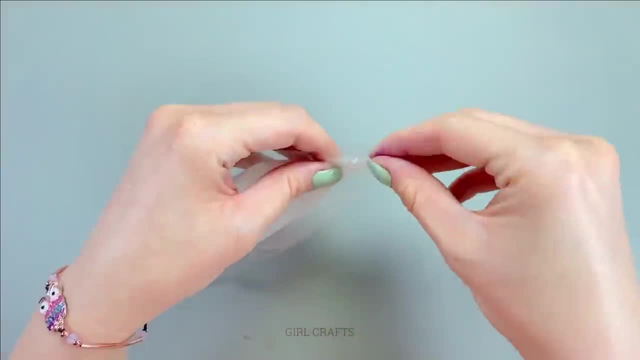 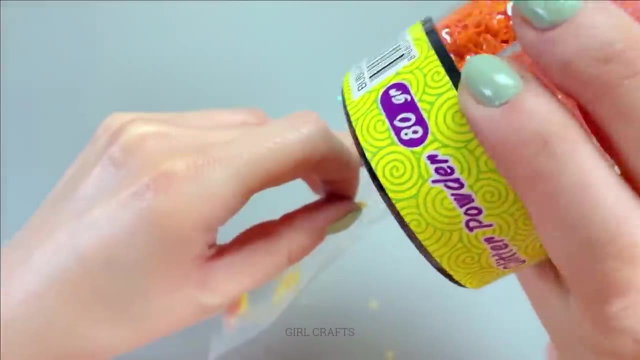 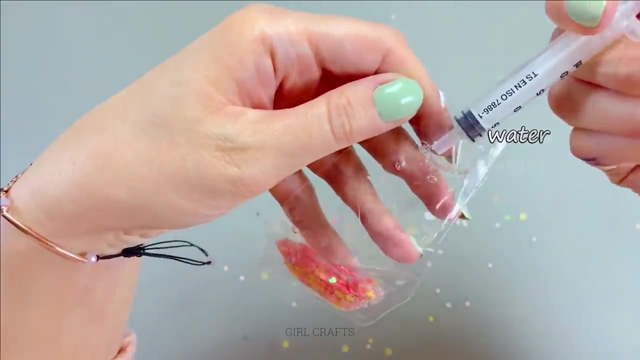 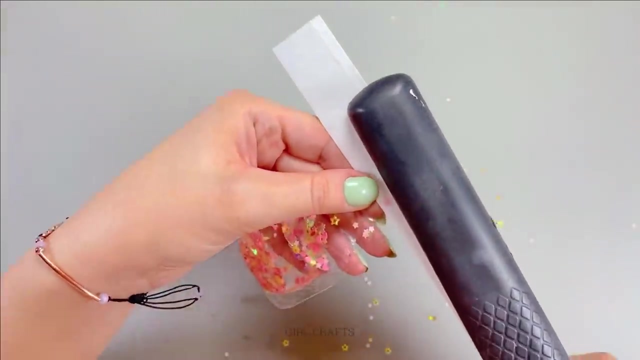 Who do we blame When our leaders are all kingpins? I can't believe that they'd out check to be made. Oh now, how do you get to sleep at night and knowing you stole and squandered the lives of others And then it's all your fault? Who robbed me? Give me back my money, My fingers. 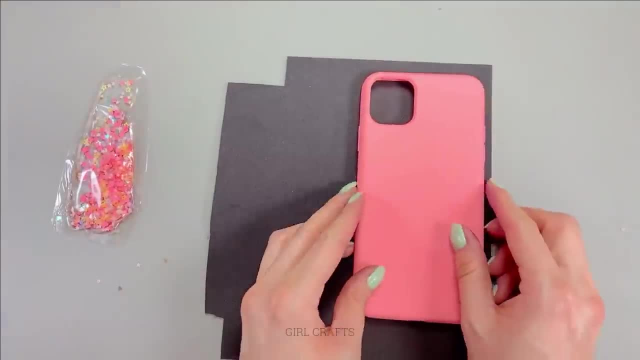 still bleed. I can't afford food for my family. When our leaders are all kingpins, I can't believe they'd out check to be made. What's up with theirellofer-a- Tik-You-Famil y and you? 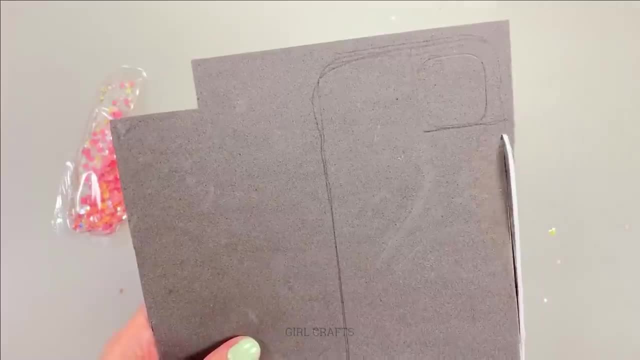 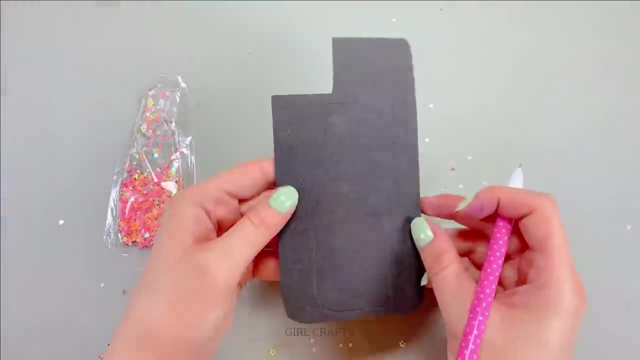 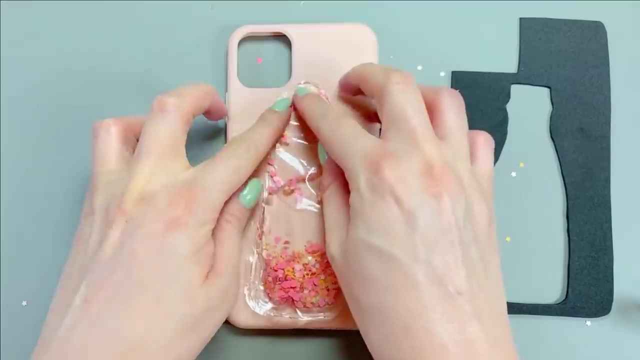 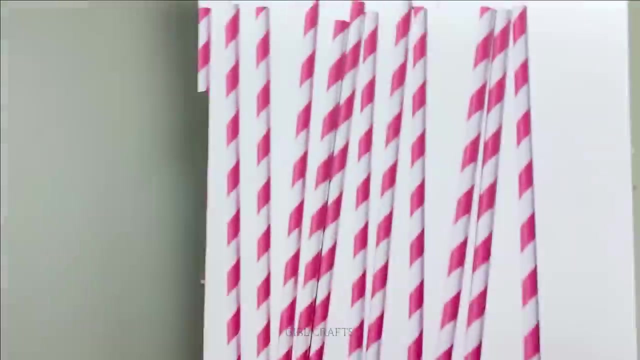 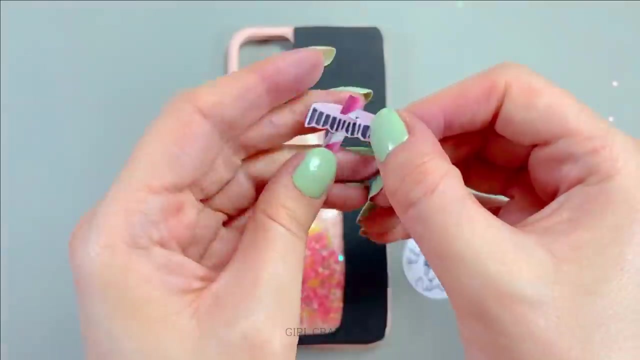 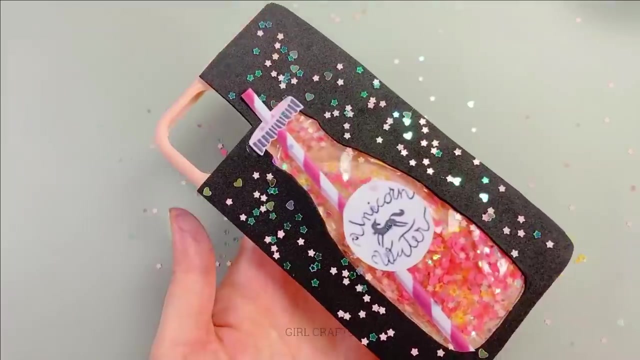 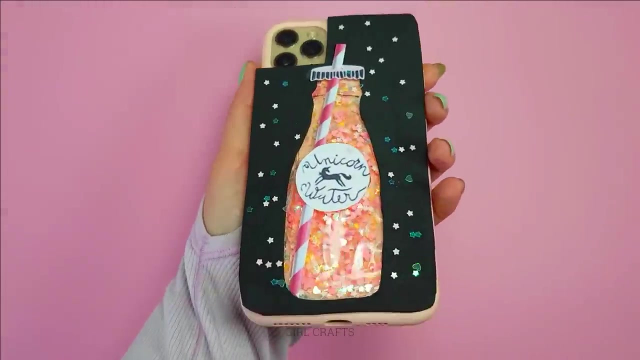 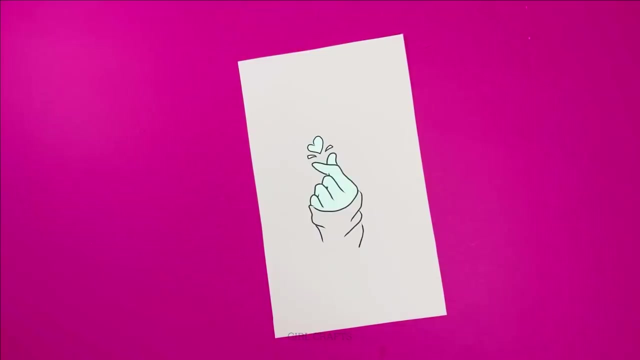 You're all wasting time on vacations, jets. all I got is a grime. Well, what's a little bit of money to you? Well, how about I sell the fuel? We're sleeping on. we're sleeping on screen. We'll be right back. 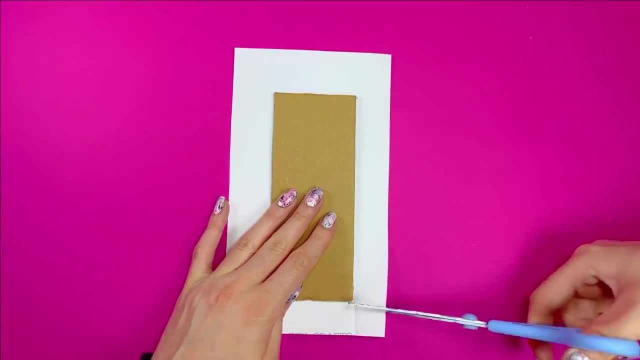 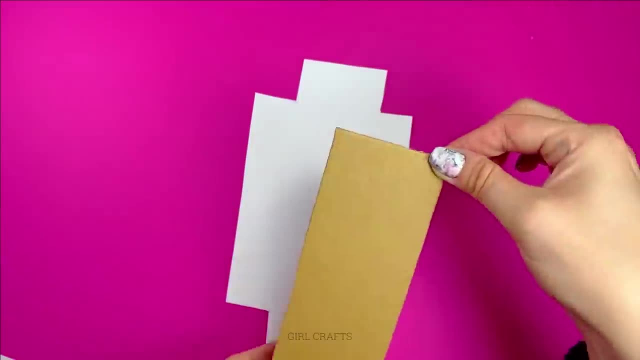 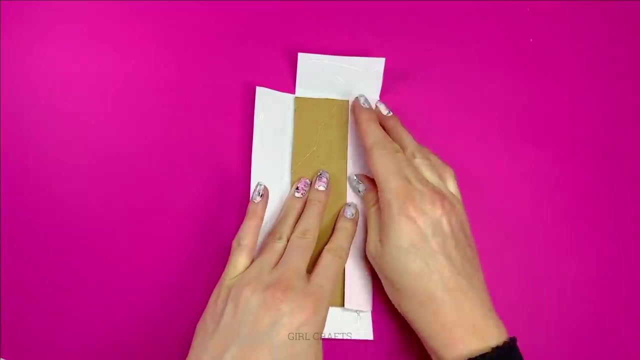 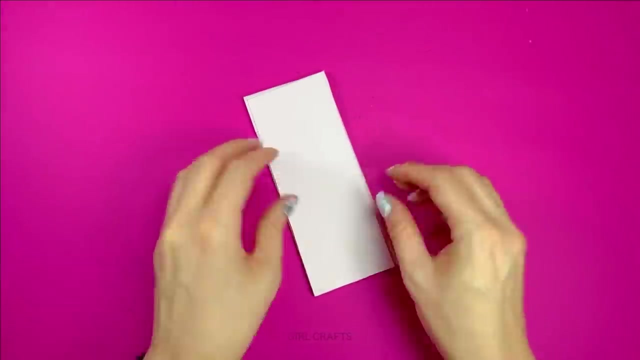 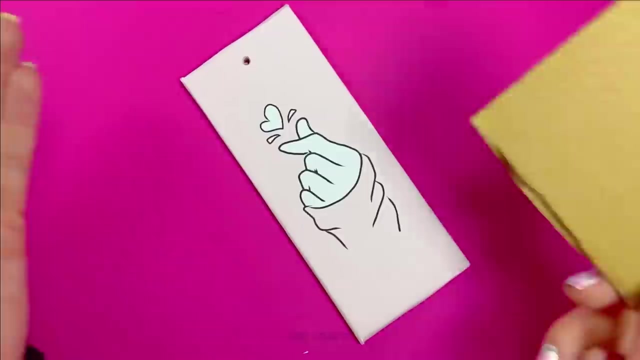 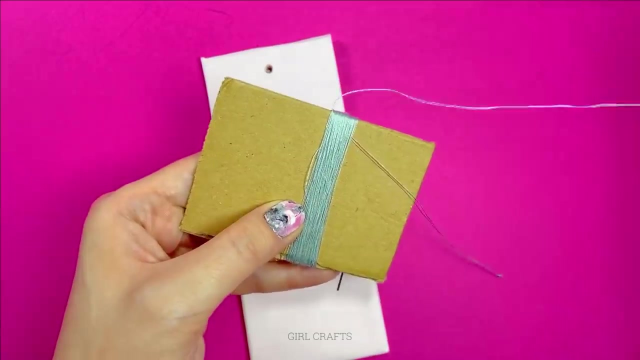 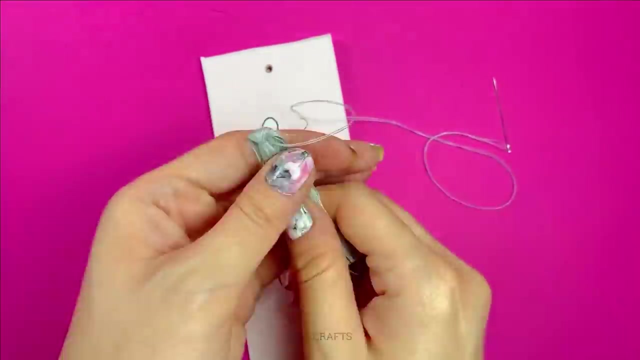 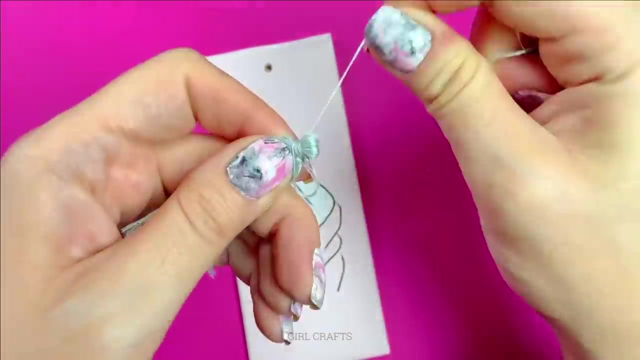 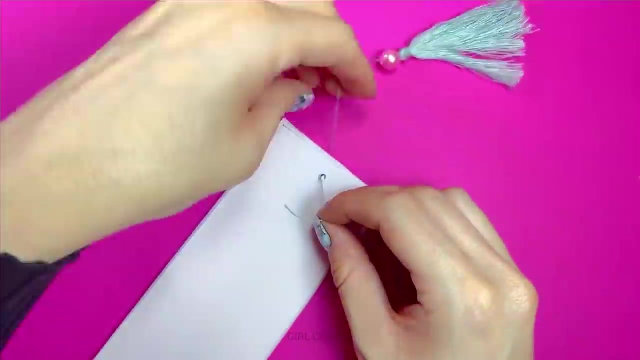 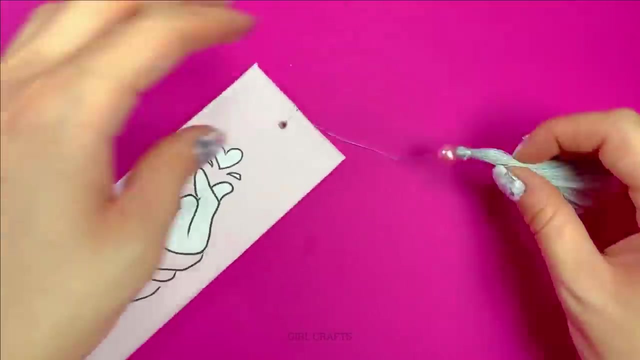 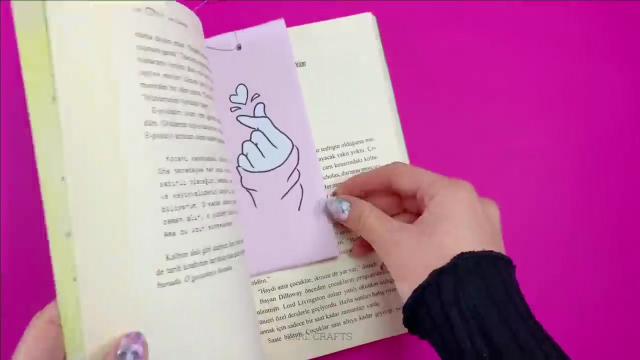 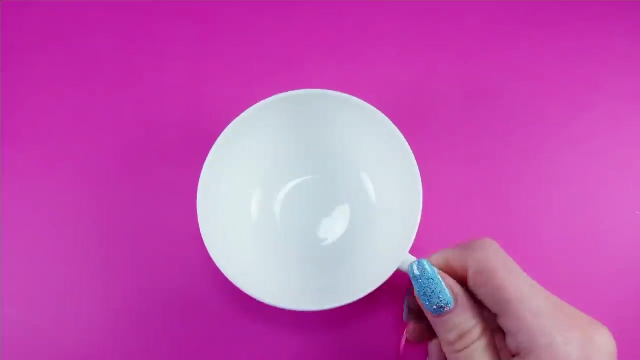 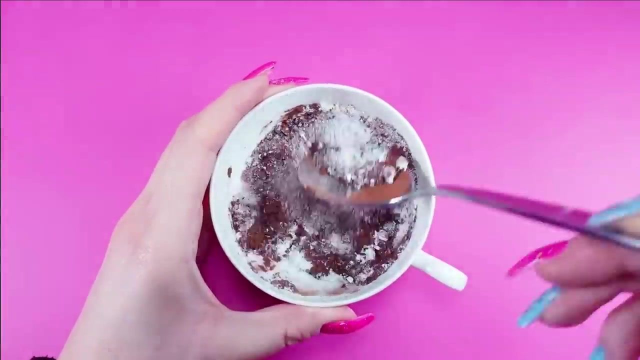 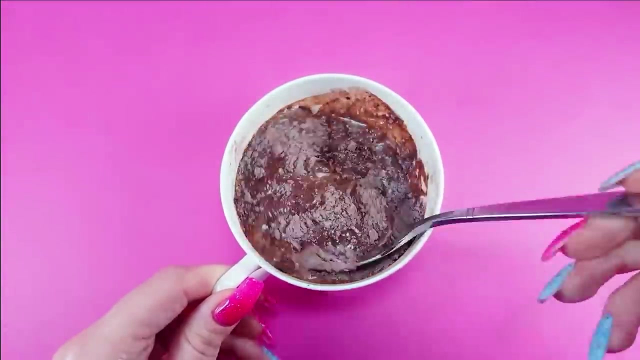 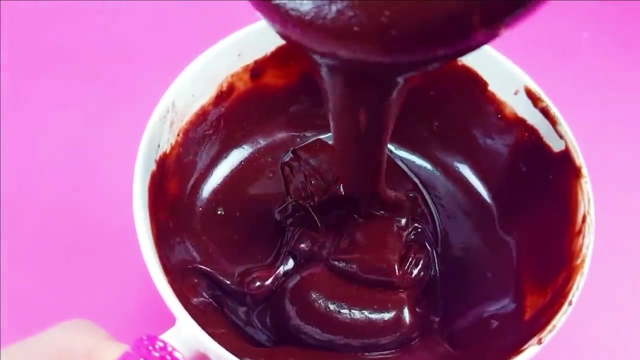 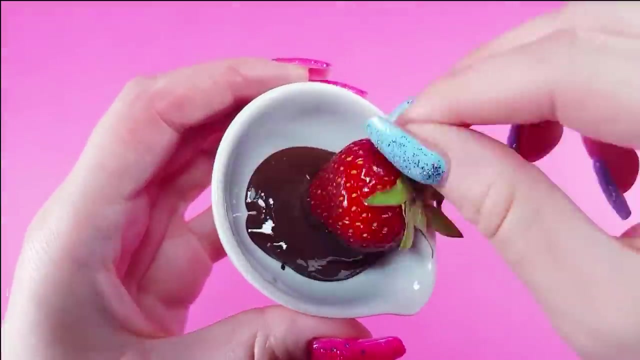 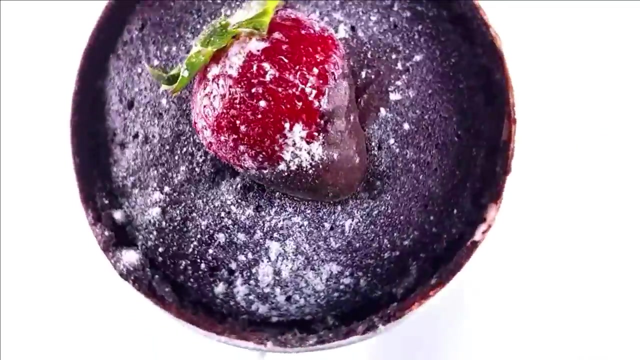 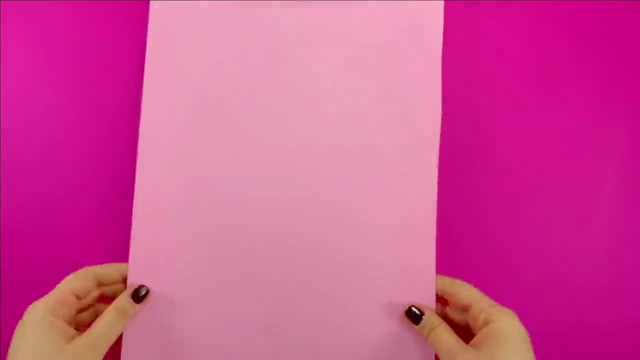 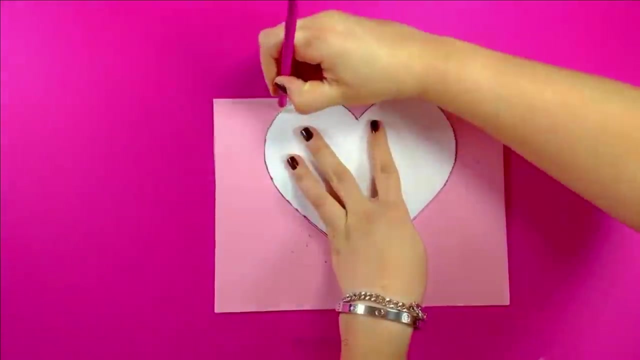 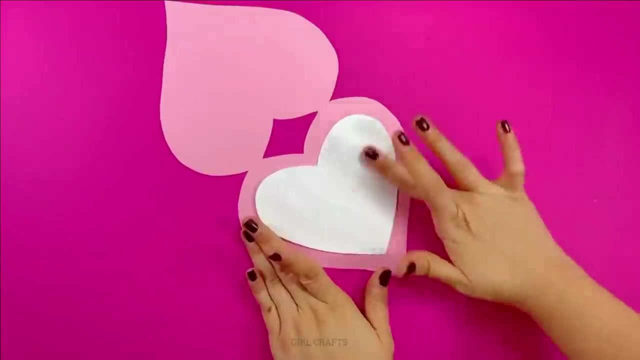 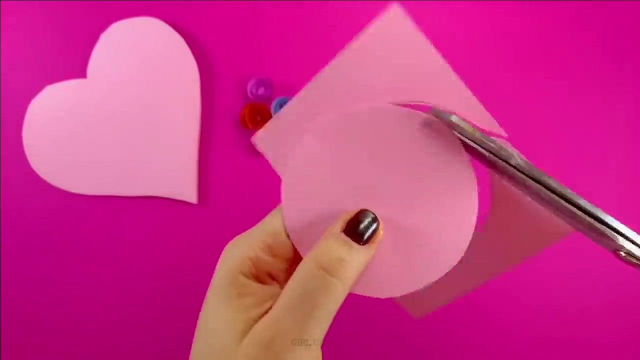 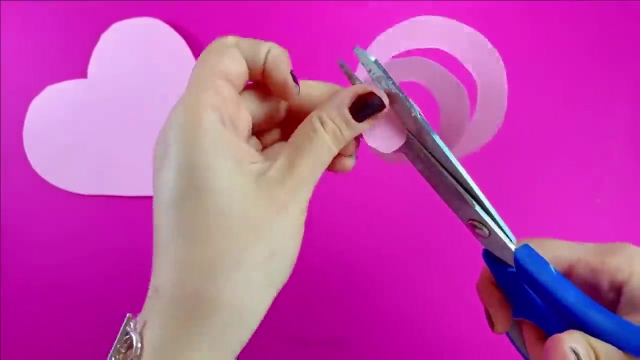 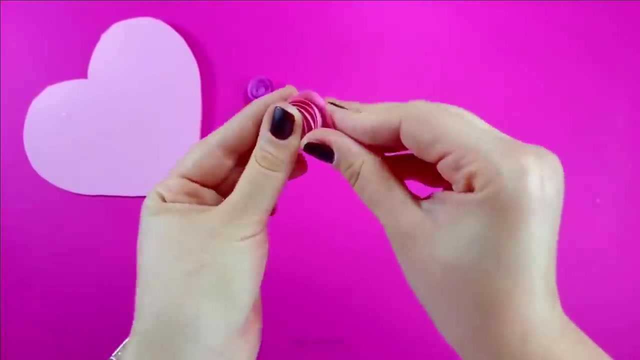 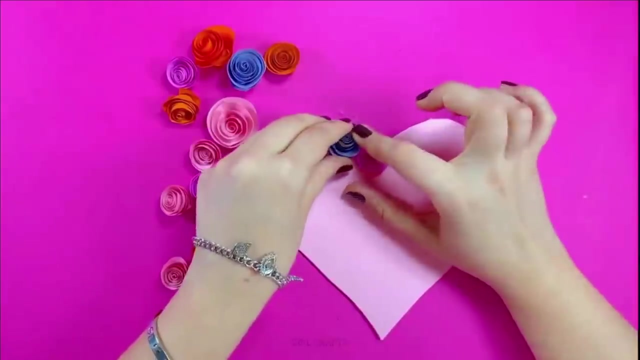 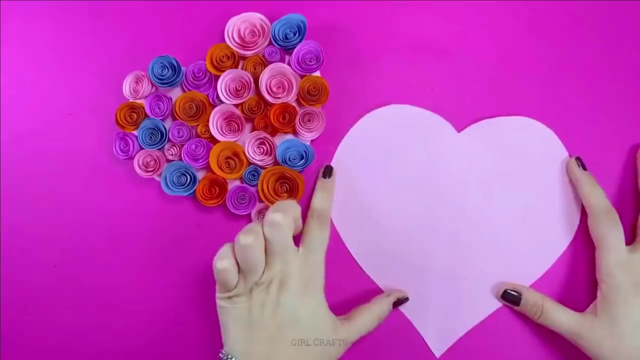 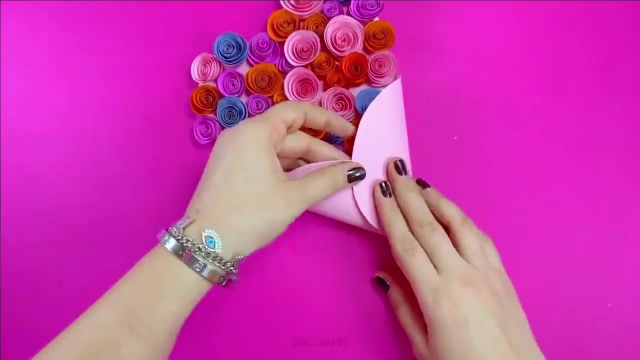 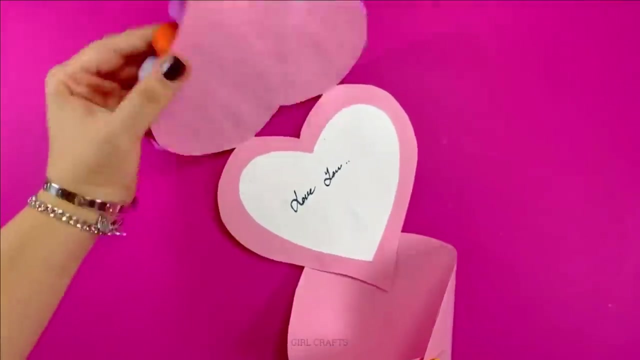 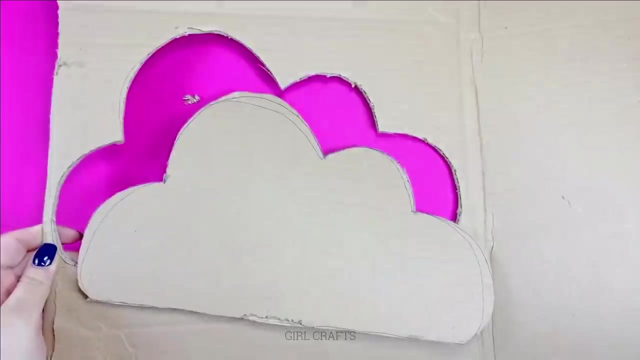 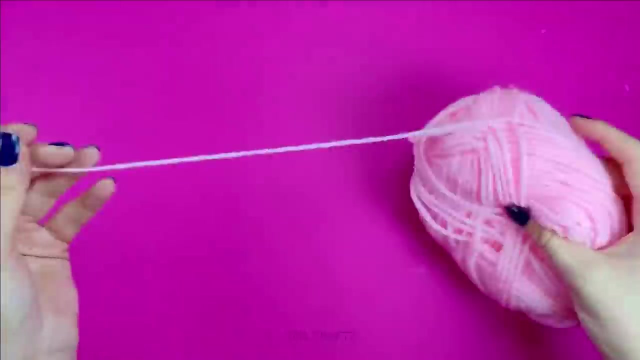 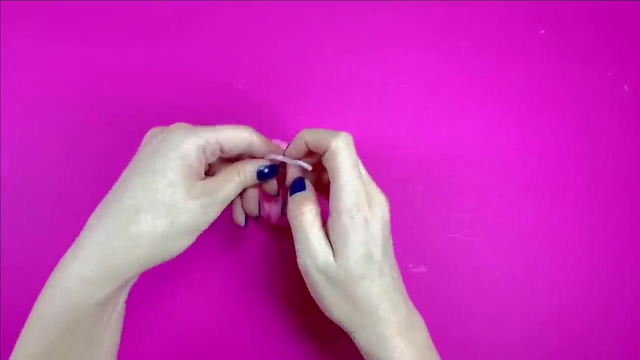 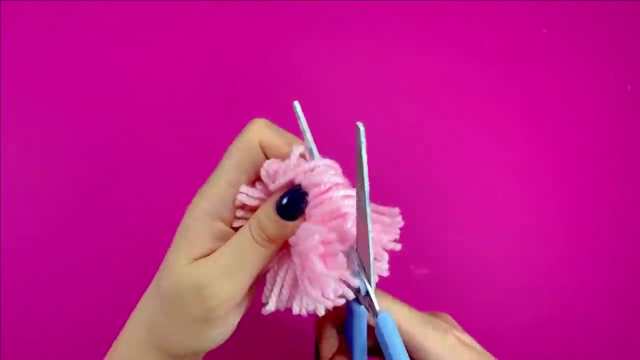 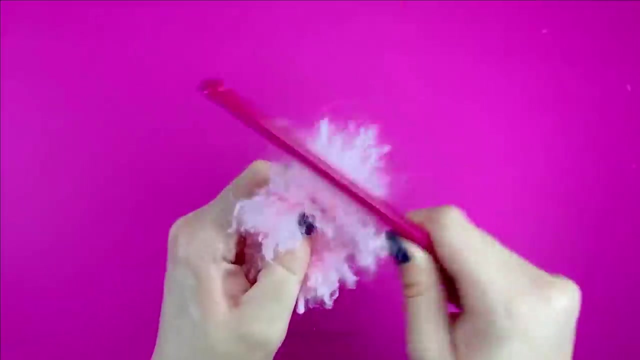 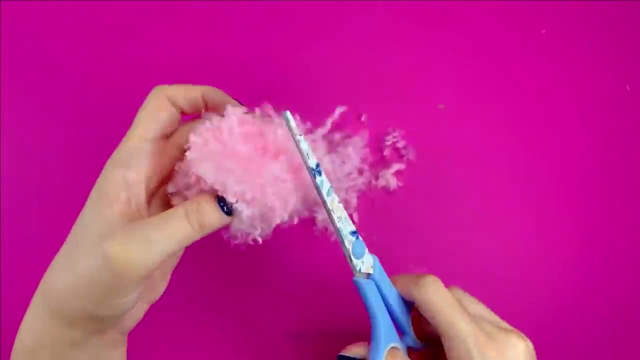 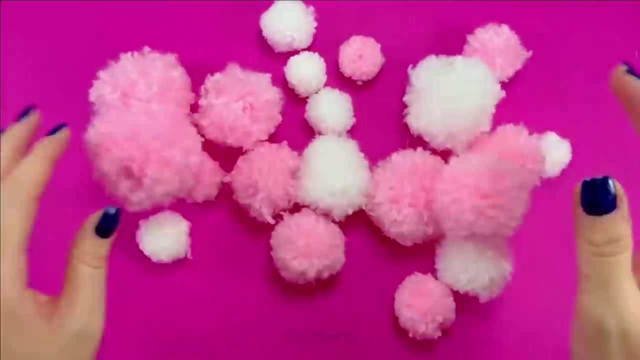 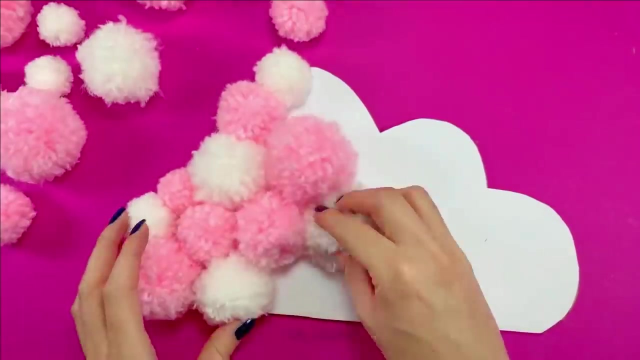 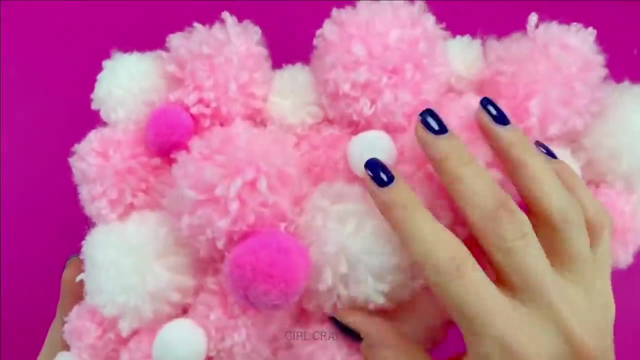 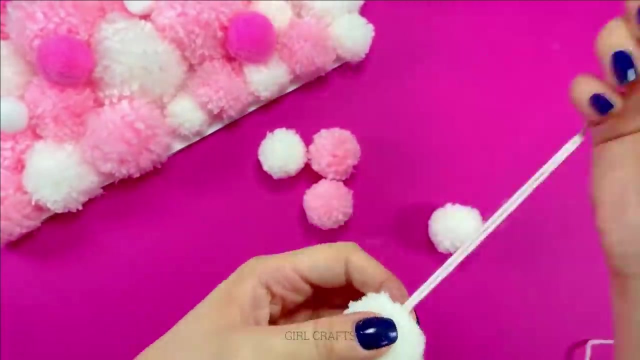 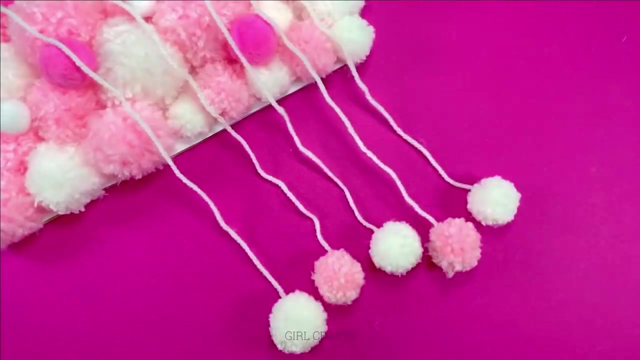 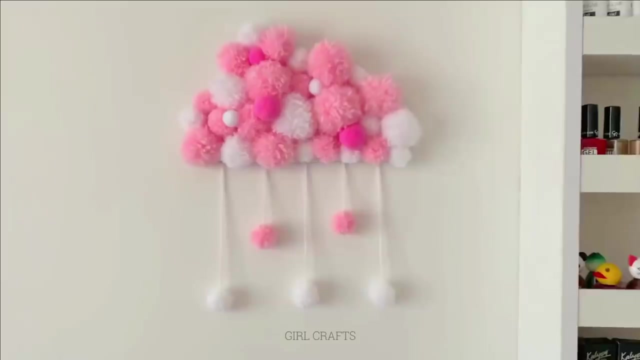 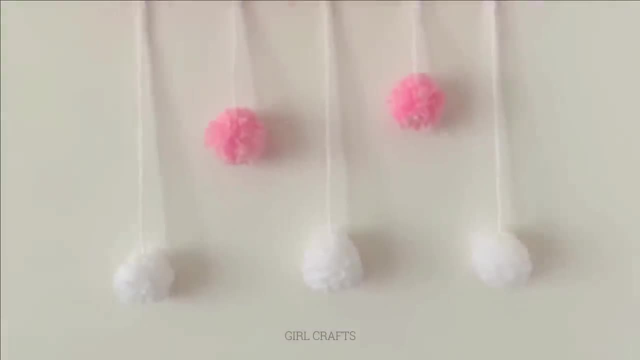 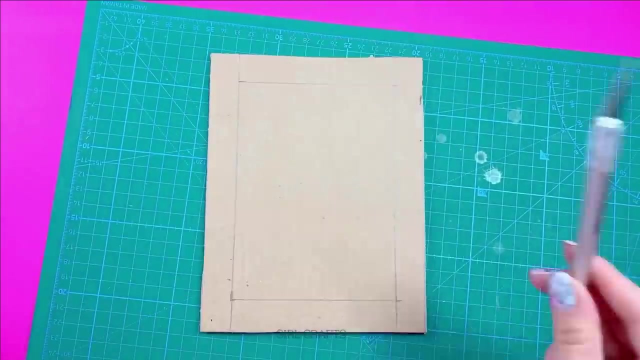 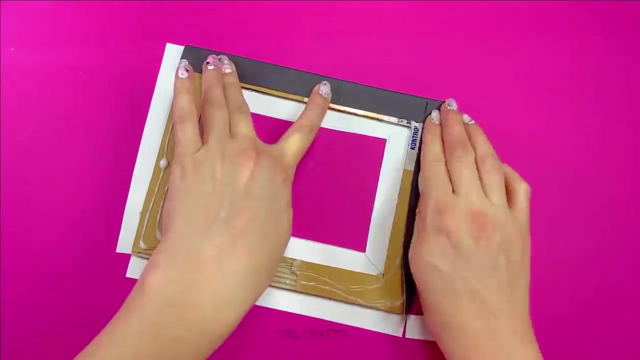 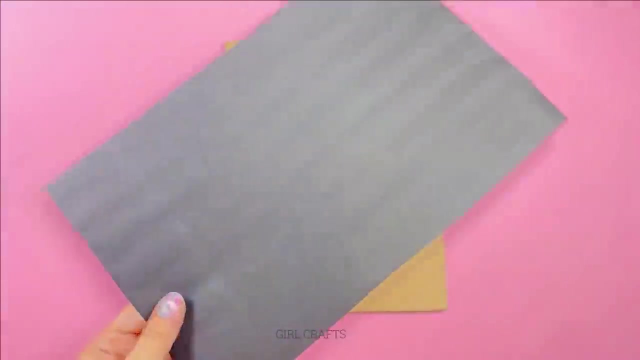 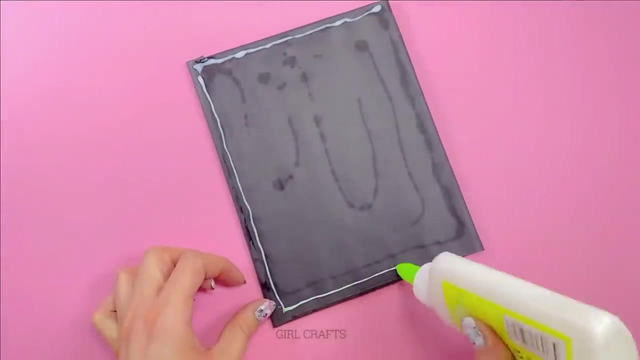 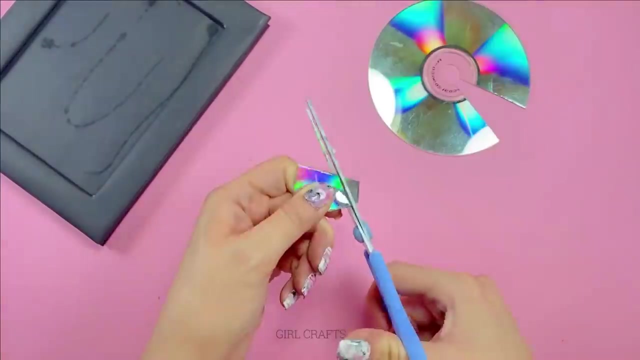 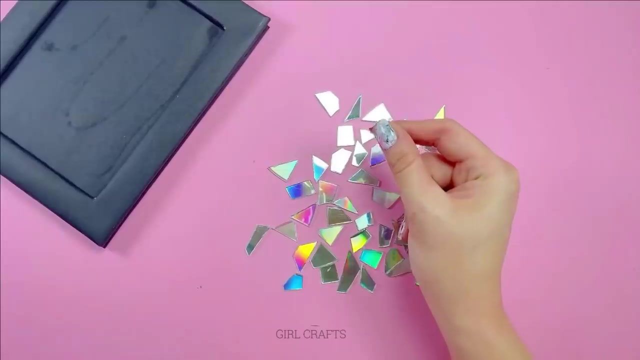 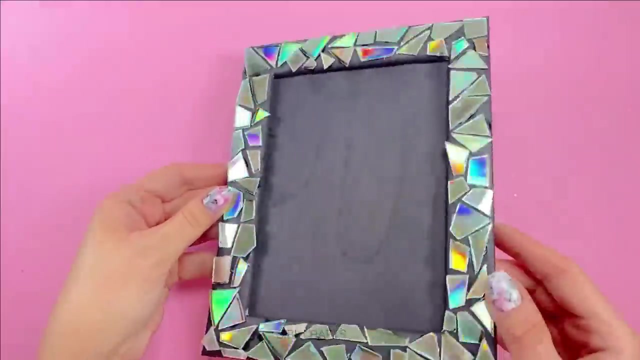 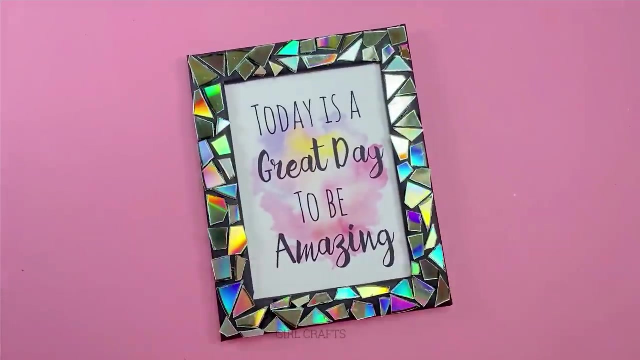 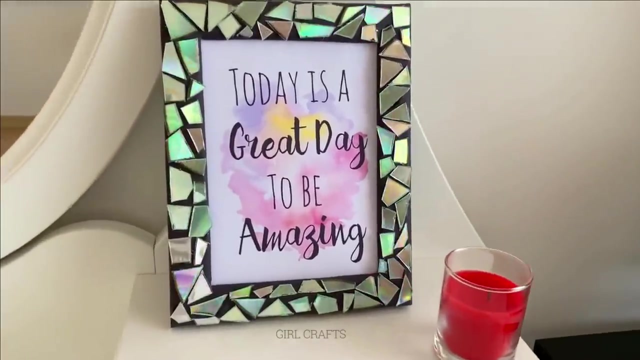 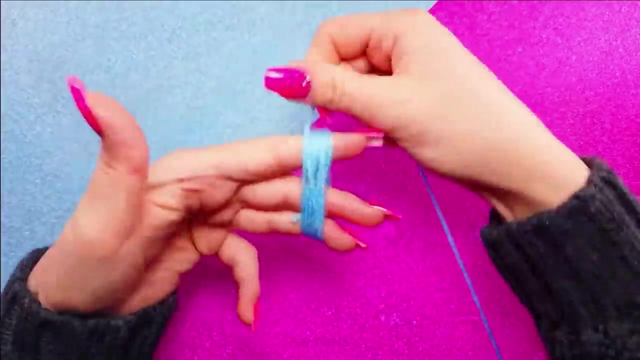 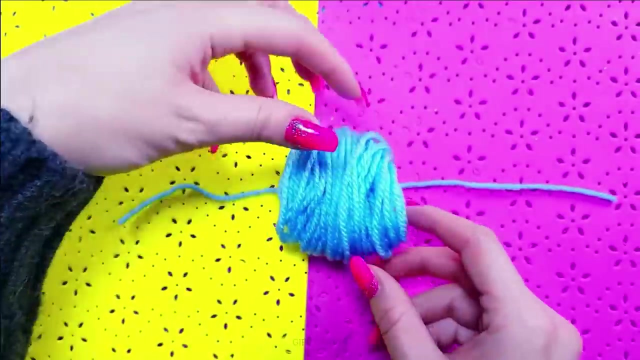 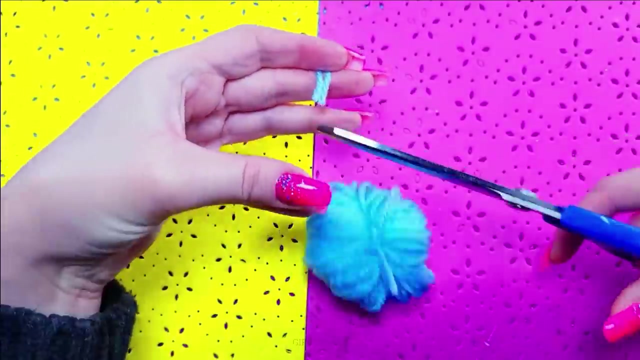 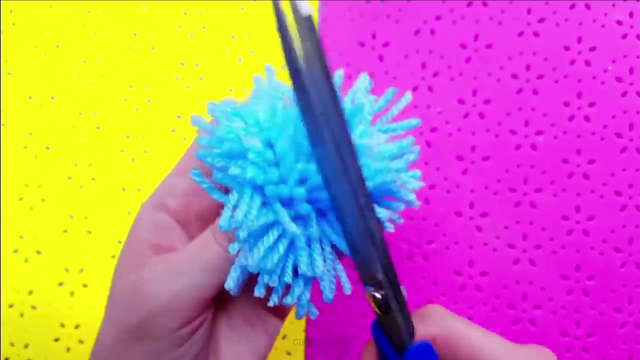 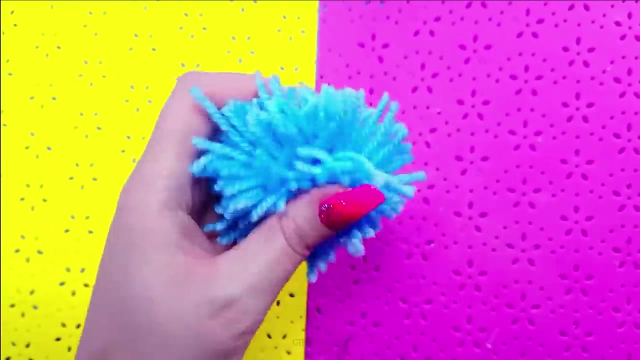 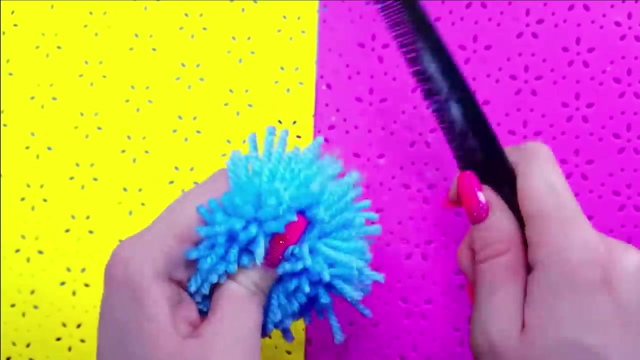 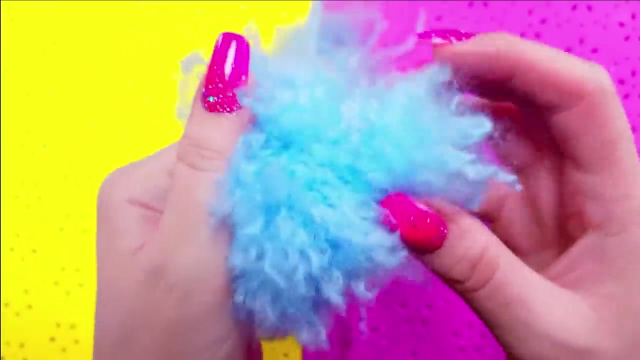 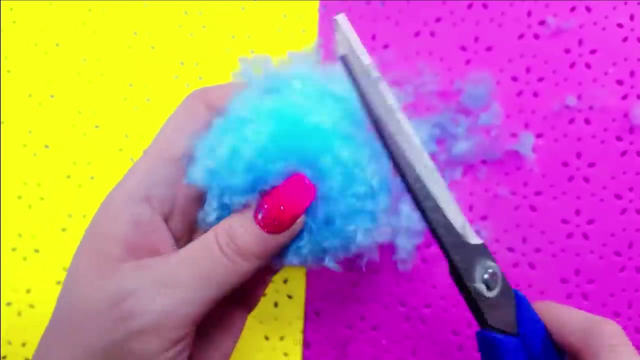 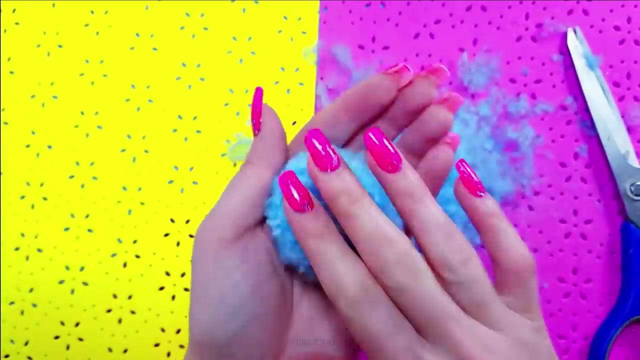 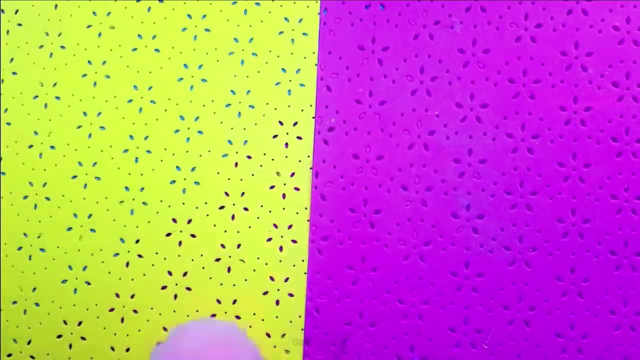 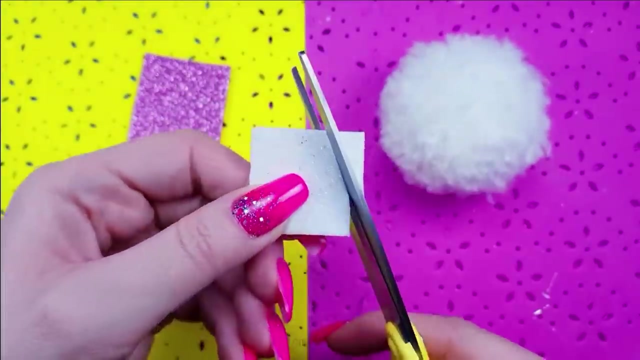 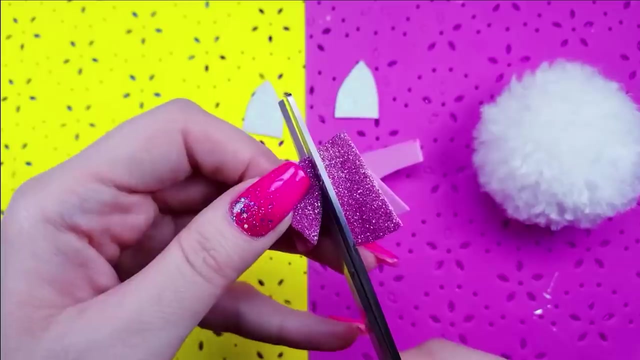 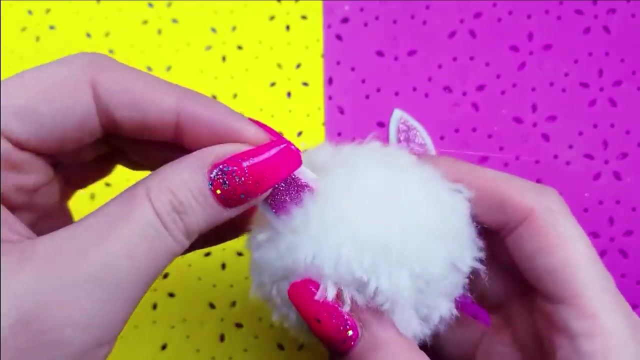 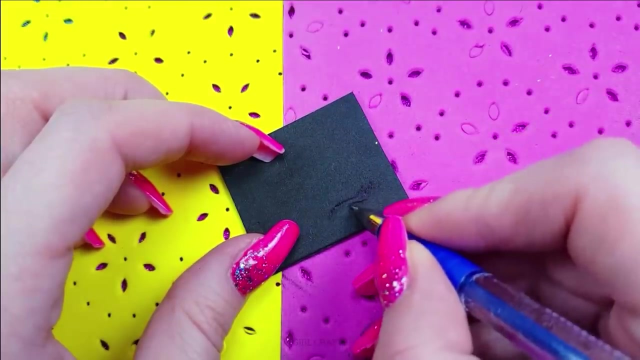 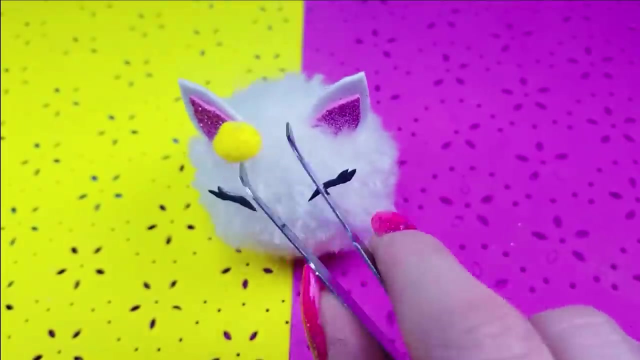 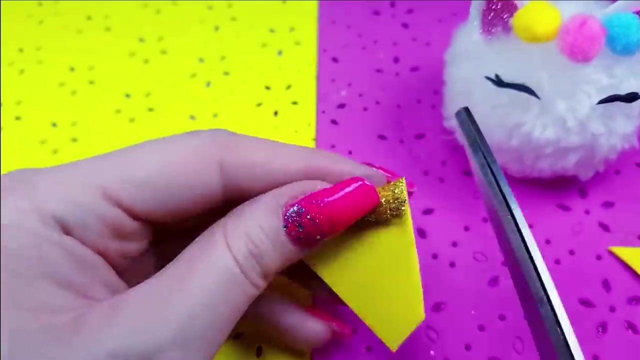 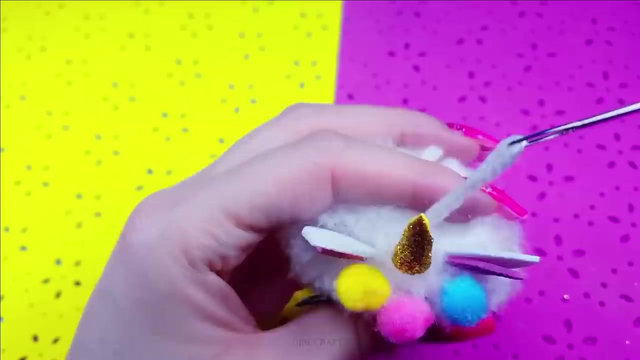 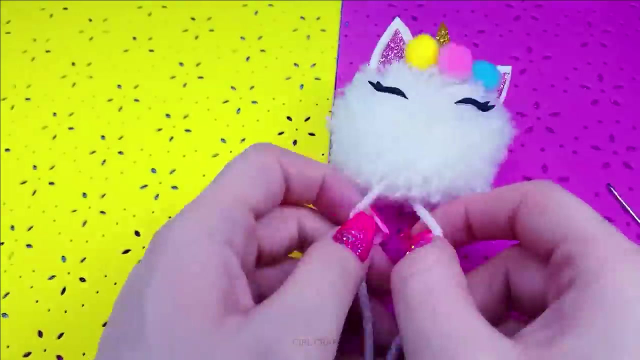 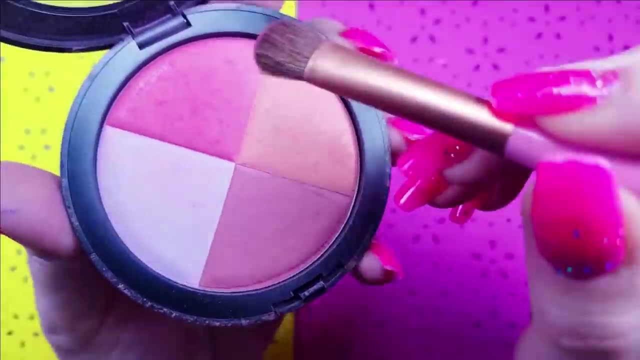 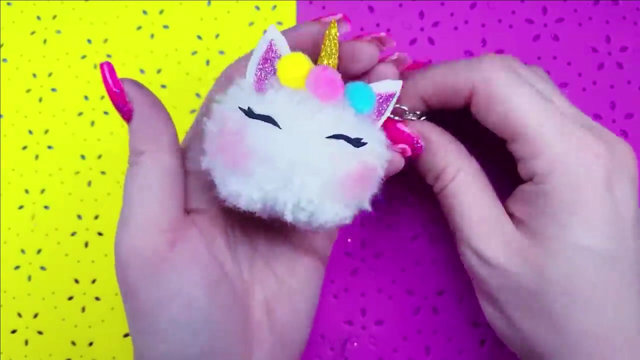 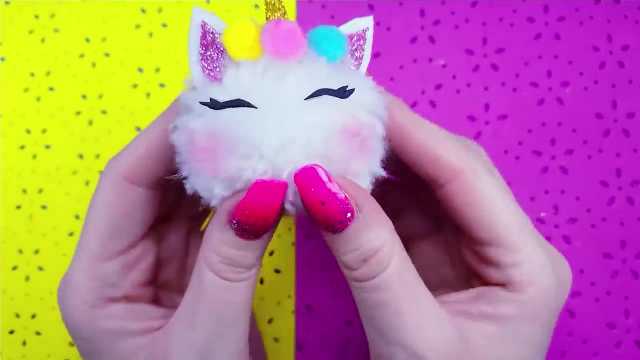 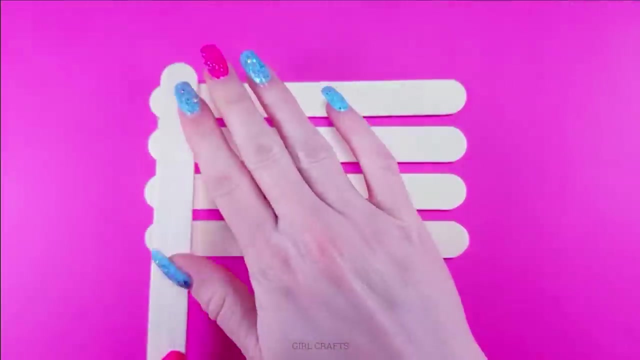 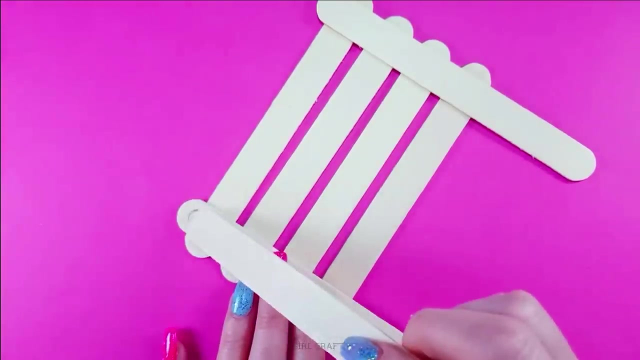 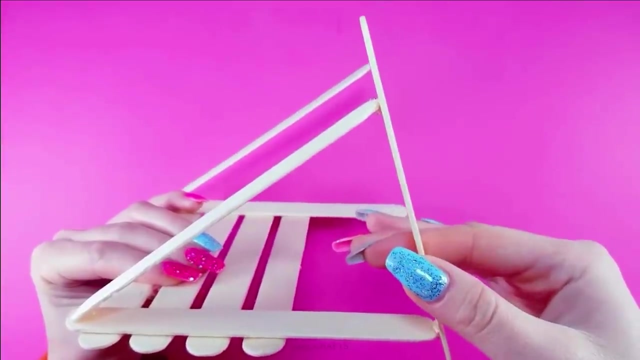 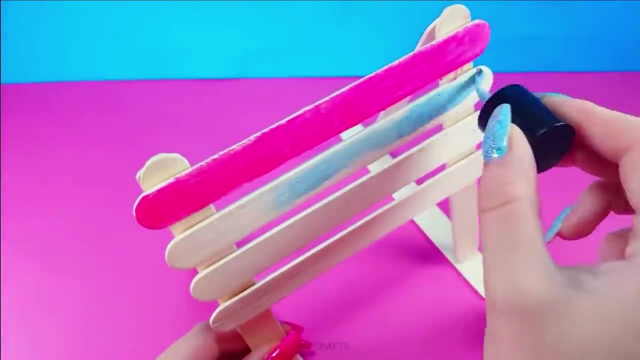 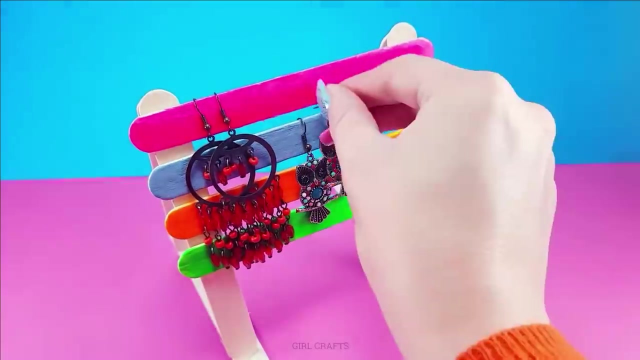 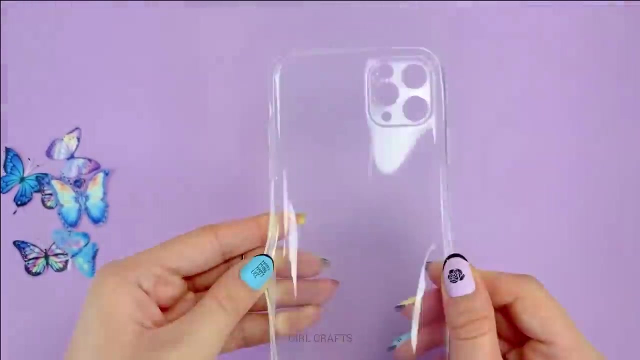 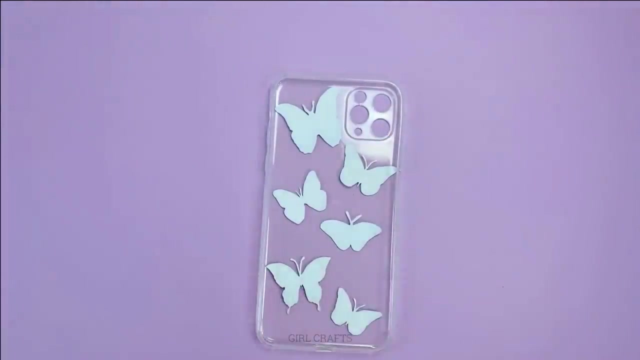 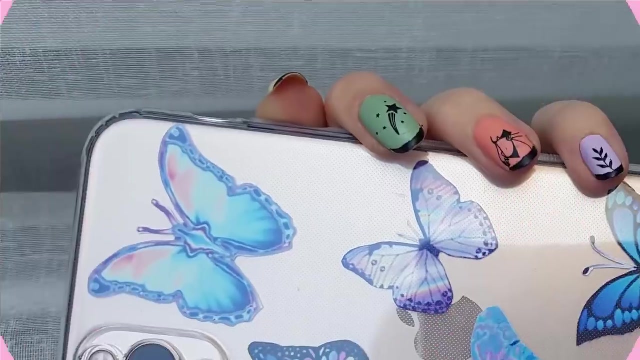 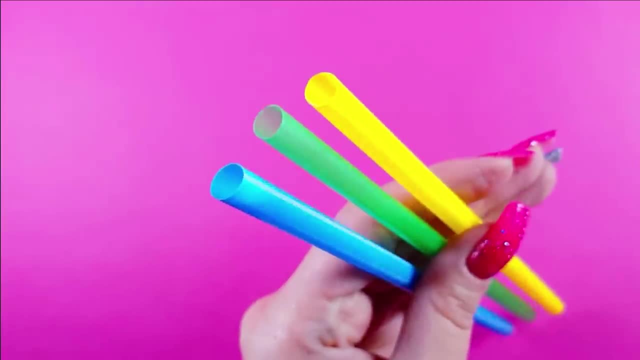 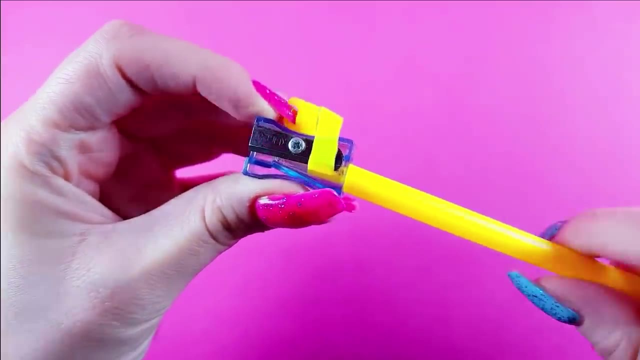 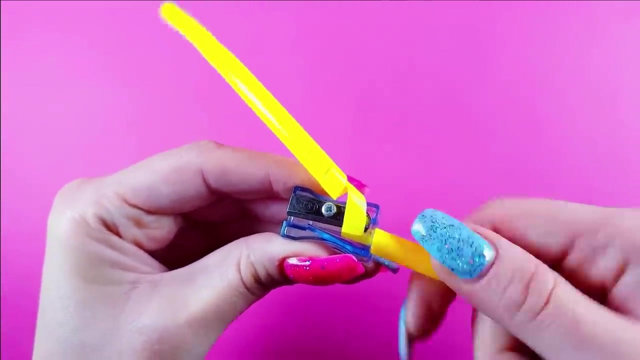 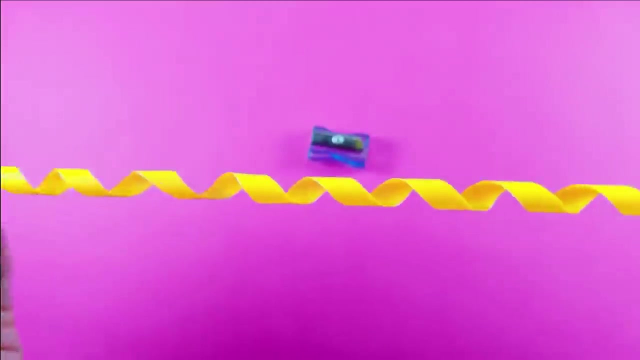 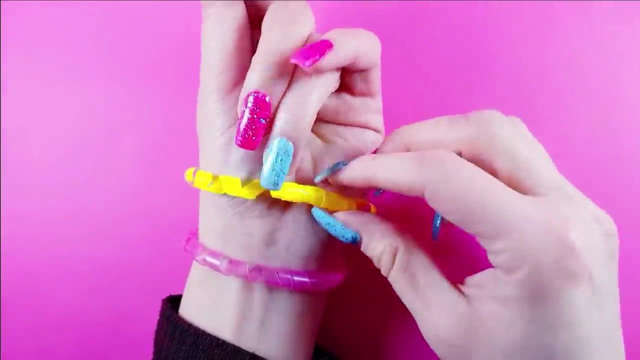 Oh, oh, oh, there's never been anybody. Oh, oh, oh, there's never been anybody quite like me. Nobody looks like me, Nobody sounds like me. Nobody's absolutely the one and only me. Nobody looks like me, Nobody sounds like me, Nobody's absolutely the one and only me. 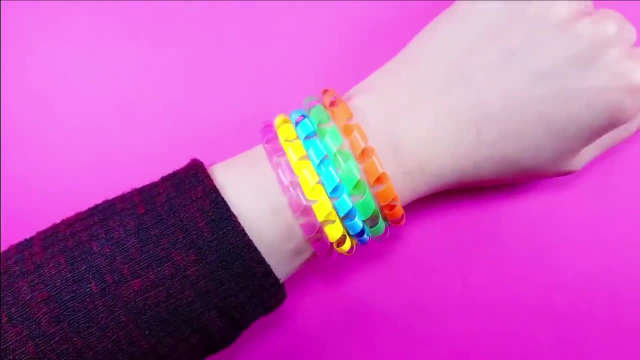 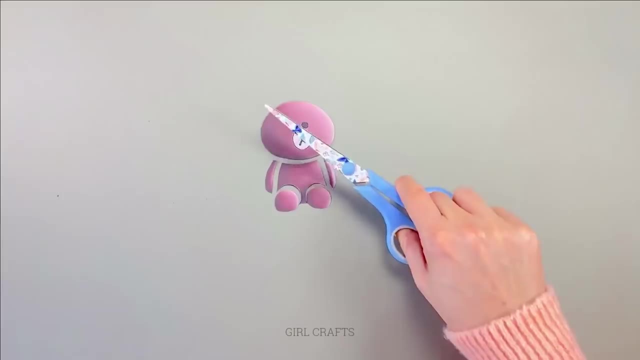 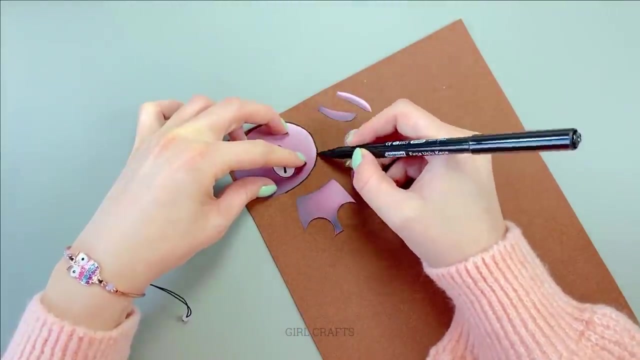 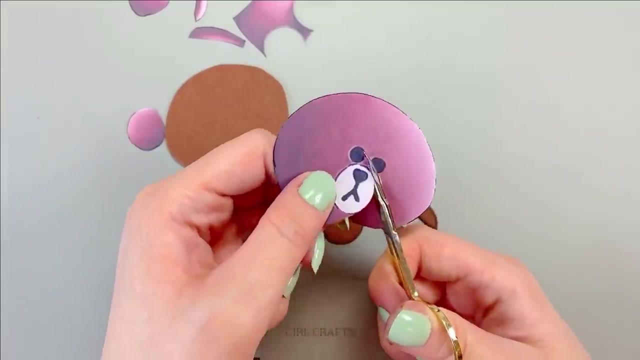 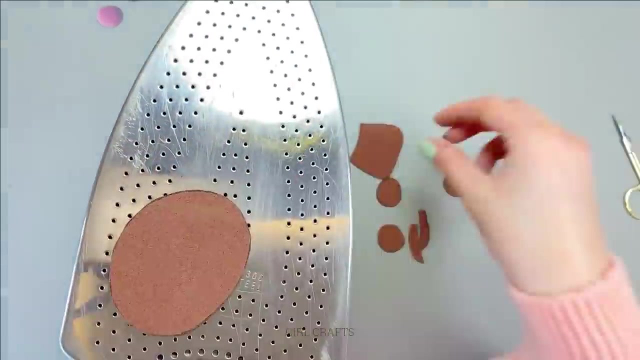 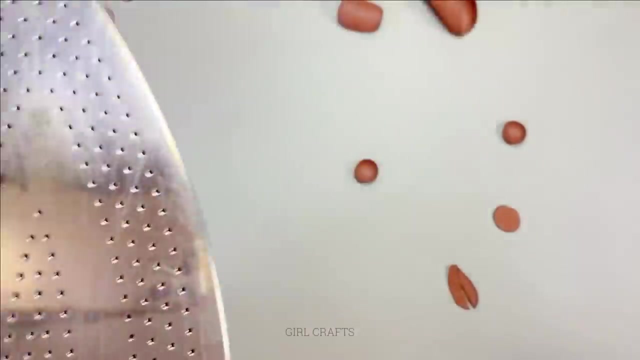 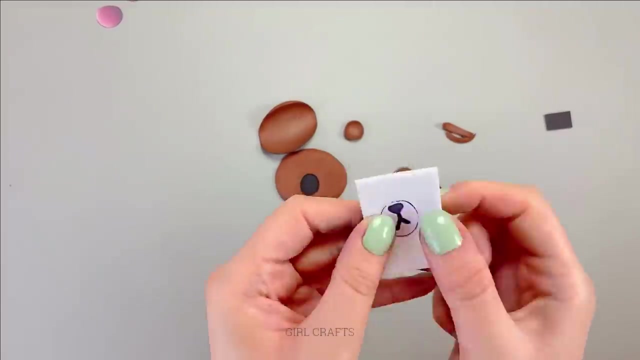 Nobody looks like me, Nobody sounds like me, Nobody's absolutely the one, and only me. The trees arched over the road like a warm embrace, Stripes of shadows all across your face. You hear a sound up in the distance, A rumble and a flash of light, and you stop there. 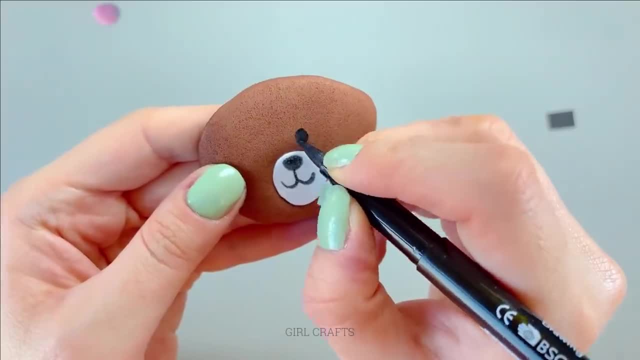 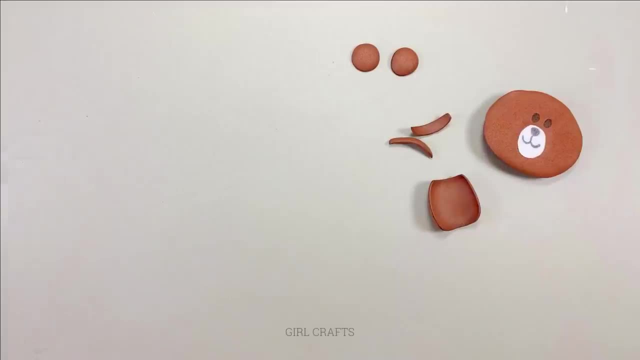 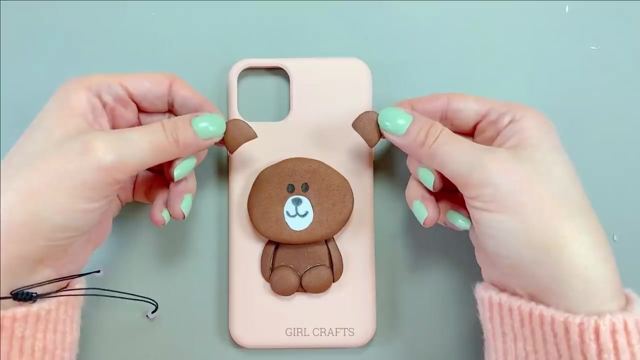 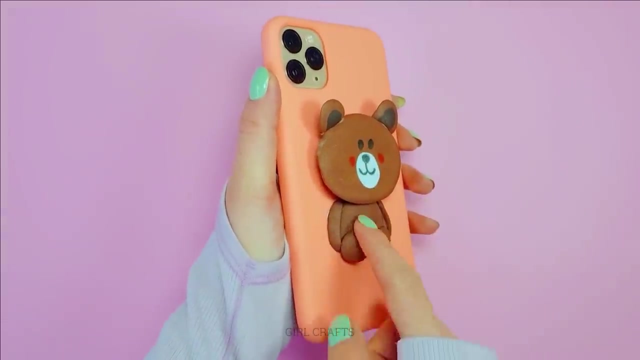 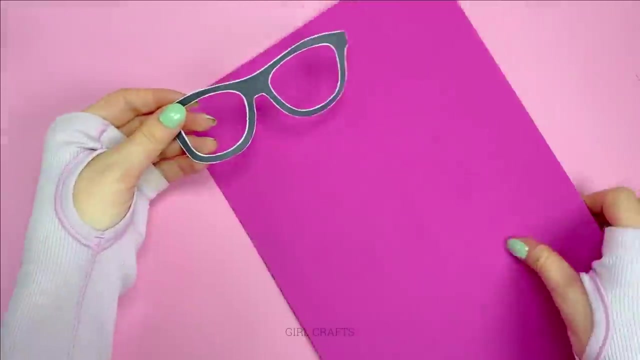 Nothing and you don't know why, Even though you've been praying for sunshine, Sometimes you know it's still gonna rain. Put a smile on and say it's alright, You don't mind it, No, you're not afraid. Not afraid to go out in the rain. 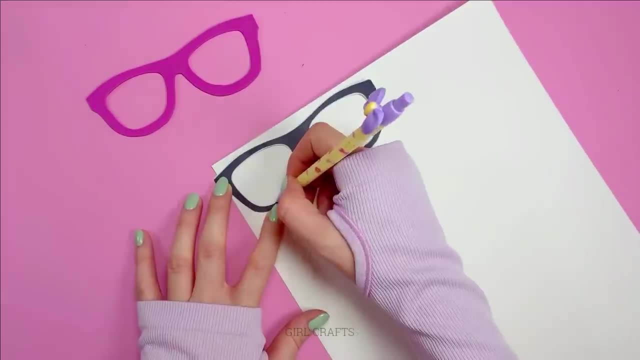 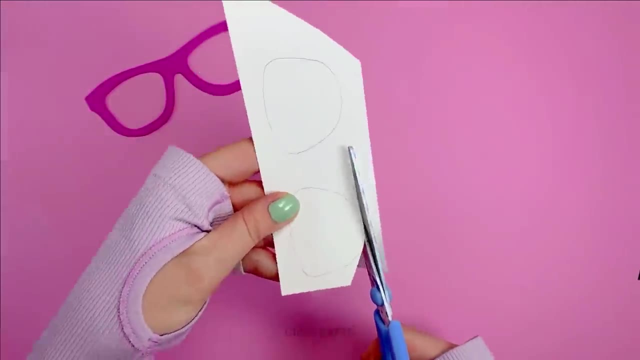 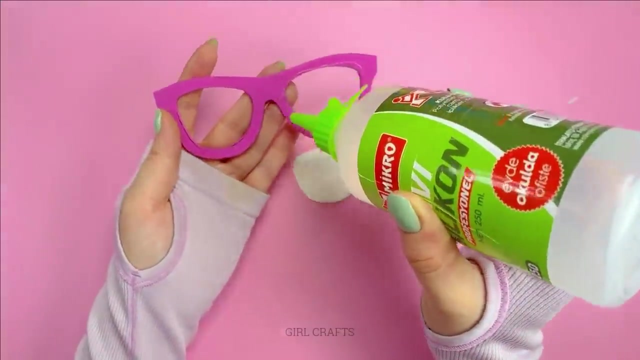 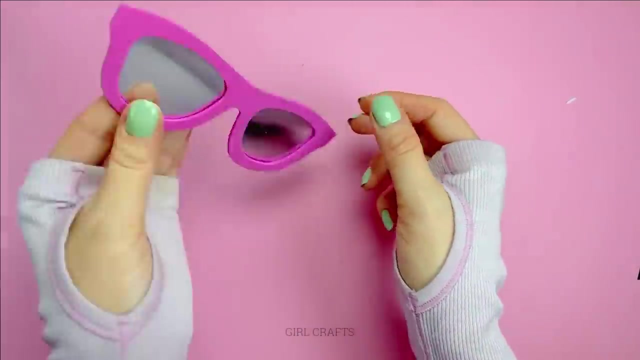 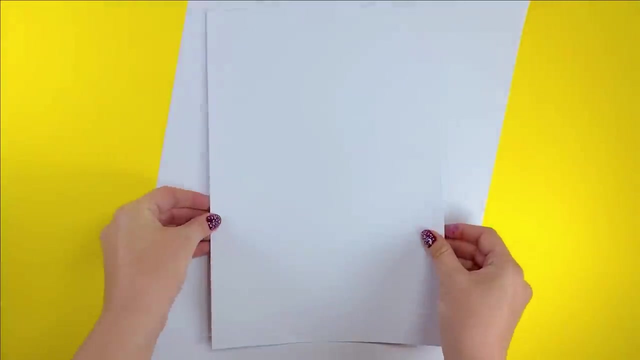 Ooh, ooh, ooh, Not afraid to go out in the rain. Ooh, ooh, ooh, Your blue jeans covered in mud Shoes, all in your hands. All this water wasn't in your hands, Didn't work the same without you. But when the devil sets too many fires, God is gonna send some rain and he'll be laughing. 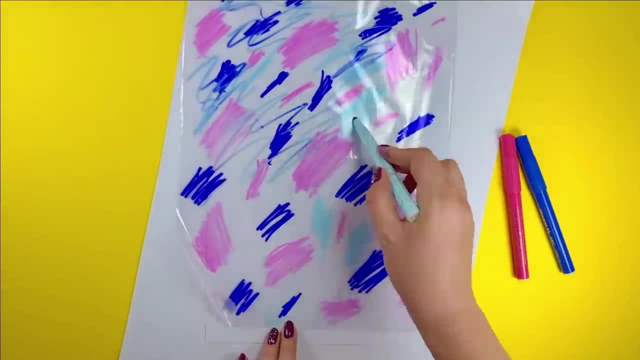 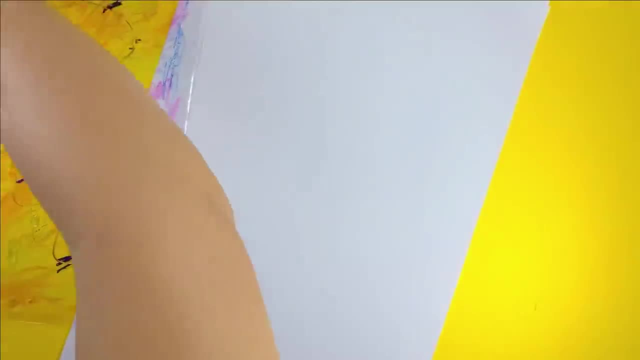 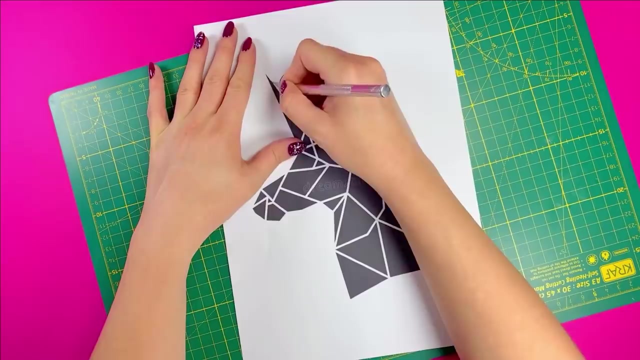 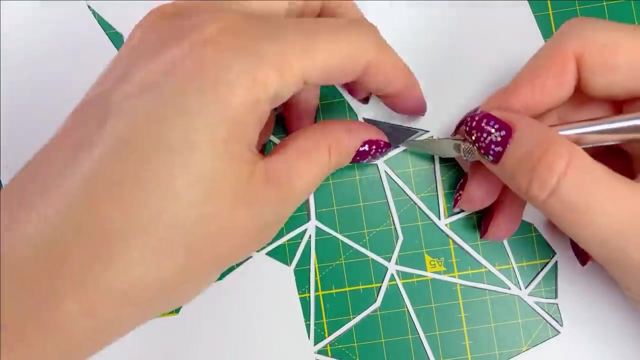 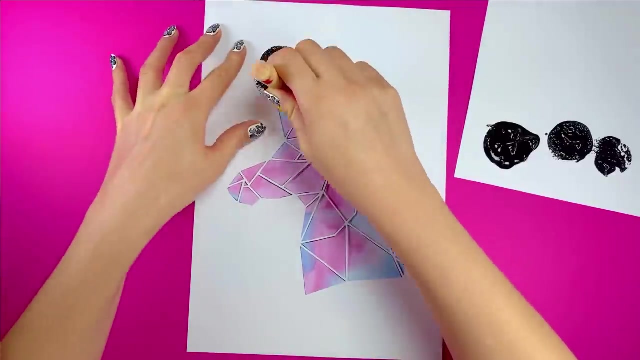 And you won't know why, Even though we've been praying for sunshine, Sometimes you know it's still gonna rain. Put a smile on his head, it's alright, You don't mind it. no, you're not afraid. Not afraid to go out in the rain. 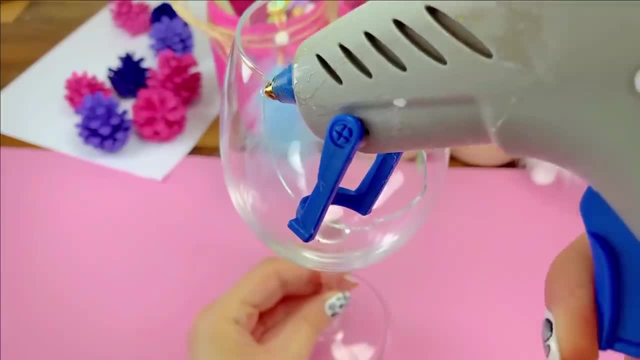 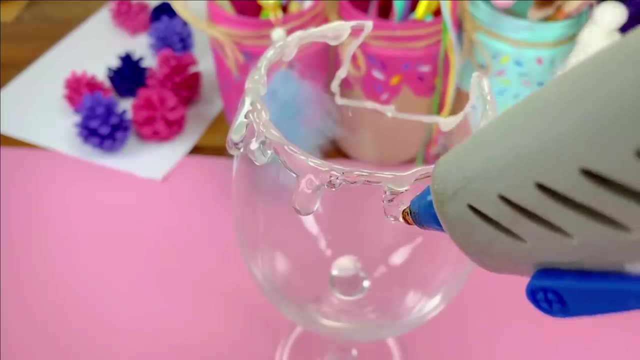 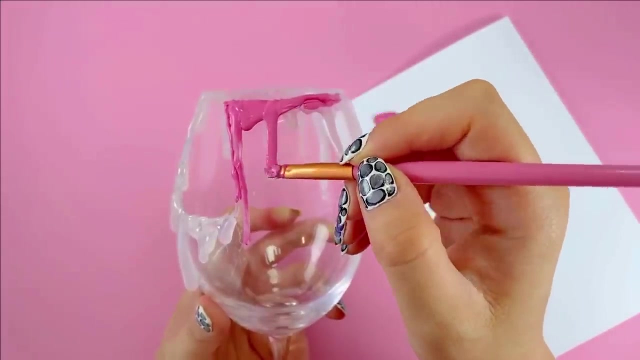 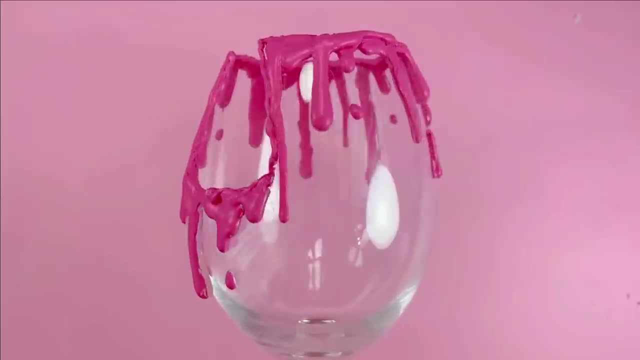 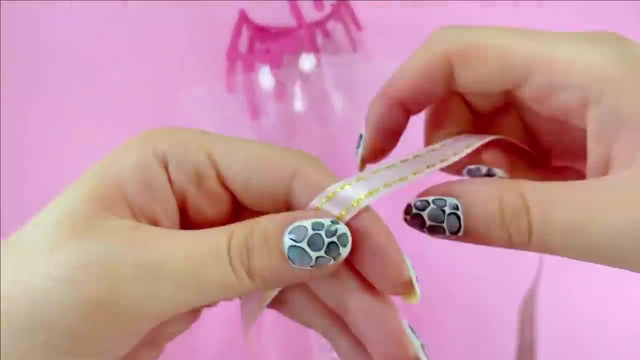 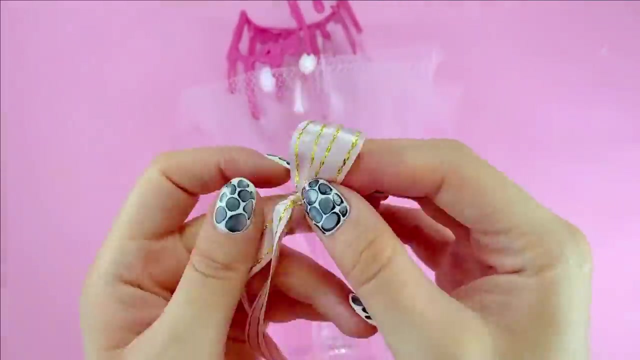 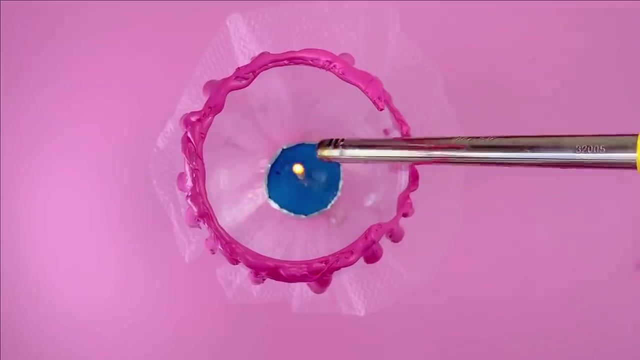 Even though we've been praying for sunshine Sometimes, you know it's still gonna rain. It's still gonna rain. now, Put a smile on his head. It's alright, You don't mind it. no, you're not afraid. Not afraid to go out in the rain. Not afraid to go out in the rain. 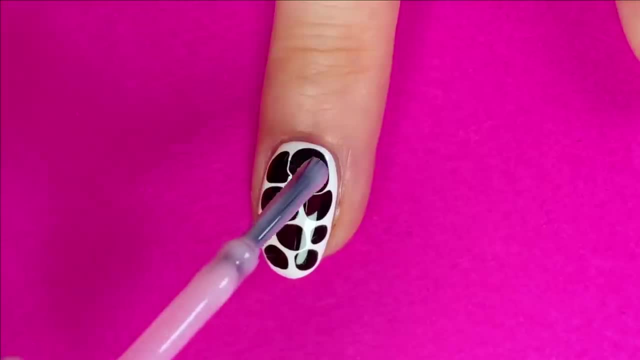 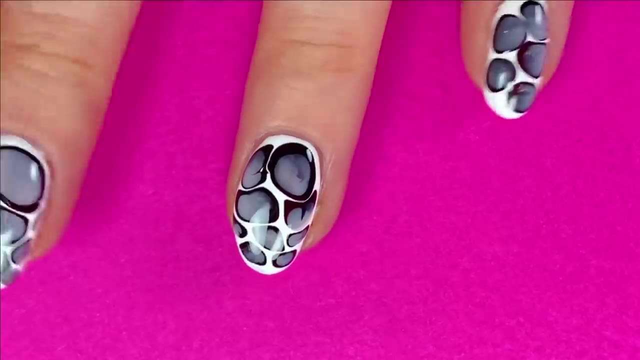 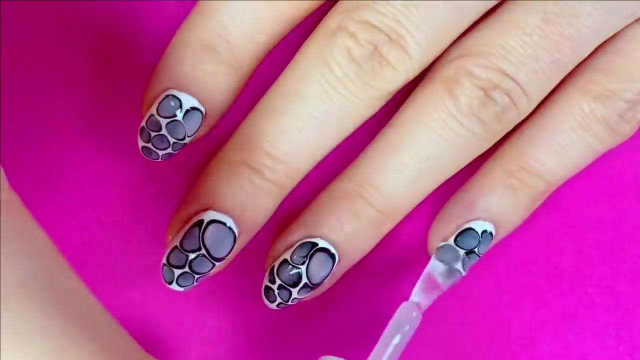 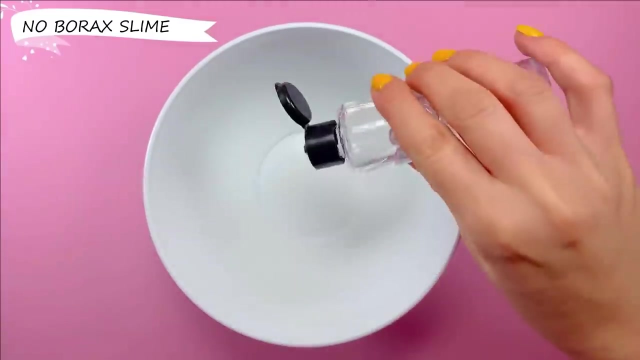 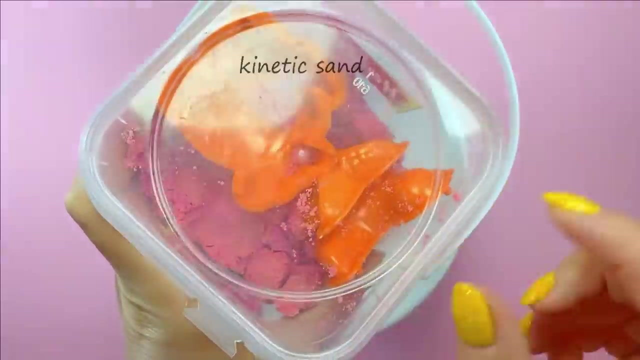 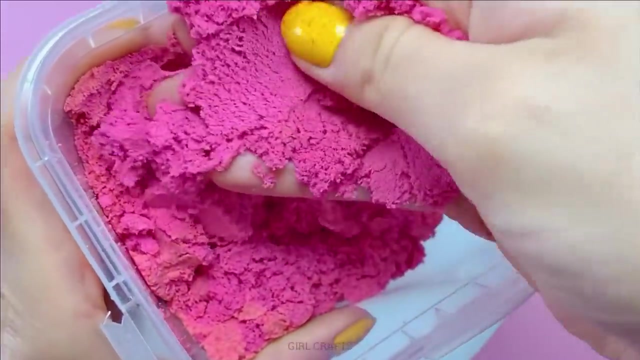 It's alright. Red, orange, pink and blue: You brighten up every room. Your smile is like no other. With you, it always feels like summer. You bring a little pop of color. You bring a little pop of color. You're the shiniest star. 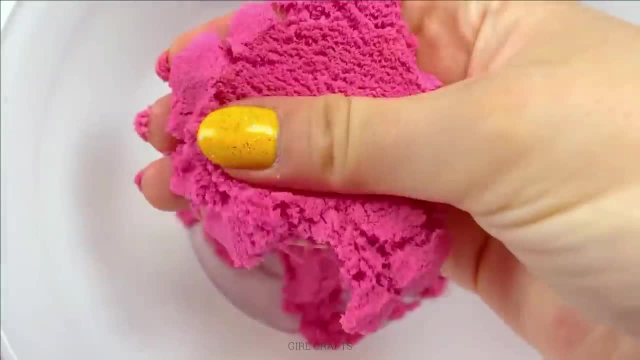 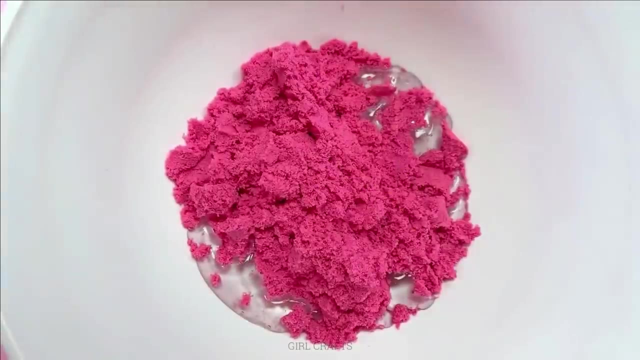 It's always bright in where you are. Oh, what a sight to see. I'm caught up in the joy you bring. So take it all to the streets And share your heart with everyone you meet. Take it all to the streets And share your heart with everyone you meet. 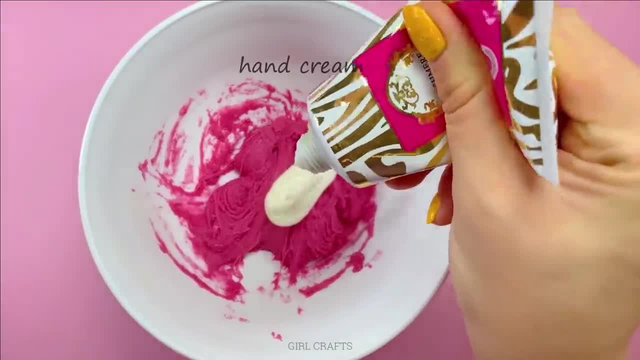 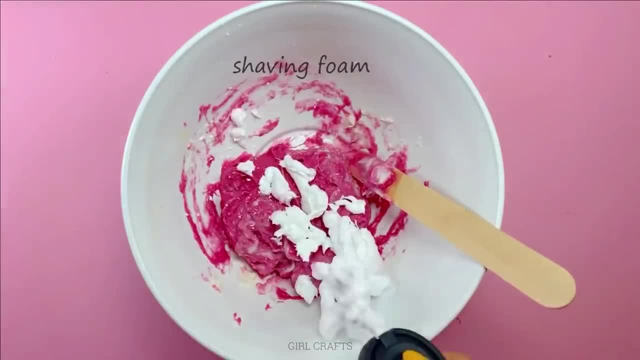 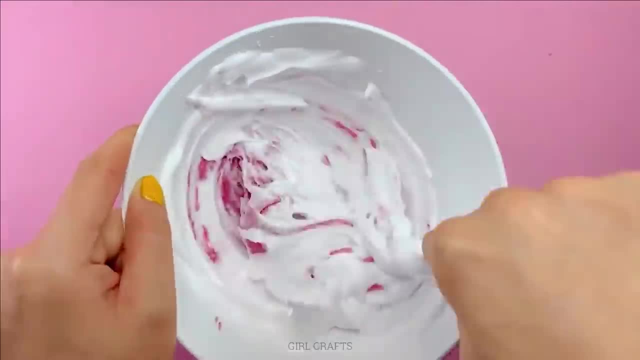 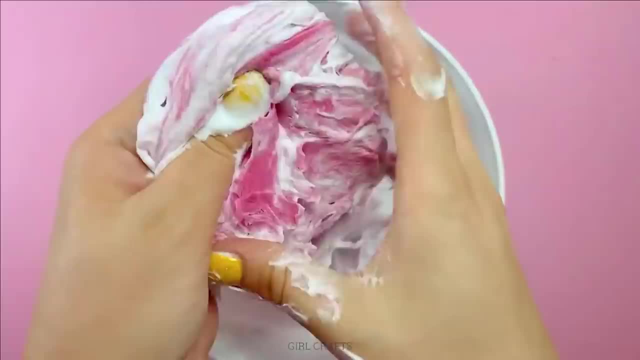 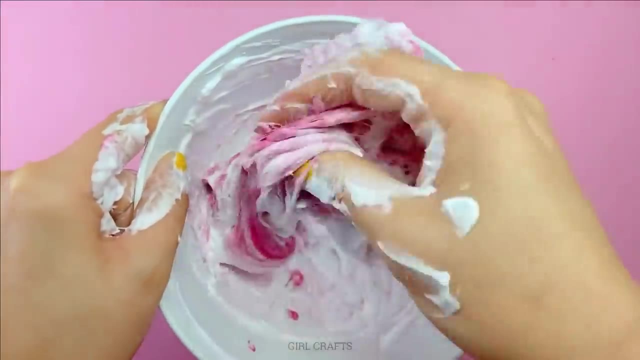 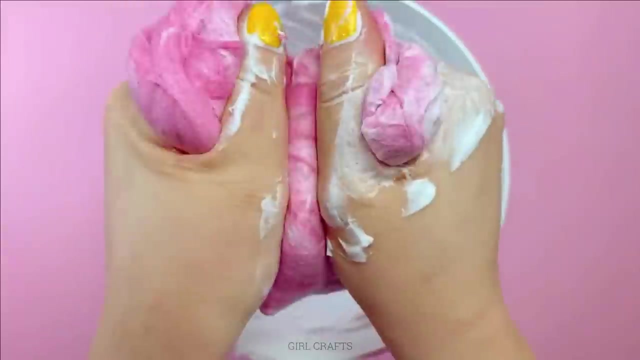 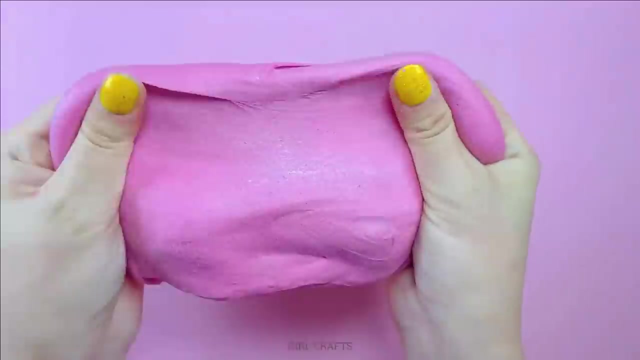 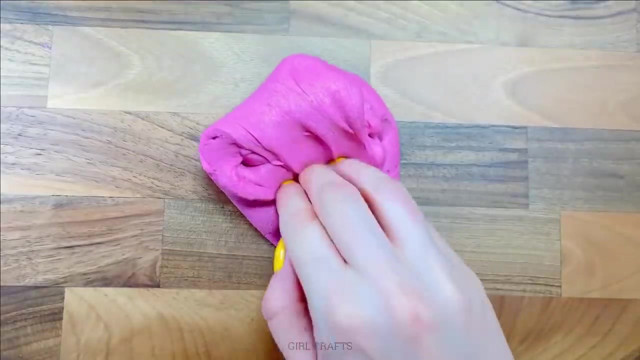 Pop, pop, pop, pop, pop the coffee. Pop, pop, pop, pop the coffee. I'm bringing it all into view. I just can't get enough of you. You bring a little pop of color. You bring a little pop of color When you smile. it feels like summer. 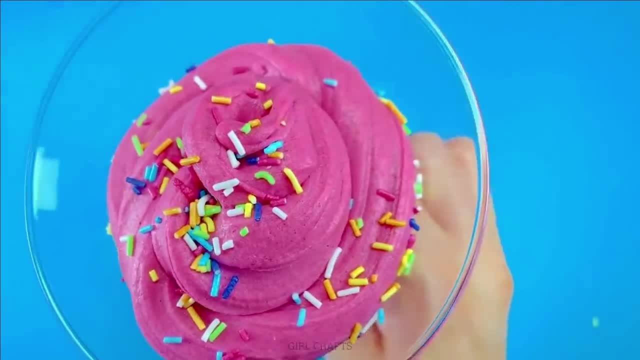 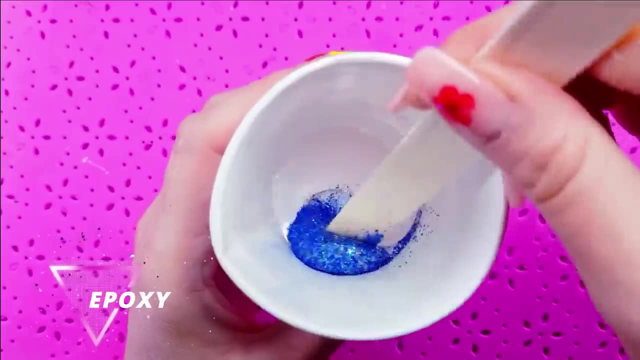 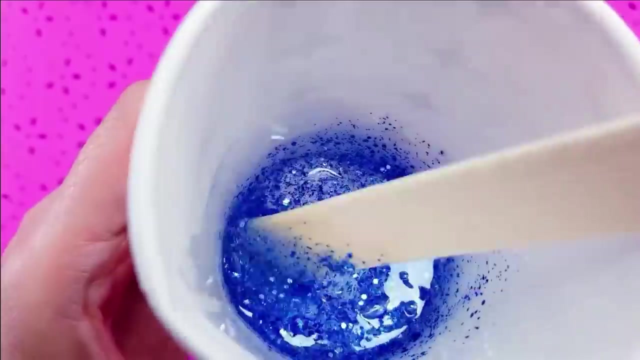 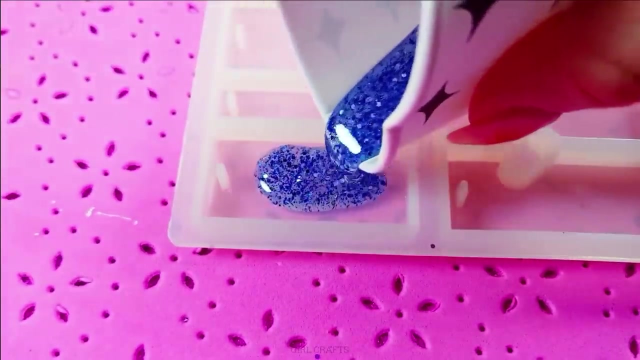 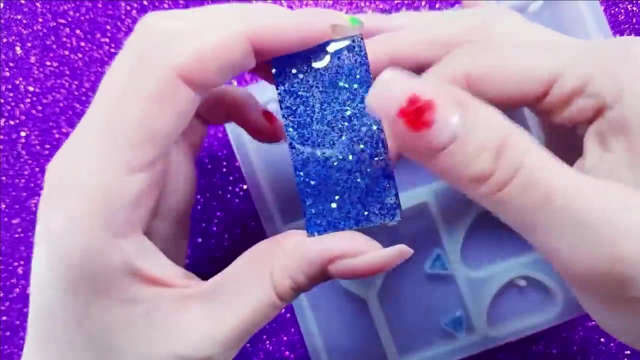 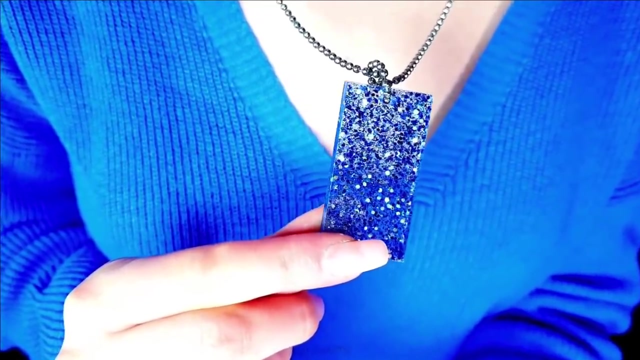 You've got a heart that's like no other. You bring a little pop of color. When you smile, it feels like summer. You've got a heart that's like no other. You bring a little pop of color. You bring a little pop of color. I cannot recall my age. But I can certainly still taste The feeling good of summer. I can't wait to see her. We're driving to the countryside. The sun was always blazing high. Nothing any better than when I was with her. Why couldn't it have lasted forever? Take me back to Piggyback. 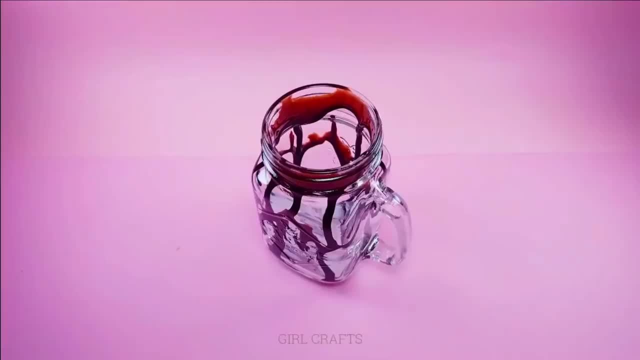 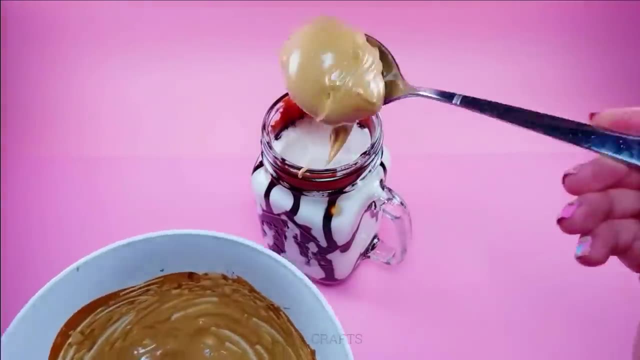 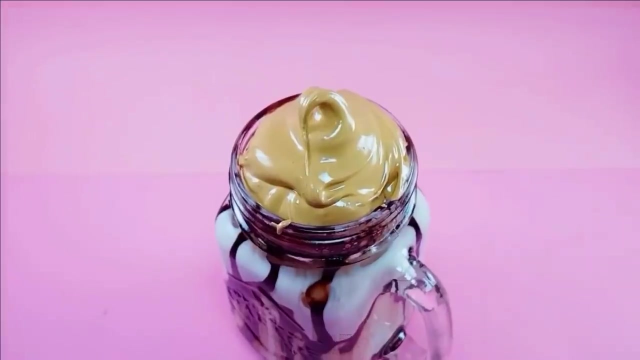 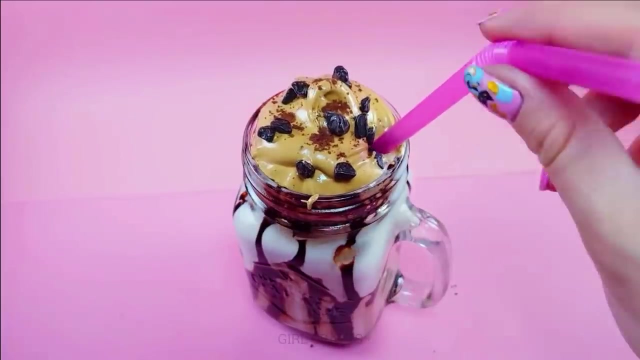 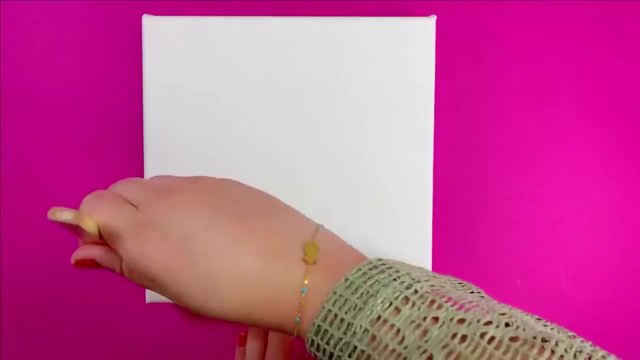 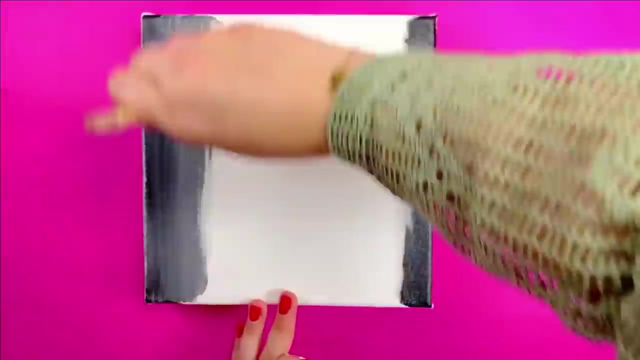 To Peking Peaches, Where the winding road goes on and on and on. Take me back to Peking Peaches, Where nothing will grow old and Nothing will go bad. What happened to the shade it broke And the simplest of what it took To fill the holes within me so that I can run free.